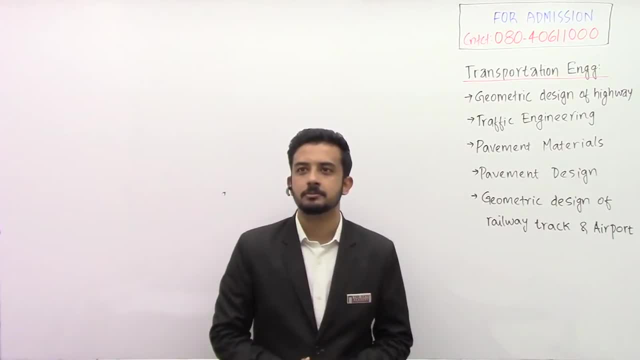 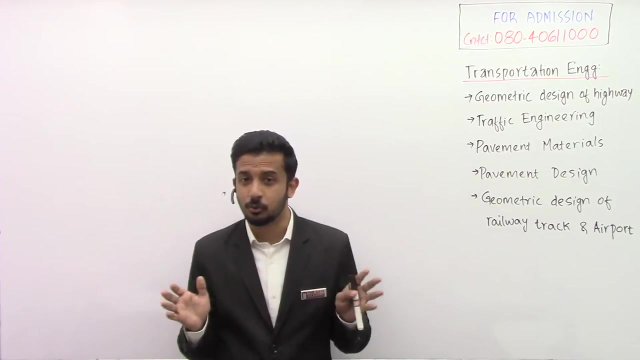 Hi friends, A very good morning to all of you. Welcome to this live session from the GATE Academy. Today we'll be having a small discussion regarding our transportation engineering subject From GATE point of view. yeah, actually speaking, transportation engineering is a. 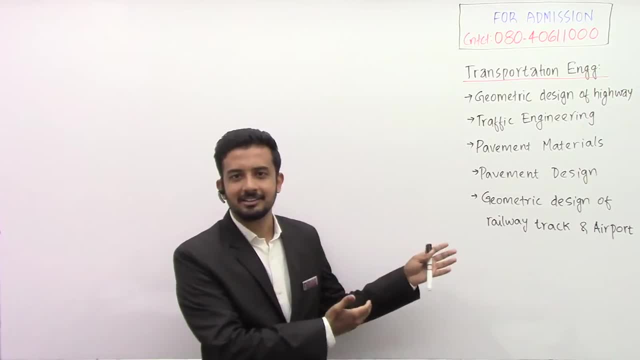 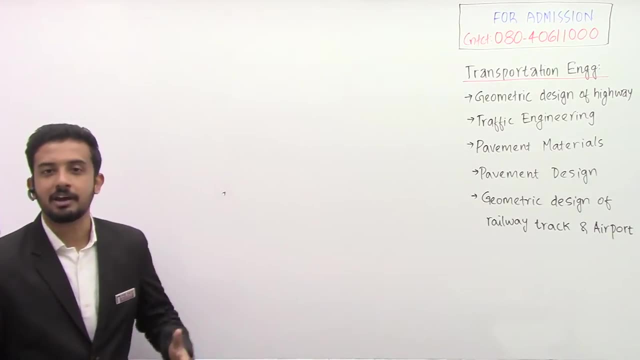 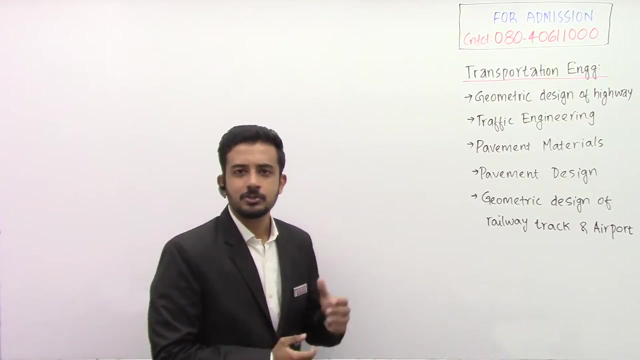 subject: right. See, it involves these chapters according to the GATE syllabus, See geometric design of highway we are having, traffic engineering we are having and the payment materials and the design and the geometric design of railway and airport. So these are the chapters we 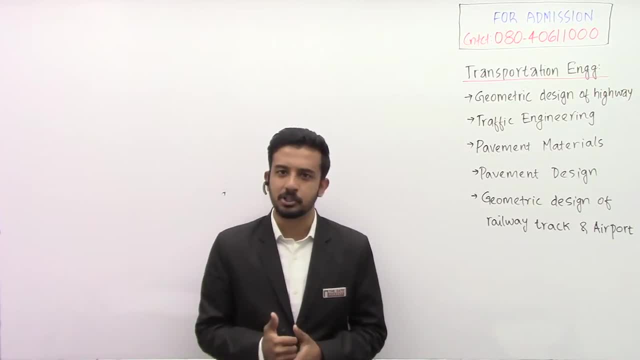 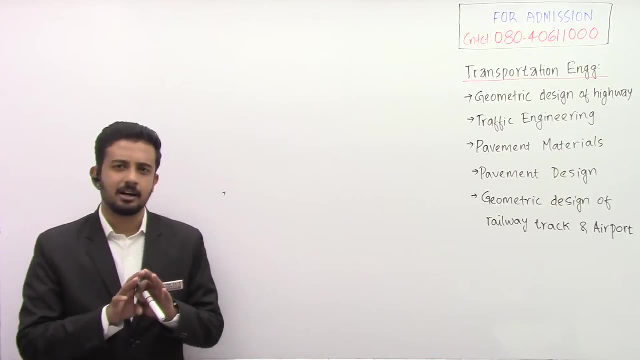 are having for our GATE examination from the transportation engineering subject, right? So you might have already gone through the syllabus and all We know that there will be an average weightage of 10 marks in GATE exam from this particular subject, right? 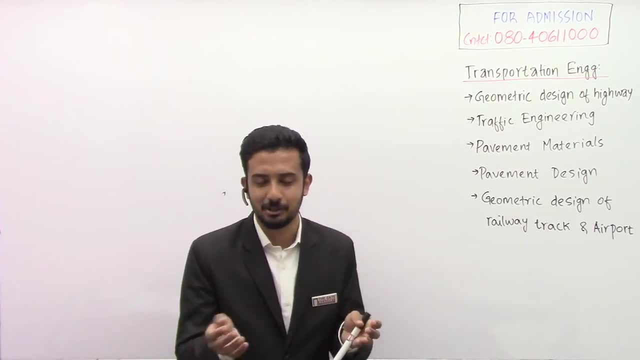 See, a weightage of 10 marks is actually not a silly. I mean, it's not a silly weightage, right, It's a significant weightage. So the importance of transportation engineering is not only the weightage, but also it is easy to score. It's an easily scoring subject. 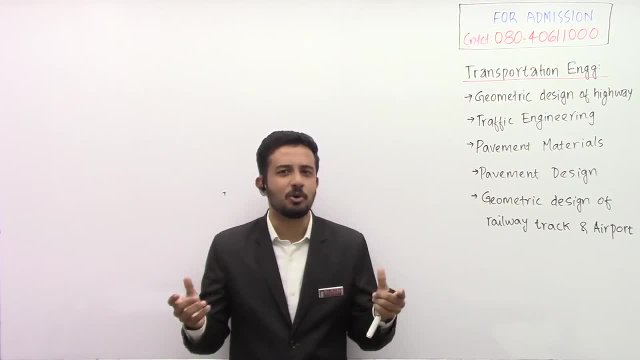 So if you're comparing with the other subjects which are having more weightage, you know the effort you have to put to get that 10 marks from this particular subject is comparatively less Right. So, yes, it's true, The concepts are more or less simple compared to other. 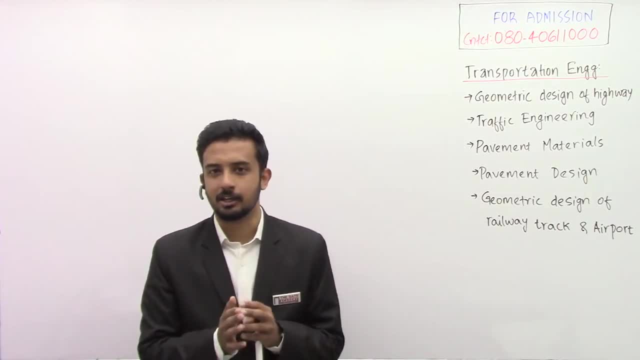 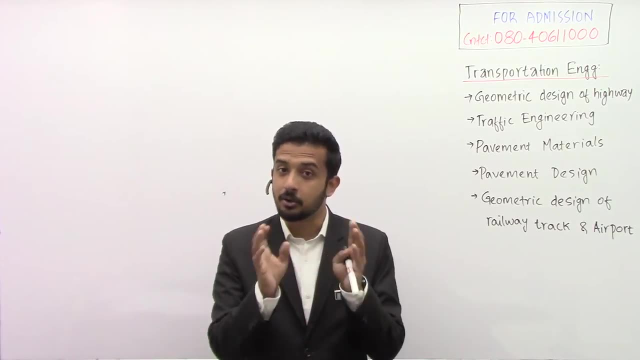 subjects. But the thing is, they can ask the questions like anything. A variety of questions can be asked, Or they can simply use two, three words in the question so that the contest is going to change, The answer is going to be changed And they will be giving all the options according to like a short list or as long as an entire list, which is a list that you can then take. So it's not a simple process to ask it, But the thing is, you have to put in the 10 marks from this particular subject and you don't have to do the research right. 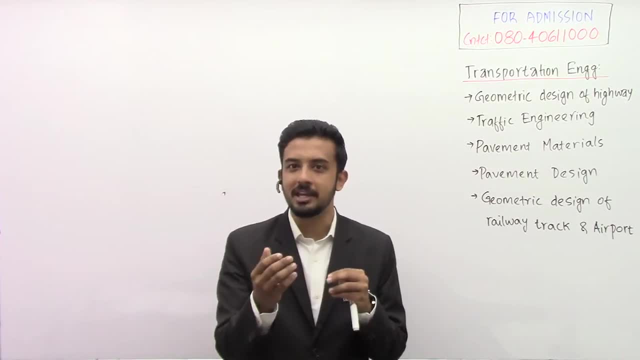 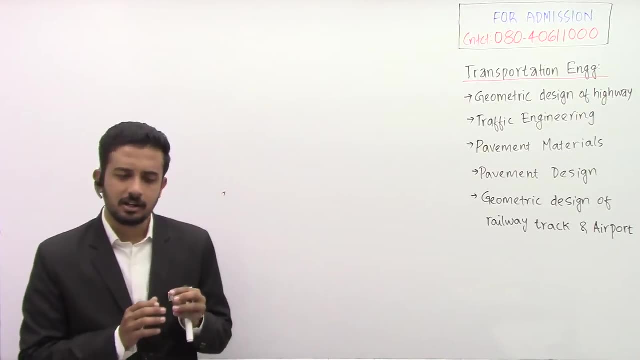 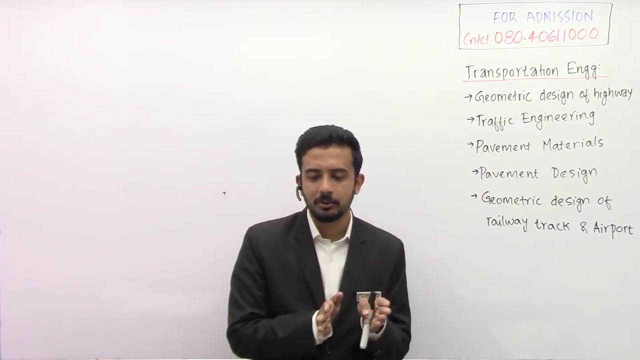 uh, what are mistakes that you can make during the exam? they will check that and accordingly they will set the options also. so, even if the concepts are simple, don't take it as silly subject. it's a very important subject. they can easily make you or they can easily deviate you to the other directions. 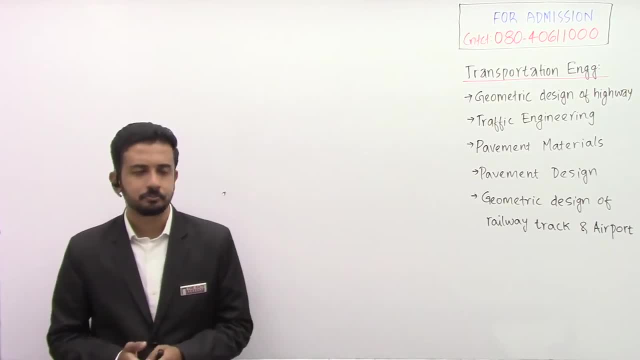 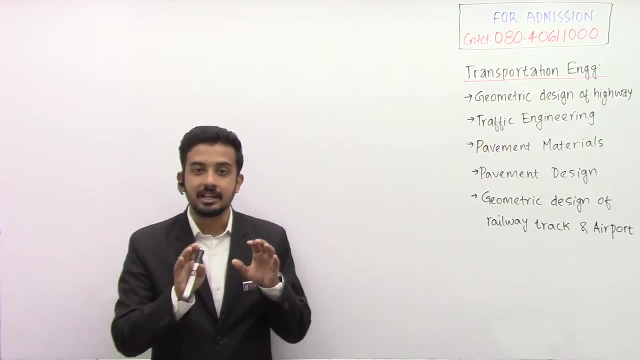 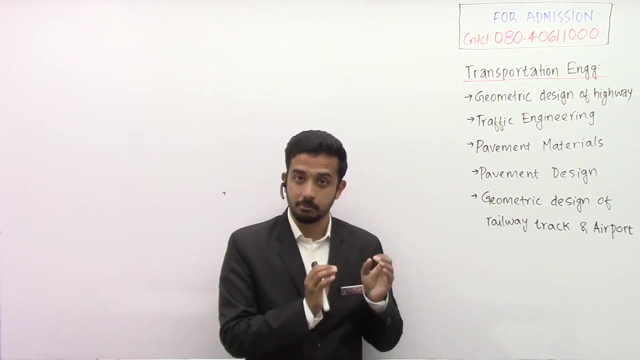 okay, so don't make mistakes while solving the questions. all the concepts are easy. some concepts are tough also. so while attending the class, after understanding the basic concepts, then go to the tough questions directly. don't go to the tough questions from this chapter, okay, from this particular subject. first go through the all the basics, study all the simple, simple formulae. 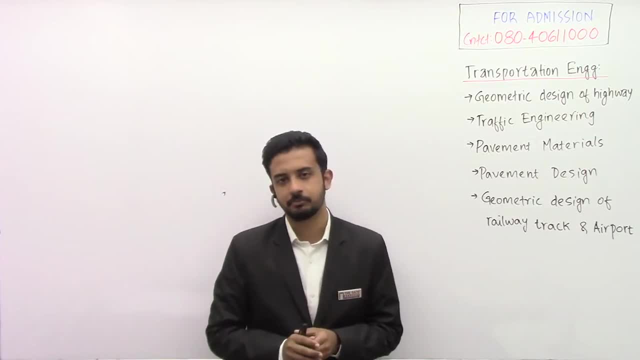 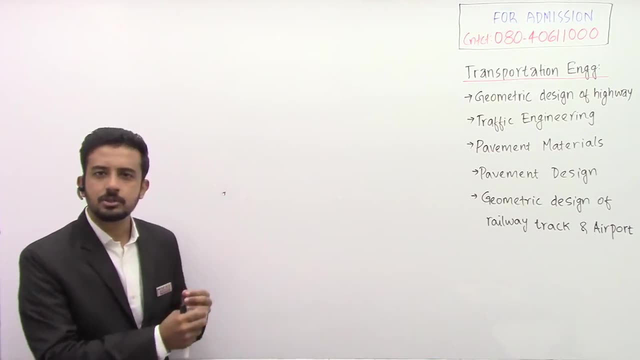 then go to the toughest formulae, then solve the tough questions. okay. yes, of course we are not having that much tough questions in gate examination, only a few other. but after solving the easy questions, okay, after solving the easy questions, the questions are tough. I strongly recommend understanding the concepts. you will be able to solve those questions, trust me. 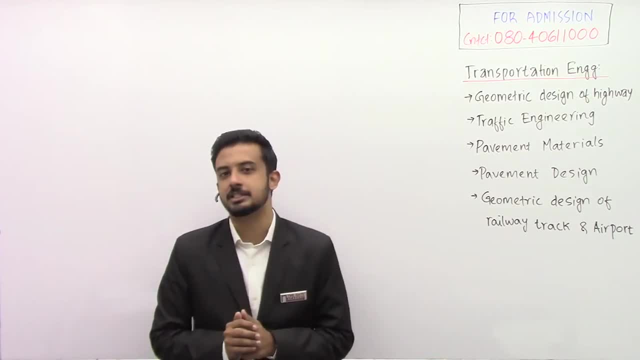 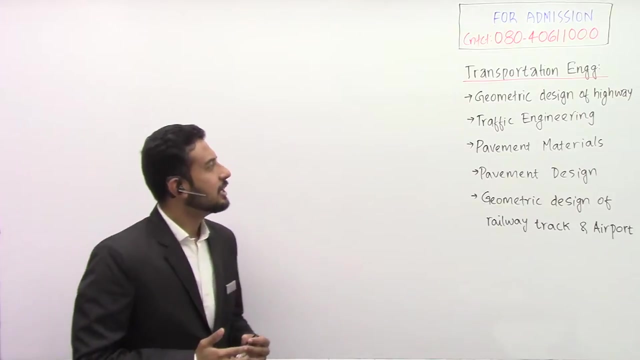 if you are attending the complete session of our transportation engineering, you will be in a position to solve whatever questions they are going to ask. okay, take, I mean, I mean trust me. okay, so in this session we are going to discuss the first chapter, geometry, design of highways, and the remaining 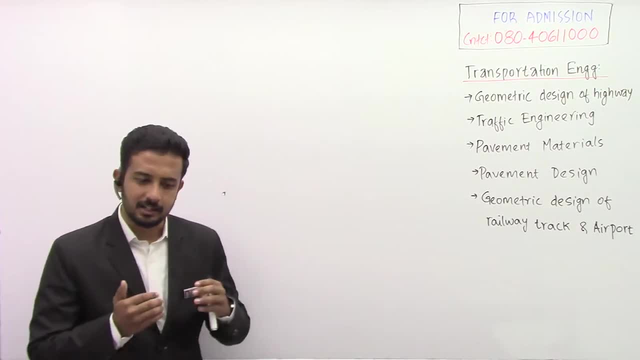 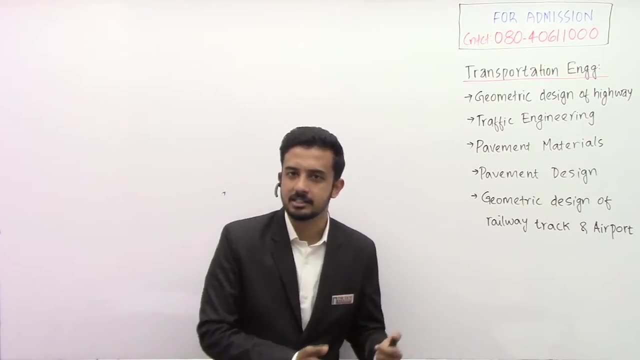 chapters we will be seeing in the coming days. in this week we will be seeing the geometric design of highways. only later, on, a later date, you will be getting the other subjects, other chapters, also from this particular subject, okay, so I hope everyone have joined. Sunil Sharma is there. good morning. 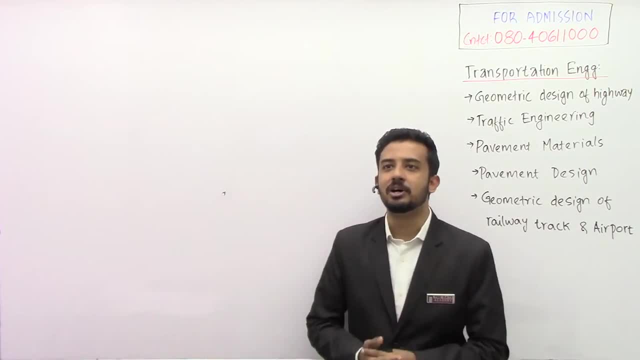 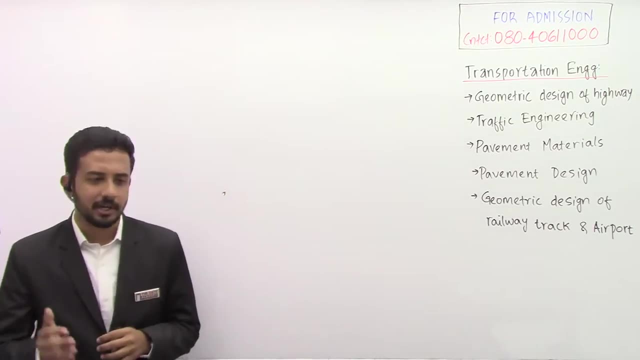 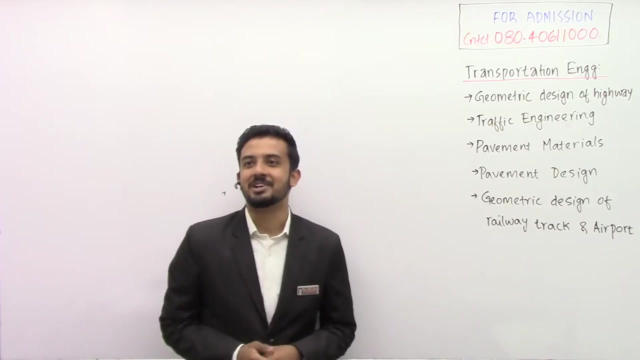 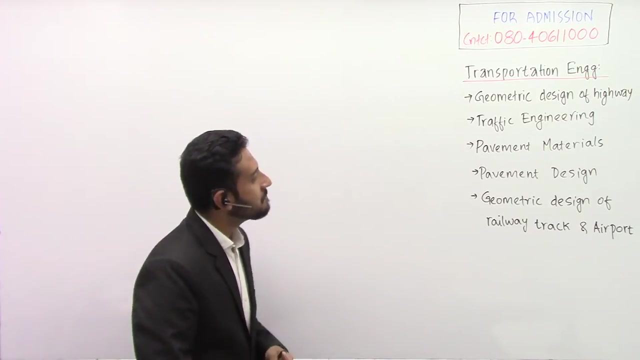 Dabashish. good morning Dabashish. Mohar Sahu is there? good morning Mohar Lokesh. good morning Lokesh. so I hope you are preparing for your GATE exam very well. so one, all the best in advance. you, yeah, one of my friend is there. hello, yeah, good morning. so yeah, we are. 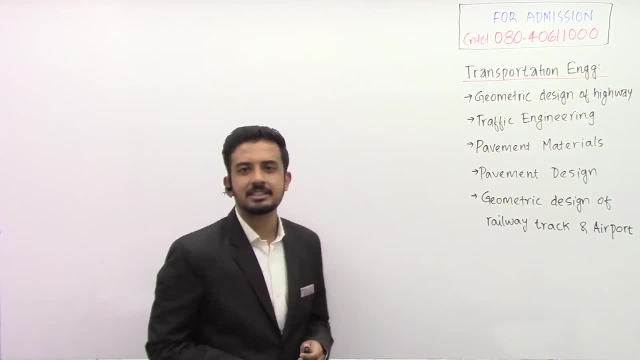 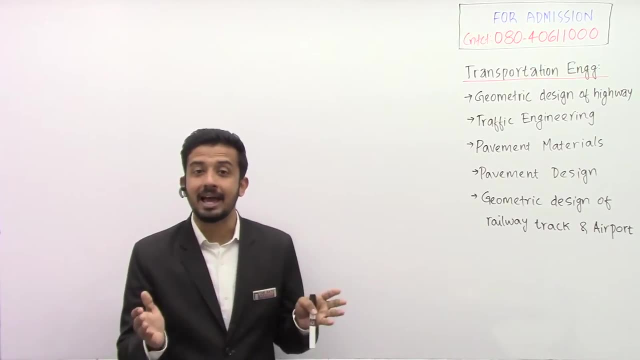 starting with the geometric design of highways. if you are checking the syllabus you can see one more hint. before this geometric design it's nothing but the highway development planning and all. it's just a theory concept only. like what are the milestones happened in our highway development activity? like what are the milestones happened in our highway development activity. 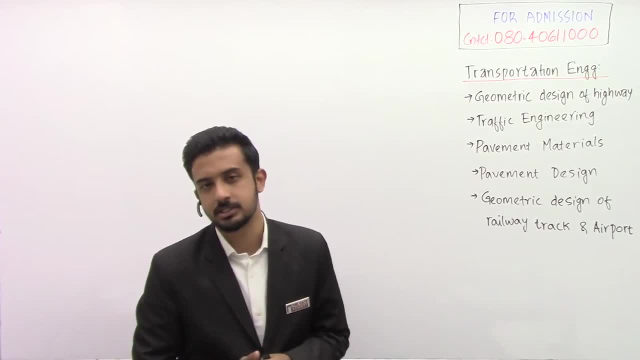 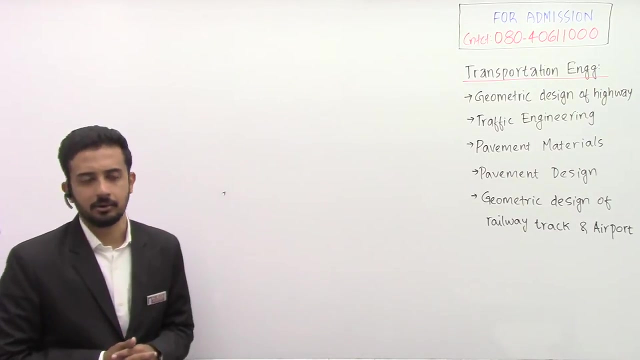 like: what are the milestones happened in our highway development activity? like you know, IRC Indian road Congress, you might have already stated in your college right. so when IRC has formed so such a milestones, maybe there so that you know IRC Indian road Congress, you might have already stated in your 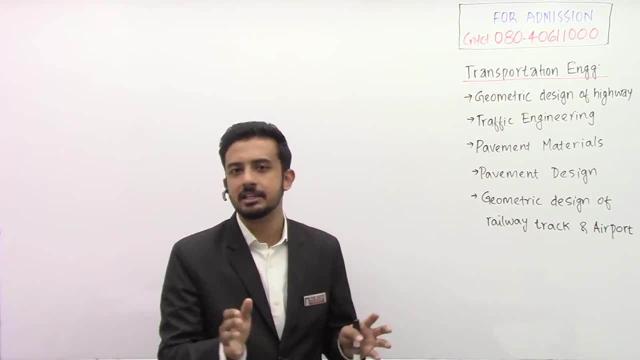 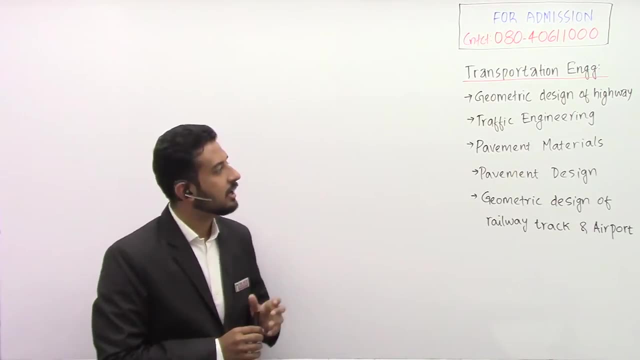 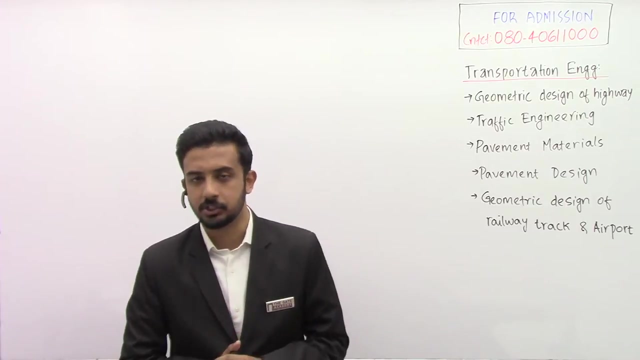 college right. so when IRC has formed so such a milestones may be there so that you have to go through its. simply some theoretical concepts and some surveys. what we are doing a lot, so it's just a matter of like some one page, two page chapter. geometry. design of highways is one of the most important concepts for gate examination. 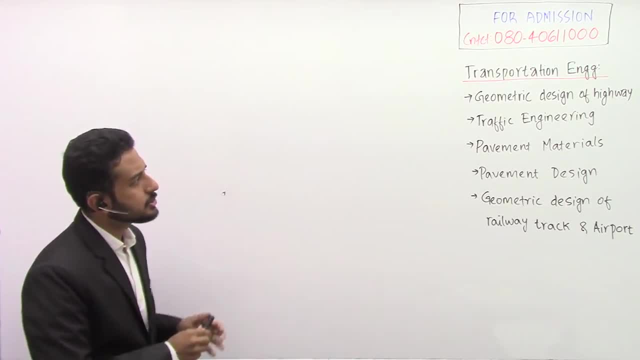 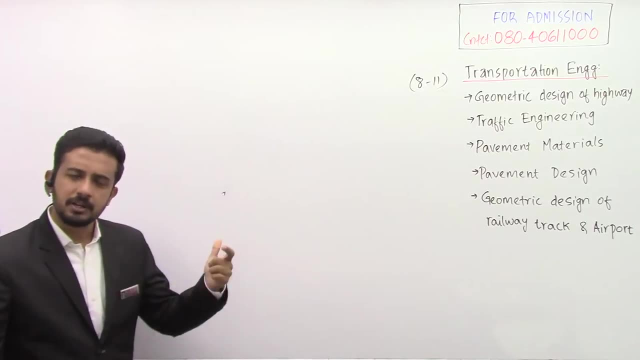 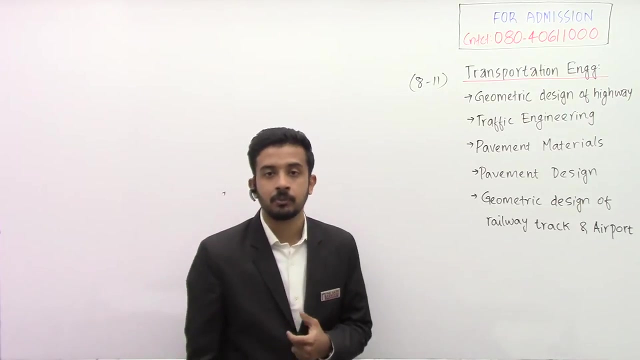 from this particular subject. okay, so i told you the transportation engineering will hold around 10 to 11 marks. you can expect 10 to 11 marks. previously, they were asking just around 6 or 7 marks only previously, till some 2015 or 16, but what happened in 2016? they have introduced. 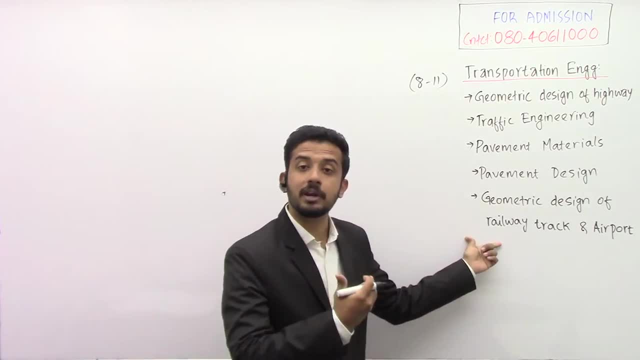 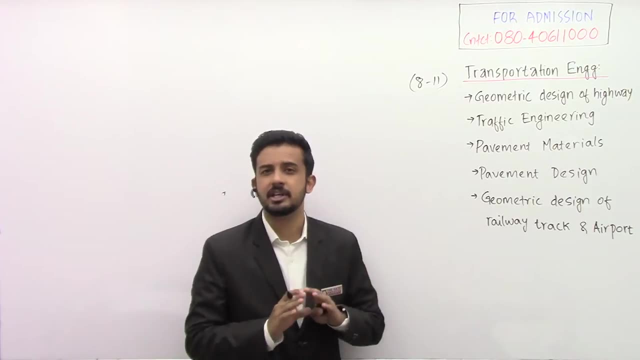 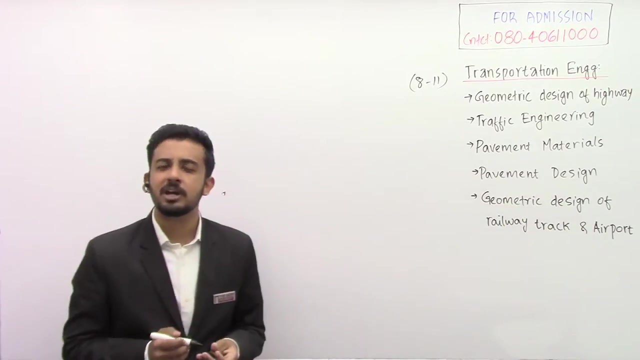 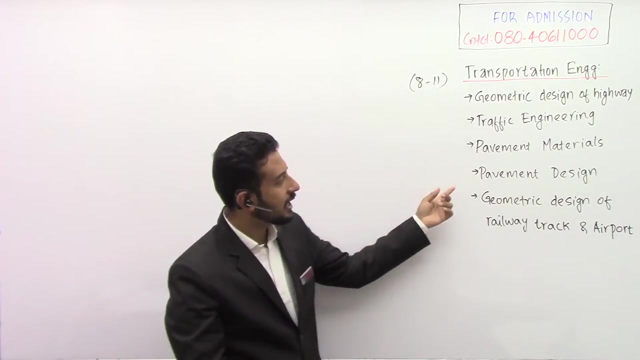 a particular chapter: the geometric design of railway tracks and airport. right, see, actually speaking, the railway engineering and airport engineering is a vast, vast chapter, but the thing is we are having only the geometric design. so what you mean by the geometric design, see for highways also, we are having two designs: geometric design we are having, as well as pavement design. 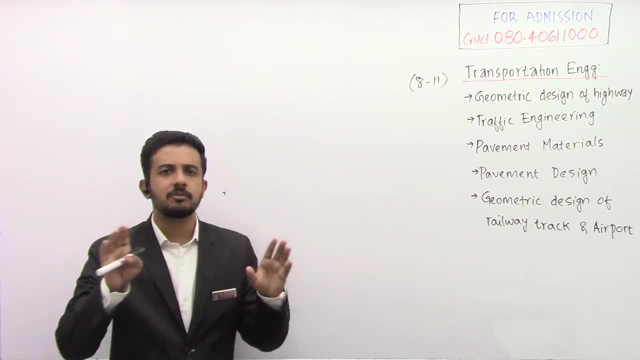 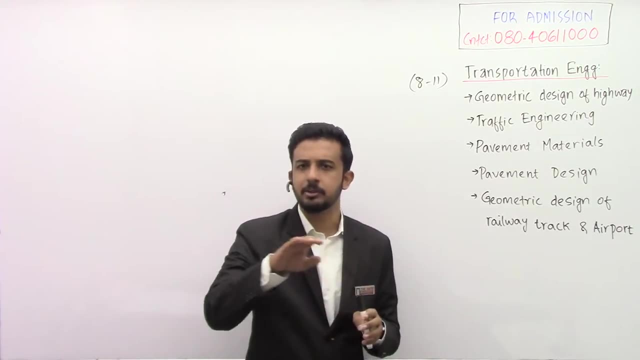 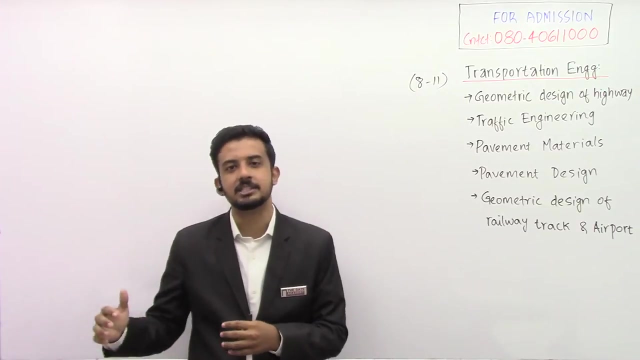 we are having. geometric design means whatever we are seeing. see the dimensions and all the width of the road. how much should be the site distance? how much should be the slope we are giving for the road like that? the super elevation you might have already studied, we will be discussing in our coming sessions. okay, so that is geometric design. 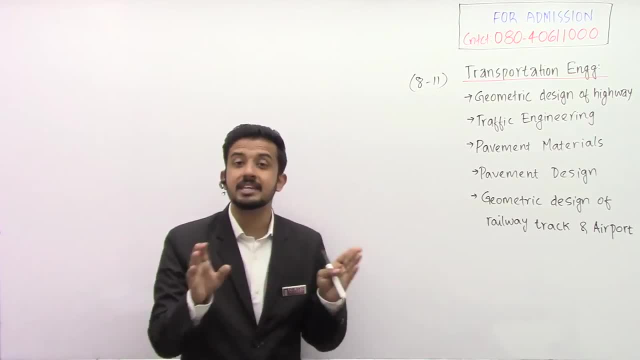 the, the what, what, i can tell, like the physical features, what are the dimensions that we call it as geometric design and whatever there below the ground? the pavement thickness, what should be the thickness of each of the roads and what should be the thickness of each of the roads and what should 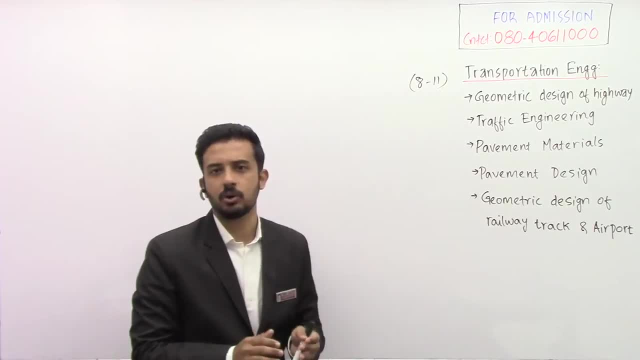 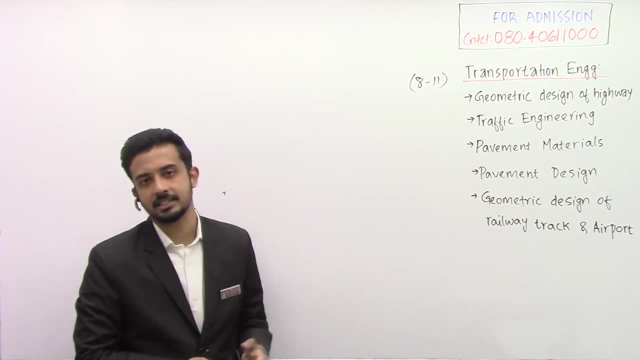 be the thickness of each of the roads and what should be the thickness of each layer, those things we are studying in pavement design. what are the stresses happening? what are the temperature stress, what are the stress due to the wheels? that we are studying in the pavement design. so such pavement design we 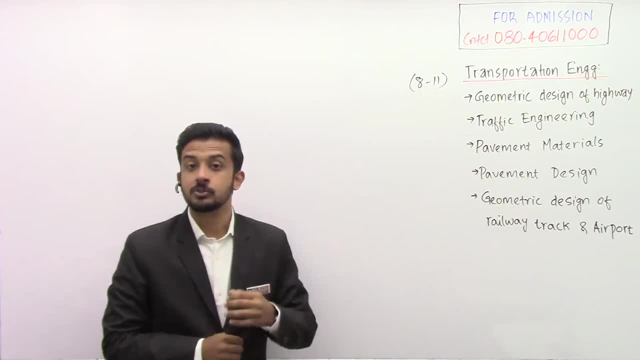 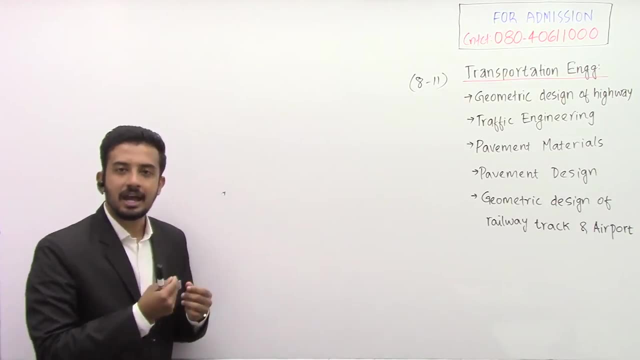 are not studying in our airport engineering and all, so that is an advantage for us. we don't have to study a lot of things to get this 10 to 11 marks. so since they have added that particular chapter- geometric design of railway track and airport- the weightage has been increased. 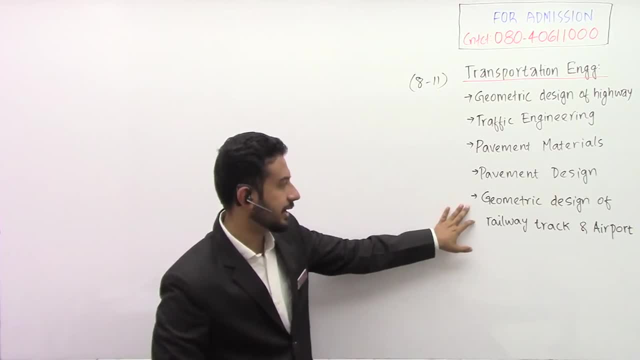 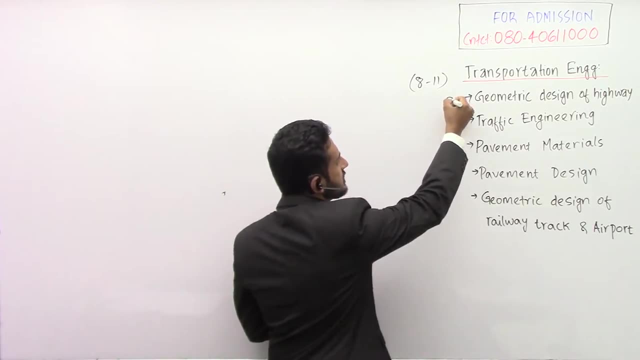 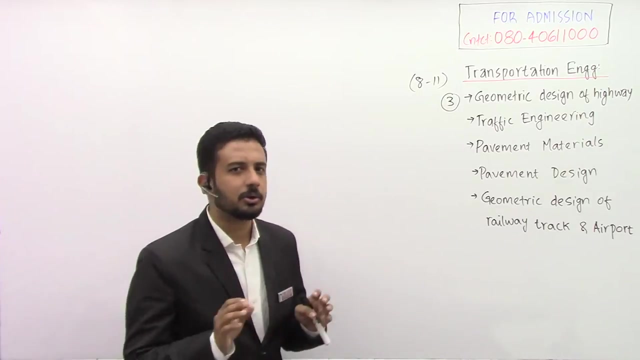 now by some two marks. okay, so a two marks you can expect from this last chapter and the geometry design of highways. it depends from year to year, but at least average three marks you can expect from this first chapter. okay, see, to score that three marks you don't have to put any extra effort. 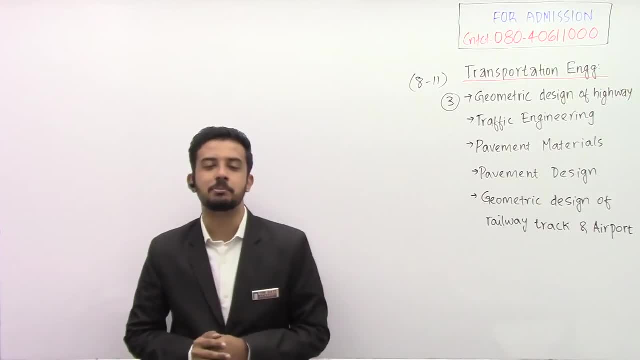 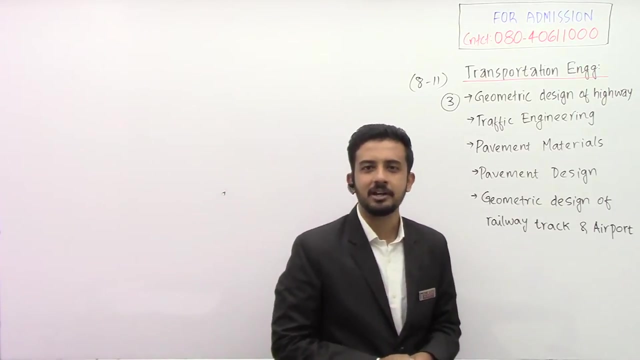 attend the all the sessions of this particular chapter. trust me, definitely, definitely, you're going to get that three marks and whatever. even if it is a toughest question, okay compared to other questions, you will be able to solve that question. so i hope- uh, everyone have joined, we can. 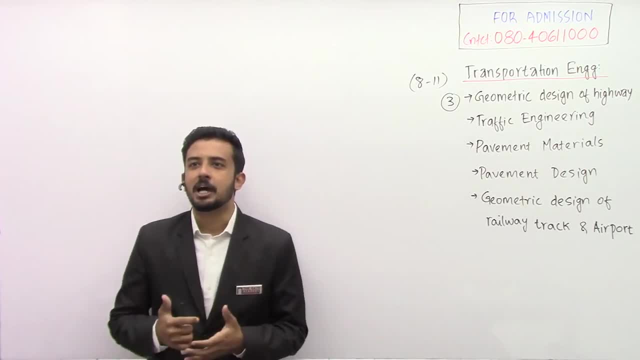 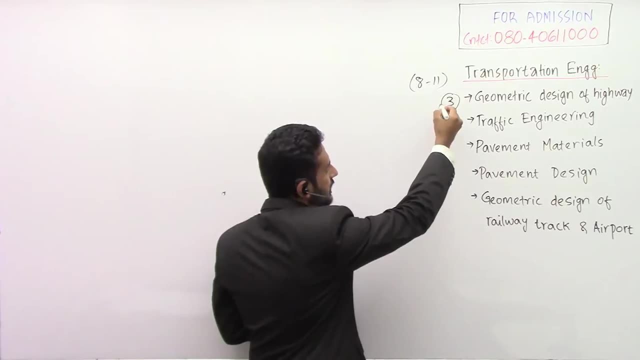 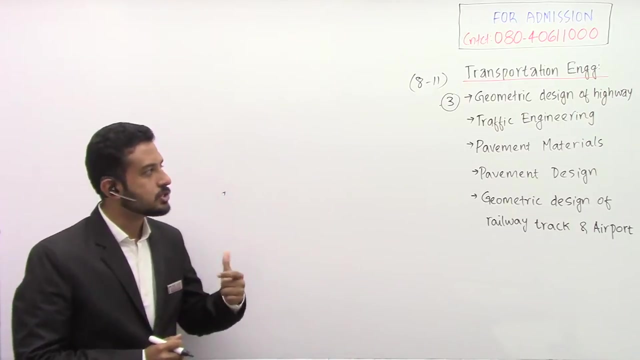 go to this chapter, right? yeah, abhishek, good morning. abhishek, sunil, good morning. okay, so we are dealing with the first chapter, geometry design of highways. we have to study uh, three, four topics under this particular chapter: geometry design of highways. the first thing is the cross-sectional elements. so what you mean by 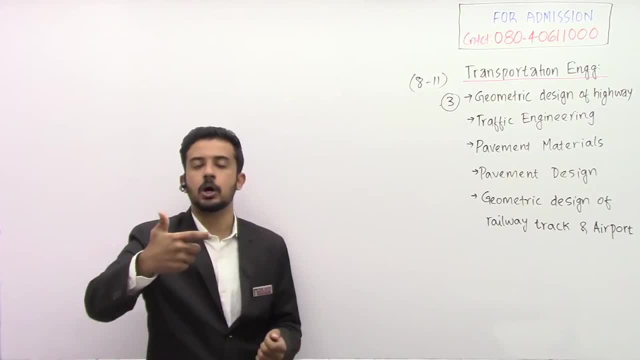 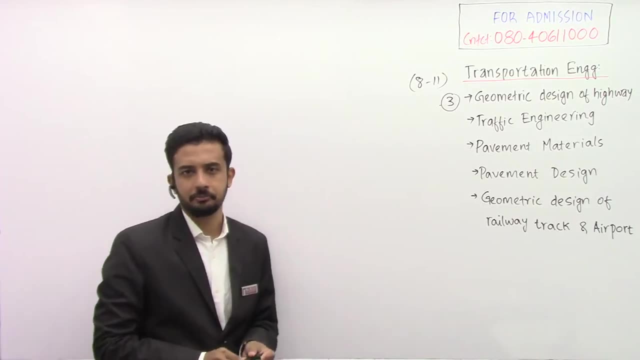 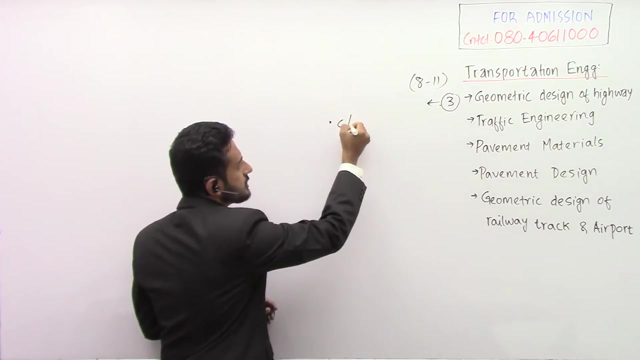 cross-sectional elements. if you are taking a cross-section of the road, what all things we are seeing, that's it the width of the road and the slope of the road, etc. okay, so first i'm just listing out what all things we are going to study under this particular chapter. we are going to 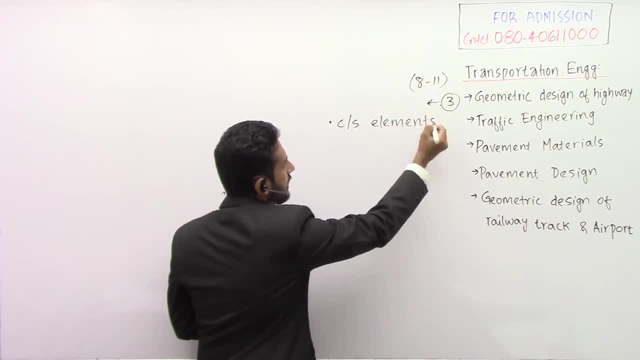 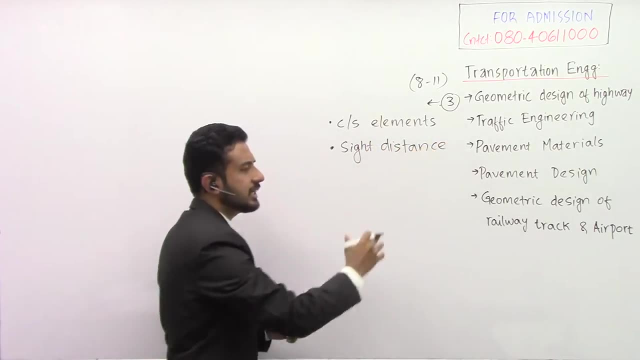 study the cross-sectional elements, then we are having some site distances, very, very short distances, and we are going to study the cross-sectional elements of the road. so very important for gait examination. the sight distance you might have already studied in the college, you might. you may be thinking that it is a simple concept, but for gait exam they can ask. 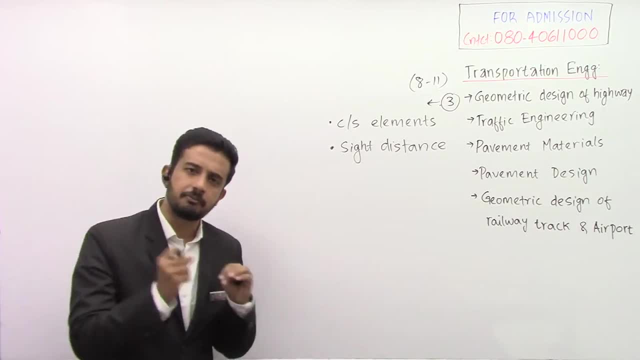 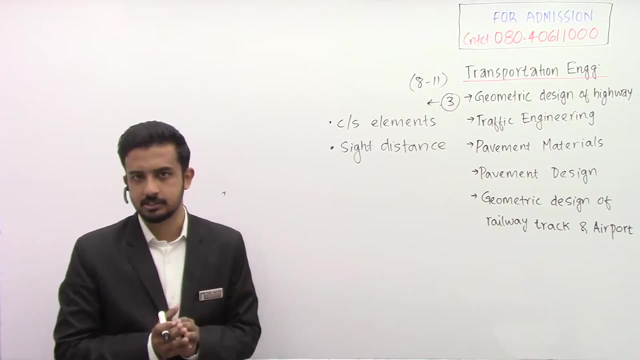 you the questions in any way. okay, don't think that every time they will give all the parameters and ask you to calculate from the question. you should identify what actually they have asked. okay, so there is high chance of making mistakes. so, sight distance: under this sight distance we are going. 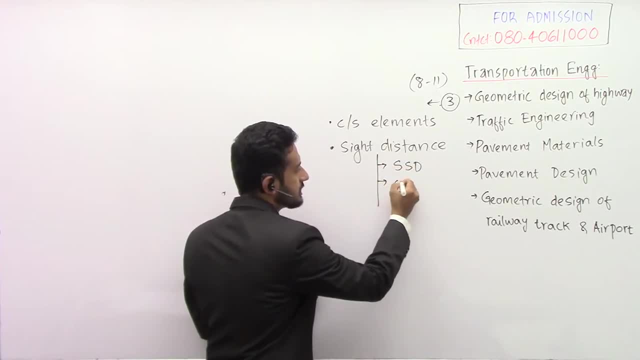 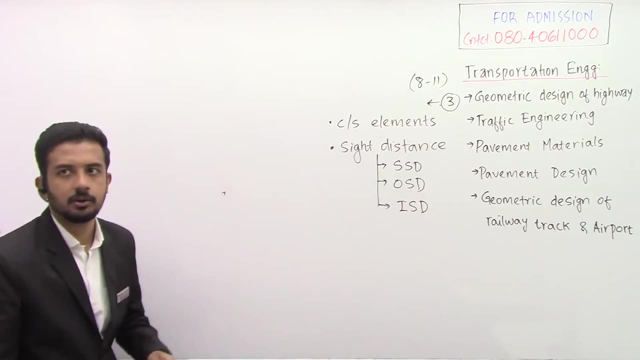 to study our stopping sight distance. then we will study our overtaking sight distance. there is one more term called as intermediate sight distance. okay, so we will go through one by one, okay, yeah, good morning teja. uh, the class will be in english, uh, because i'm more comfortable in english. but 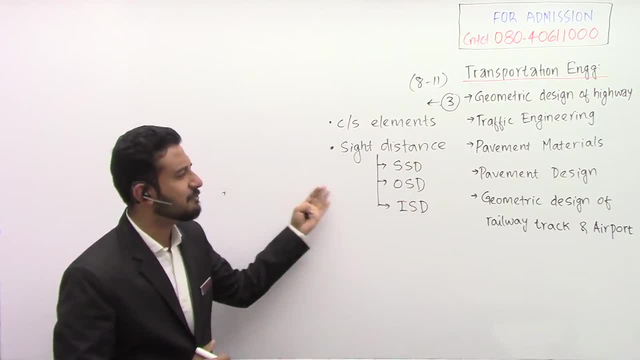 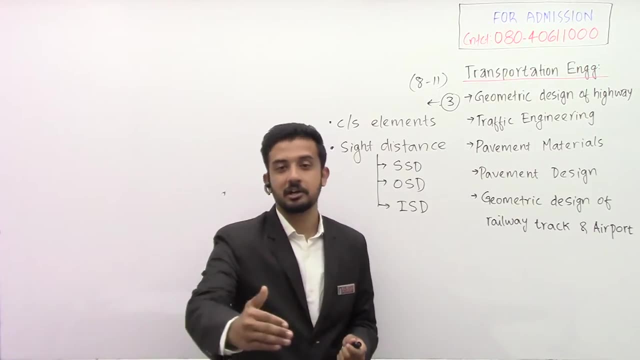 don't worry, we will be using simple, simple things. only see, everything is related to our day-to-day life, right? see, whenever you are going on the road by taking your vehicle, or you are traveling on the bus, whatever it is, you're seeing everything. what should be the width of the road? 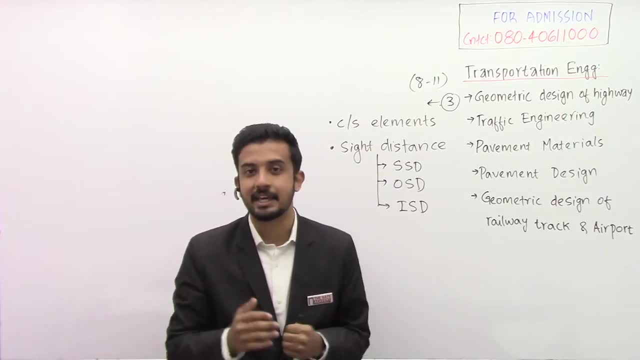 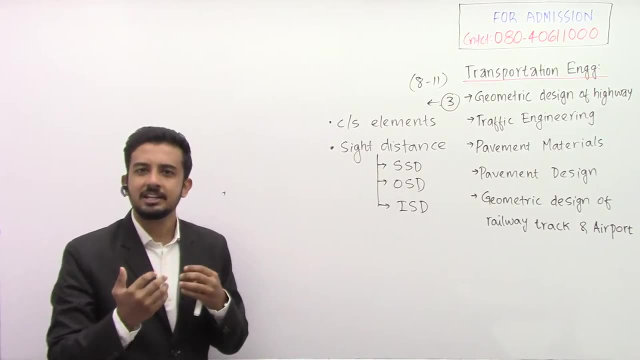 how many vehicles are coming when the congestion is happening. everything you're seeing in your day-to-day life, right. so that is the important, that's the beauty of this subject: you can correlate with your day-to-day life. so whatever we are studying easily, you will be understanding those. 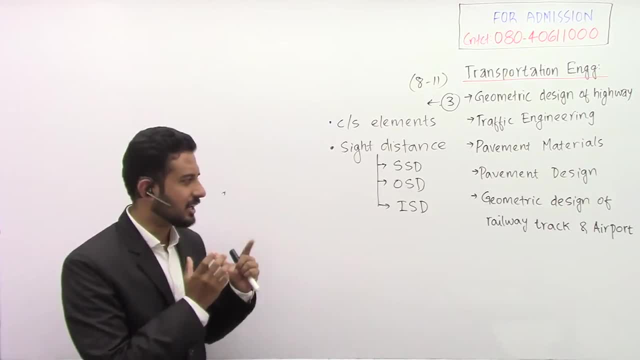 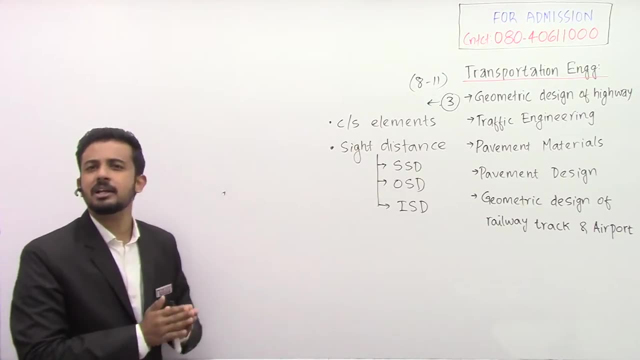 things. only difficult part is calculation. if you are understanding that tricks, if you are understanding the formula, it's easy. that person also. okay, so the class will be in english, but it will not be going to affect you. okay, don't worry, easily you will be able to follow. 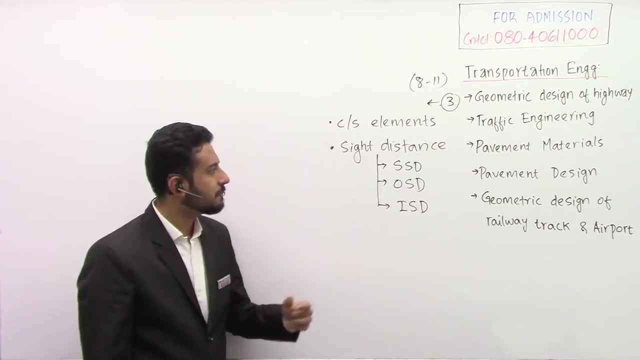 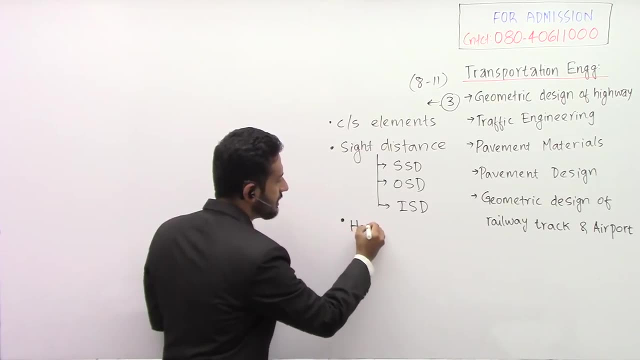 so intermediate sight distance we are going to see, see, we'll discuss one by one. i'm just giving you the overview sight distance. then we are going to study some aspects of horizontal curve. so many things will be coming under this horizontal curve, such as super elevation. is there? 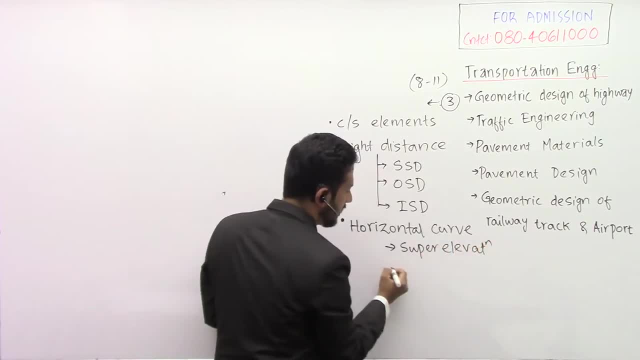 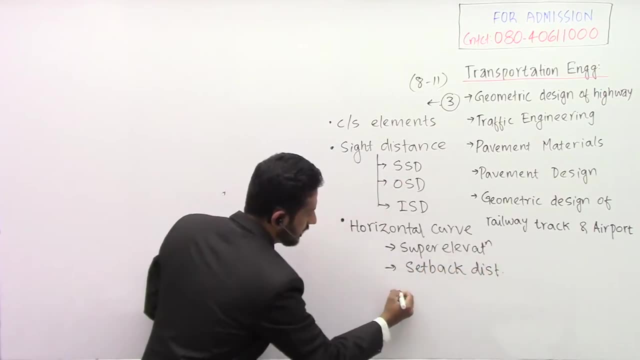 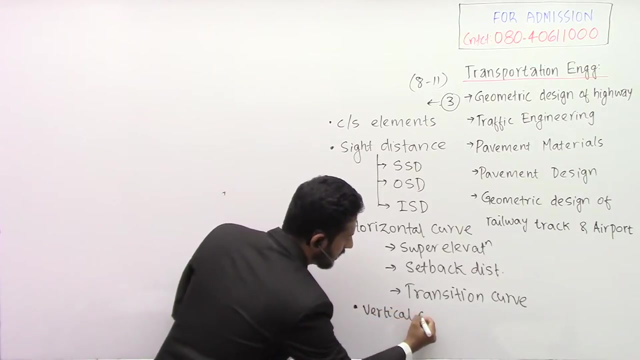 very, very important for gate examination: super elevation. is there, then some setback distance? we will be studying setback distance. then some transition curve: is there? i'm just giving you some important things. only remaining portions we will be studying in our coming sessions. after horizontal curve, we are going to study our vertical curves. okay, what is the difference? 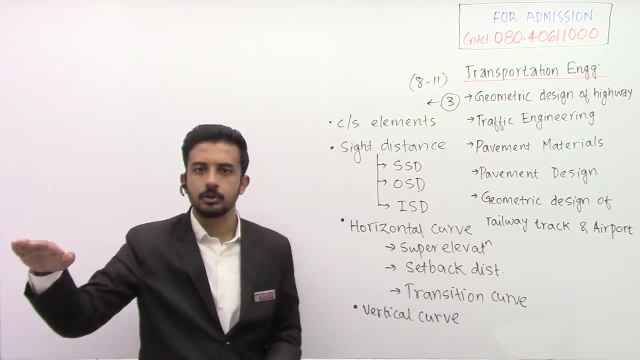 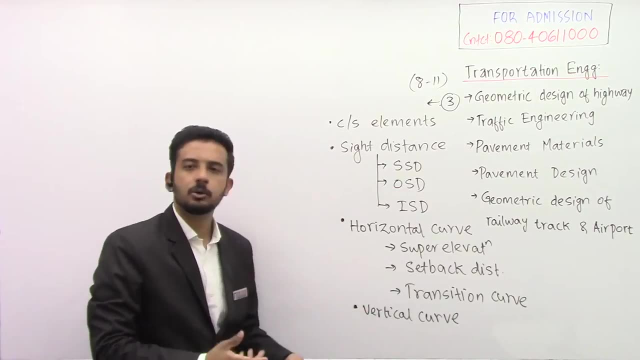 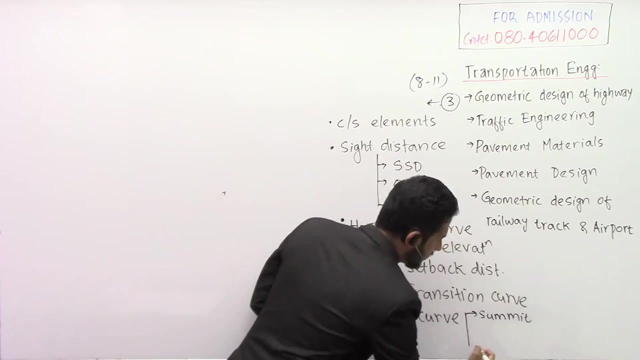 between this horizontal and vertical. if it is on a horizontal plane, it is called as horizontal curve. if it is something like hilly portion, it is called as vertical curve. there are two types of vertical curves: one is the summit curve and the second one is the valley curve. so, regarding this also, we will be studying in our 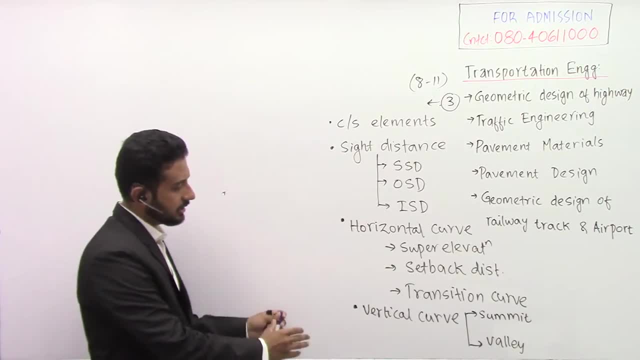 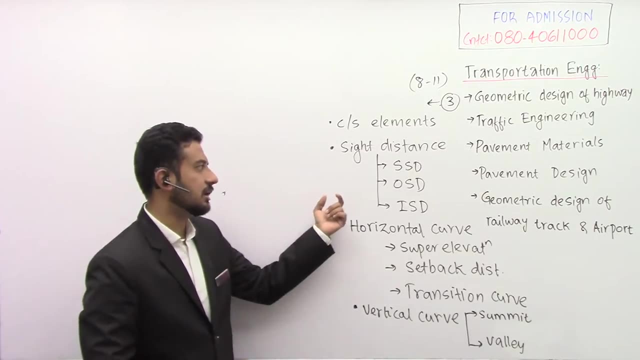 coming sessions. okay, so these are the topics, important topics we are going to discuss. so maybe in this session we will be discussing the cross-section elements and the sight distances. maybe till this stopping sight distance depends on our time. so we are, we are having a two hour. 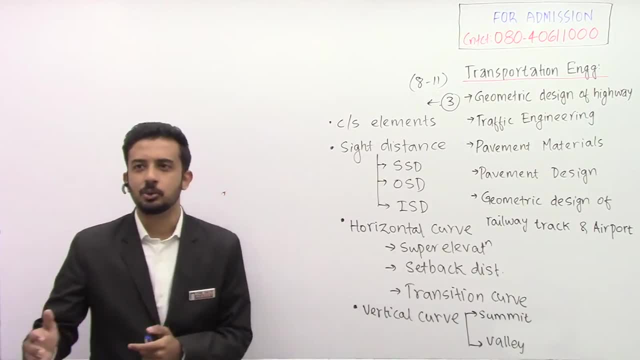 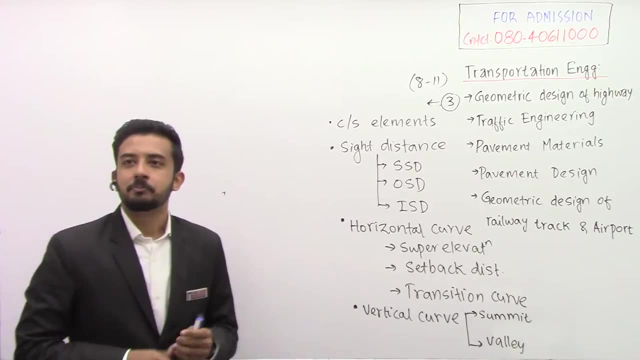 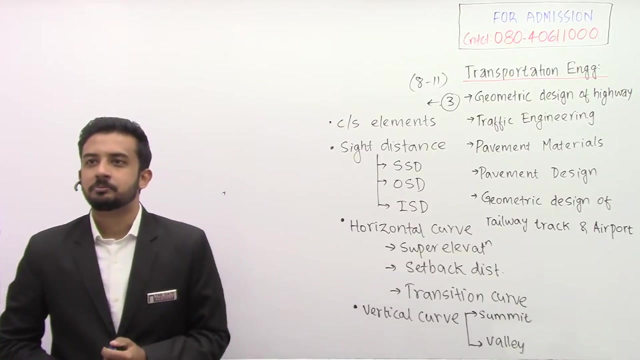 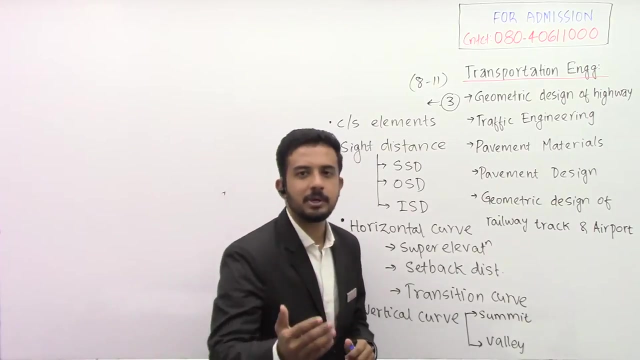 session today, so tomorrow again, you will be getting a two hour session like that. we will be covering the first chapter. okay, yeah, hi, john, good morning. uh, this session will be for two hours, so later you will be getting the remaining, also for uh. one more thing for all other subjects: if you're having any query, uh, you will be getting. 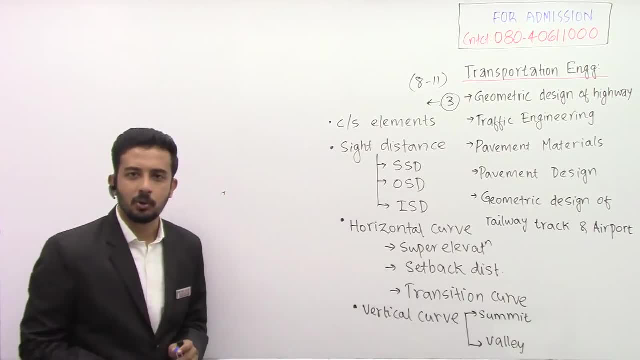 a live uh classes timetable. so we'll be providing you. you can go through the timetable and whenever some classes are happening, you can go through it and visit. okay, so better subscribe the channel and click on the bell icon so that you will be getting the instant notifications. 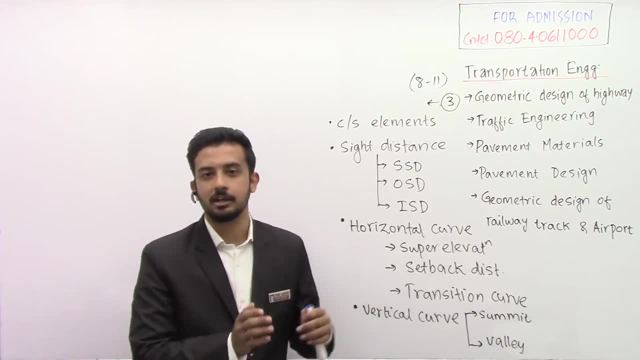 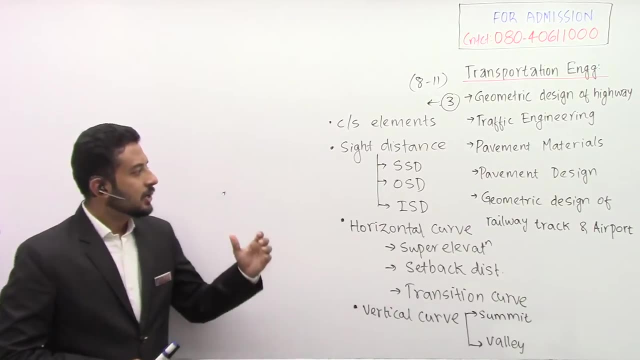 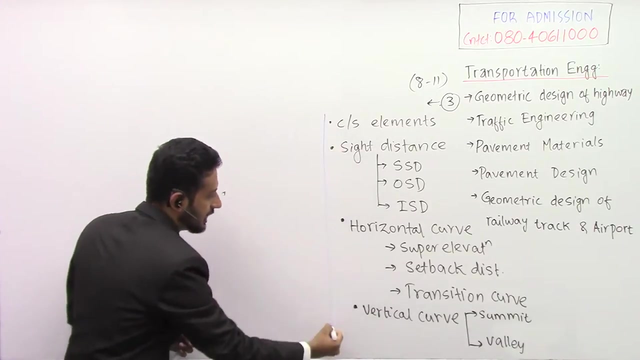 whenever some chapters, whenever some subject is going on, you will be uh getting those notifications instantly. okay, so subscribe the channel and click on the notification button. so, coming back to our subject, so these are the things we are going to discuss uh in the in our session. so let's see uh till. 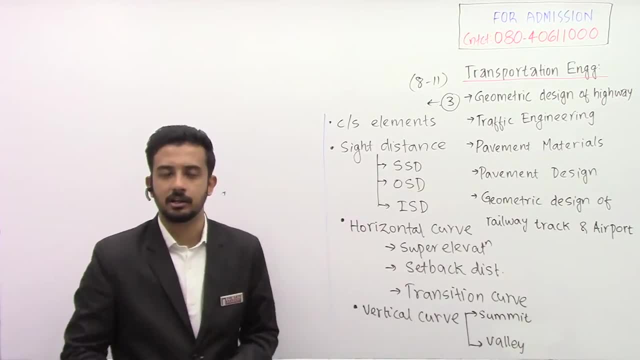 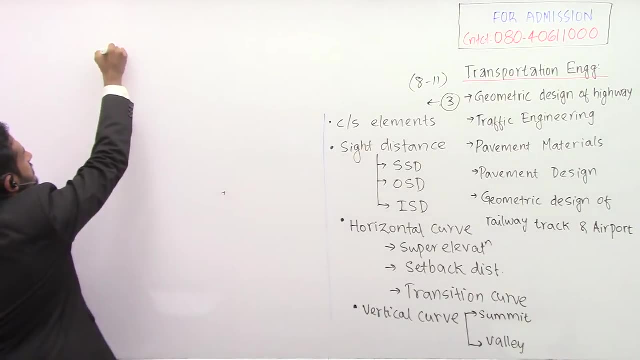 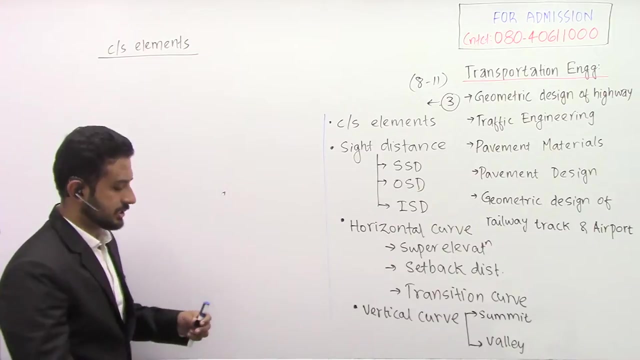 whatever portion we can cover today, remaining portions will be coming in uh covering in the coming sessions. okay, so we are going into our first topic: cross-sectional elements. cross-sectional elements, so cross-sectional elements. i have already told you what you mean by this, cross-sectional elements. so we are going to discuss in this session, so let's see. 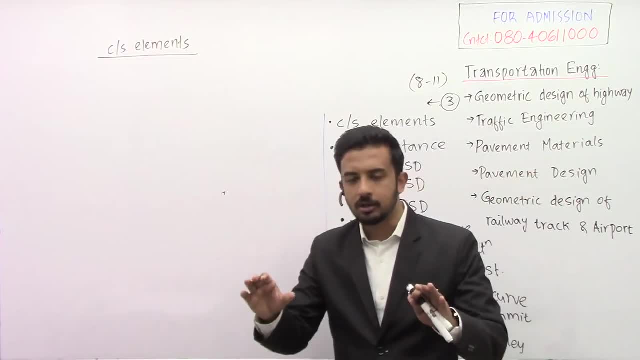 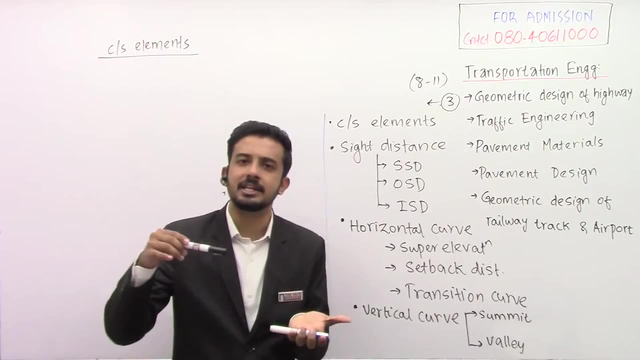 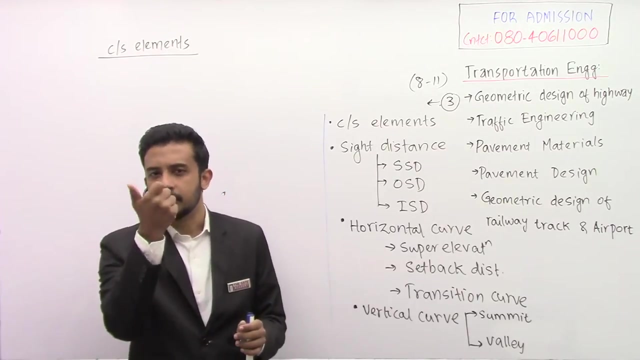 element, nothing but whatever we are seeing on the road. see, the width of the road is there? then some see, you know, whenever a vehicle is going and if it is applying the brakes, finally it is going to stop, and all right, because of the friction. so the friction is actually a cross. 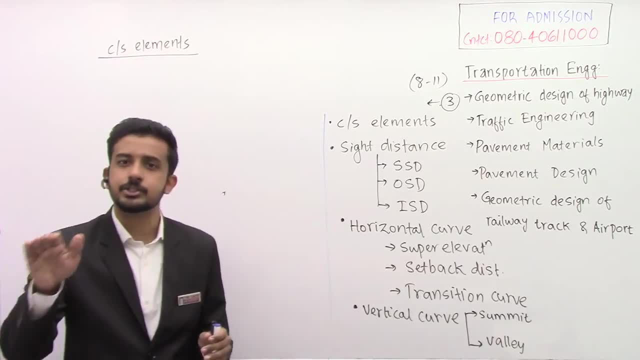 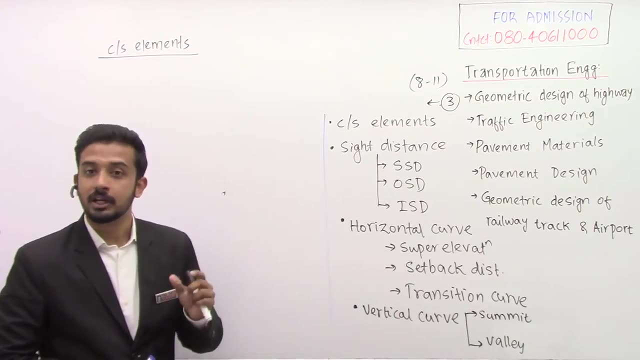 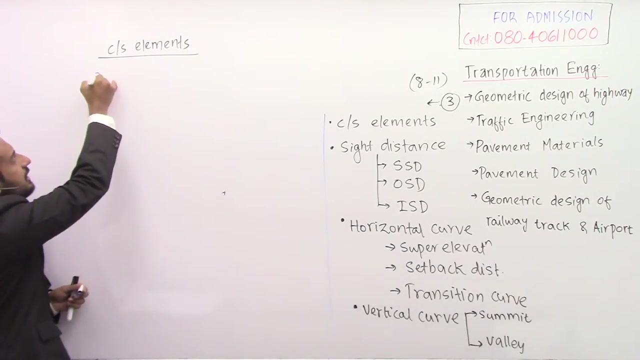 sectional element and the camber. you might have studied the slope of the road. so those things are coming under cross-sectional elements, the important cross-sectional elements i'm giving you. remember those things many times they are fast for one mark. okay, so the first cross-sectional element is nothing but the coefficient of friction. coefficient of friction, or you can simply write: 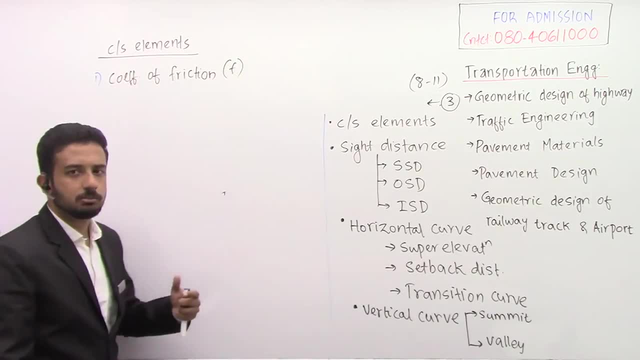 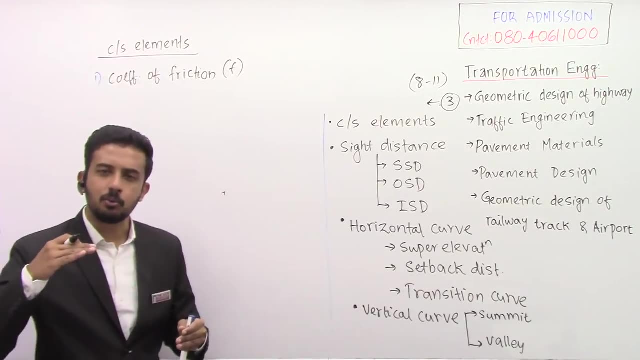 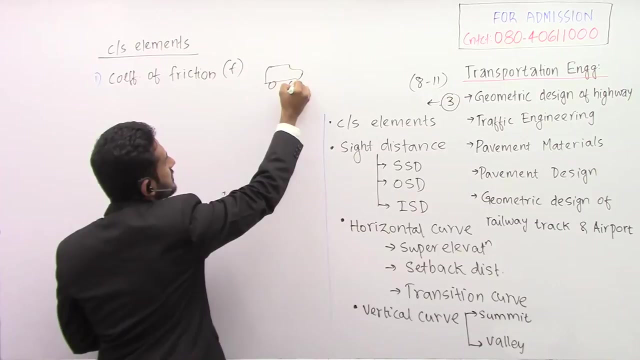 it as friction. we generally denote with the letter small letter f, coefficient of friction. see actually what you mean by this coefficient of friction. we know whenever a vehicle is applying the brakes- see, suppose this is our vehicle. a car is there, i hope, looks like a car. so we are applying the. 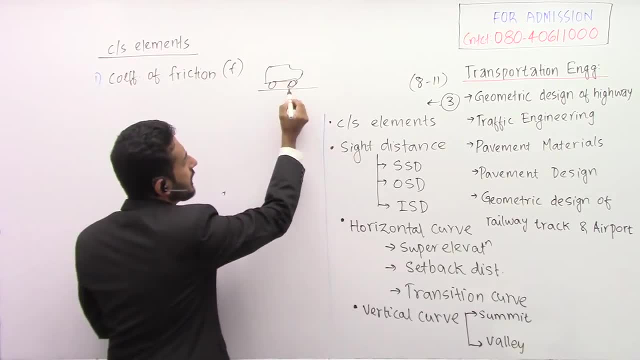 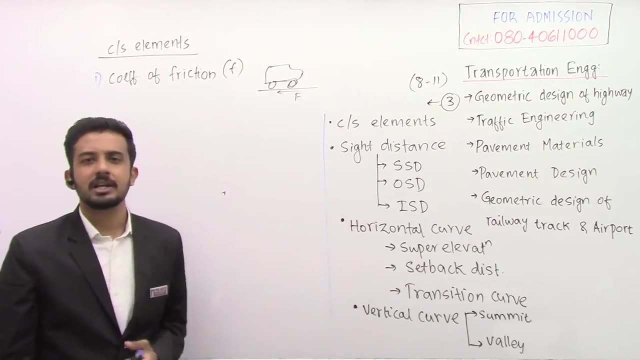 brakes, so it is going to stop right. so whenever we are applying the brakes, a frictional force will be acting against or against the direction of motion. so what is that frictional force? it is nothing but a coefficient into the normal reaction. i will discuss those things again. 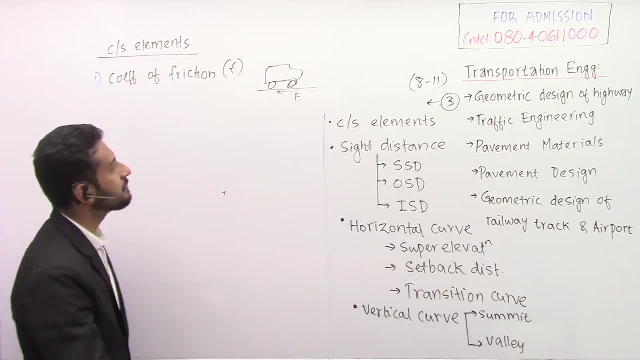 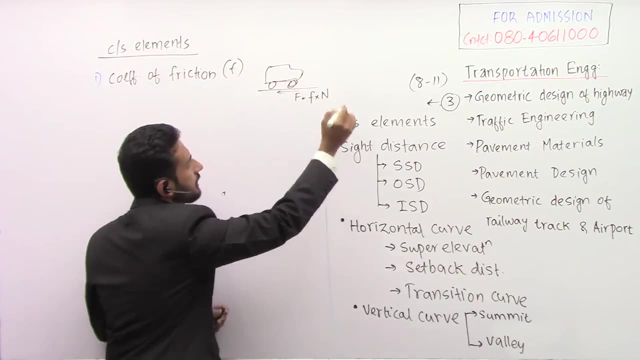 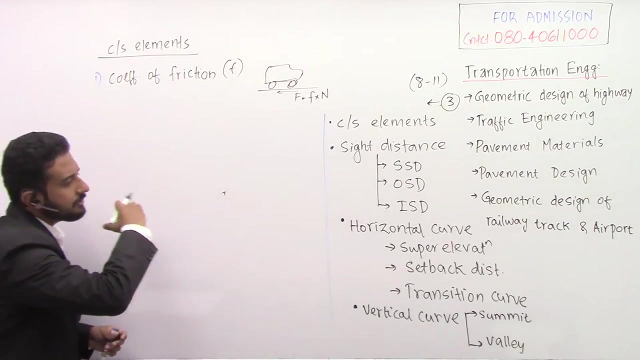 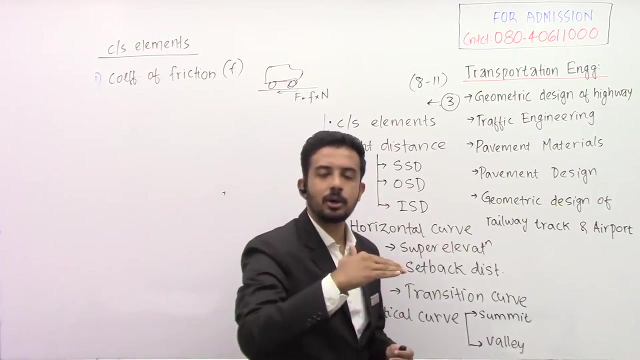 while we are discussing this, stopping sight distance. okay, so that frictional force developing is nothing but a coefficient of friction into the normal reaction developed. that coefficient, we are calling it as coefficient of friction. okay, so if it is in the longitudinal direction, what we have discussed now is in the longitudinal direction, whenever you are applying. 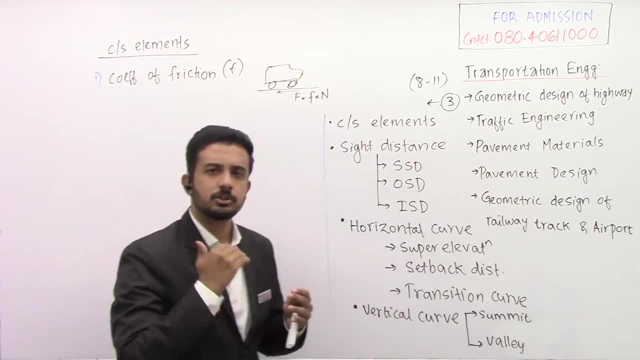 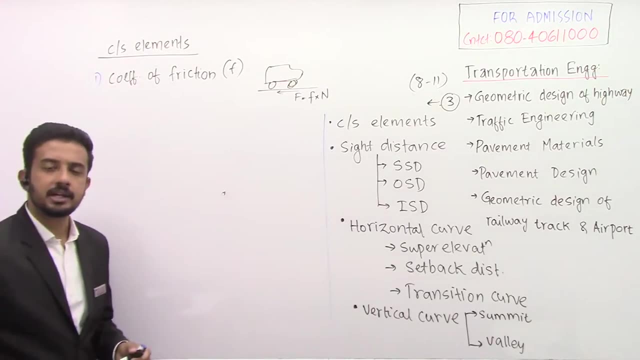 the brake, your vehicle is going to stop right. so that is in the longitudinal direction. what you mean by longitudinal in the straight direction, so that friction- i can call it a coefficient of friction, so in the으. however, the point i am not going to explain the傾 comforting far way. first, 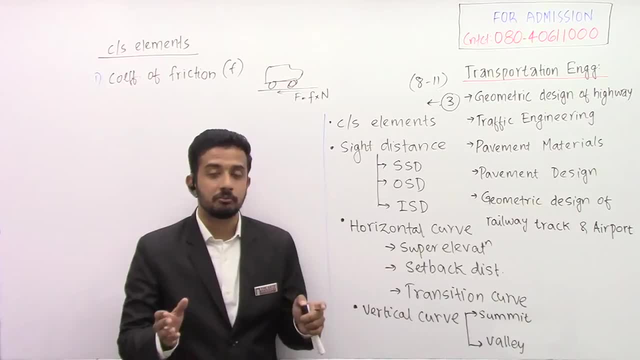 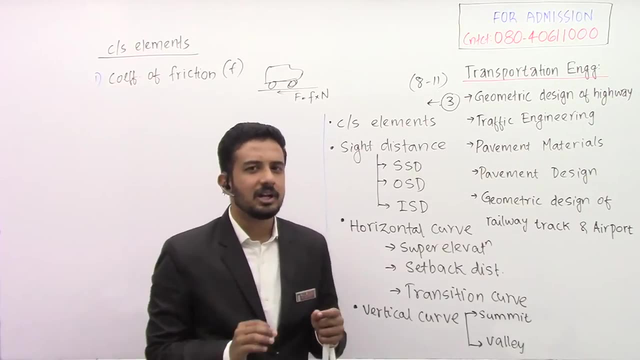 but the coefficient is called as coefficient of longitudinal friction. there is one more coefficient: coefficient of lateral friction. so what you mean by coefficient of lateral friction you might have already studied. whenever we are turning the vehicle on the curve, your vehicle will definitely have a tendency to go sideways right. you might have already. 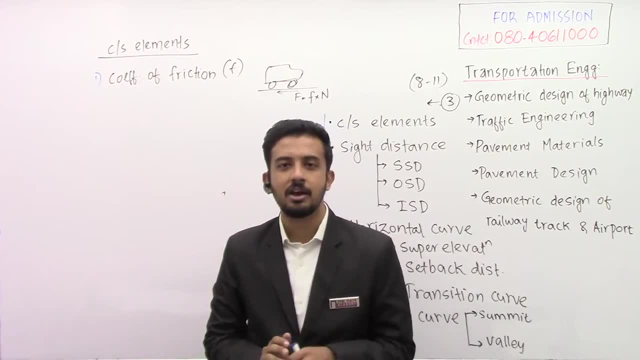 experienced in your life. whenever you are riding your vehicle on the curve, there will be a tendency for you to go outside the curve. so, whatever you have chosen in the decision for you, imagine, let us가지고, you want to have the situation as surplocated you have. 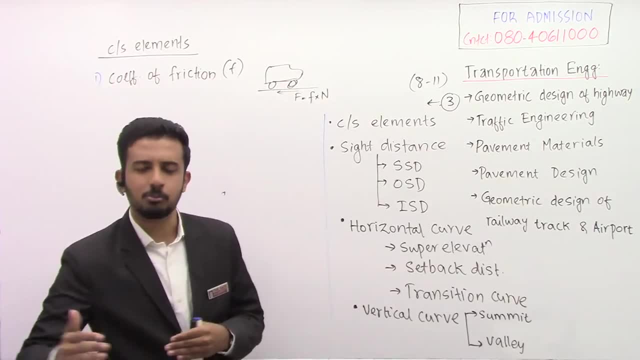 to have the state that is out of alignment sideways. so we are looking at the sun right sidewise. whatever that is turning at AEZE type, you have the potential to go outside the curve this. So who is resisting that moment? or I can tell it as skidding technically. 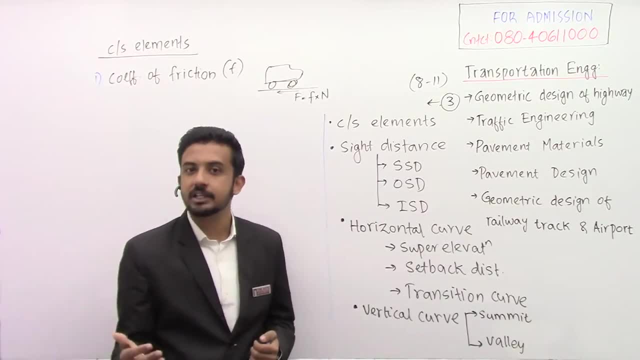 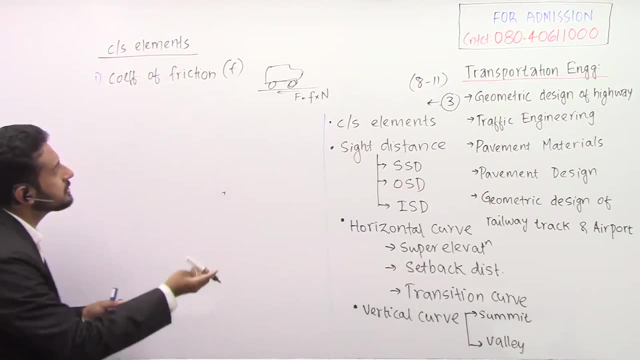 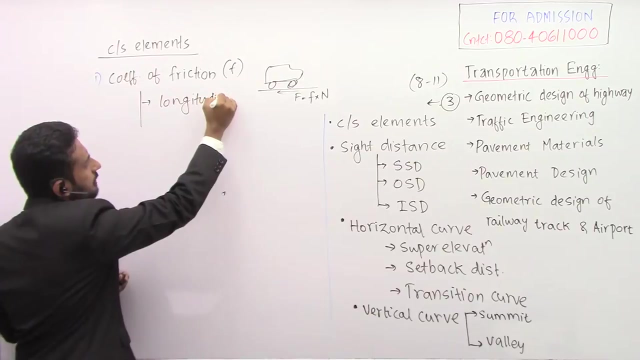 Who is resisting that skidding? Nothing but the frictional force from the side right, So I can call it as coefficient of side friction. So there are two types of coefficients: The coefficient of longitudinal friction and coefficient of lateral friction. 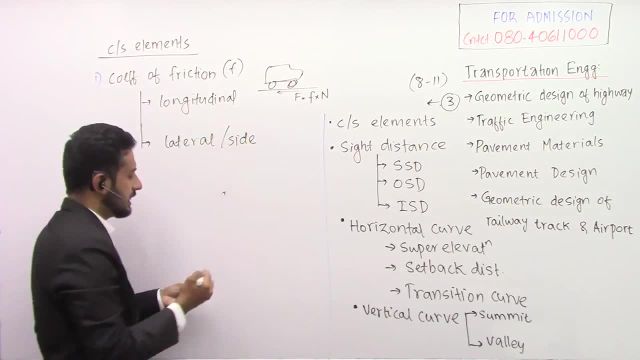 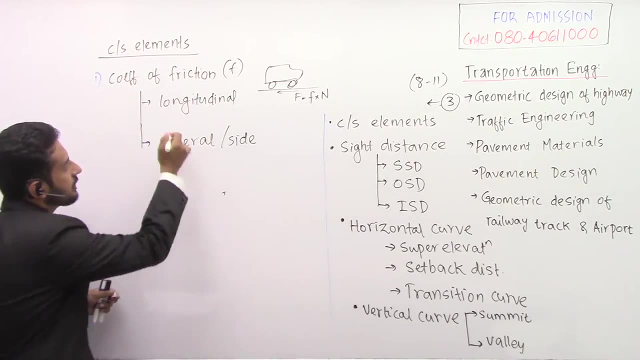 Or I can tell it as coefficient of side friction. The important thing regarding gait exam is: what are the values of this coefficient of longitudinal friction and coefficient of lateral friction? Generally, for design purpose, this coefficient of longitudinal friction will take it as 0.35 to 0.4.. 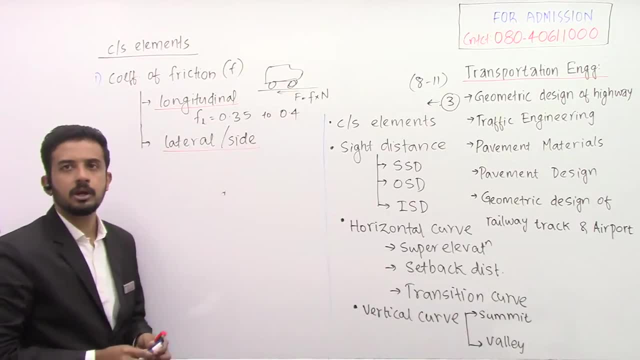 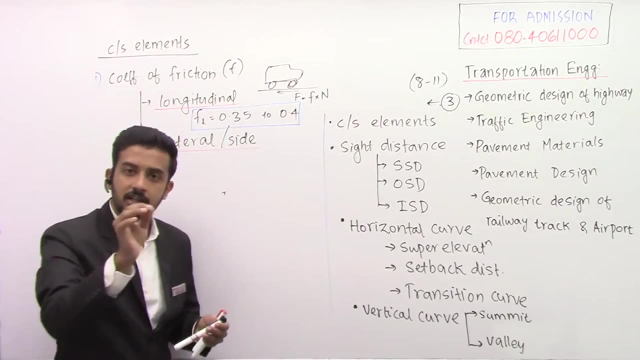 It doesn't mean that in the questions which they are going to give always the value will be in between this. So in the gait exam they can give you any value, Whatever value they are giving for the numerical questions. take as it is. 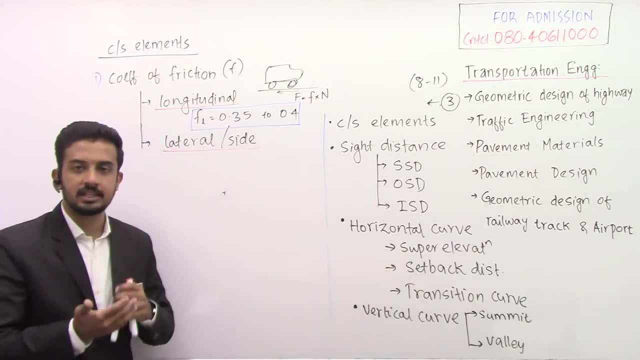 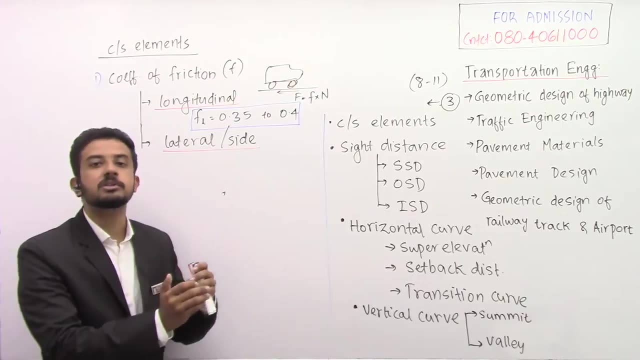 We will be seeing some numerical questions, some practice questions, gait questions, everything we will see. Then you will understand that For design purpose generally we will take from 0.35 to 0.4.. But for lateral we are taking 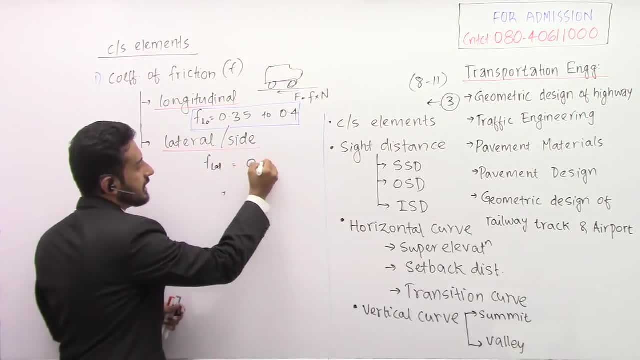 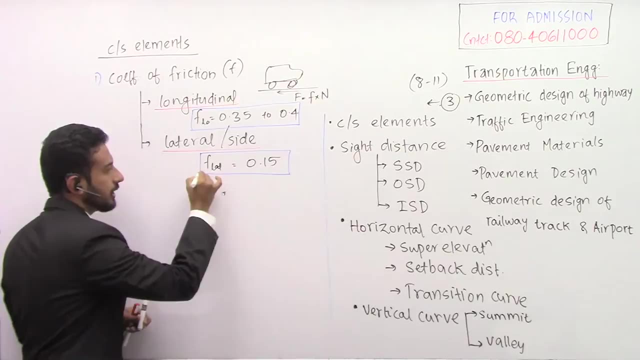 so this is longitudinal, this is lateral For the design purpose. the maximum value we are going to, we are going to take is 0.15.. It is very, very important. It's two, three times. They are fast for gait examination. 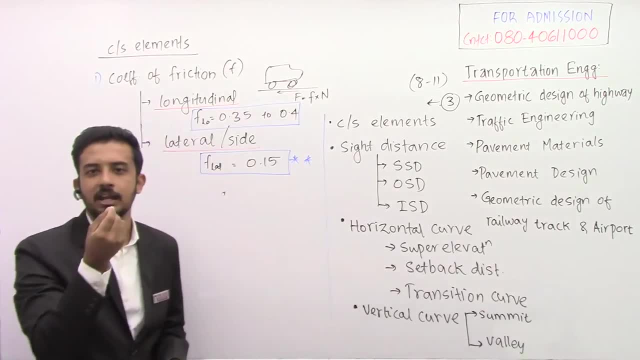 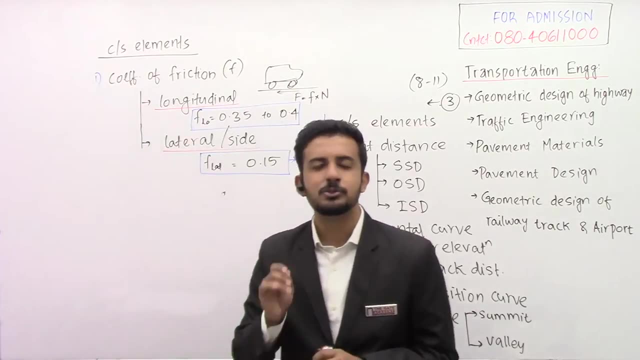 For one mark. See, just by hiding a value- 0.15, you are going to get one mark. A one mark can change your score and rank like anything. So don't take any topic as silly topic, Because you may be thinking. 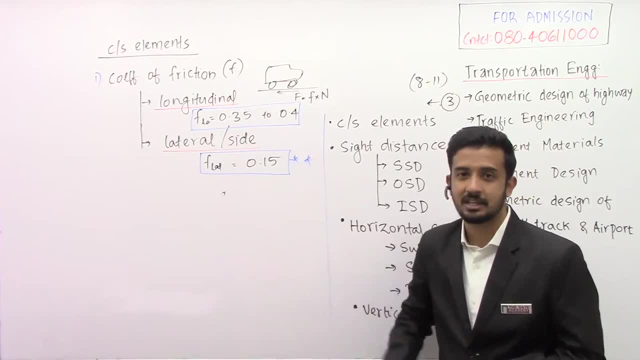 these are simple things. We have already studied in our plus two physics and all this friction, But it's not like that Very important. So many, so many basic things. they are fast for one mark, So take care of those things. 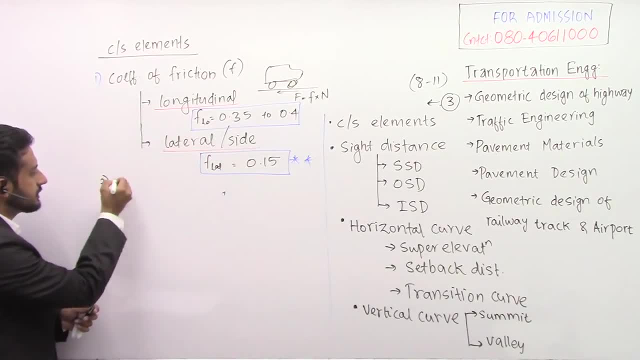 That are our friction. Then we are having the undulations, Or I can tell it as unevenness. So what do you mean by unevenness? You can note it down parallelly, What do you mean by unevenness? See, while you are riding your vehicle. 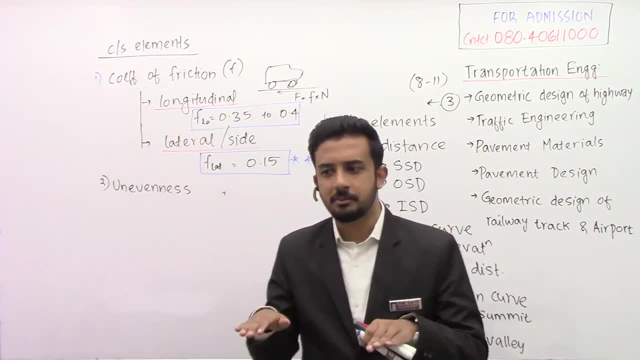 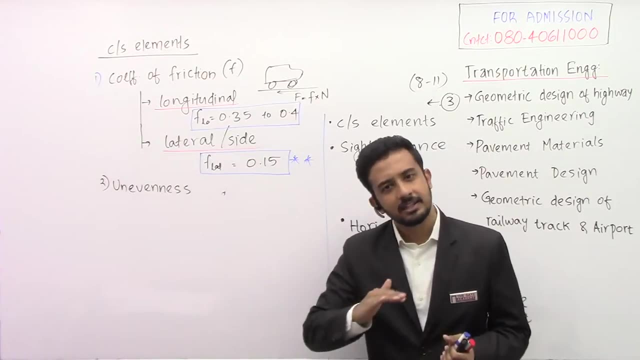 or you are going in some other vehicle. you might have experienced some see some undulations right, So you may be going smooth. If it is a national highway and all it's an important national highway, then the road may be smooth. 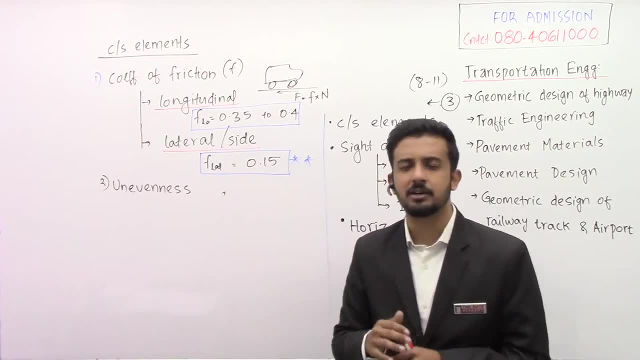 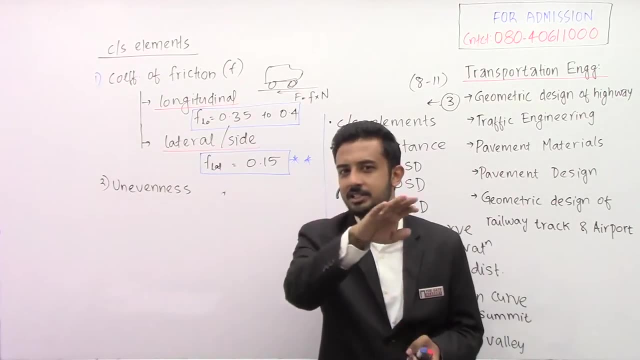 Otherwise, generally in our village road and all the road quality may not be that much good. Right Because of the improper maintenance and all, So sometimes you may be going something like this: Right Because of some undulations on the road. 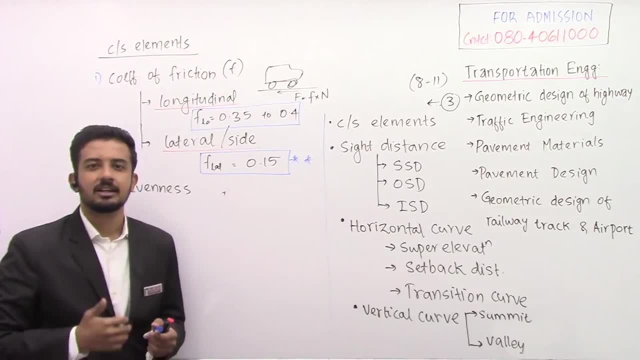 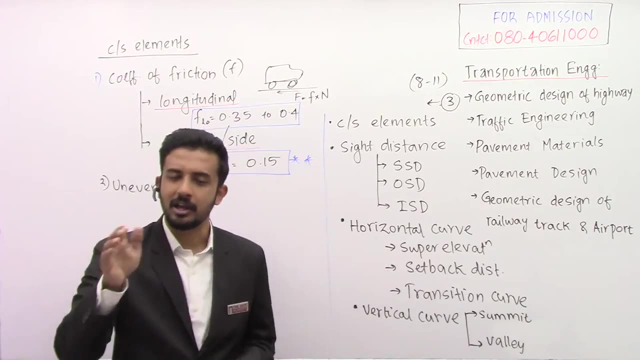 If the undulations is only little bit, then it's fine. What if it is very high? Then you may have some discomfort, Right. Also, the driver has to reduce the speed. You may have to lower the gears, So the petrol consumption also will be high. 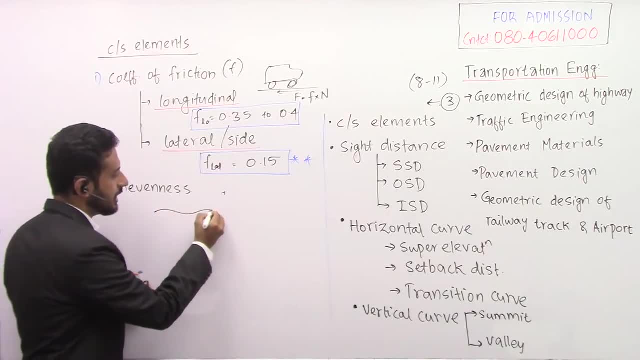 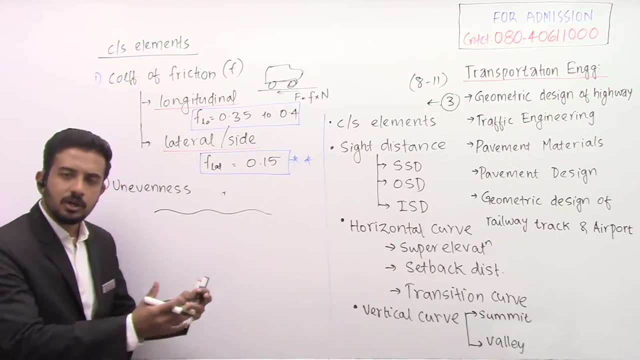 So much of problem will be happening Right, So that undulations, minute undulations. we are calling it as unevenness Generally. how we are going to measure this unevenness? We are taking a stretch of some 1 km. 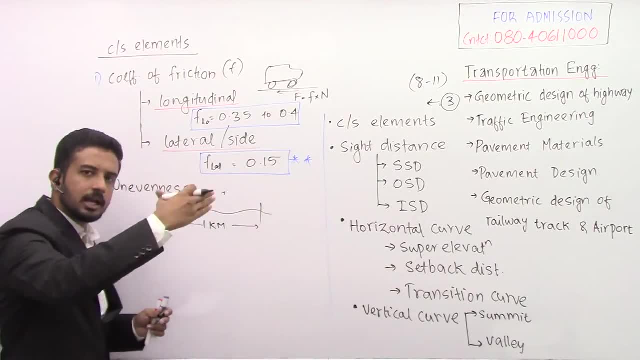 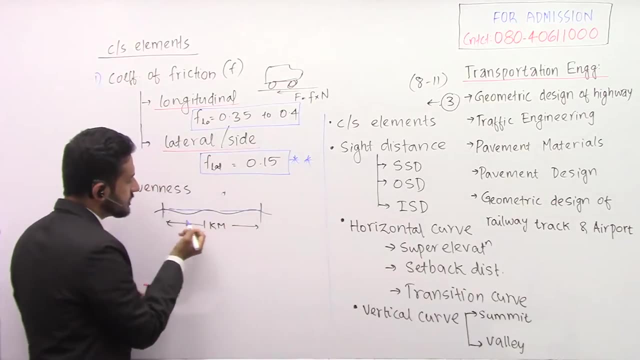 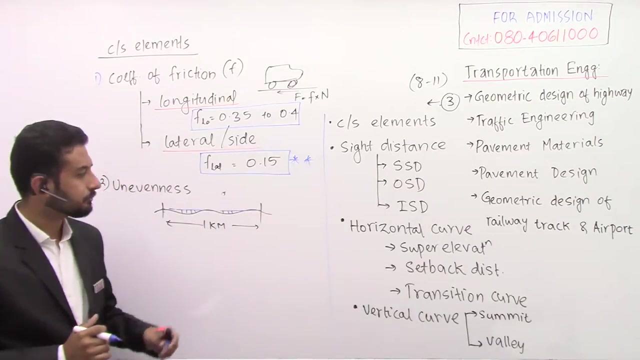 And in that 1 km, what is the cumulative undulations? See, at each point, maybe the road may be somewhat like this before, Okay, So at each point we are having some undulations Right And we are going to measure that. 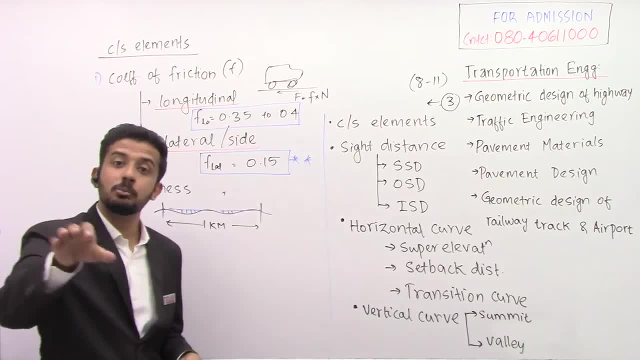 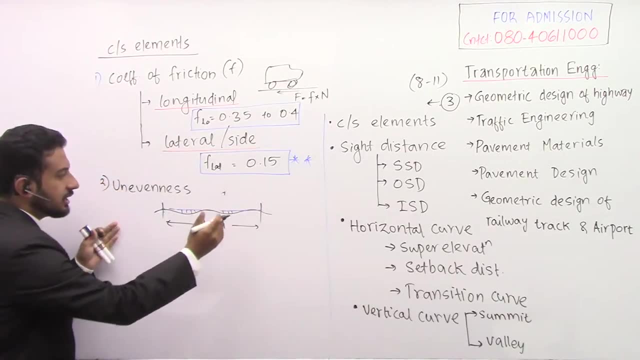 We are having some instruments. Using the instrument we are going to measure that, what is the cumulative undulations? What is the sum of these undulations in 1 km stretch? Okay, The instrument we are going to use for this unevenness is nothing but. 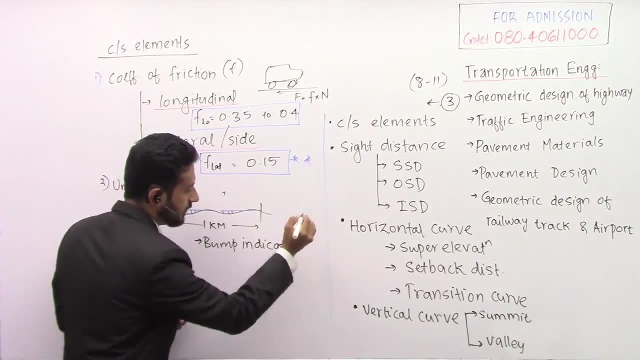 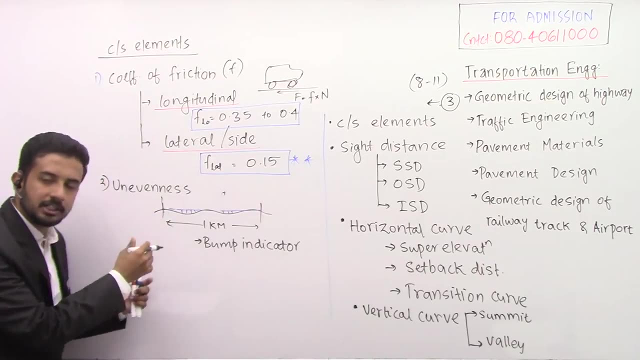 the bump indicator. Note those. note the name of the instrument. We are using the bump indicator And using the bump indicator, we have started measuring from this point And we are going through this road And whenever the 1 km stretch is ended. 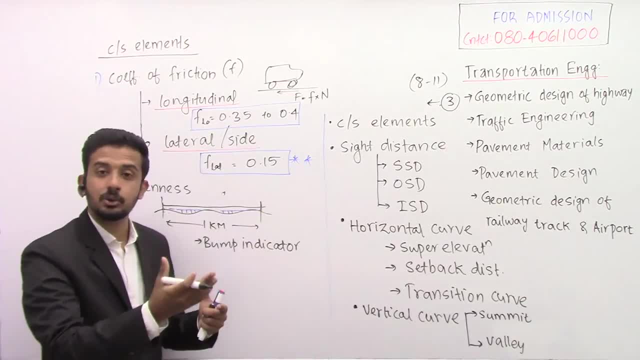 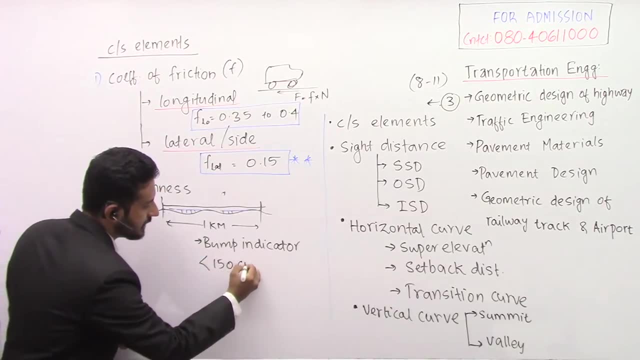 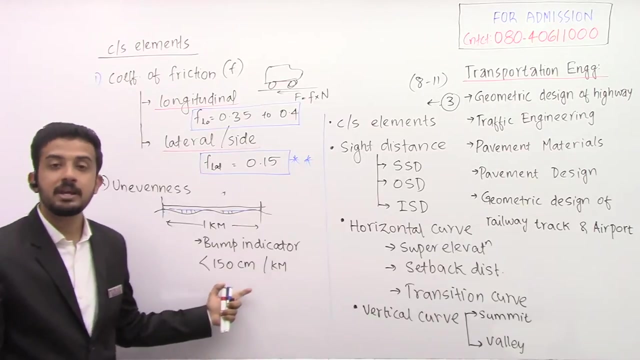 we are going to check what are the measured undulation value. The cumulative undulation value: That should be less than 150 cm per 1 km. Okay, This cumulative value in 1 km should be less than 150 cm per km. 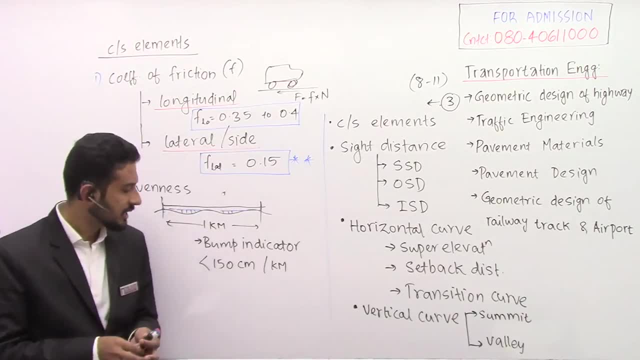 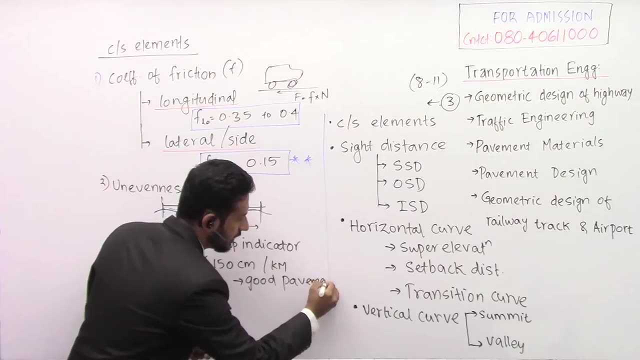 Okay, If you are referring the text books, you can see some other values also. The thing is, it is for some good payment, For a good payment, So note down the unit In case, if they are asking in terms of some mm and all, 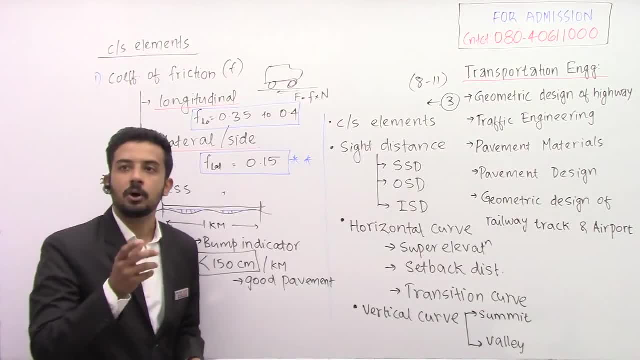 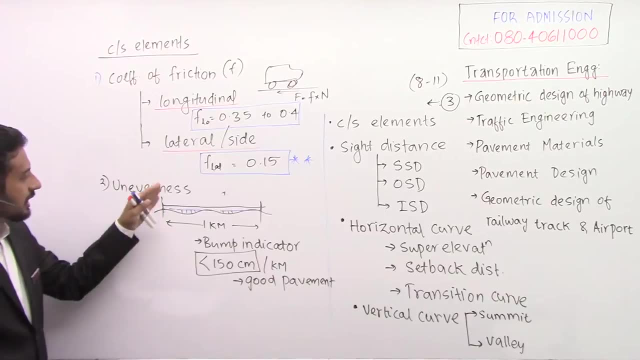 it will be 1500 mm. Okay, So always check the unit As already given this name: bump indicator, Very good. So these points you have to remember. I told you these are simple concepts But can be asked for one mark. 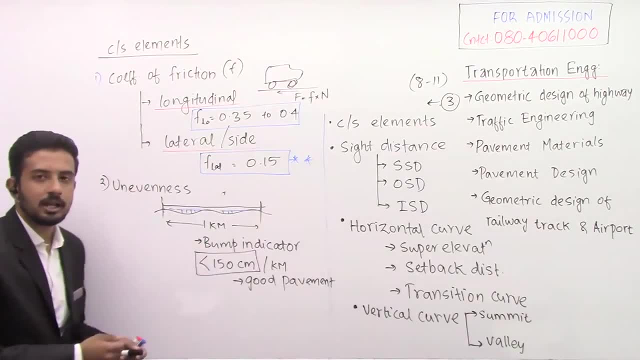 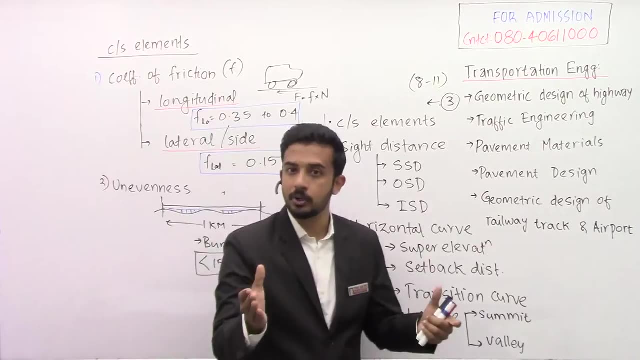 So the instrument name, you remember, and the value also, you remember. Suppose, if the measured value is more than 150 cm per 1 km, What it indicates? See, don't think that it is 1.5 m undulation. 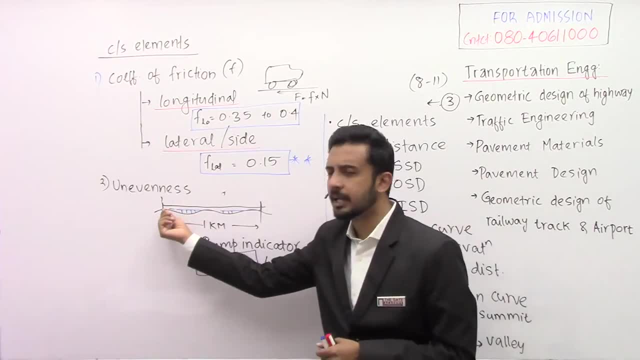 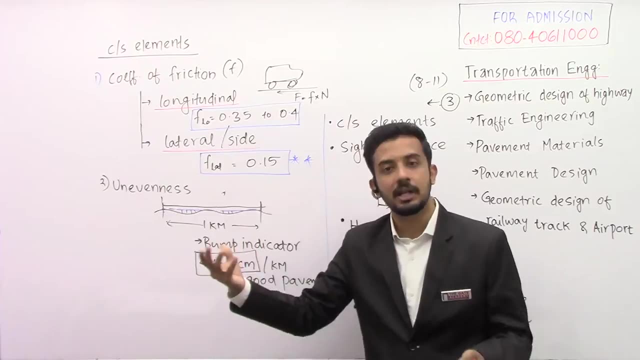 It is not like that. Cumulative value, suppose here some 10 cm or some 1 cm undulation only. Then I am measuring, measuring, measuring and I am adding that That's what cumulative undulation. Okay, So suppose it is beyond our limit? 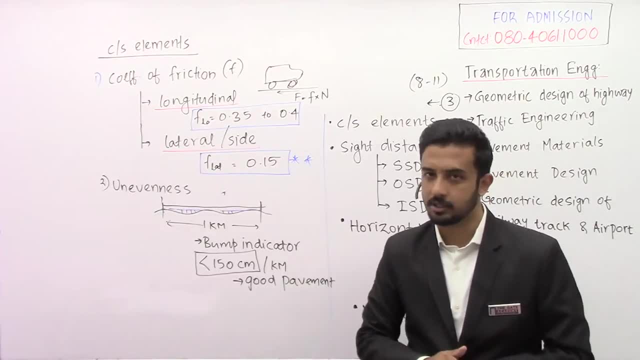 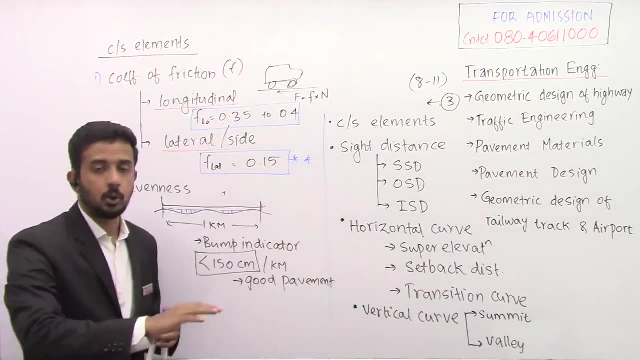 What we have to do. We have to do the maintenance work, Otherwise it is going to affect you. like anything, You will not be getting much comfort while riding. You have to lower your speeds. Definitely it is going to affect. So that is our unevenness. 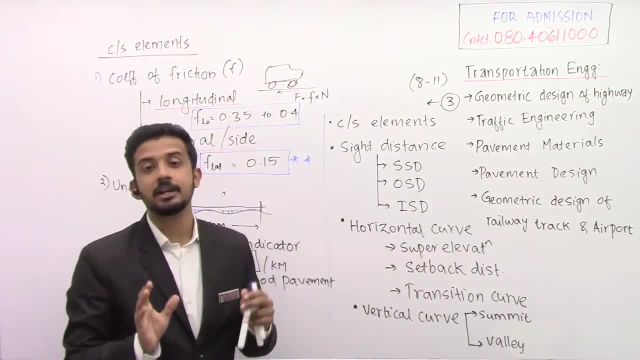 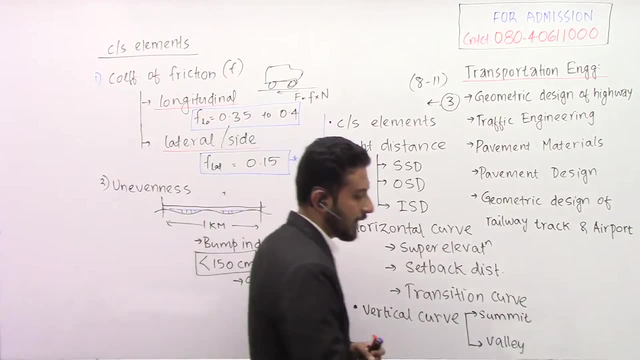 Then we are going into one of the important concepts from GATE exam point of view. That is nothing but the camber. Okay, So I am going to rub this portion. I hope you have already noted down these things, So I am going to write. 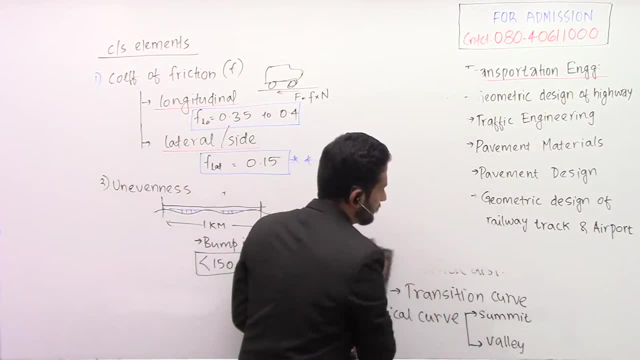 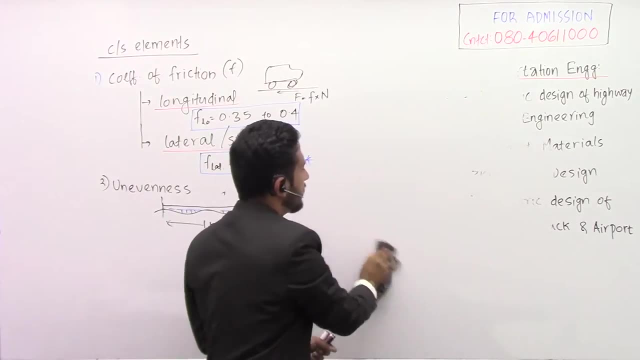 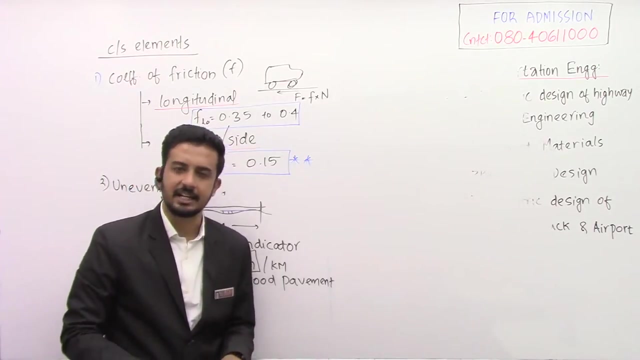 here Camber is nothing but the slope that we are going to give on the road surface Right. You might have already studied, But see, from naked eye we will not be realizing that there is a small slope on the road Right. 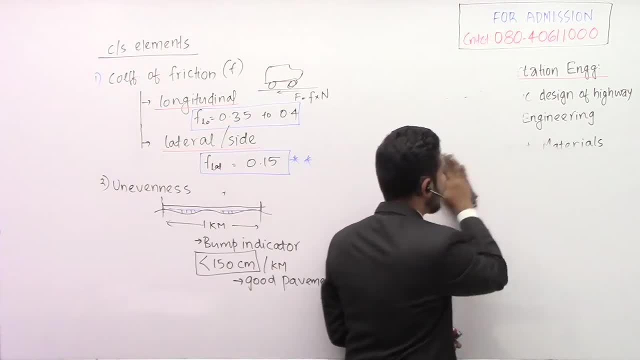 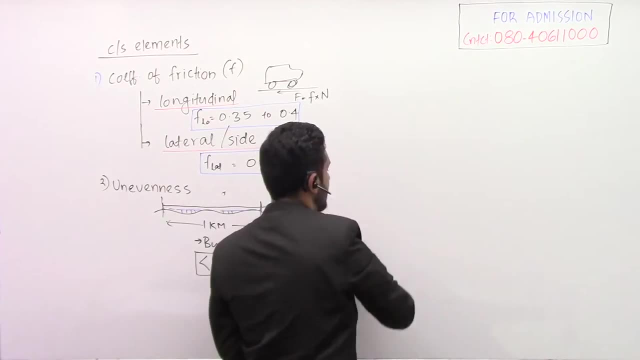 It may be some minute slope, only Some slight slope. It will not be that much high. That's why we are not From the naked eye. you are not able to realize that there is a slope. actually, It is nothing but a transverse slope, Not a longitudinal. 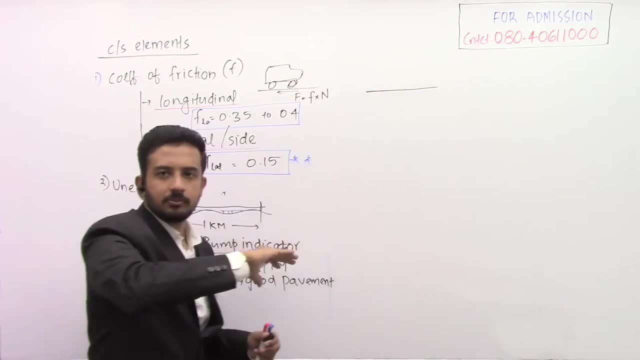 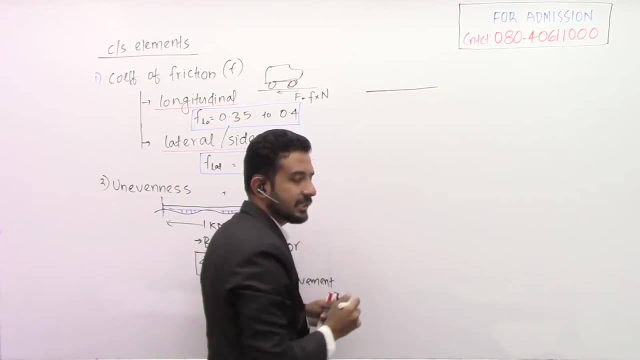 slope. Suppose. See, suppose this is the cross-section you are seeing towards the board. So this is the width of the road, And actually it will not be like this horizontal. Suppose this is your horizontal plane. The actual road may be something like this: 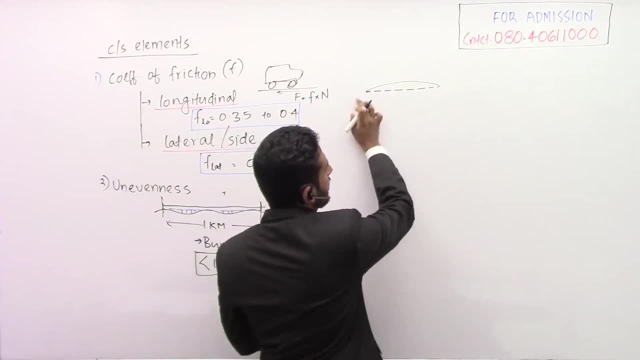 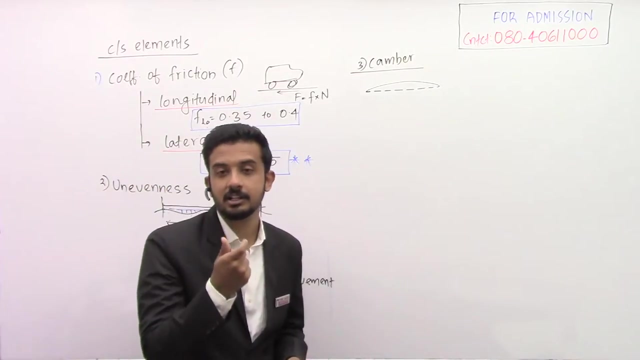 Okay, It is called as that slope. That transverse slope is called as camber. So that is our next one, Camber. Okay, So that transverse slope, See for gate examination. even that definition is asked. 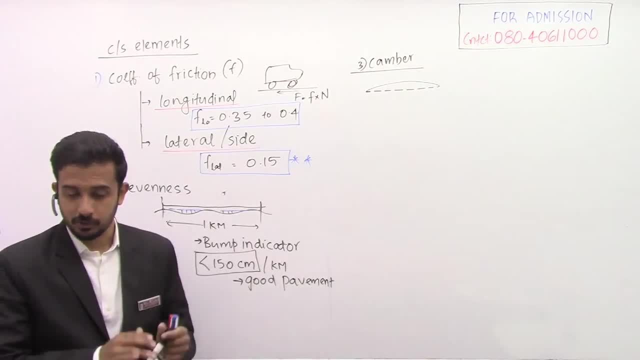 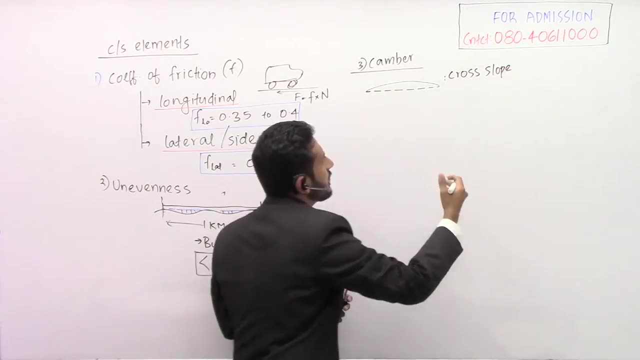 For one mark. What is the longitude, Sorry? What is the cross slope? It is nothing but the cross slope Or transverse slope. I can tell. So the cross slope provided on the road is called as dash. They have given four options. 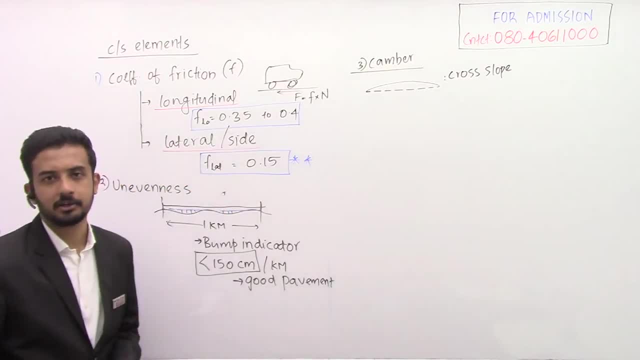 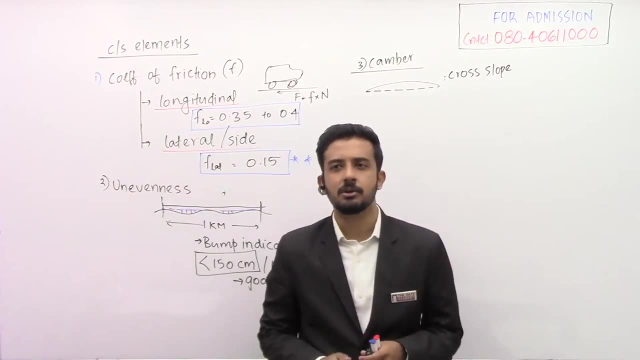 One option was camber. Even the definition is asked for one mark. Okay, See why we have to give a slope over the road. If it is a plain road, that is better. no, Why we have to give a slope. 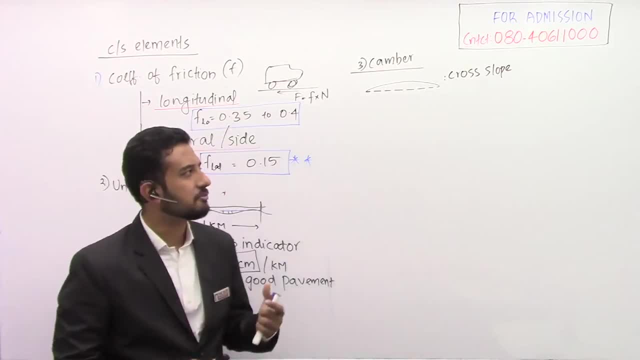 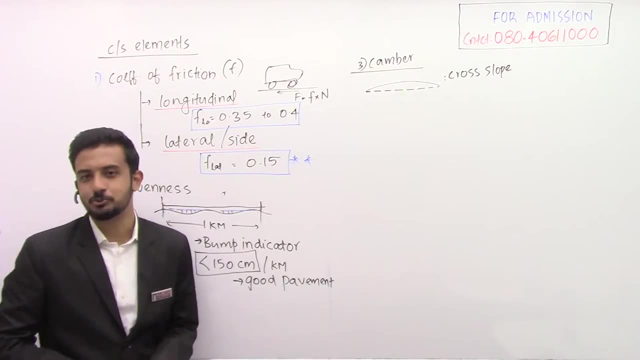 Just tell me What is the necessity of giving a slope, A cross slope, What may be Very good Abhishek, Drainage purpose, Very good, See, suppose rainfall is happening. Yeah, Yeah, Good, Debashish Good. 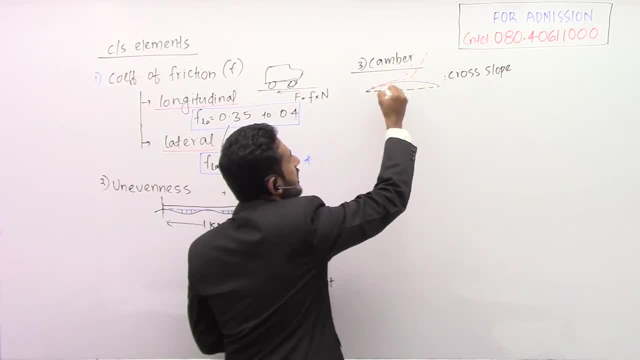 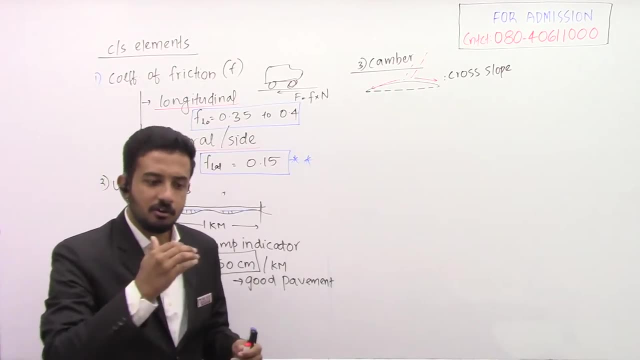 So if some rainfall is happening, it has to drain off to this side. Right, It has to drain off to this side. Side drains may be there, Drainages may be there. First, the water has to reach to the drainage, Right. Yeah. 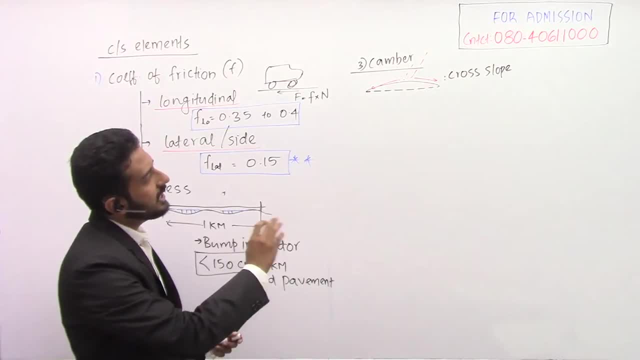 Very good, Abital Varun is also giving the answer. Very good. So that water: first it has to reach the side drains, Then only it can go Right. So first it has to reach there. That's why. 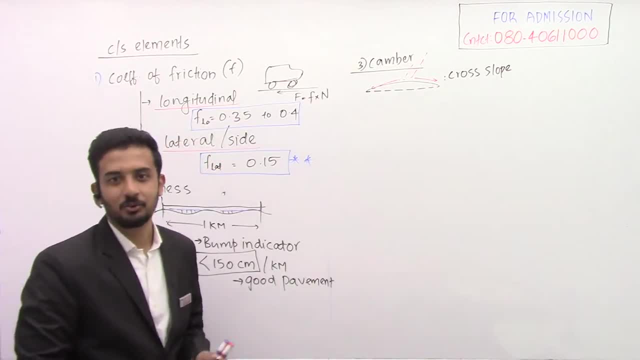 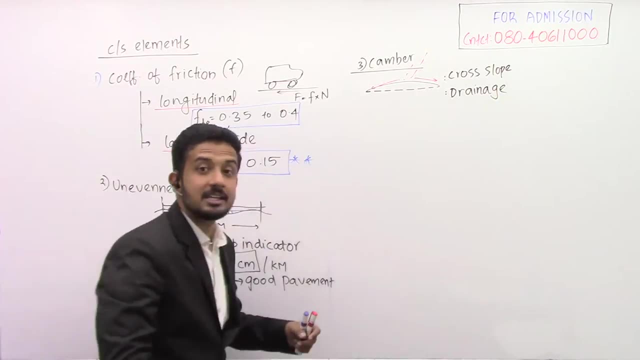 we are giving the camber. So that is also a gate question Why we are giving the camber. It is for drainage. So all the important concepts of camber is asked in the gate exam, So can be asked again. Okay, 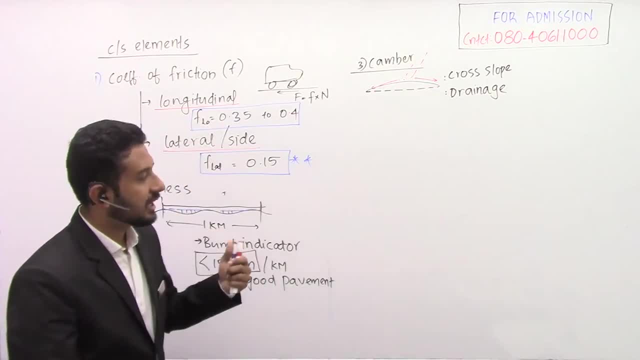 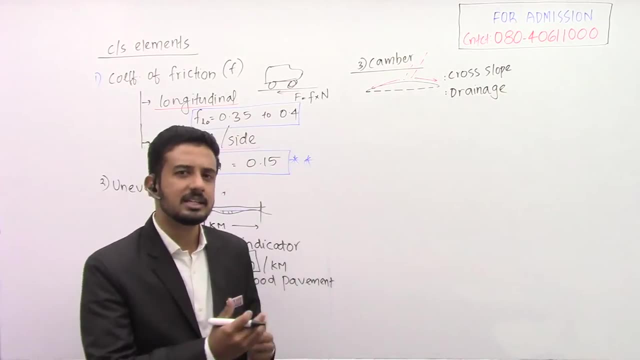 And some numerical portions can also be asked in this camber. Some other theory concepts are also asked. I will give you that also And some numericals also. we will see There is a chance they can ask a numerical question also from this particular concept. Okay, 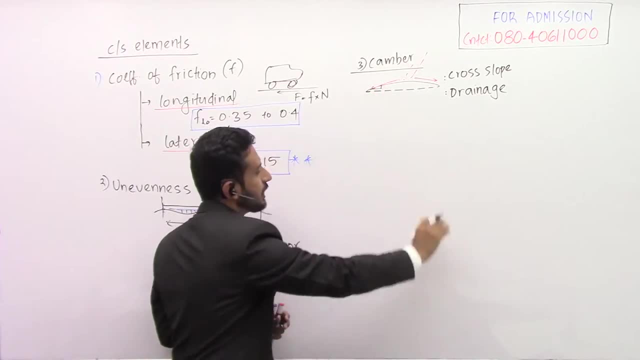 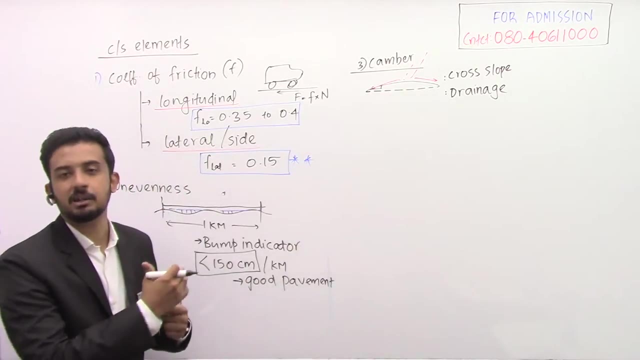 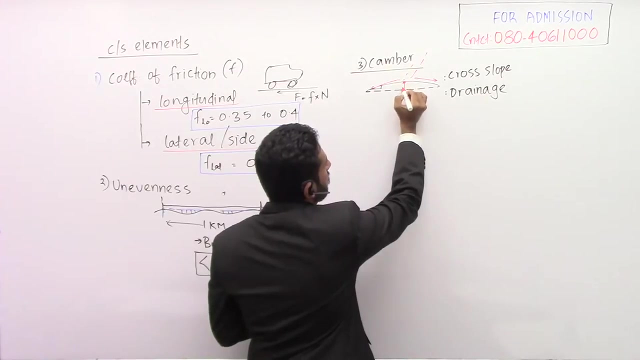 So what is the camber, This particular slope? So there are two concepts for this particular concept of this cross-sectional element. camber One is: what will be the height of this highest point? What will be this highest point? We call that crown. What do you mean by crown? 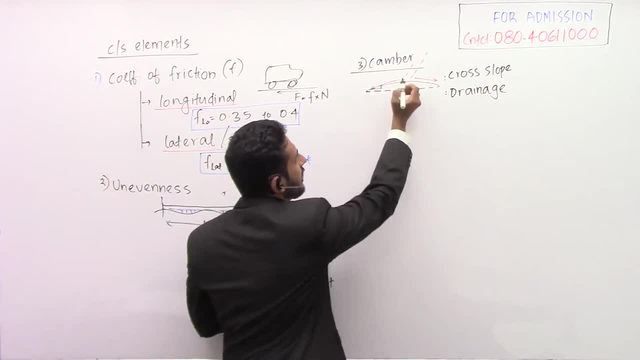 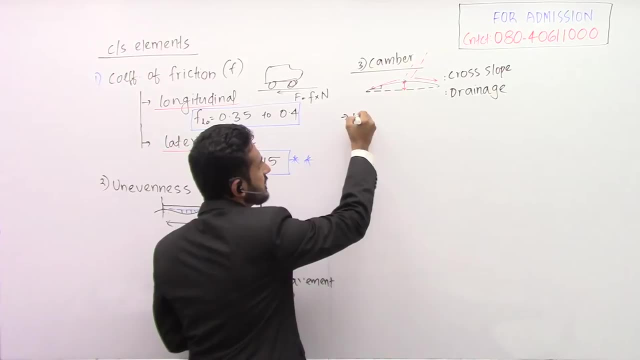 The something we are putting on the head Right. So this we call it as crown point. So either they can ask you what is the height of a crown, So first concept is height of a crown, Either they can ask you that. 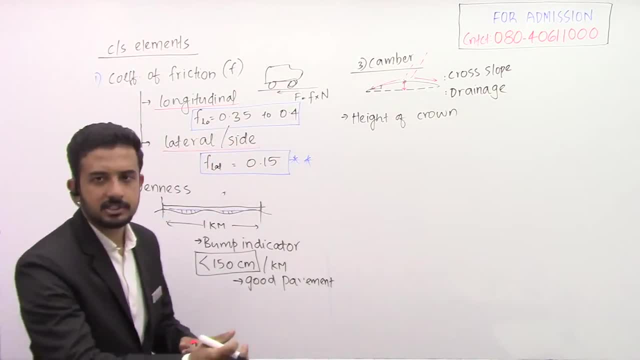 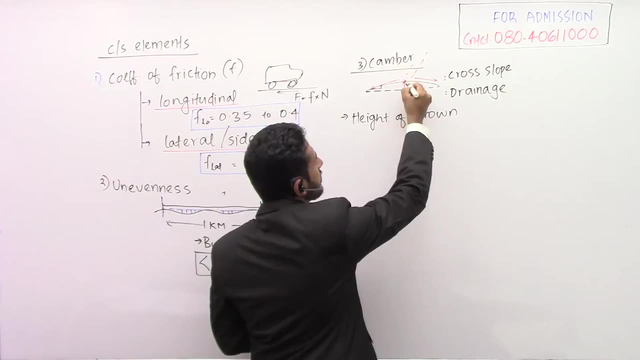 or there is one more concept I will give you after some time. So first we will see this height of crown. So what is this height of crown? Nothing but this height W. I can, I am just denoting as Yc. 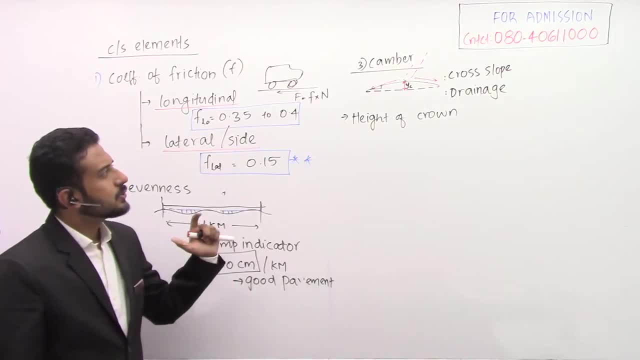 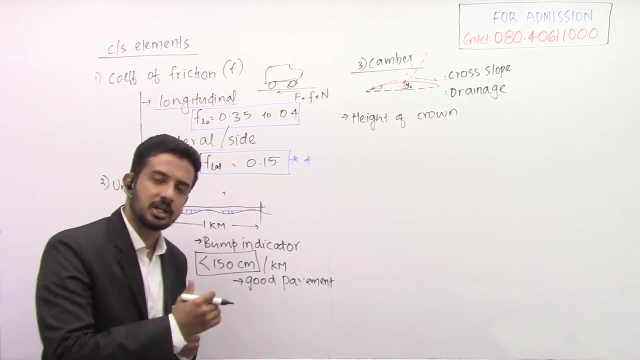 Height of the crown C. Okay, So depends on the shape. actually, the equation of camber is going to change If it is a parabolic camber, if it is a straight line camber, the equation of the camber is different, but the height of the camber 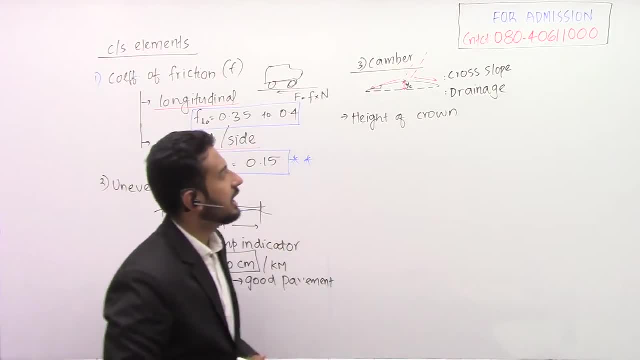 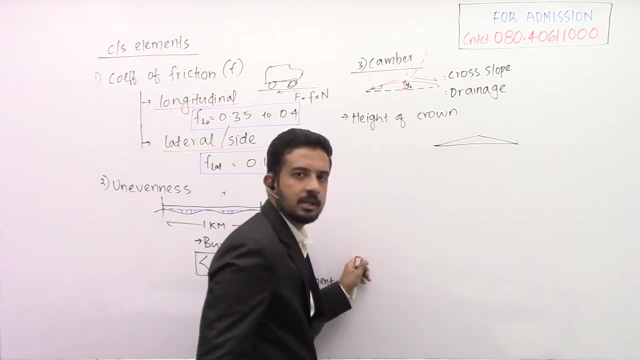 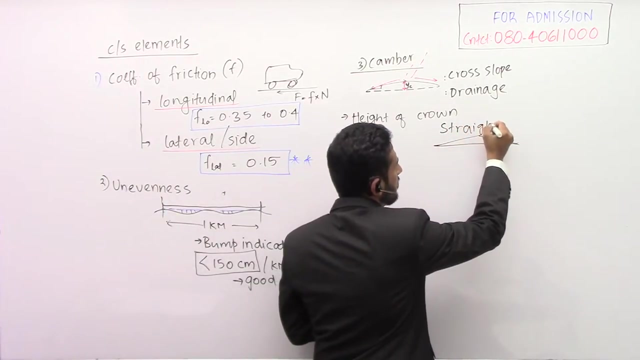 is. height of the crown is same. I am telling it once again: A camber can be a straight line camber, which means these are straight line portions. This we are calling it as straight line camber. So it can be a straight line or straight. 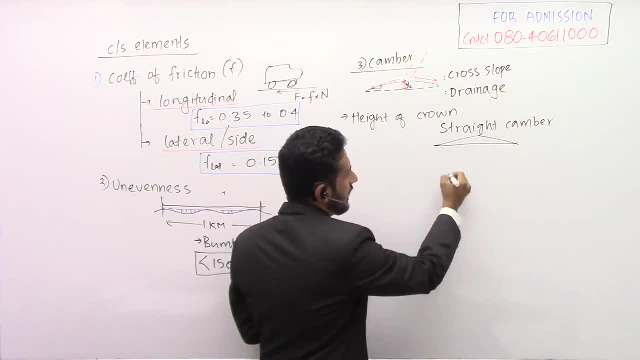 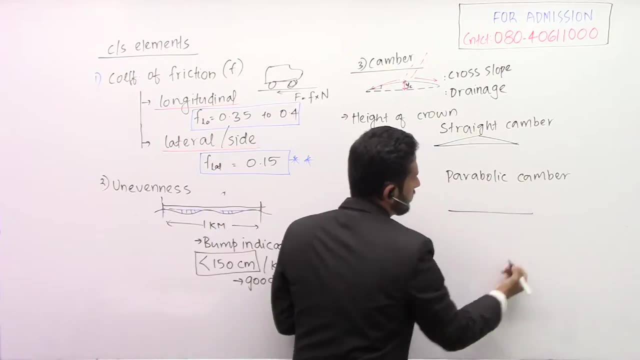 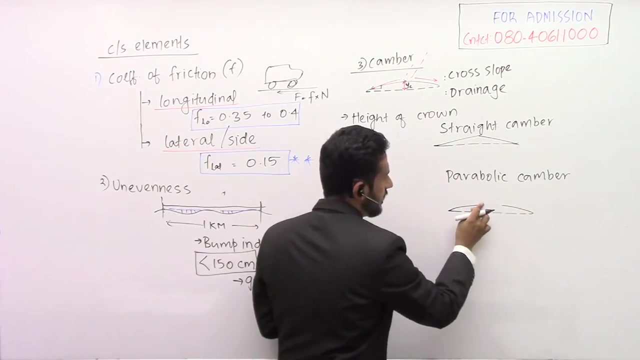 camber. It is a straight camber and sometimes it can be a parabolic camber also. What do you mean by a parabolic camber? then This is our horizontal line. This is our horizontal line. Then it will be something parabolic. Okay. 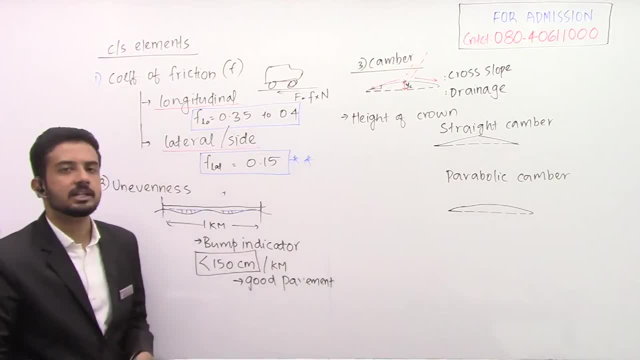 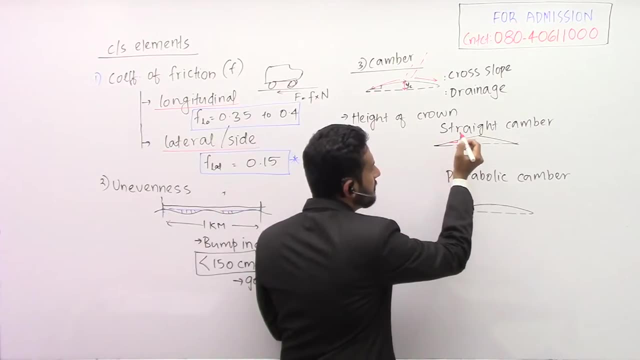 So it will be something like this: So this is parabolic camber, that is straight camber. Okay, Yeah, Good, Good, Already they are giving the reply. So suppose I am telling the slope is 1 in n. 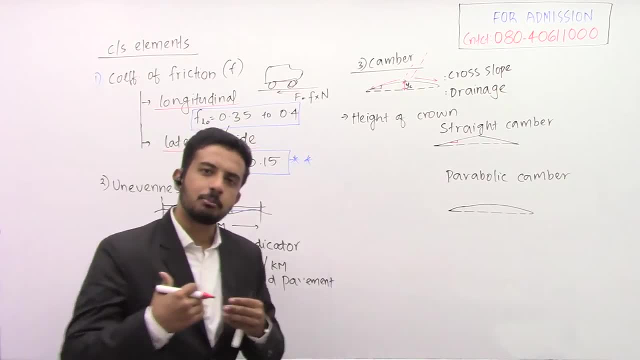 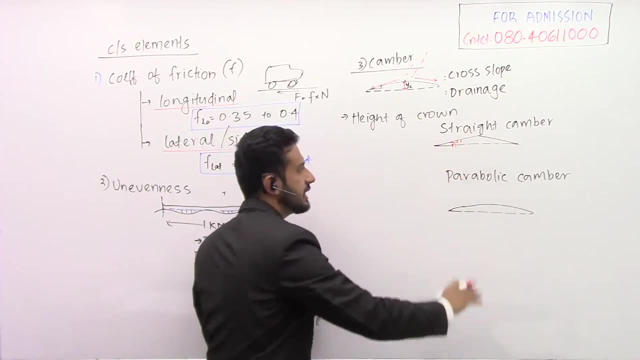 So what do you mean by 1 in n? If you are moving n meters horizontal, you will be getting 1 meter vertical, Right, So this is 1, this is n, Suppose that is the slope. Okay, So I am telling, if 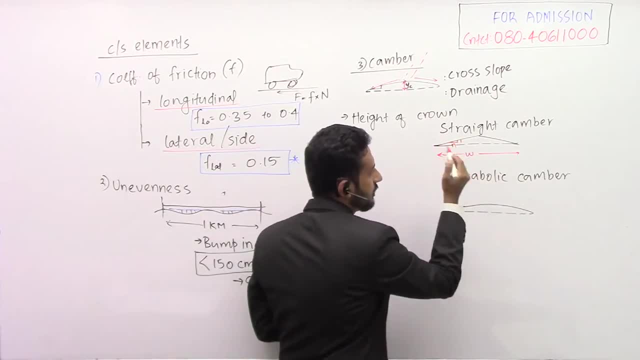 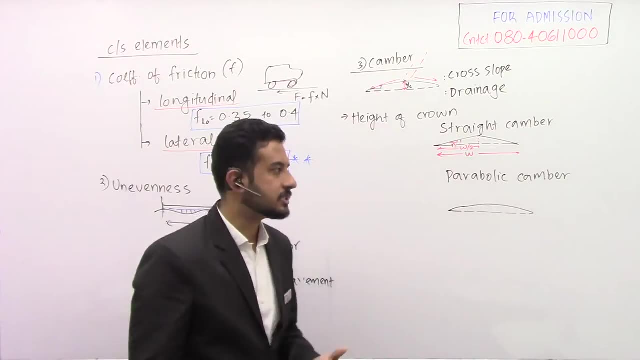 width of the road is w. Width of the road is w Till this crown. what will be the depth? What will be the width? W by 2.. Right For n horizontal for n horizontal, you are having 1 vertical. 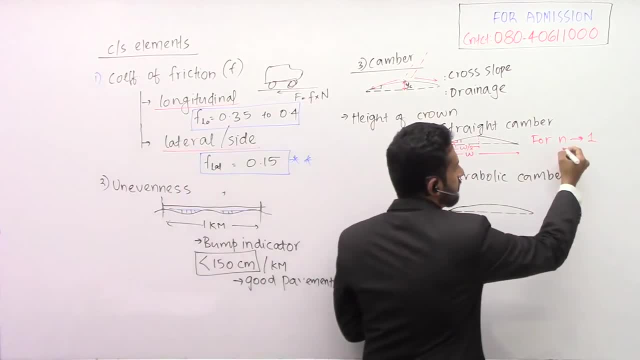 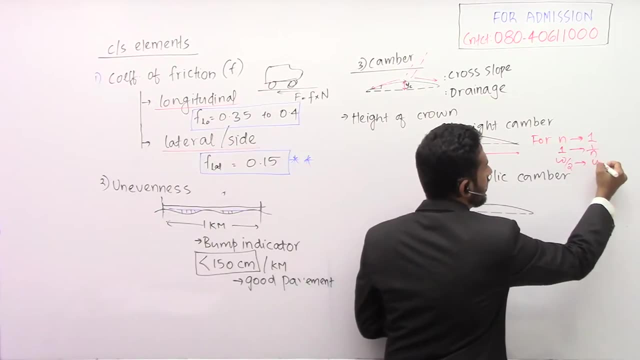 Right. For n horizontal you are having 1 vertical. Then for 1 vertical you will be having 1 by n vertical. Then for w by 2 horizontal, how much you will be having w by 2n Right? 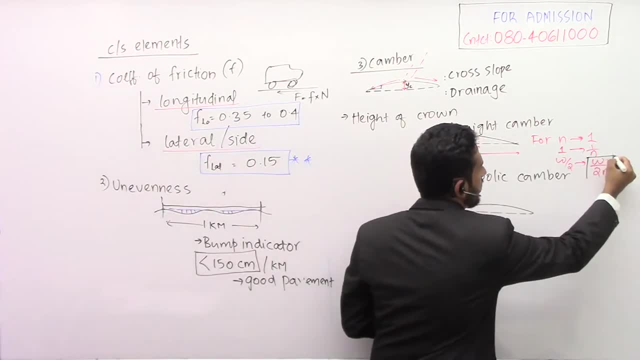 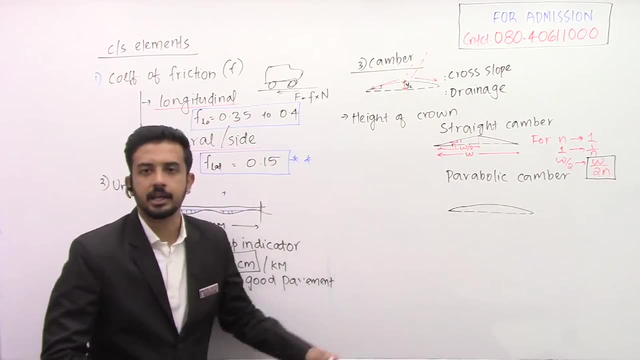 It is nothing, but the height of the crown will be. how much Height of the crown will be w by 2n? What is that? w? Nothing but the width of the road. I will write again: n is nothing, but if the slope or if the 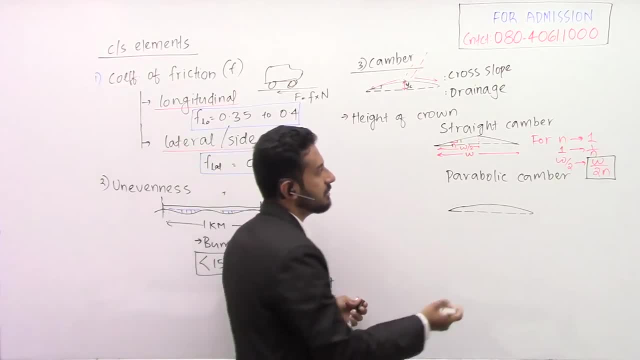 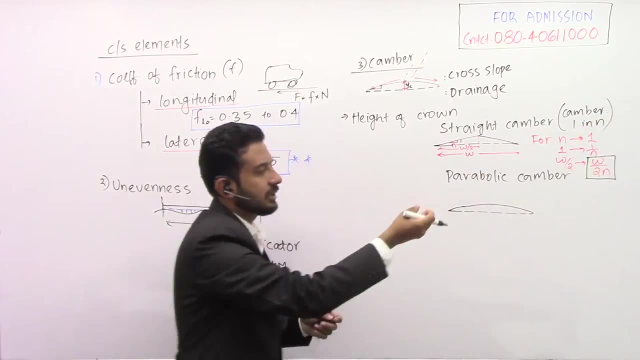 camber is 1 in n. If the camber is 1 in n- Suppose the camber is 1 in n- Then n means what? In that equation, w by 2n, n means what The 1 in n We can represent. the 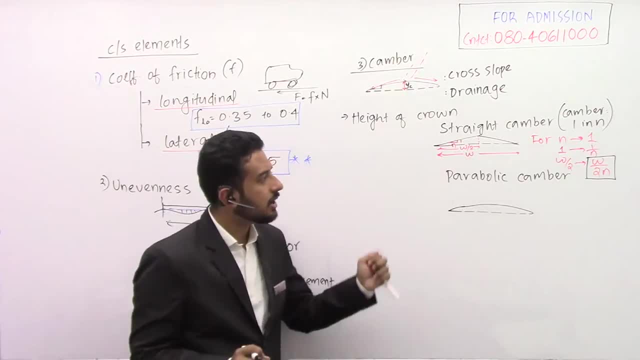 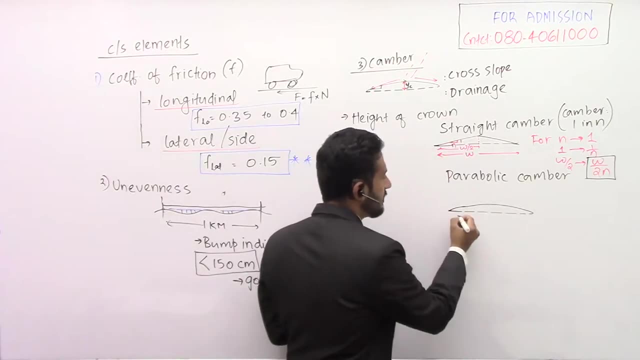 slope either in terms of percentage, or in some decimals, or in 1 in n term Right. So parabolic camber. there is an equation for parabolic camber. If I am taking a distance x from here, correspondingly, I am just telling. 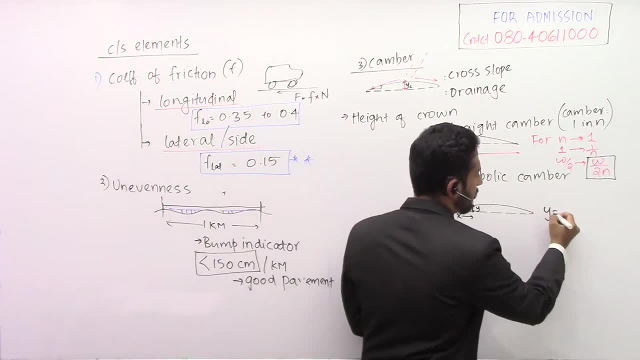 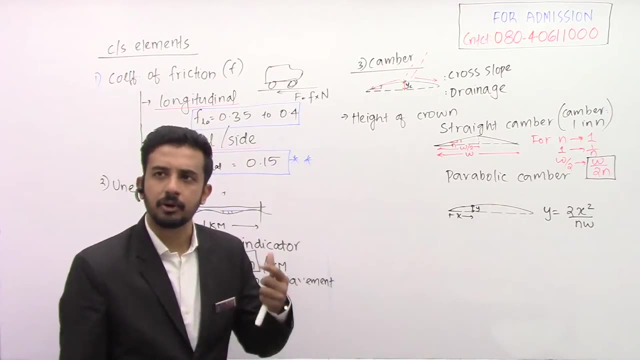 that that is y. There is an equation for parabolic camber. y will be equal to 2 x square divided by n? w. That is a standard equation for any horizontal distance, x. The height of the camber will be 2 x square divided by n w. 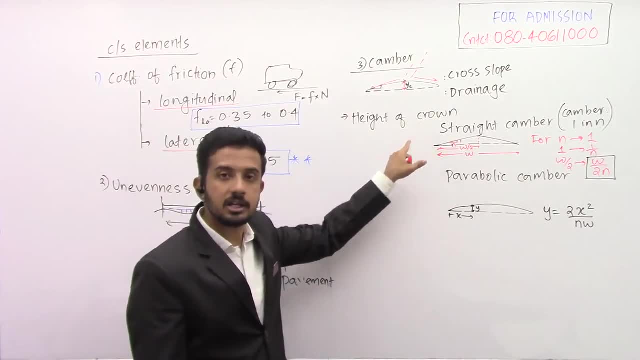 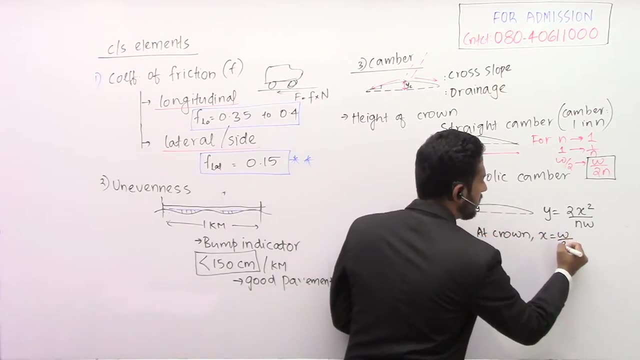 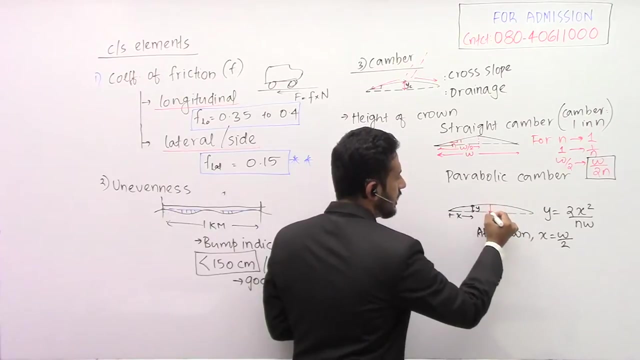 But we are interested in height of the crown. Height of the crown means what? What is the distance of x? x will be equal to w by 2.. Right Crown means what? At the center portion? So if the total width is w, 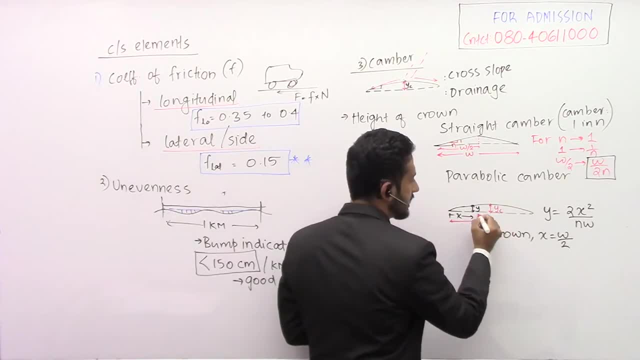 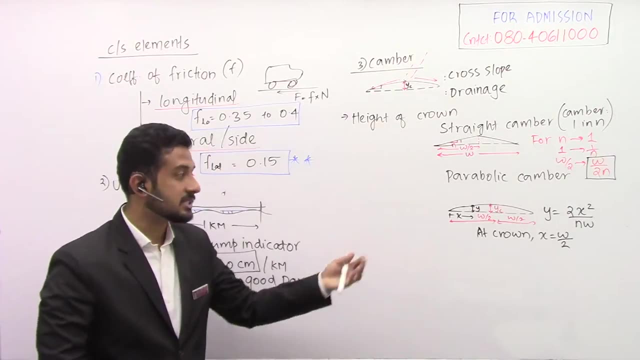 this is our y of crown. So till here. what is the x distance? w by 2.. Remaining portion is w by 2.. Like that, Okay. So x is w by 2.. If you are substituting the value, 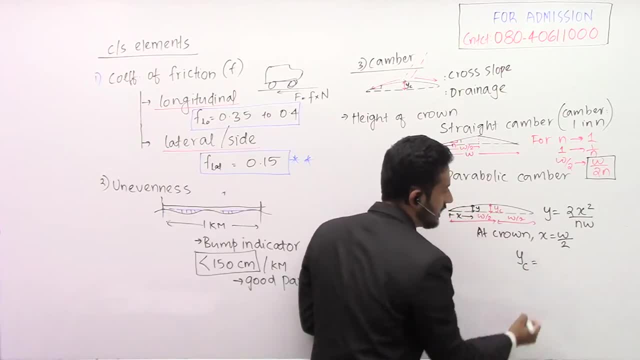 of w by 2. in this x you are going to get yc, What it will be: 2 into w by 2 square divided by n w, Right? So if you are calculating what you are going to get, so just check it. 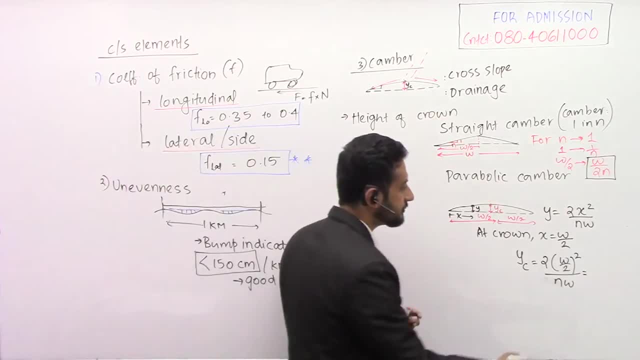 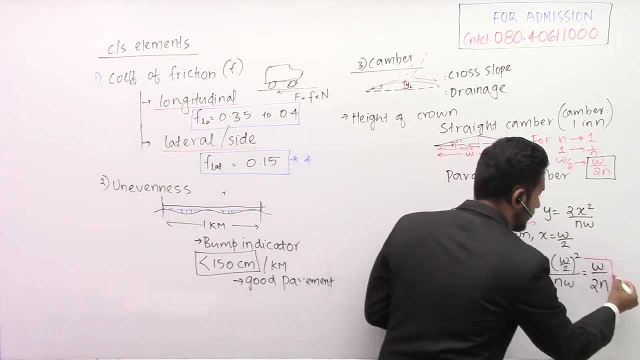 If you are substituting w by 2, what you are going to get- Just check it. You are going to get w by 2n, Right, The same equation you are going to get for height of camber if it is a straight. 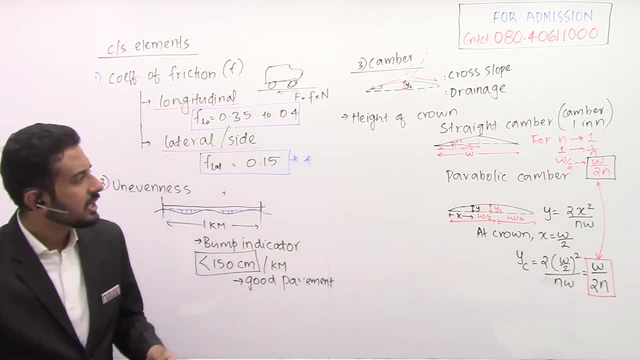 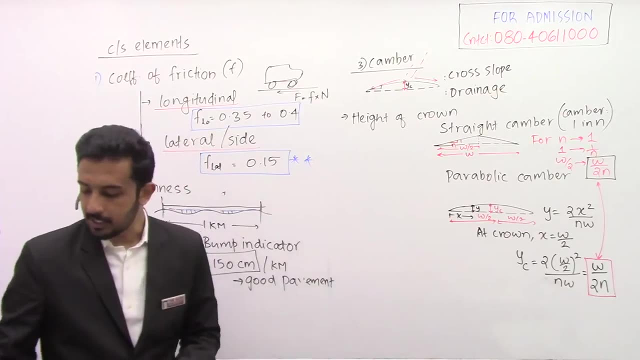 line camber or parabolic camber? Okay, There are some disadvantages for that shape: straight line, straight camber. Yeah, Very good, Devbashish For parabolic camber. also, we are having some disadvantages. Okay, So, practically. 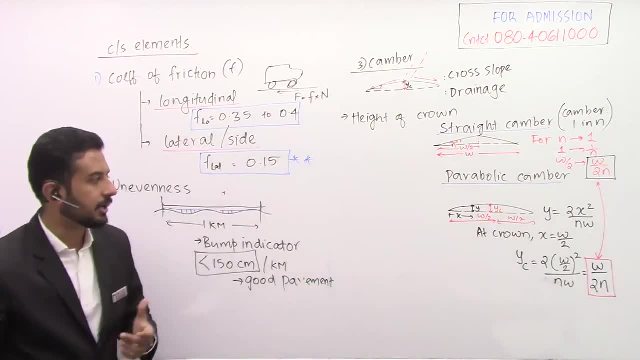 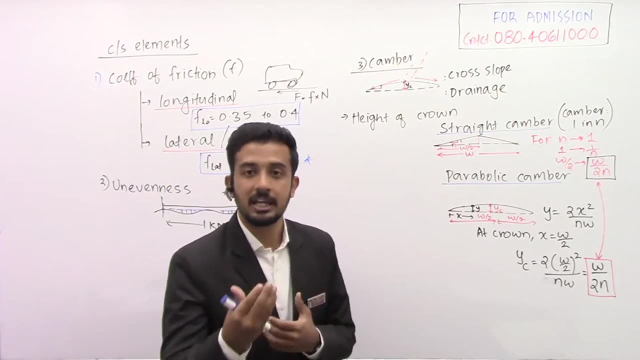 we are giving a combination shape of the straight line camber and parabolic camber. See what is actually the disadvantage For gait examination. they may not be asking Just for your information. for your knowledge, I am telling: Straight camber is actually. 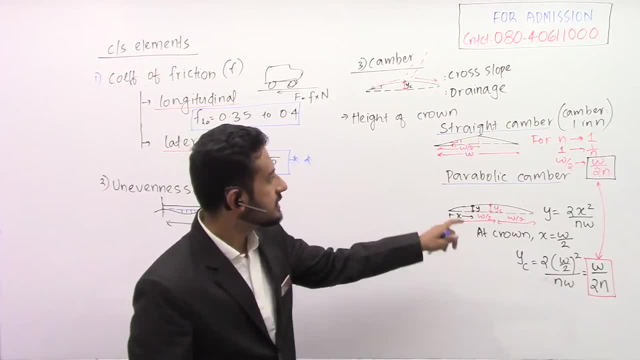 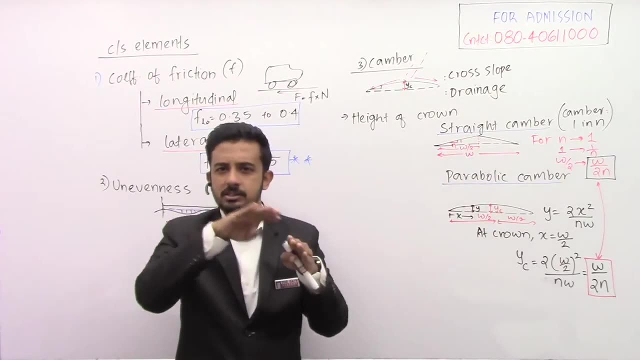 will affect the fast moving vehicles. See, fast moving vehicles means they have to overtake, Right, Just assume here what it is there: Some corner, some pointer shape On the center of the road Right, See, just imagine you are going in your car. 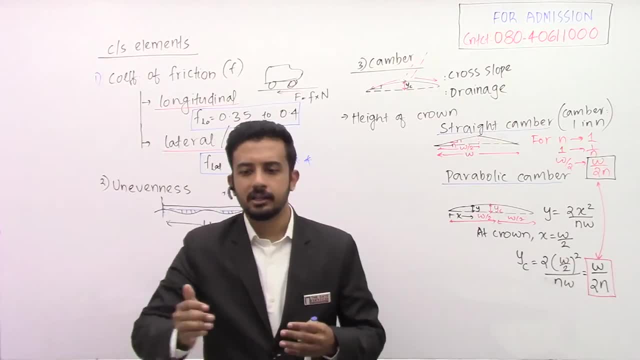 One auto, risha, is there You want to overtake. Whenever you are overtaking, you will be using the center portion of the road, Right. What if there is a pointer shape like this? Definitely you are going to get some discomfort, Right. 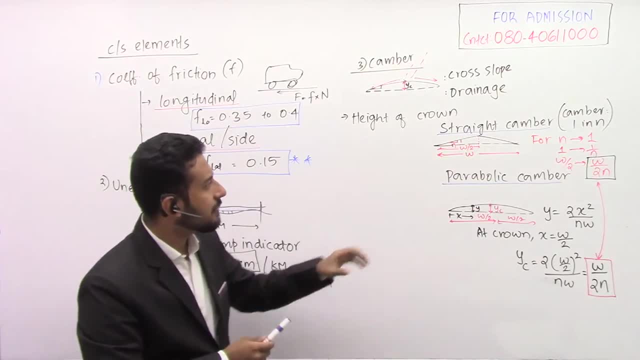 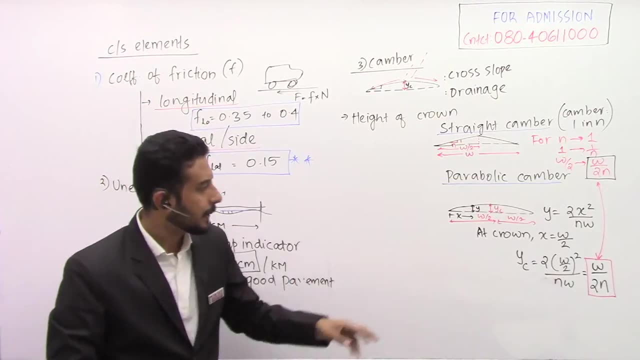 So higher, the faster moving vehicles will be having some problem on straight roads, straight camber roads. What is the problem for parabolic camber? If it is a parabolic camber, it is good for high speed vehicles. Right, It is a smooth curve. 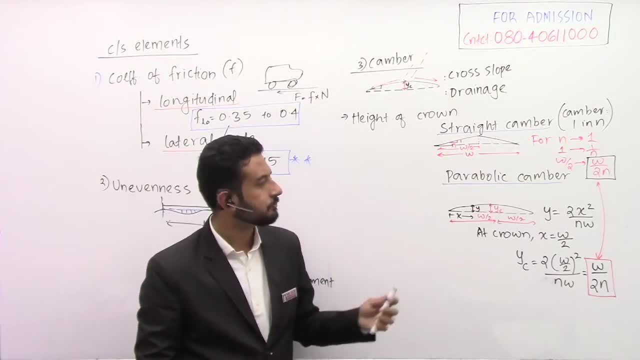 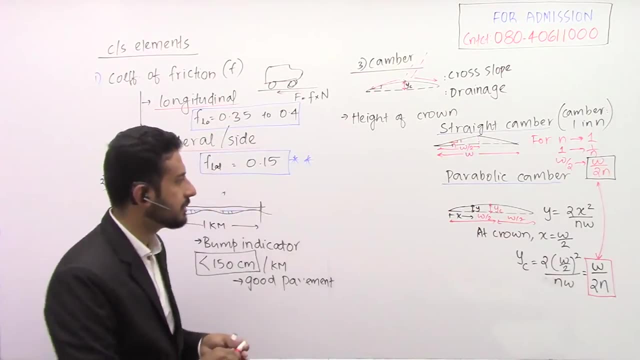 So easily you can overturn and all You will be having much comfort. But the problem is for parabolic camber. here it is having more slope, Right See, which is having more slope means more slope in the sense at the edge. 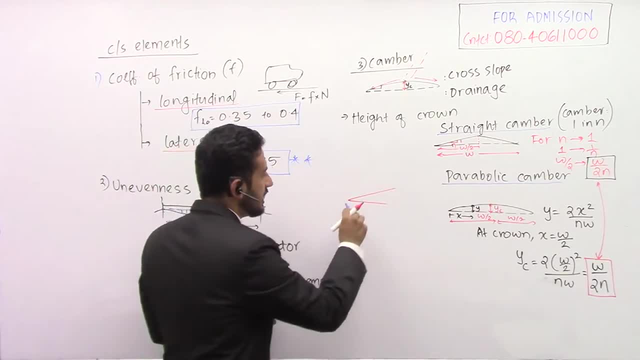 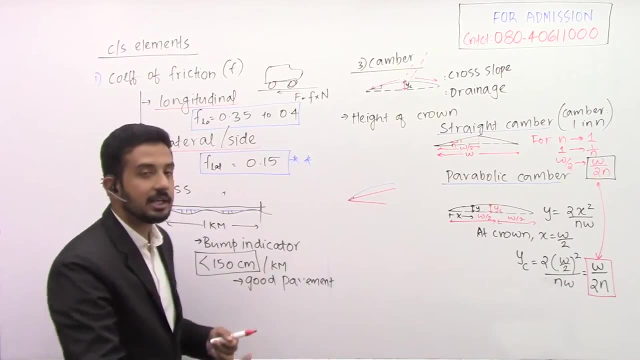 If it is a straight line camber, the side is like this. If it is a parabolic, it may be something going like this: No, So more slope at the edge is happening for a parabolic camber. So for: 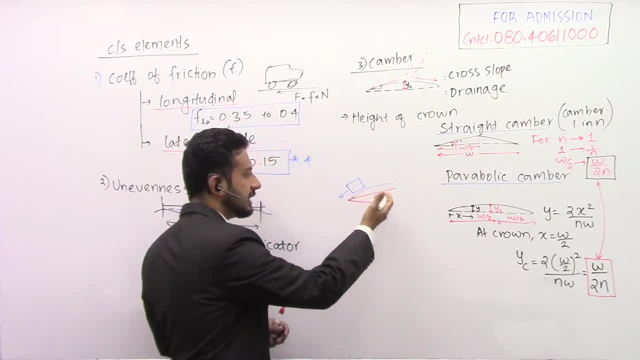 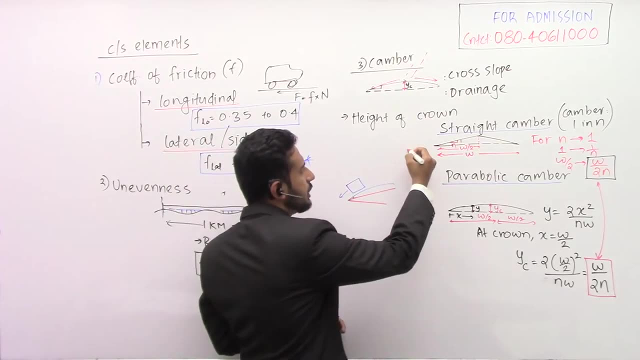 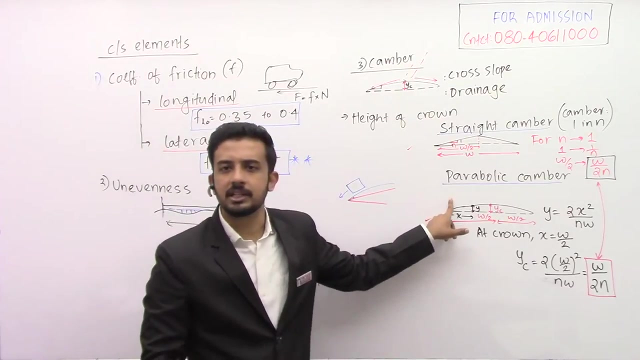 slow moving vehicles. there is a chance that they may be coming out of the road Towards the inner side. they may topple. Okay, So this is disadvantage for high speed traffic. This is disadvantage for slow moving traffic. Why slow moving traffic? this is: 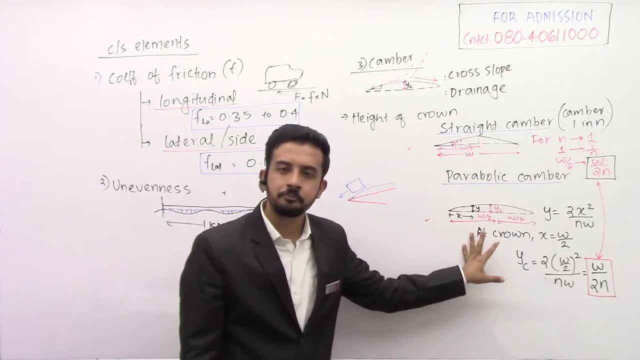 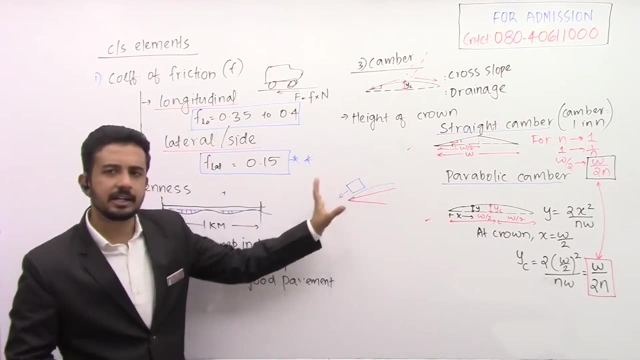 advantage It is having some more slope compared to straight line at the edge portion. Okay, At the edge portion it is having something like this: So if a truck is there, something like that Truck is there. So some small 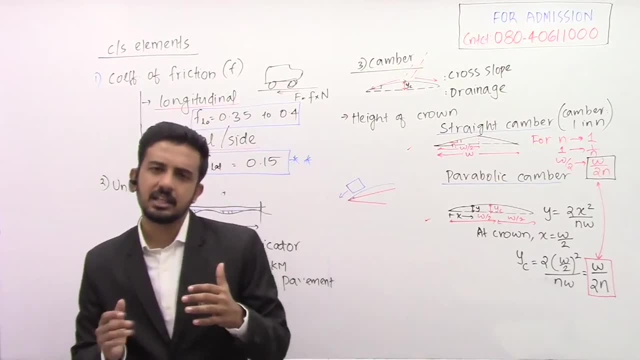 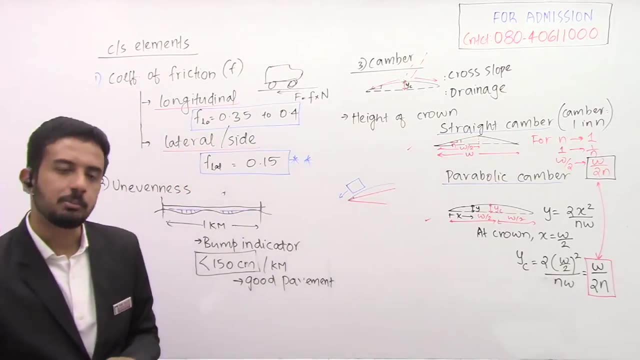 slowly moving vehicle is there, There is a tendency. there will be a tendency for those vehicles to come towards the inner side of the road. Okay, So that is why, practically, we will be using the straight line camber and the parabolic camber. 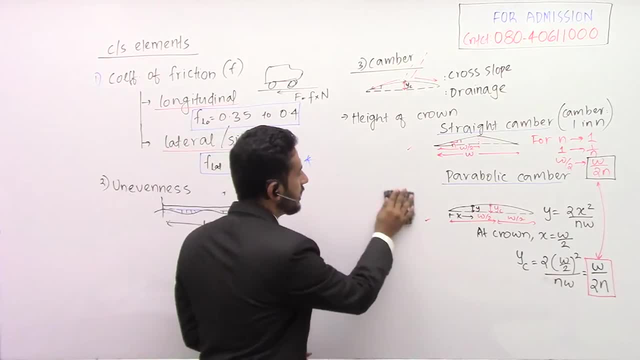 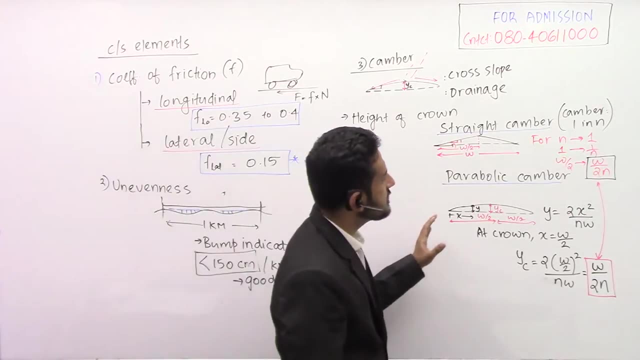 Okay, So remember that equation W by 2N very, very important. They can ask you some numerical questions for that. Okay, Now see, most of the time they may be giving you the value of W. What is the width of the road, Suppose? 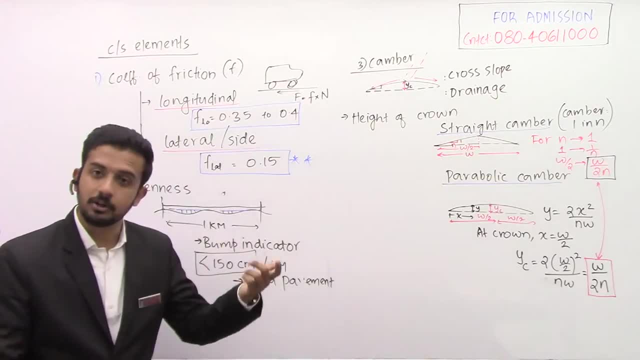 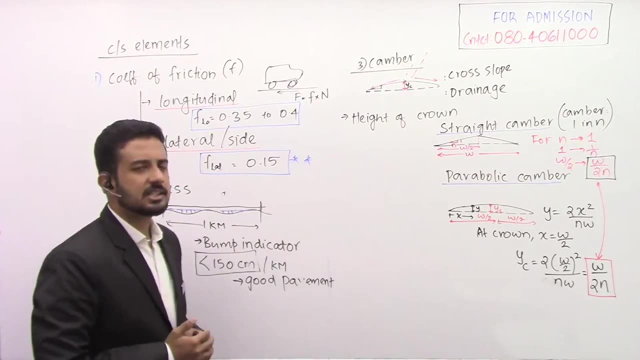 if they are not giving you the value of the road, sorry, the width of the road, you have to substitute that. So IRC, Indian Road Congress, IRC is giving you know, IRC is giving all the specifications for right. 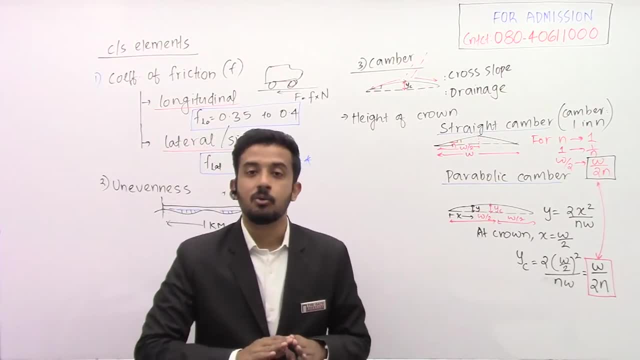 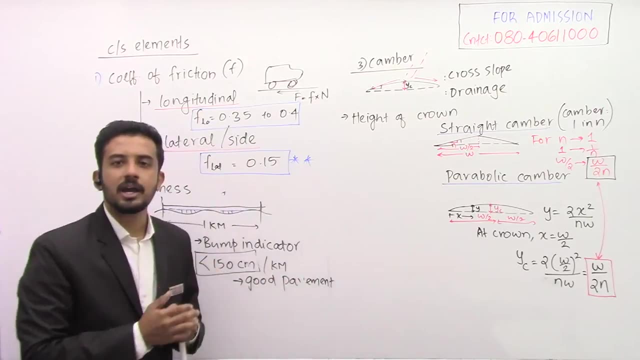 What are the rules you have to obey, What are the specifications, What are the values you have to take for each parameter? Everything, IRC is only giving us right. So, according to IRC, there are some minimum value of the width of the. 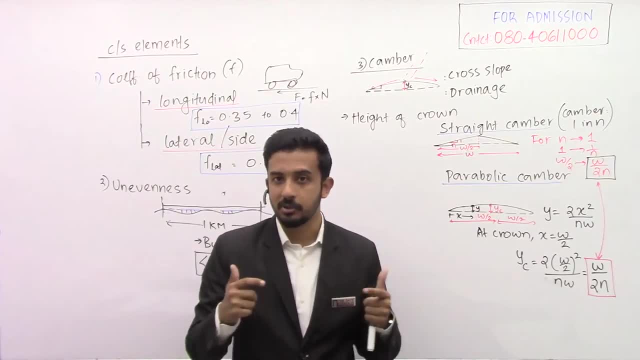 road. If it is a single-lane road, how much should be the width? If it is a two-lane road, what do you mean by two-lane? Vehicle will be going in this road and one more lane will be there. 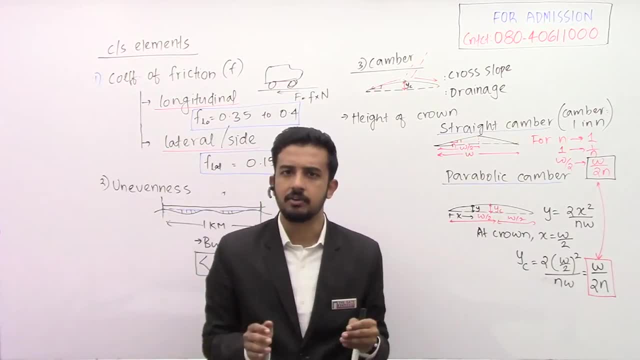 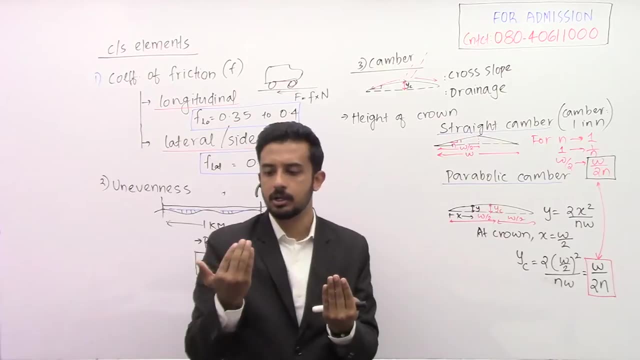 So if it is a two-lane road, what is that? Generally in National Highway, definitely it will be two-lane or four-lane and all What is four-lane? One direction here, one direction here. one direction, one direction. 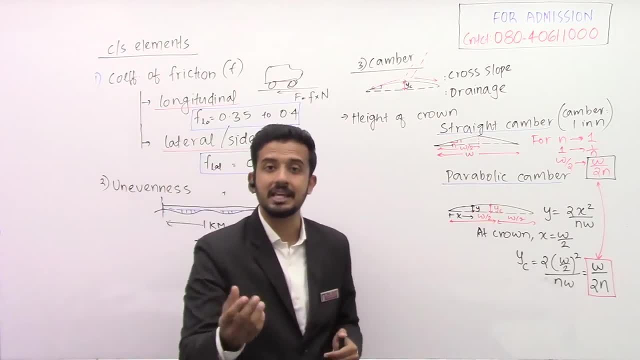 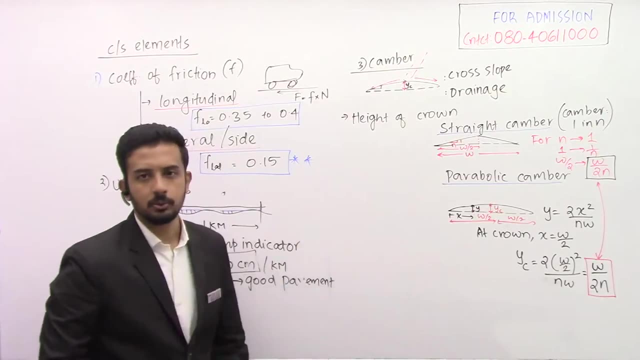 Right, There will be some separations. Practically we call it as median and all. We'll see that, Okay. So in case, if they are not giving you the value of W, then we have to take those values which are given by. 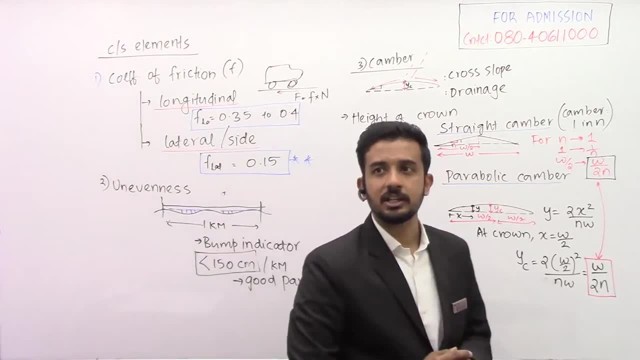 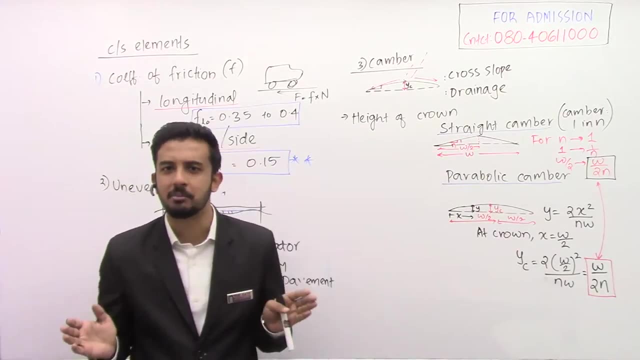 IRC. Okay. So Debashish is asking whether we have to refer IRC for examination purpose. Yes, actually you have to refer, but it is not possible to refer all the parameters, right? That's why we are giving the class Okay. 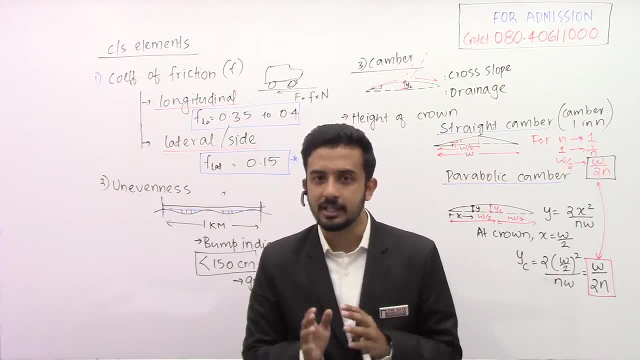 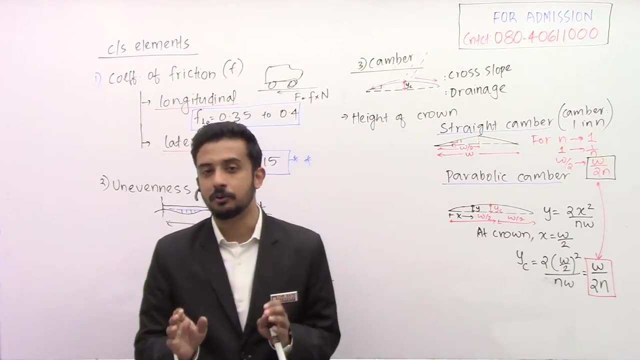 All the important parameters that is required for the examination, everything from minute portion to the toughest portion we'll be discussing here. What are the values we have to remember? Yes, I'm going to give you those IRC values for W that you have to remember. 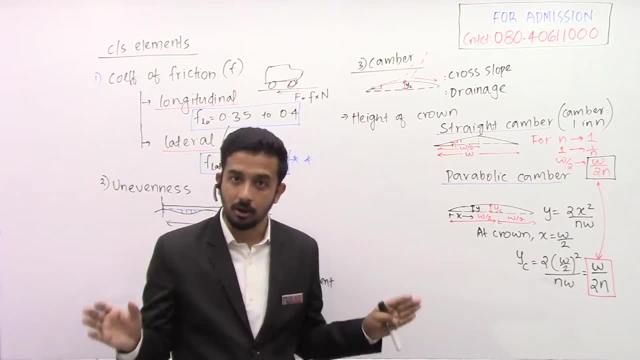 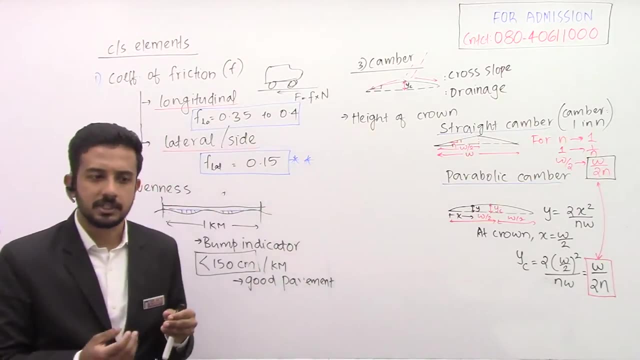 Okay, So all the important parameters. IRC is actually giving lot of specifications, All those things we don't require. So it is not possible to read the IS code for other subjects and IRC specifications. It is not possible to read all those things right, Because we have to. 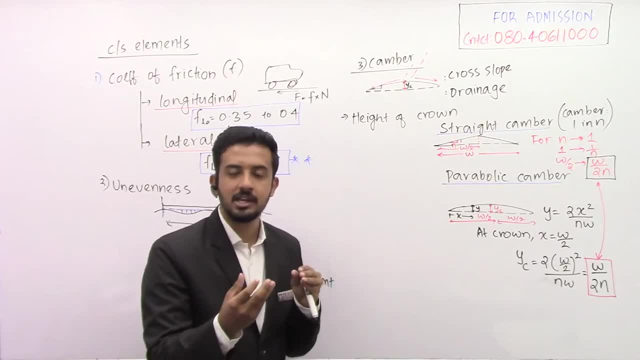 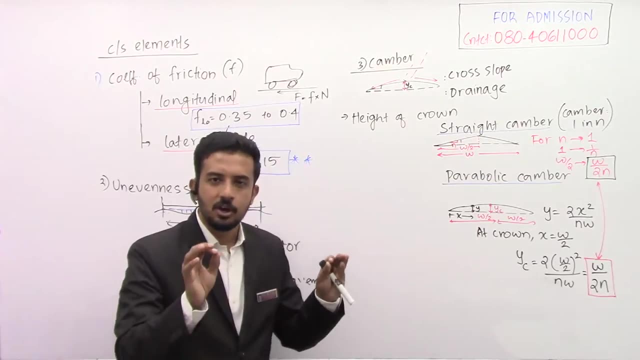 filter. We have to understand what all things we have to study and what all things we shouldn't study. No need to study, That's it Right. So don't go behind all the concepts. What is required for GATE examination? crisp and clear. 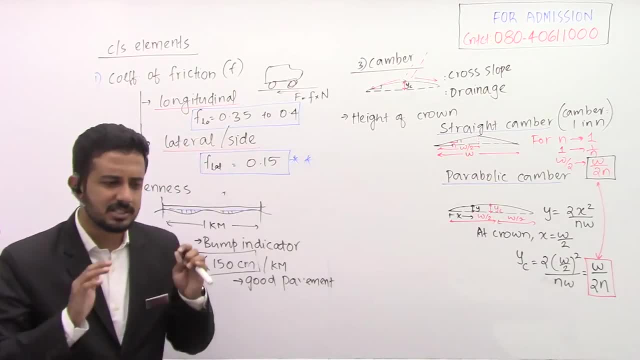 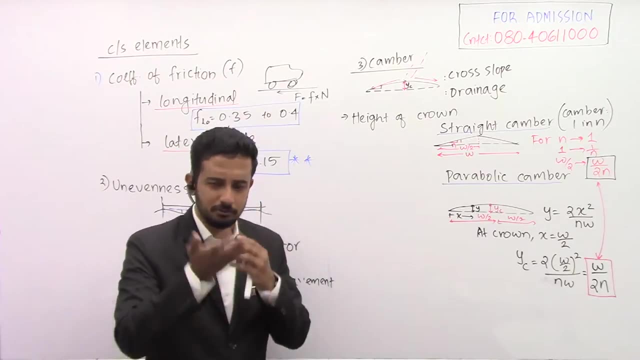 that we are going to discuss. Okay, That only will help you. Otherwise, if you are studying all the things, you are going behind all the concepts. finally, you will not be able to remember all those things. Okay, You have to recollect everything. 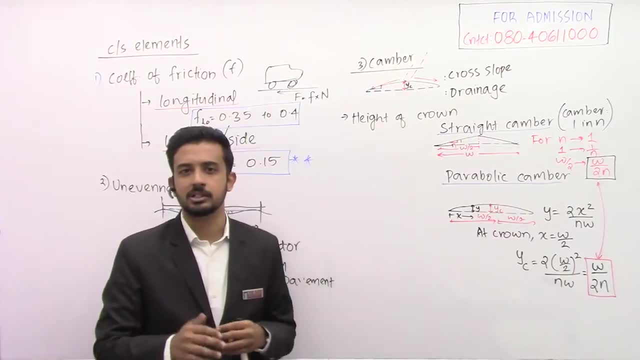 during the examination hall. right, You are going to study lot of equations, lot of formula from all the chapters, So better study crisp and clear thing. That's why I recommend you to attend the classes regularly and study what, all things, is actually required. Okay. 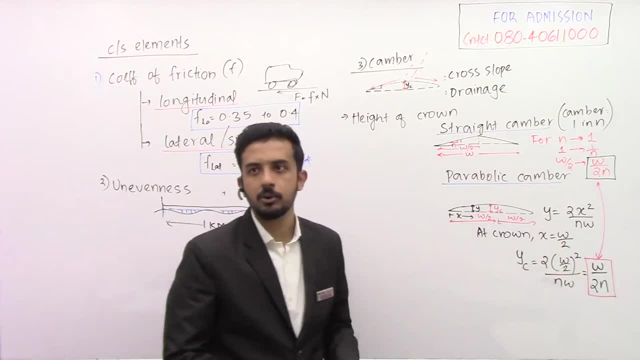 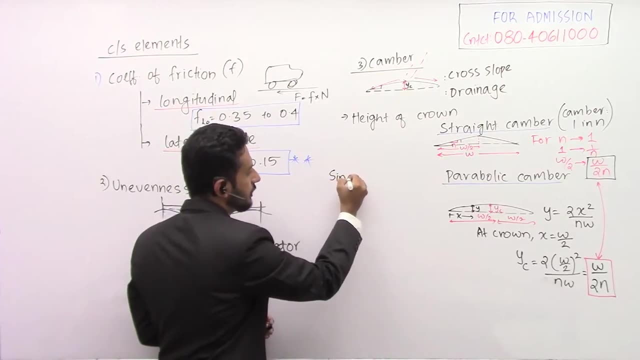 So in case, if they are not giving the value of W- the width of the road, IRC is giving some value and as per IRC for a single lane road, you can write here for a single lane road, the width of the road. 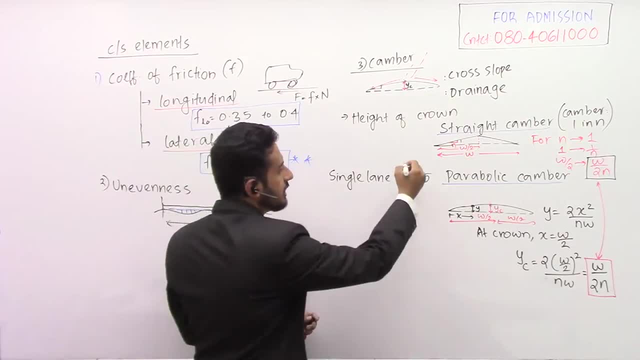 should be 3.75 meters. Okay, So this is in meter. This is in meter. This is what. This is the width of road or width of carriageway. Nothing but that W value In case if they are not giving. 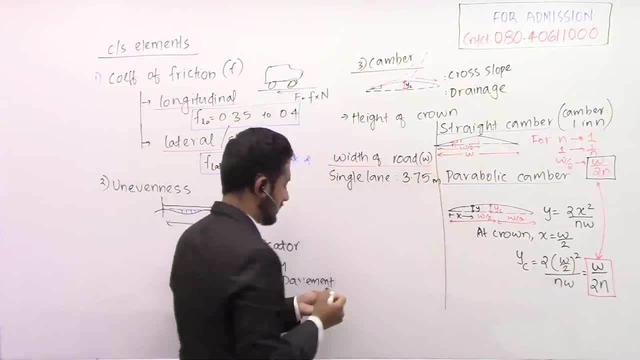 in the examination. Yeah, Very good. So single lane road: 3.75 meter For a two lane road. actually for a two lane road there are two cases. Just remember that thing For a two lane road, if a curb is. 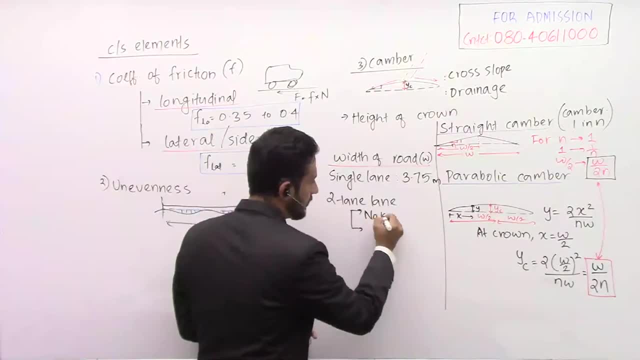 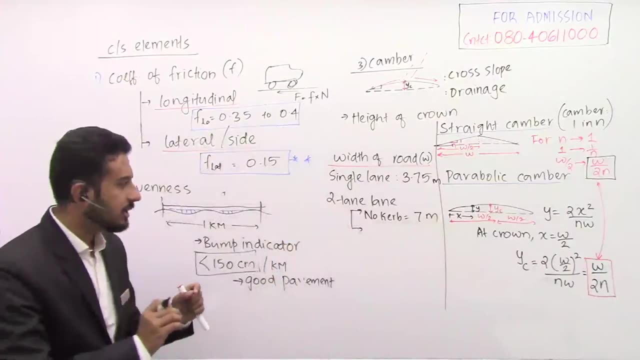 there. Okay, Suppose there is no curb, So let it be no curb, then it is 7 meter. Yeah, Someone is replying: Very good, Uptal, 7 meter. But there is a twist. There may be some raised curb, is there? 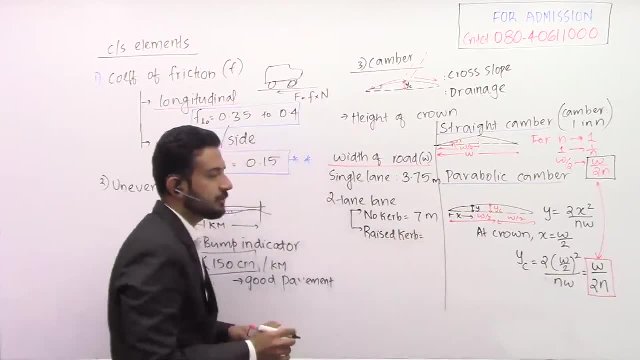 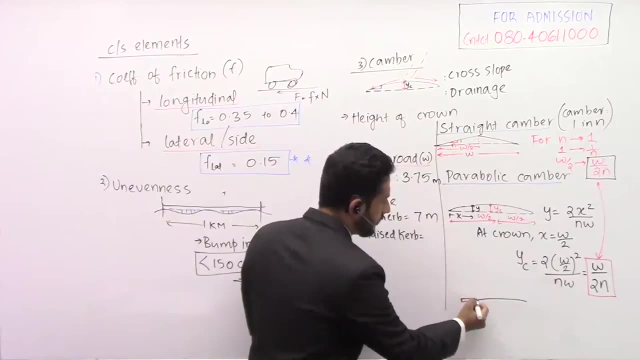 What you mean by this curb? Curb is nothing, but yeah See, suppose you are having the road here. Here you are having some footpath. Okay, This is your footpath, This is your road. Here also you are having your footpath. So 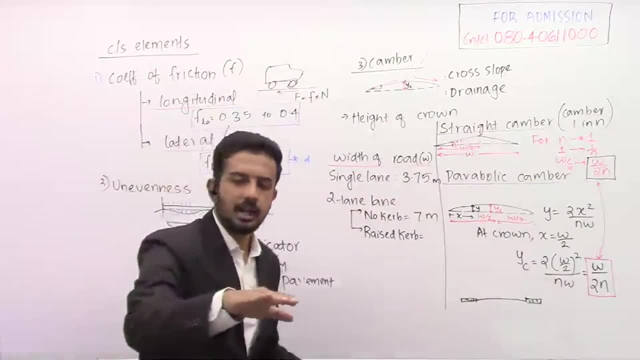 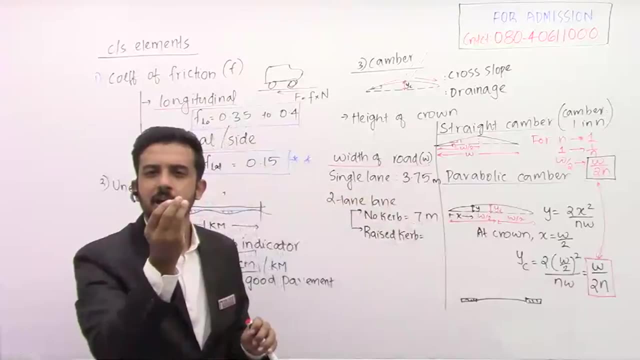 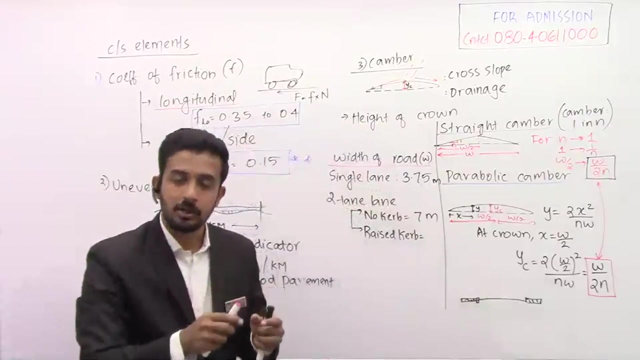 there is a separation in the elevation. Your road is here and then your footpath. So just to differentiate between the road and the footpath, we are giving some what I should tell some element here between the road or the carriageway and the footpath. 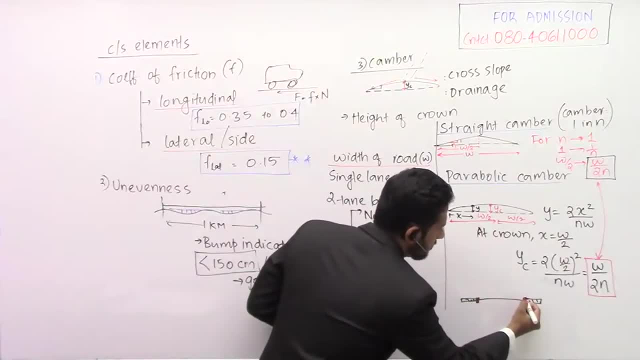 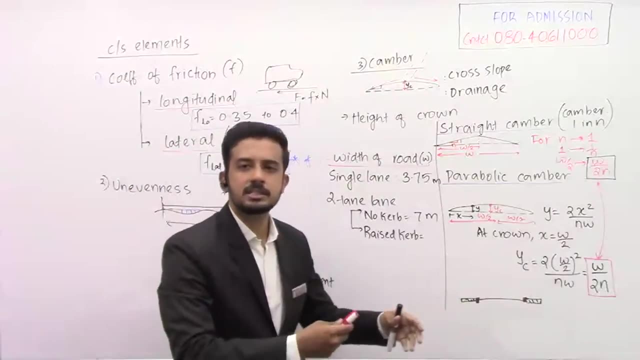 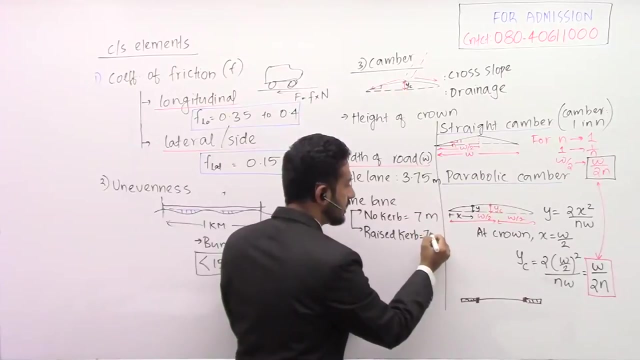 So this portion, we are going to give some element which we are calling it as curb. Okay, Curb, So suppose a curb is there, then we have to give some 0.5 meter extra. Yeah, Very good. So if raised curb is there, then 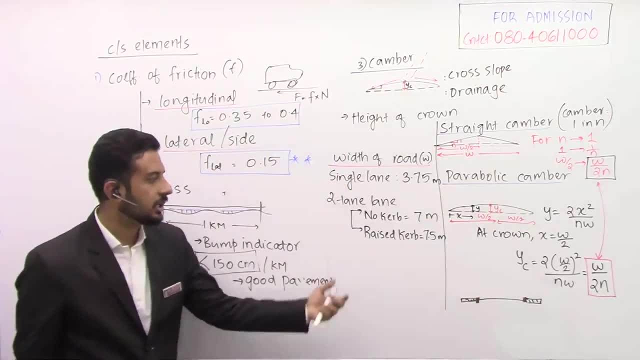 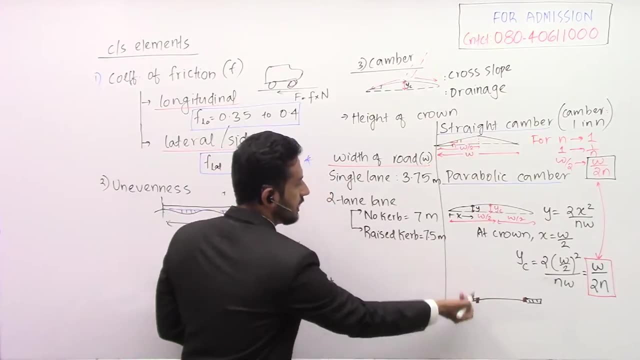 7.5 meter. Otherwise, if nothing is mentioned, it is 7 meter By default. it is 7 meter. If they are giving there is a raised curb in some element we are using. If they are giving that there is a curb. 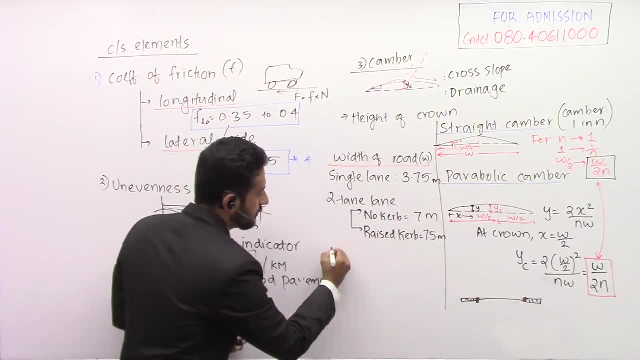 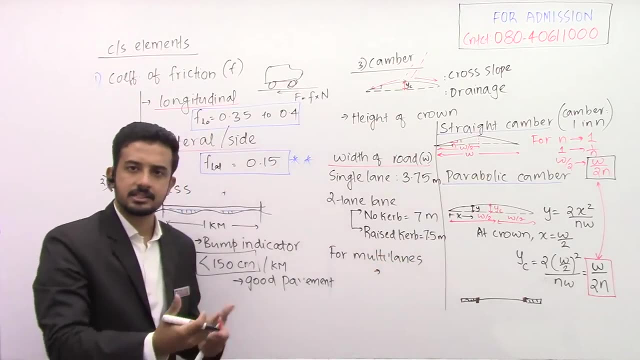 then 7.5 meter. Okay, And for multi lanes. what you mean by multi lanes? If it is a 3 lane or 4 lane, or 5 lane, 6 lane, anything, Whatever be the number of lanes, whatever be the number of lanes. 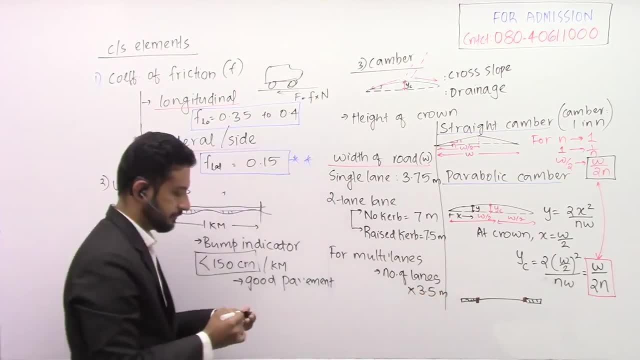 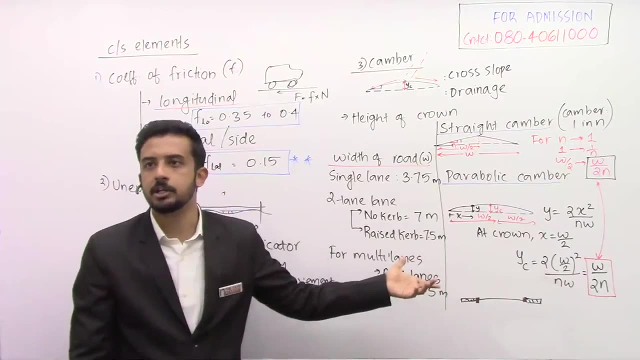 multiplied by 3.5 meter. Okay, See, the default condition for lane is what? 7 meter? Nothing but 2 into 3.5.. 7 meter, Okay, Yeah, Very good, So n into 3.5. we are taking. 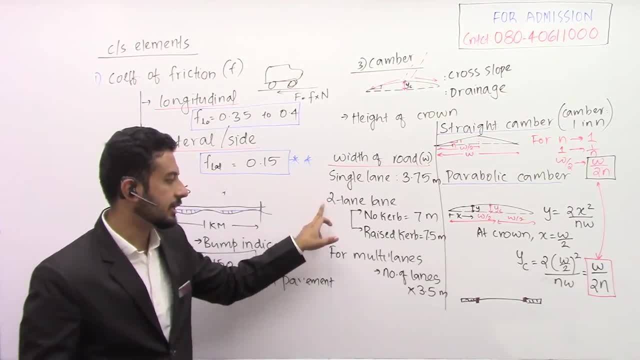 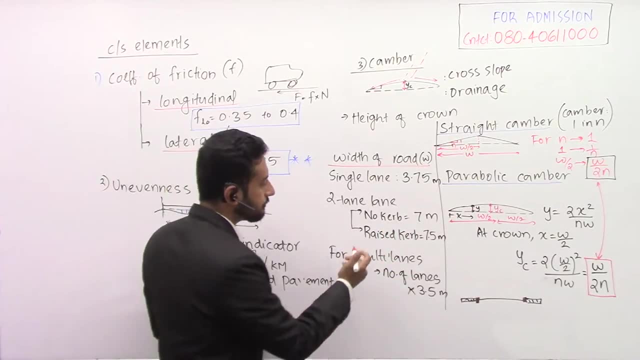 in general, but only exceptional case is single lane. It is not 3.5.. We are giving something extra 3.75.. And for 2 lane, if there is a raised curb it will be 7.5 meter. 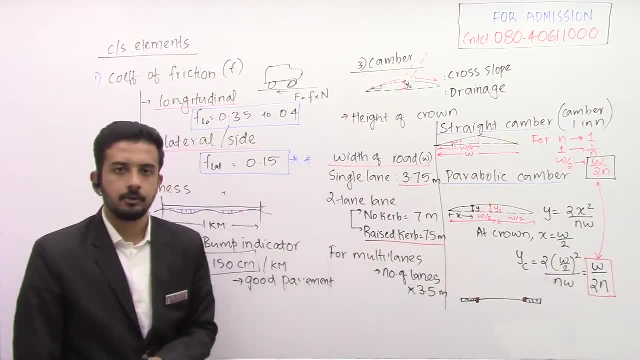 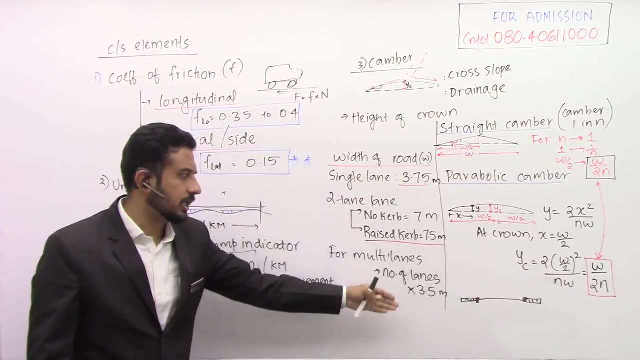 So remember those things. Other things are: n into 3.5 meter. Okay, See, this is a previous gate question. for one mark, 3.75 meter, So they can ask you anything. And also these values we will be using in. 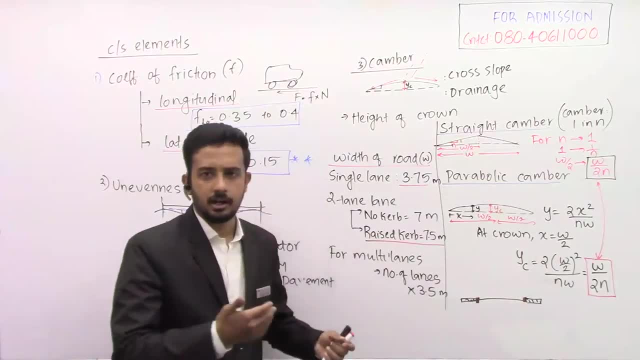 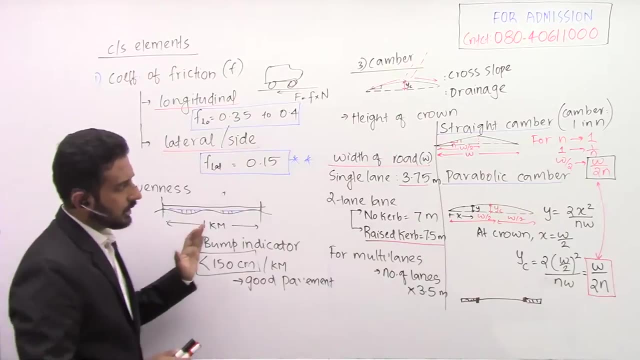 our other numerical concepts, also in horizontal curve and all in the coming sessions we will be studying There also. we will be using those concepts. Okay, So that's it. If they are not giving anything, by default it is curve 7 meter, Otherwise they have. 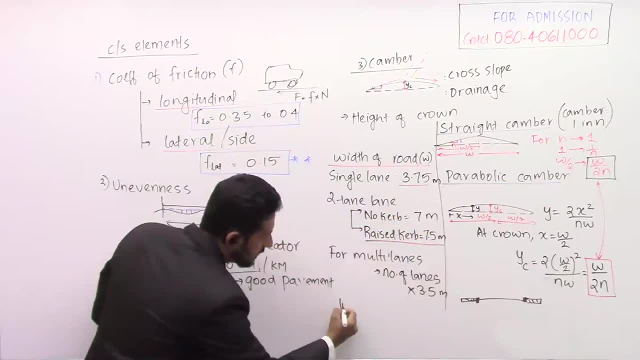 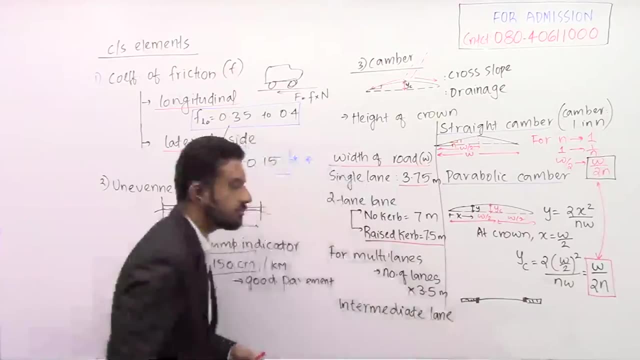 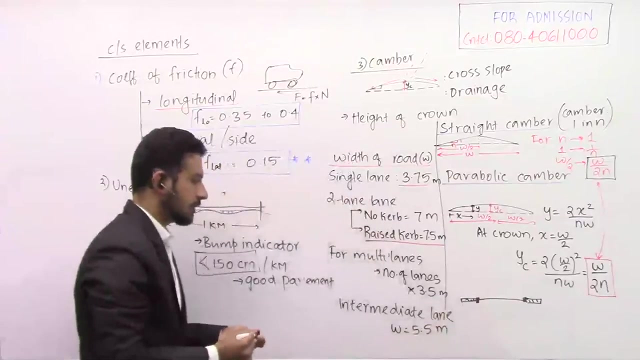 to give it. See one more exceptional case: is there The term called intermediate lane. There is a term called intermediate lane, Whereas the width is nothing but 5.5 meter. Okay, Because of some site restrictions, we may not be able to give. 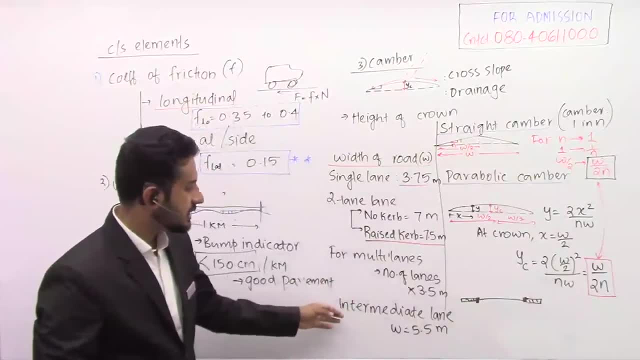 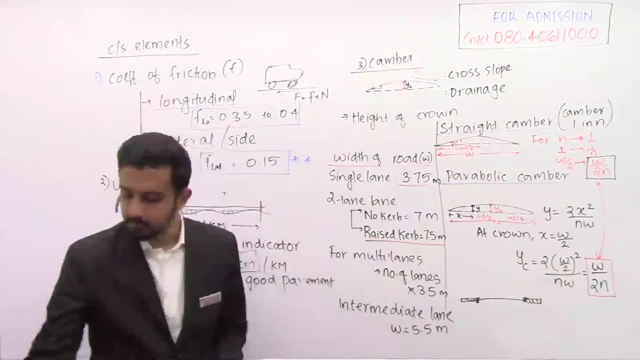 for a 2 lane range, the exact 7 meter. So in such cases we are giving only 5.5 meter. At least 5.5 meter we should give, So just remember that term- also Intermediate lane, So in case, if they are, 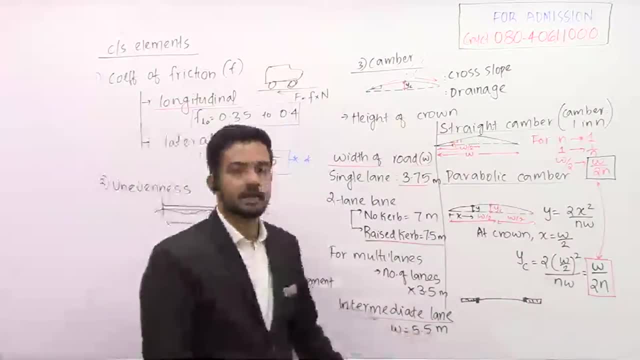 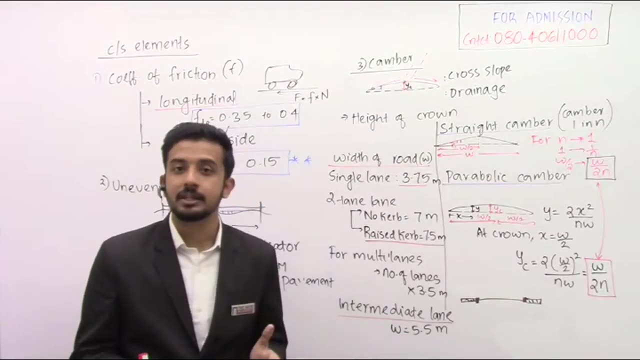 asking what should be the minimum width of intermediate lane? it should be 5.5 meter. Is camber is provided in CC payment? Yes, of course, In all the payments we are going to give camber, But the thing is for. 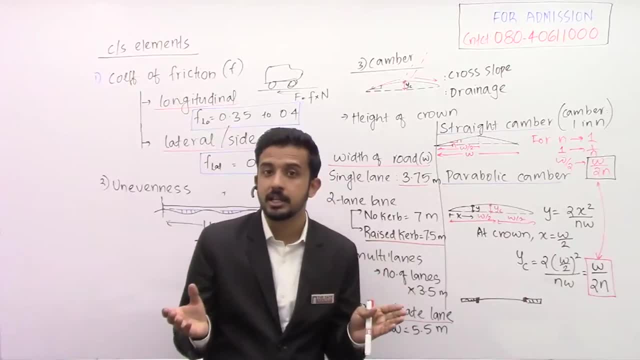 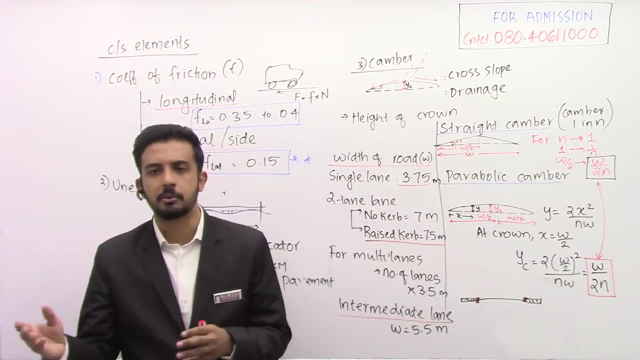 cement concrete payment. cement concrete payment means it is superior road, Right, Rigid pavement- I can tell Slight some minute camber we will give- compared to our other normal roads. We will see that value. So good question, We will see. 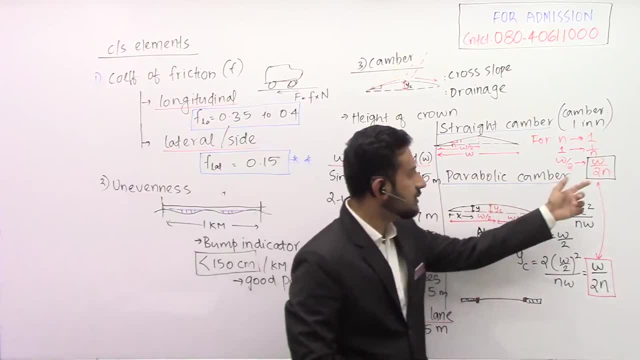 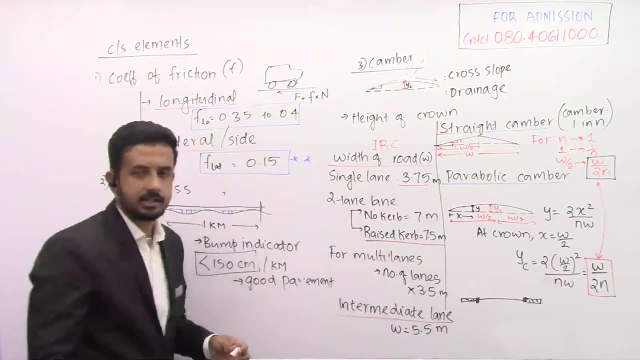 that Okay. What are the values at all? So in case, if they are not giving the value, we have to take as per. IRC See these values have given as per. these are given by IRC, Indian Road Congress. So remember those values. 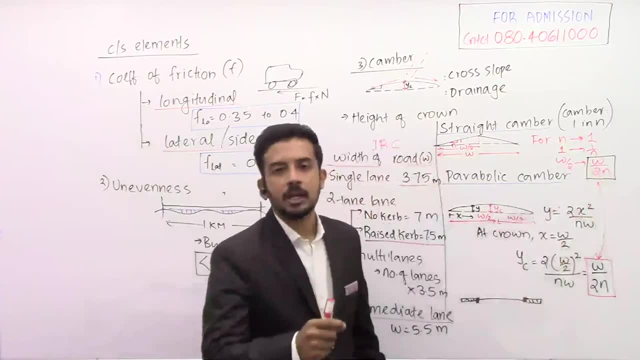 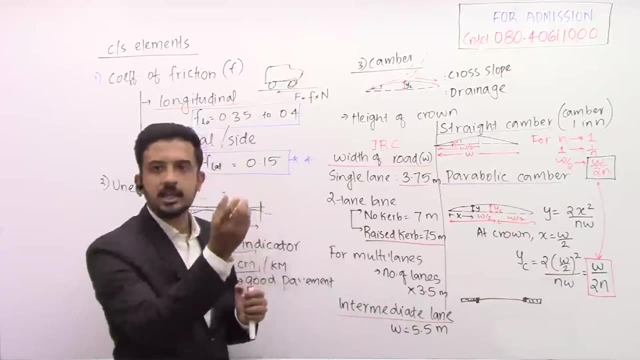 in case, if they are not giving. And what is this here? Nothing but the slope, One Indian 20,, one Indian 30,, one Indian 40, like that they will give. So that second term of one in N, the value of N. 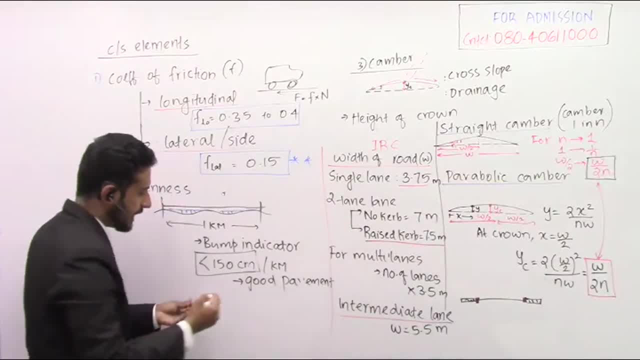 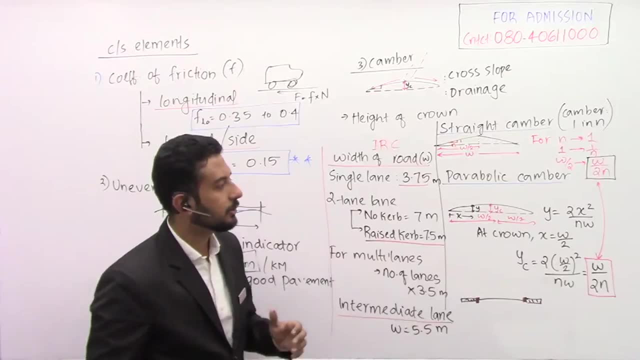 Okay, So I told you, sometimes they are not going to give you the value of W, Like that. if they are asking you a two marks question, they are not going to give you the N value also. Otherwise there is substitution only. 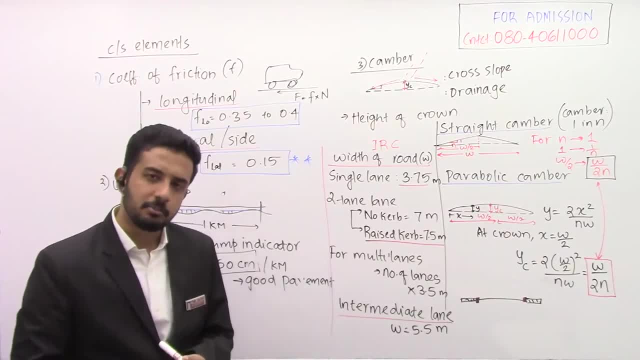 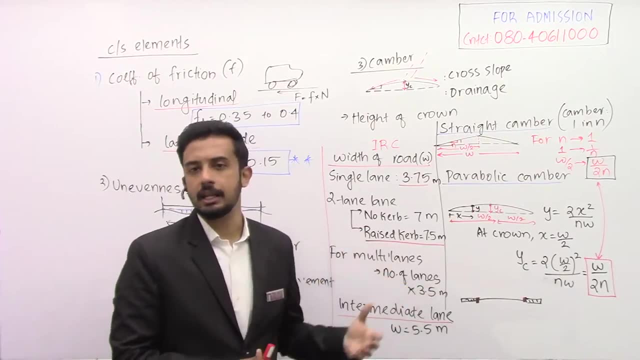 So they may not be giving the value of W and they may not be giving the value of N. Okay, Both they will not give, but they will give some other parameters, such as two lane, three lane, like that. So from that, 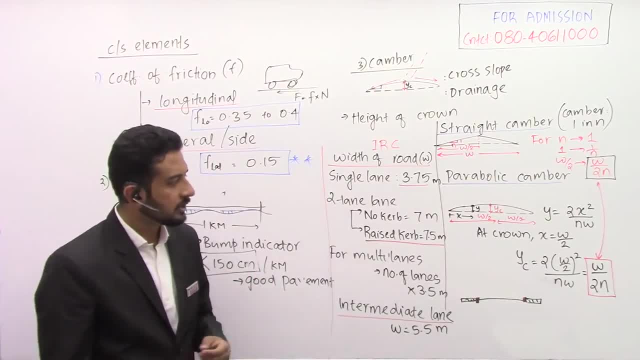 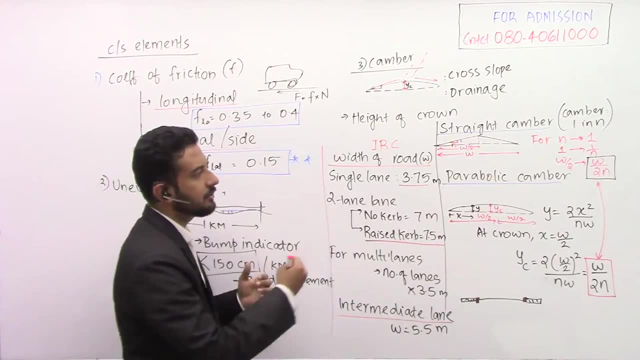 we have to select. what are the values of W and N? Okay, So I am giving you how to calculate, or how to take the value of N as per IRC, and how to calculate that height of crown value. Okay, So I am going to rub this and 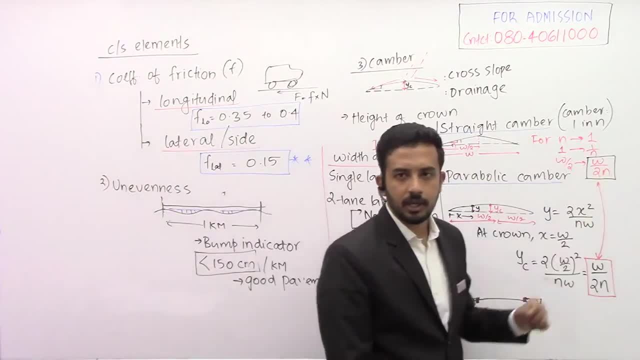 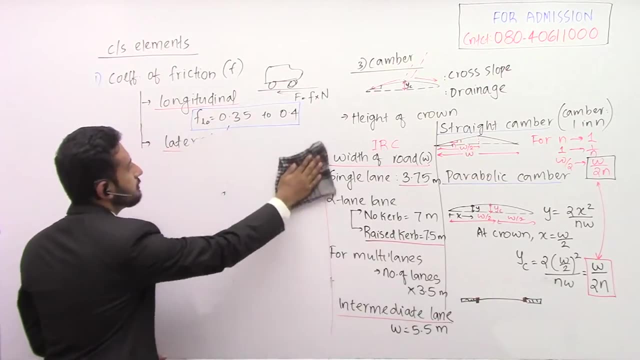 I am going to give you, in case, if they are not giving the value of N, how to select that value. Okay, So there is a recommendation of some set of recommended value as per our IRC, So we have to select the values of N from that. 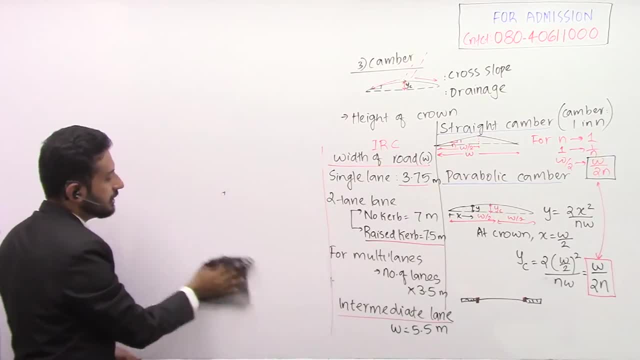 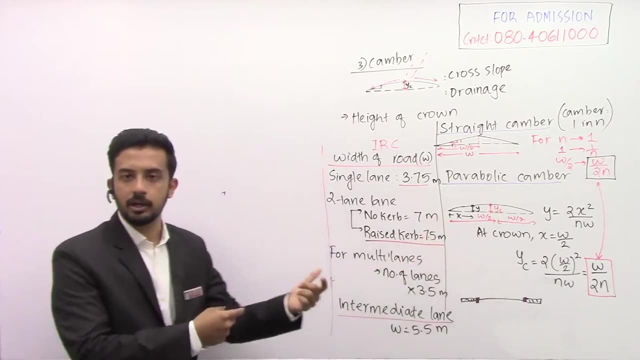 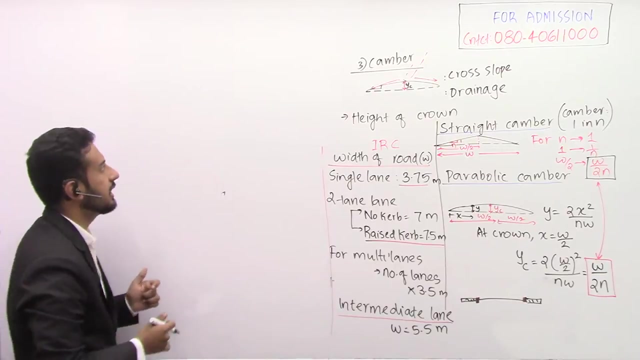 particular table. Okay, So note down that table Very, very important. They have already asked some one more question from that. and also the same parameter we may be required in that- numerical portions also. Okay, So the recommended value of camber as per IRC. 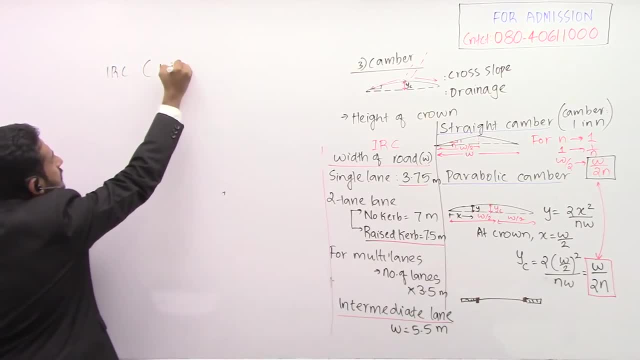 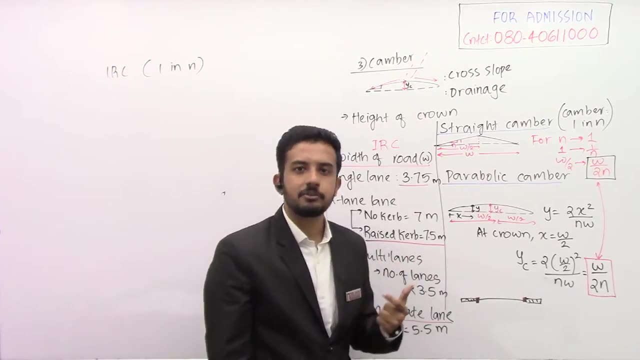 Okay, So IRC recommendation for camber. So the one in N value Depends on the type of the road and the rainfall. We have to select what is the value of camber. Okay, See why we are giving camber To drain off the rainwater. 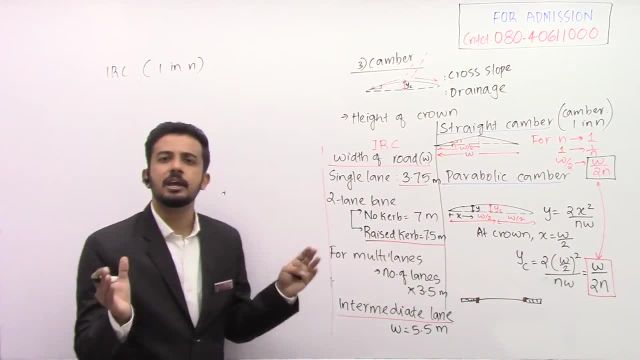 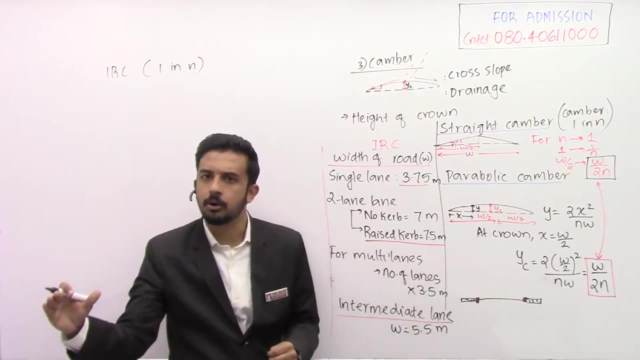 Right, So definitely, if it is having very heavy rainfall, if it is the road is going to construct in a heavily rainfall area, then we have to give some more slop. Water has to remove, water has to drain off easily. If the portion, if the area, 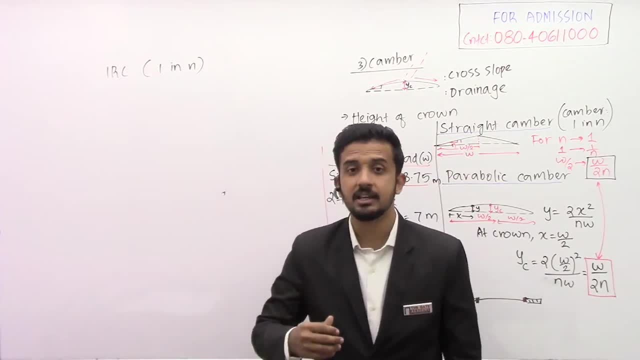 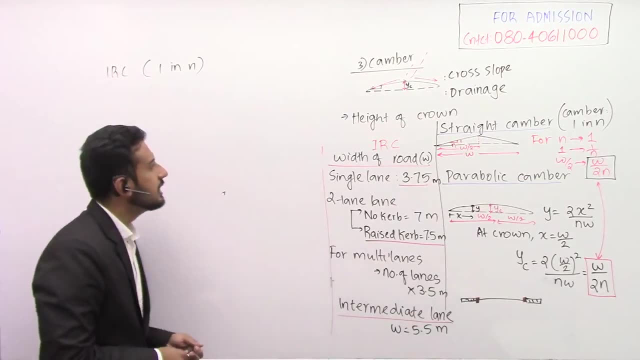 is not that much rainfall area. If it is a less rainfall area, then we don't have to give more slop Right. Some minor slop will be sufficient Right. So according to the road, I can tell it as cement, concrete road. 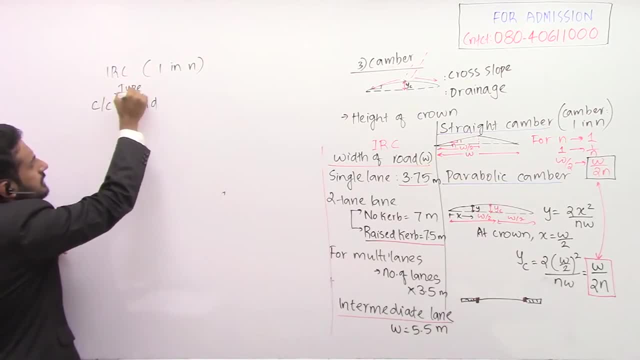 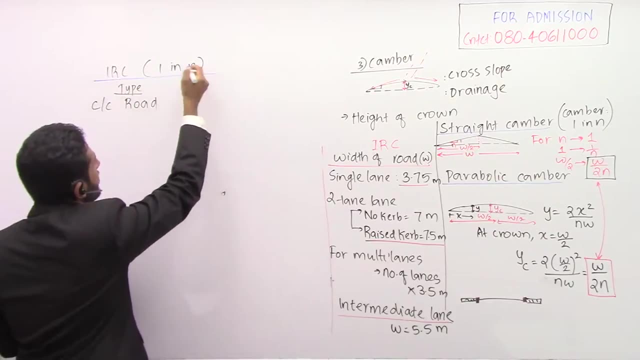 Okay, You can tell it, as this is type of road. This is the type of road and I am going to give you the camber value also. Okay, So this is, as per the camber one in N, So the type of road we will be writing in. 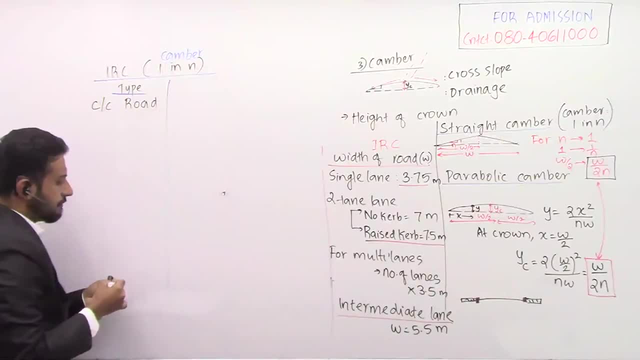 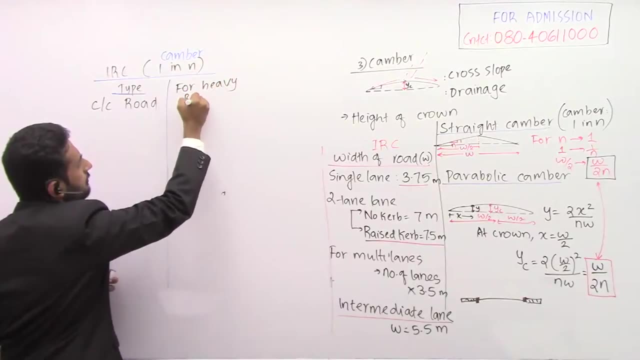 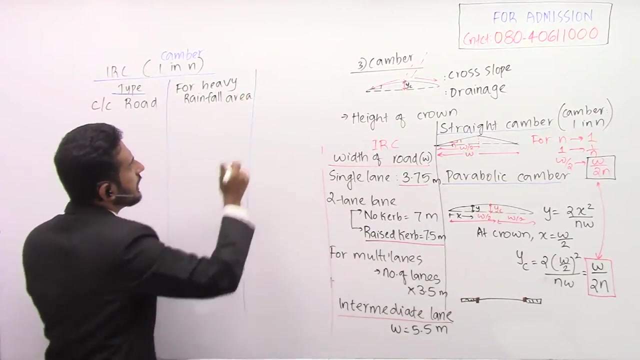 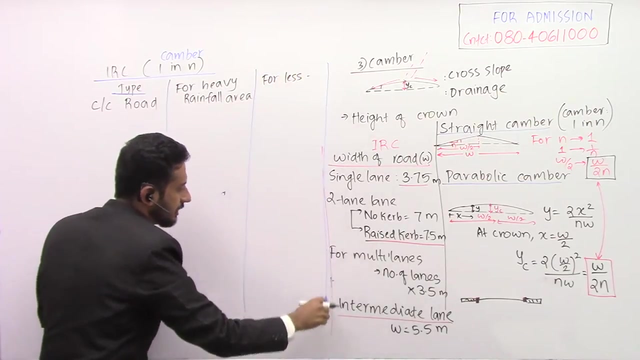 the first column, Then the camber value for heavy rainfall area, For heavy rainfall area, And the next column will be for less rainfall area, For less rainfall area. So we don't have to check what, which or how we will be determining whether 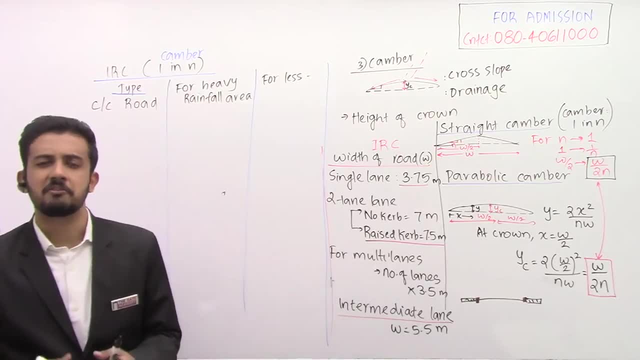 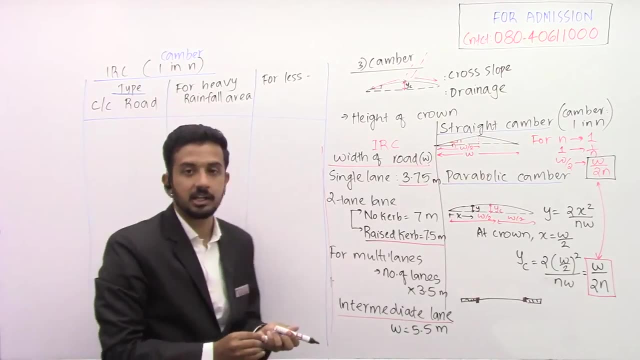 it is a less rainfall area, whether it is a high rainfall area. We don't have to think about those things. It is already tabulated which all things, which all areas are coming under high rainfall area, Which all portions are coming under less rainfall area. So they will. 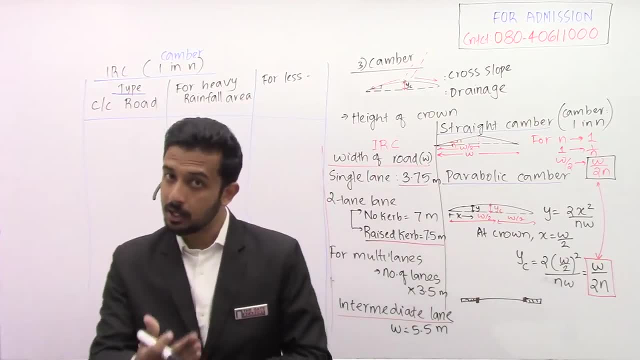 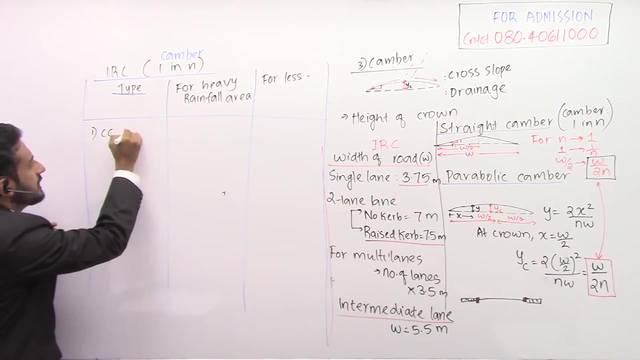 be giving in the question as it is. We will see the questions also How they are going to ask. Okay, So okay, The first one is the cement concrete road. I am just writing it as CC. What is CC? Cement? 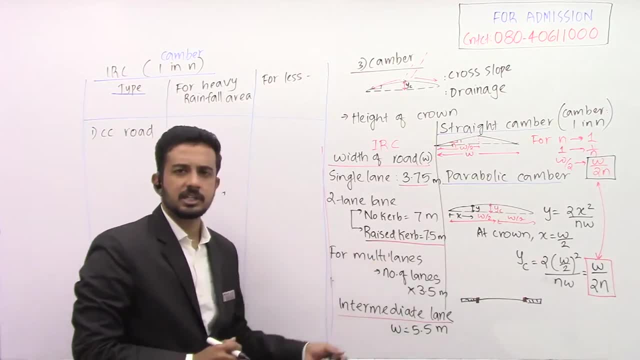 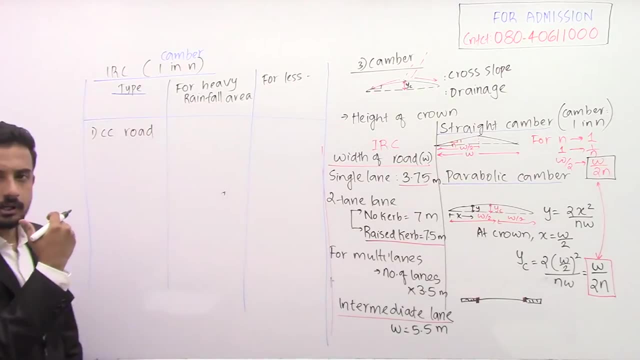 concrete. Nothing but our rigid pavement. You might have studied flexible pavement, rigid pavement and all Flexible pavement is nothing but bituminous and rigid pavement is nothing but cement concrete. Okay, So, cement concrete road is the first one, And cement concrete as well as some. 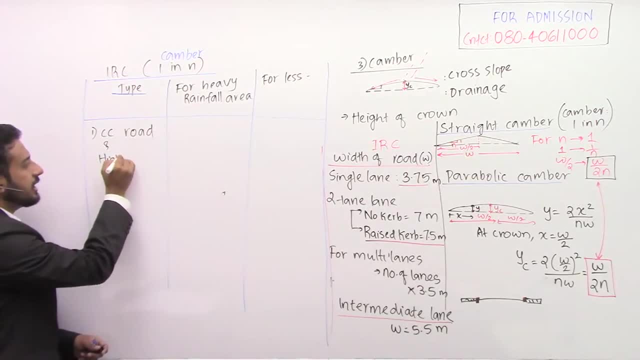 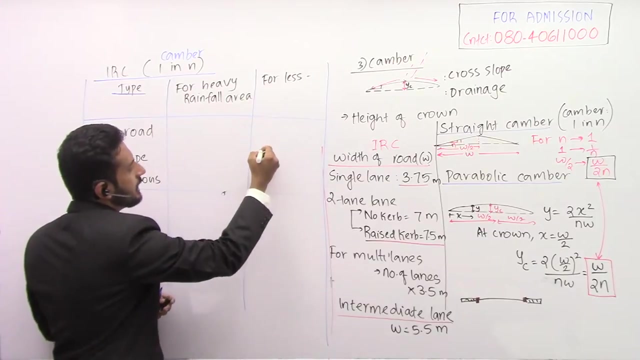 high type. Suppose some high type bituminous pavement may be there: High type bituminous Cement, concrete road or high type bituminous pavement. If it is of this category, then the one in value will be 1 in 60 and this will be 1 in 50.. 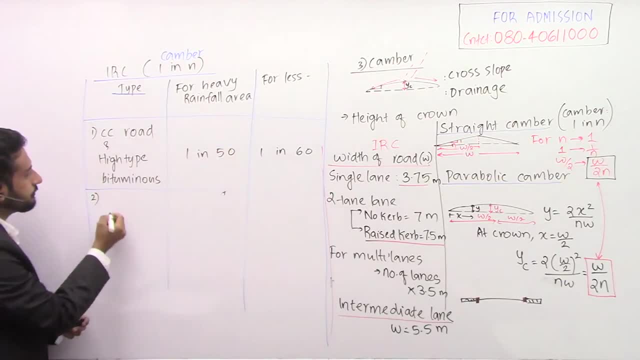 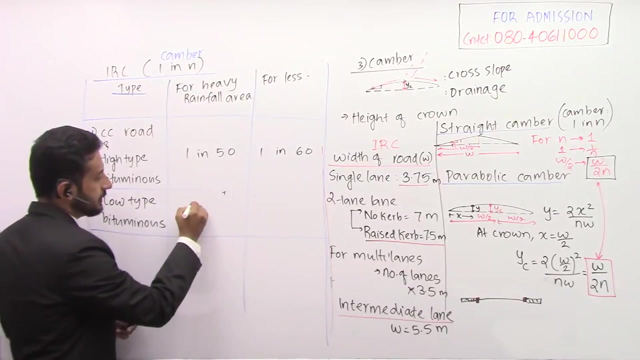 So we are writing. So, if it is a low type, bituminous pavement, no need to confuse what is this high type and low type and all They will give as it is, That much in detail we don't require actually. Okay, So this will be. 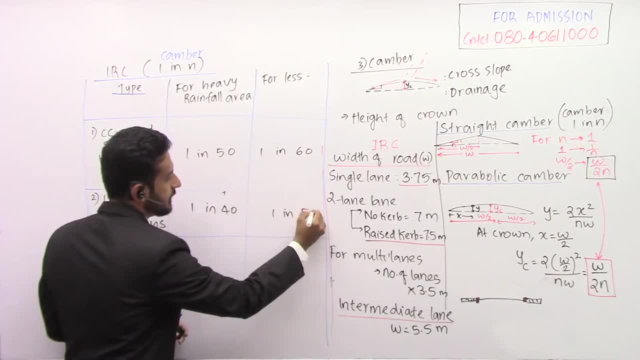 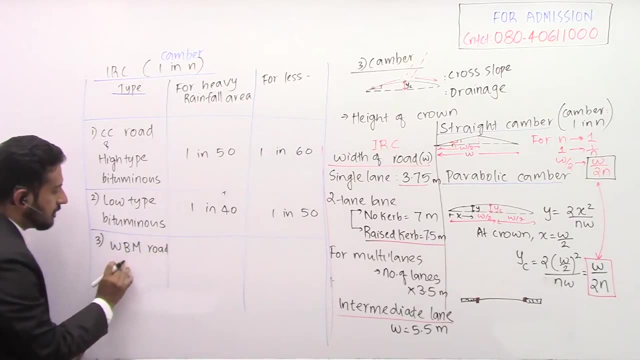 1 in 40. This will be 1 in 50. You have to by heart these values. WBM road. What you mean by WBM road, Water bound mechanism, You might have studied. You might have heard that word already, Right. 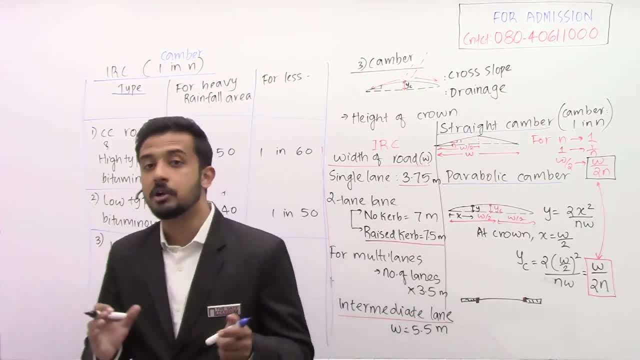 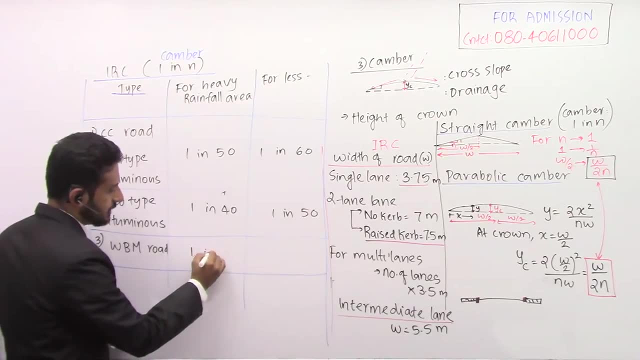 Water bound mechanism, How to construct water bound mechanism and all we don't require for our exam. Okay, So study the things crisp and clear What all things are actually needed. This is 1 in 33.. This will be 1 in. 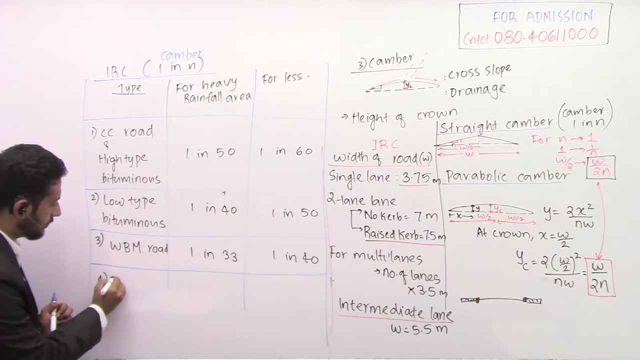 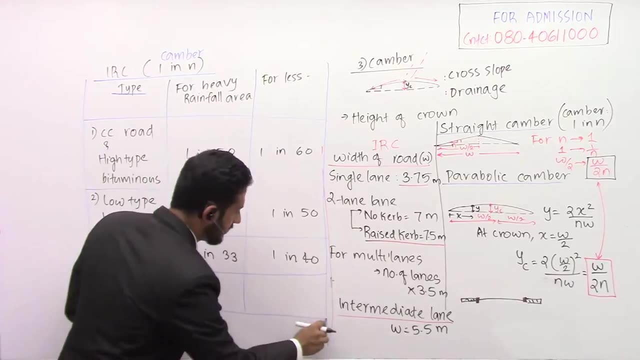 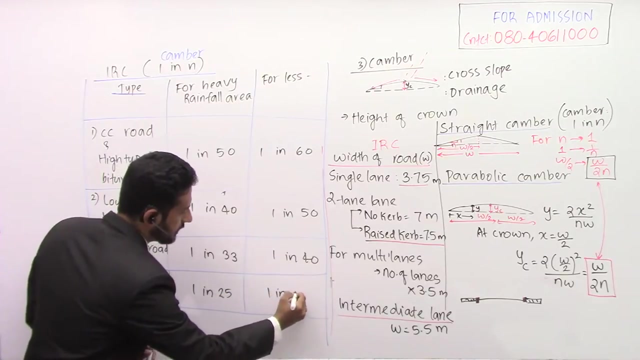 40. Then we are having earth road. We are having earth road, So if they are asking the questions, they will exactly give the same wordings. If it is earth road, this will be 1 in 25 and 1 in 33.. 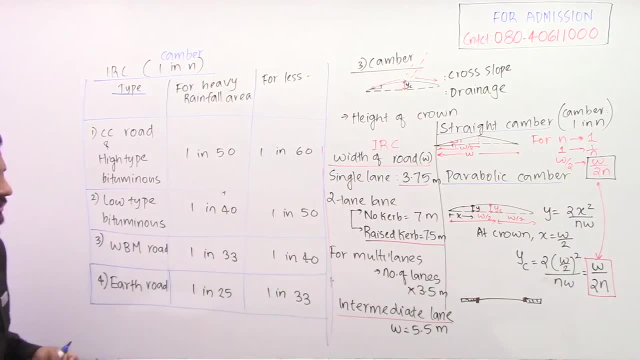 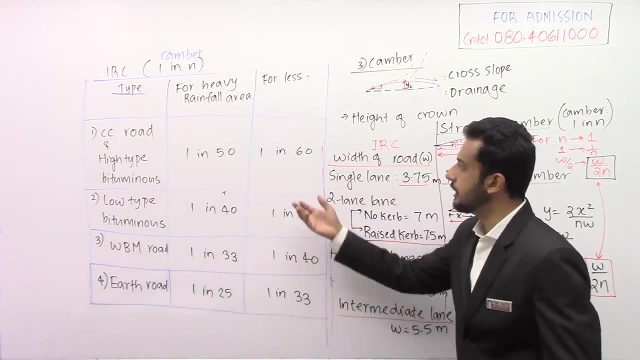 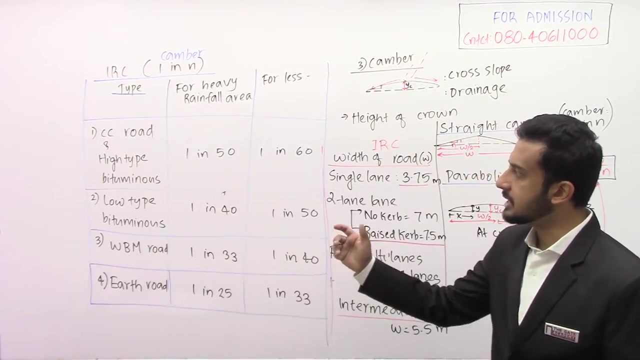 So you have to remember these values, You have to by heart these values, Because they have already asked the values directly, This value. they have already asked What will be the camber, The recommended value of camber as per IRC for a cement concrete. 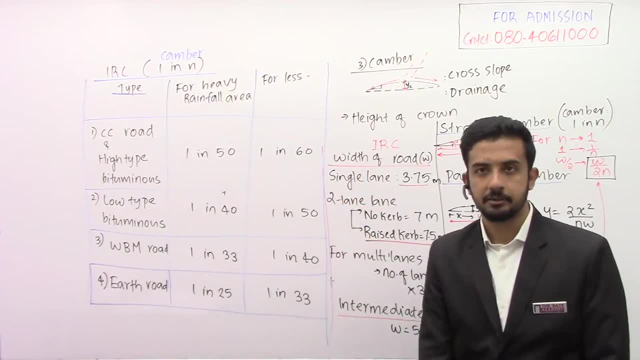 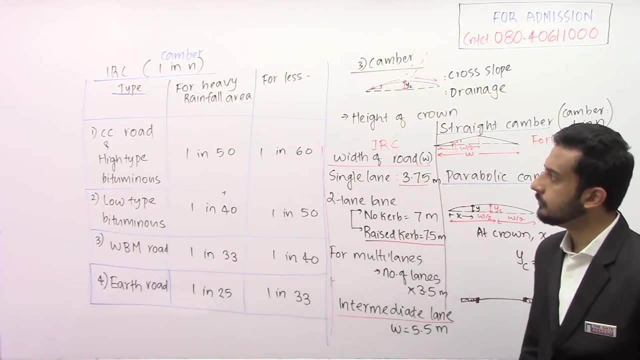 road for less rainfall area. So, like that, they have already asked the question. So anything, Any value from this table, they can ask you. Okay, So if you have completed writing, please let me know. I will give you the numericals. 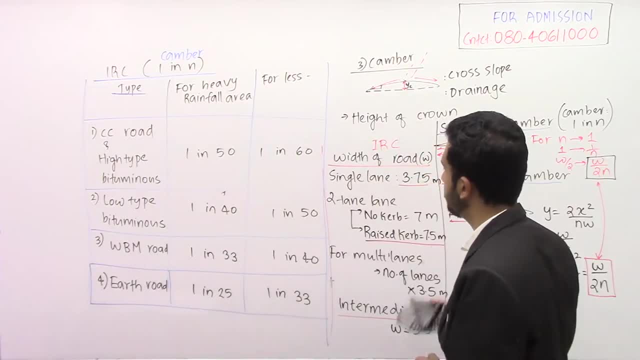 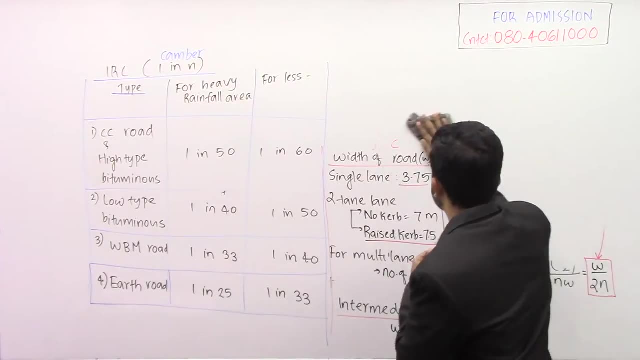 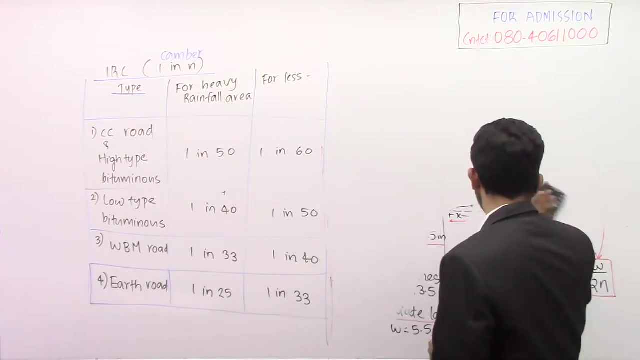 how they are going to ask. If you have completed, please let me know. Better write fast so that we can complete so many questions, We can practice so many questions, How many questions we can solve. that many we should do. Then only we will remember. 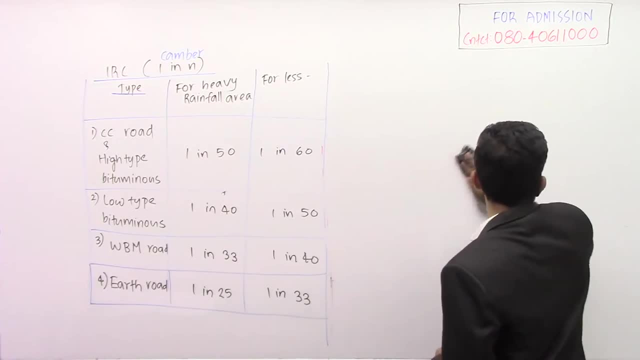 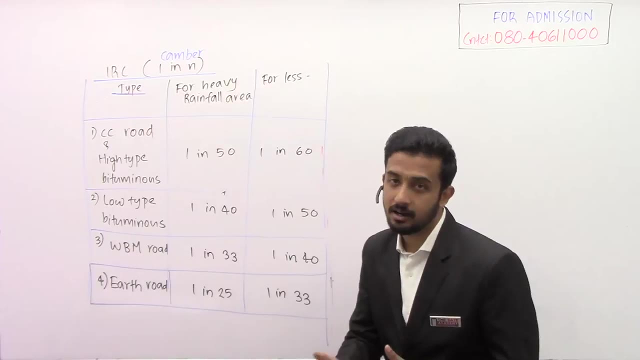 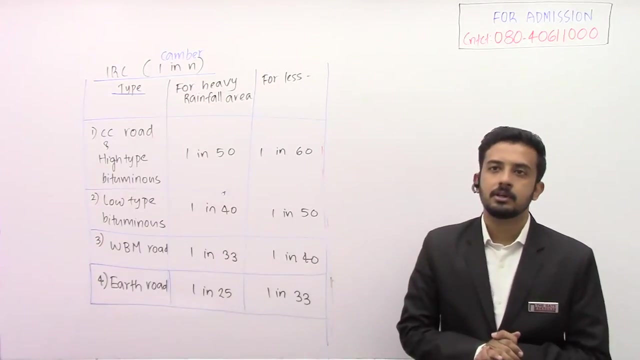 the formula and all. Only practice makes you perfect, Especially for GATE examination. See, for GATE examination, you don't have to work hard, But you have to work smartly. That's it. Whatever we are studying, crisp and clear things you should remember. 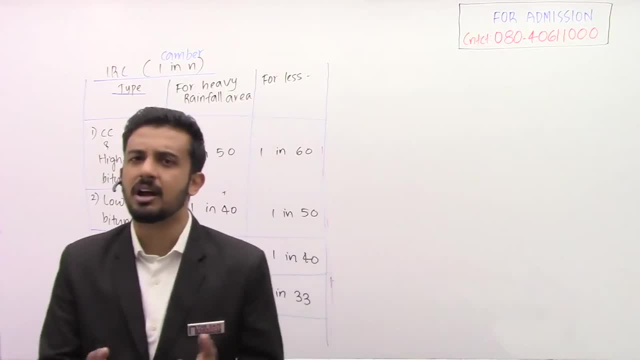 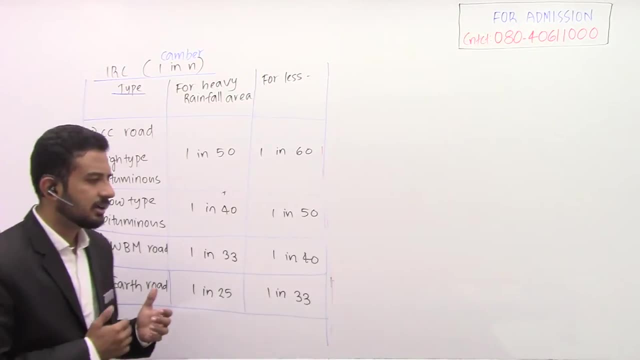 So solve so many questions and remember the formula: GATE is not for hard workers, It is for smart workers. So remember the things. No need to go to deep and understand. what are these types of road, how it is constructed- Those things we don't. 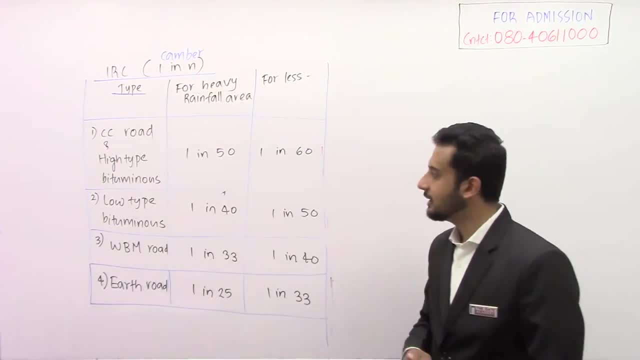 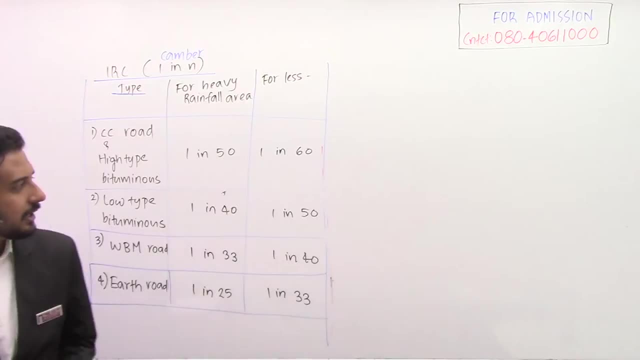 require. If you need that, yes, well and good, You can go through that, but after the GATE exam? Okay, Don't waste your time. Fine, I told you this question has already asked. I will give you that theory concept also. 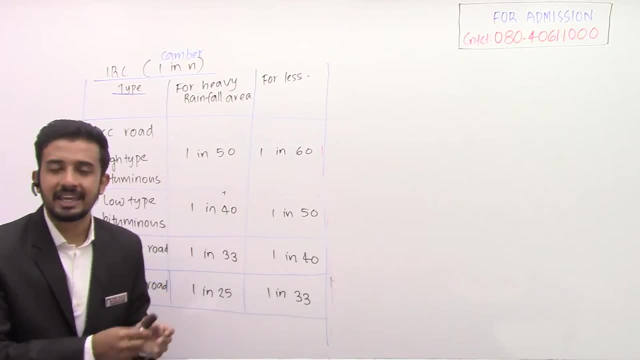 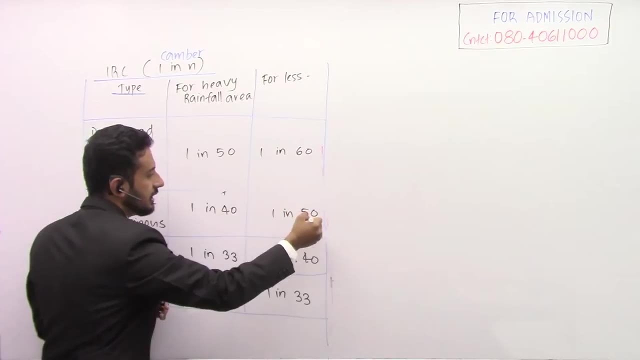 Okay, See directly. I told you it is 1 in N Means. what is that N? What is that N? N means? it can be 60,, it can be 50, it can be 40,, it can be 33,, it can be 25 and all. 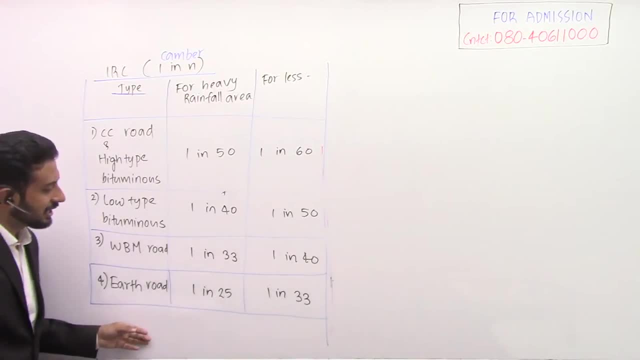 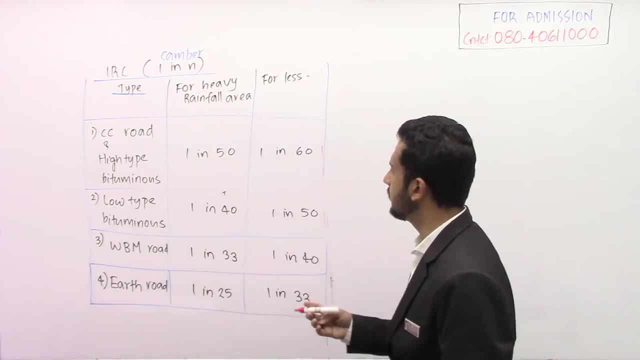 Is there any trick to remember it? Yeah, Okay, See, you can make your own tricks to remember. That's a good thing to make some tricks to remember. Okay, I will tell you something. See, just remember this thing: only 60.. 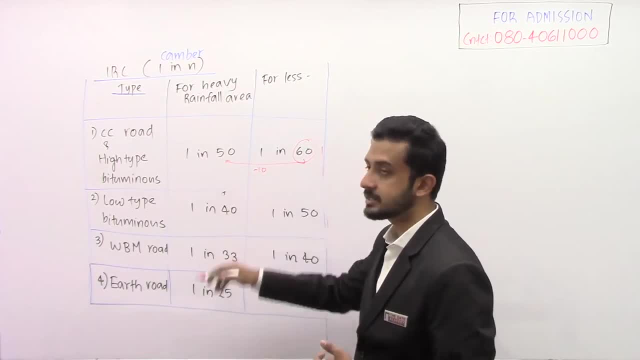 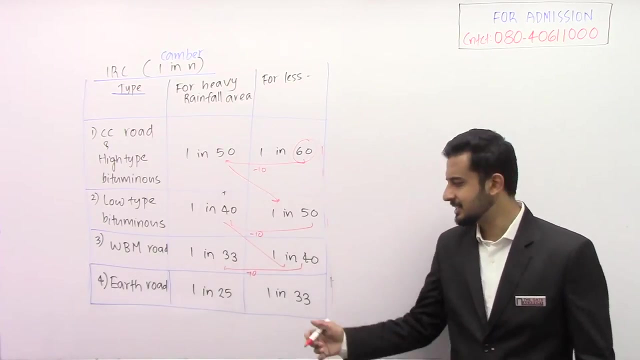 So it will be minus minus 10.. Then take directly here. Again, it is minus 10.. Take directly here. But here, if you are minusing 10, then you are going to get 30.. Right, This is my trick. You can go, you can. 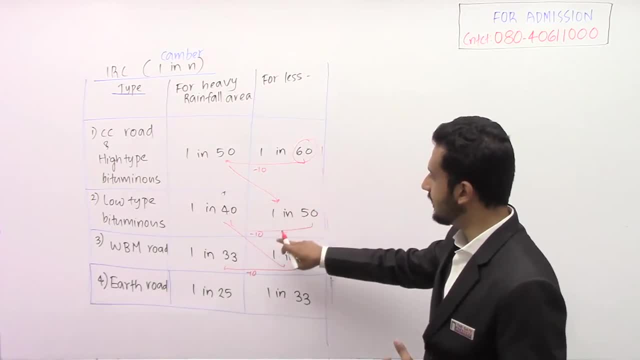 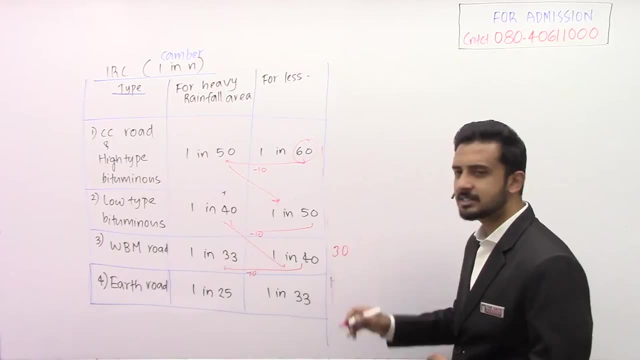 accept that trick or you can make your own tricks, No problem, See till here. it is okay: Minus 10,, minus 10.. So if it is minus 10, you should get some 30. Right? So since it is 30, 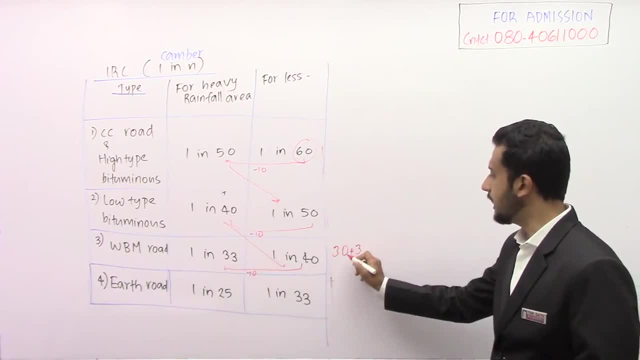 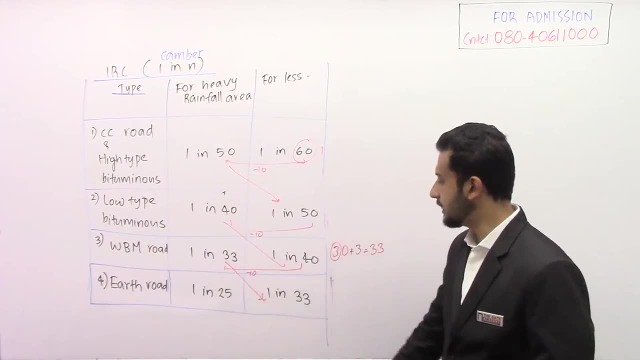 I know there is some change here, Right? So I am just going to add the first letter, 3.. So it will be 33.. Something like that you remember So directly. it is coming here: 1 in 33.. So if it is 33, our trick. 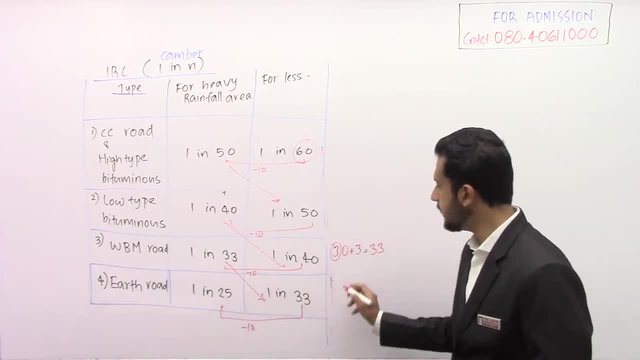 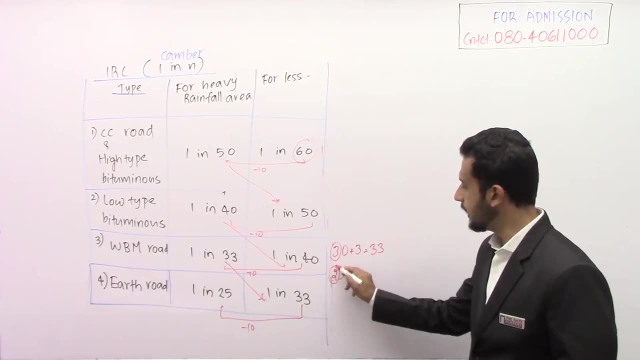 is what Minus 10.. If it is 33, it should be, it should be 23.. Right, So it should be 23.. So, since it is 23,, I am adding the first one, So it will become 25.. 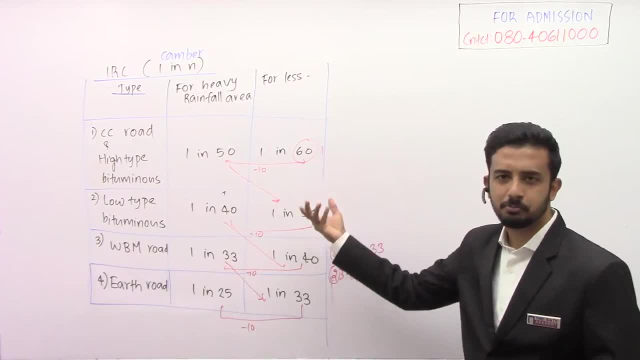 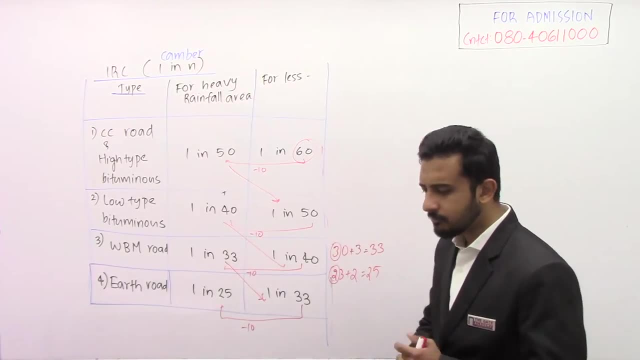 So that is 25.. So at least you can remember like that, or in terms of percentage also you can remember. Yeah, very good, In terms of percentage also you can remember. But the thing is, it will be better if you are studying in this format, Because that 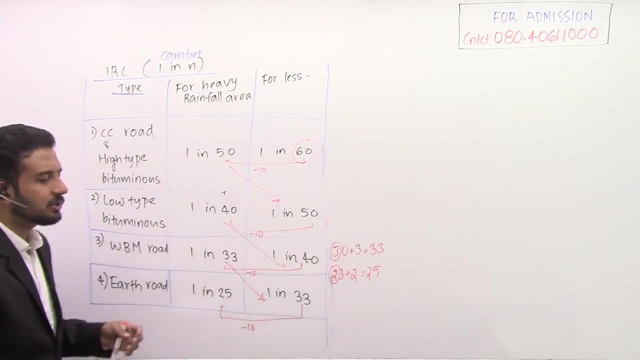 w by 2n. if you are studying in percentage again, you have to convert into this form. Okay, So 60, 50,, 50,, 40,, 40,, 33,, 33,, 25.. Fine, So this thing will be always. 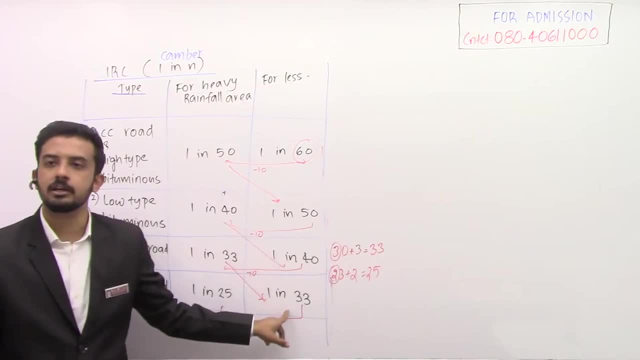 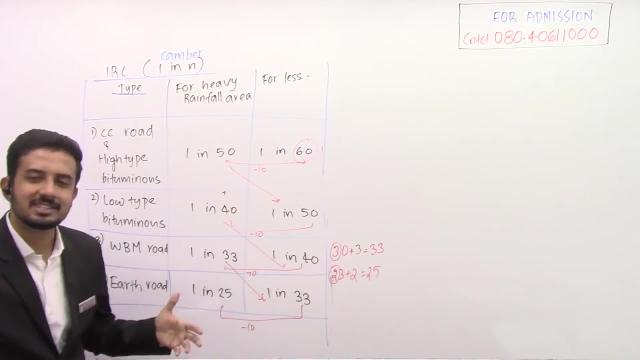 whatever here, it will be in the next column, Whatever will be here next column, Whatever will be here in the next column. Okay, Like this we can remember. definitely, Definitely. you can remember. Make some tricks and remember And see, not only that, the 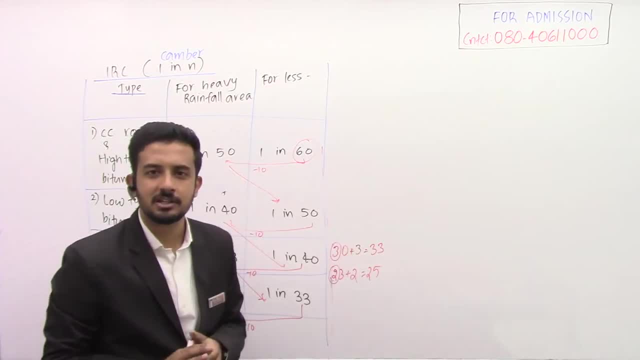 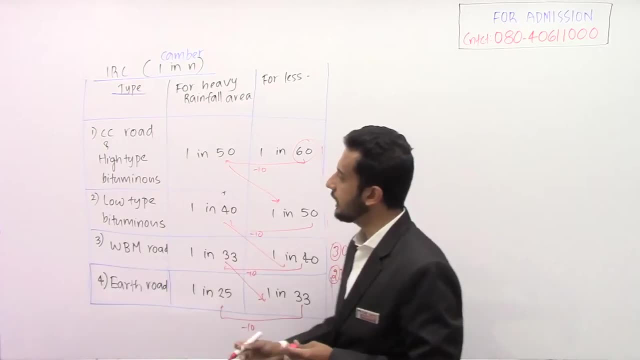 parameters. also, you should remember First who will be coming first, Who is having more mark, Right? So exactly, first column will be heavy rainfall, Second column will be less rainfall. And also, see, this is nothing, but we are arranging in the order of quality of the payment. 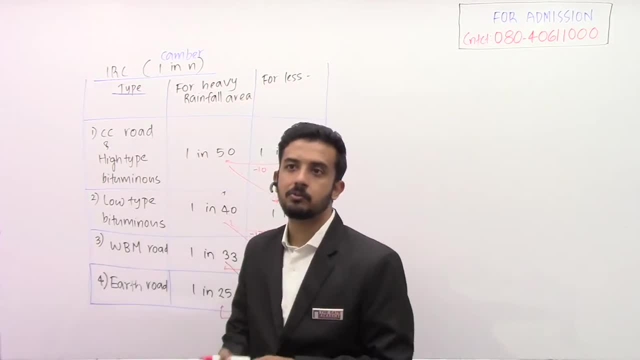 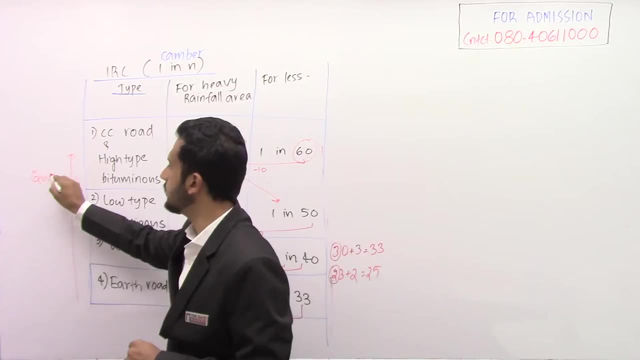 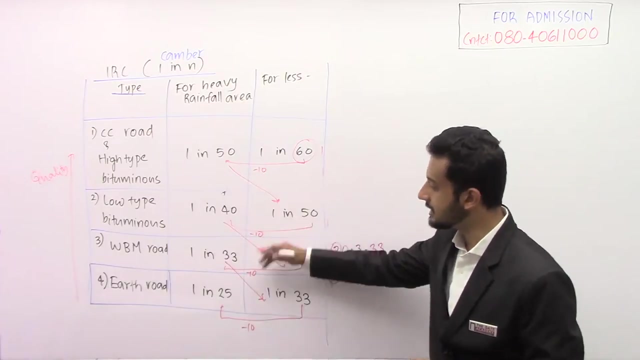 CC payment means cement, concrete payment will be having highest quality. So the quality- if you are checking here, it is having highest quality Quality is increasing, Right? So whenever the quality is decreasing, camber is also decreasing. Okay Sorry, camber is increasing. 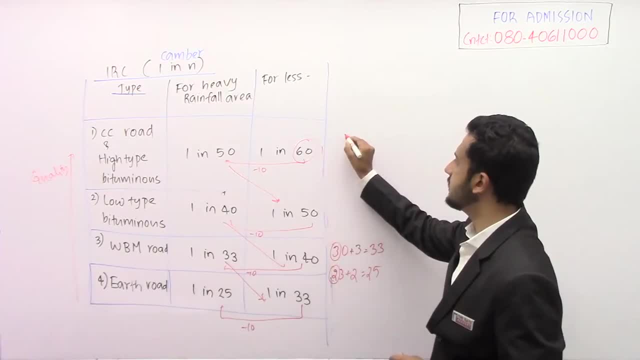 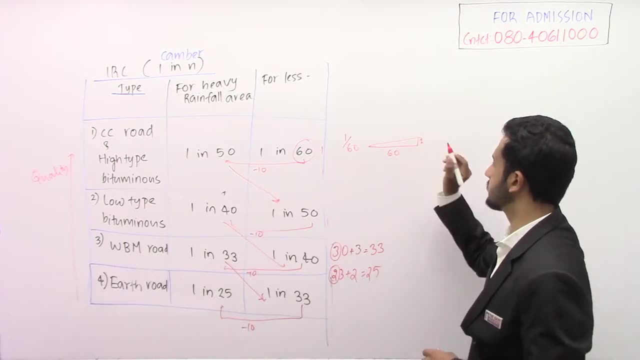 It is 1 in 25 now. So what do you mean by 1 in 60? Nothing but 1 by 60. Whenever you are going 60 horizontal, you are having 1 vertical. It is something like this. What do you mean by 1 in 33? 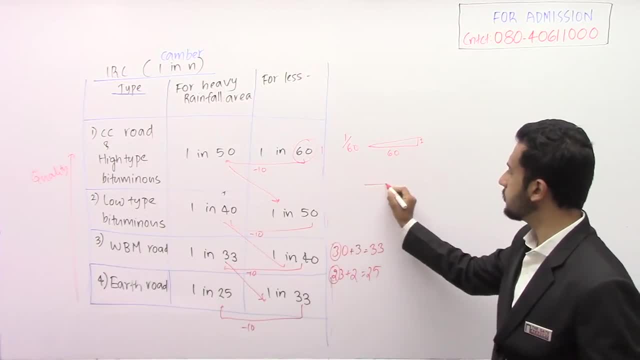 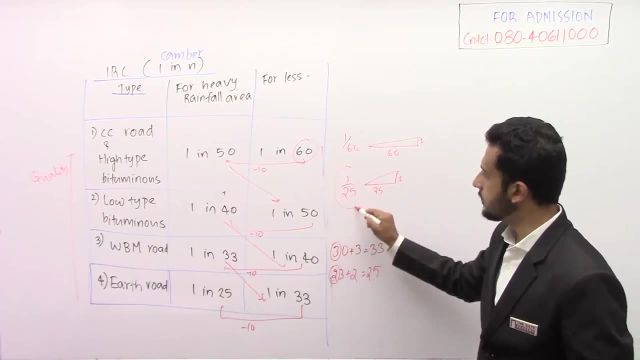 or 1 in 25?? Whenever you are going 25 here itself, you are having 1. Means that is 1 by 25. So 1 by 25 is more compared to 1 by 60. So as the quality is decreasing, 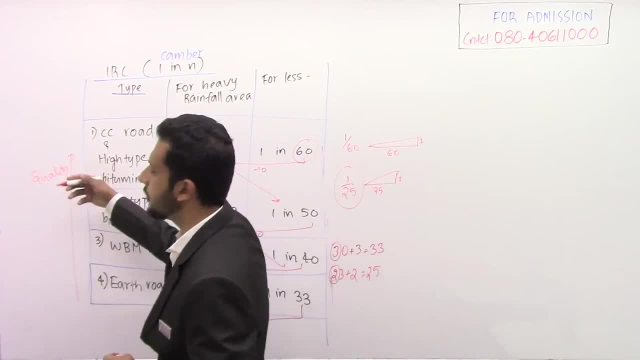 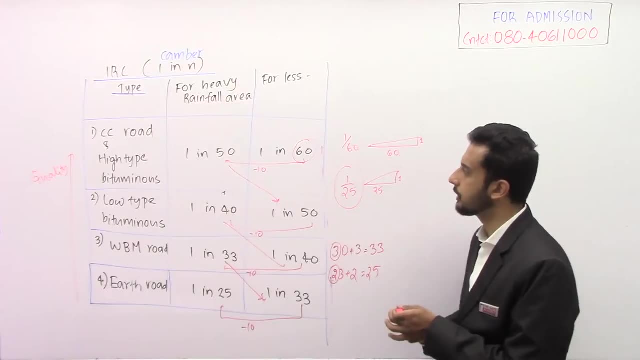 camber is increasing. That point also you remember. You can write it as a note after this. So as the quality is decreasing, camber will be increasing. It is reciprocal Right. It is having highest quality. So 1 in N, Nothing, but 1 by 60 is less. 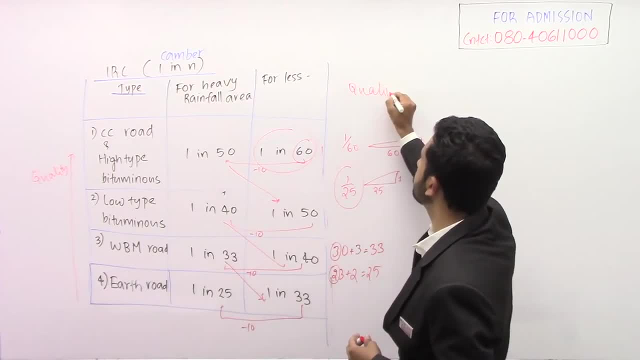 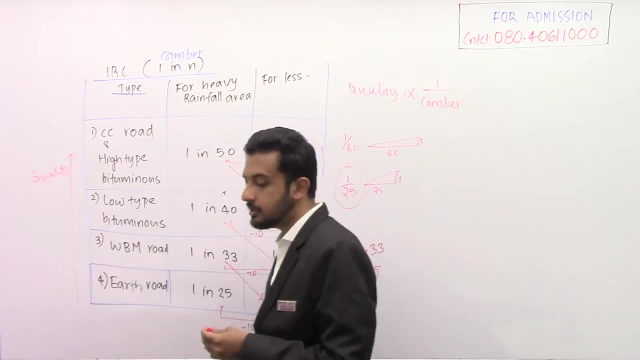 value. So you can write that point: as the quality of pavement increases, the camber is going to decrease. Yeah, That is why someone has asked whether in cement concrete pavement we are going to give camber or not. Yes, we are going to give, But it is. 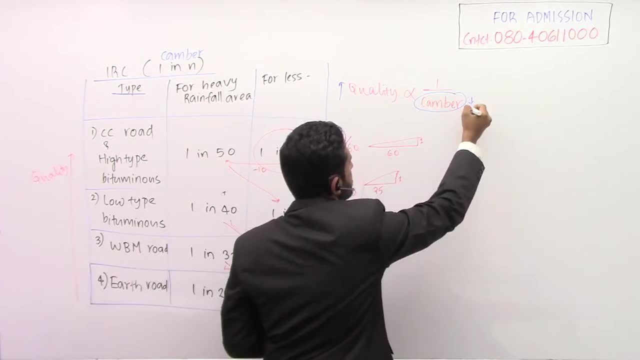 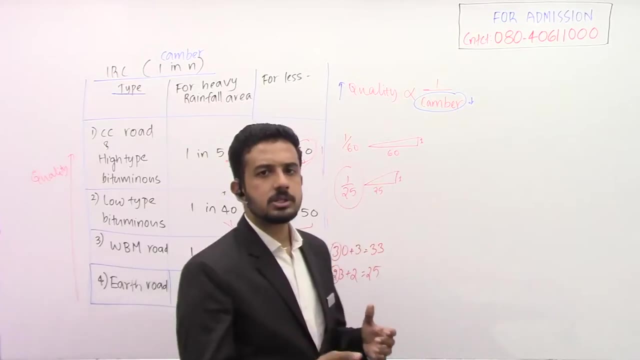 having highest quality. So the camber will be very less. That is what I told: Very less camber. What is the recommended value? 1 in 60. See, suppose in the question they are giving some other value, Then we have to take as it is. 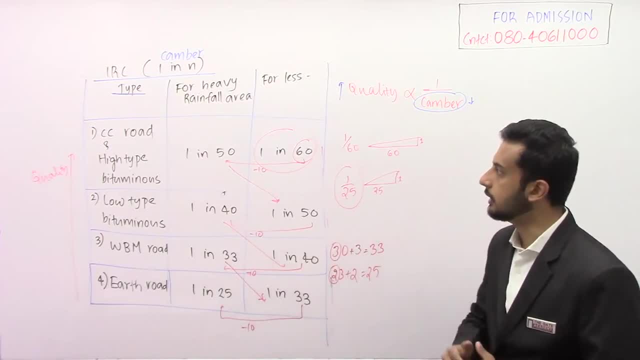 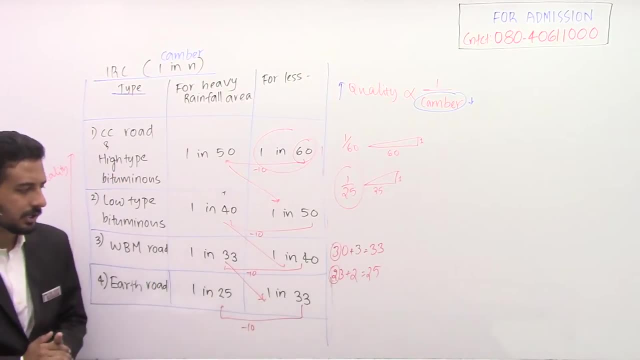 In case, if they are not giving, then only we will go through this table given by IRC. Okay, So I am giving you a numerical question, Rather than just by hiding all the formula or the parameters. just apply in the questions and see how to use in our GATE exam. 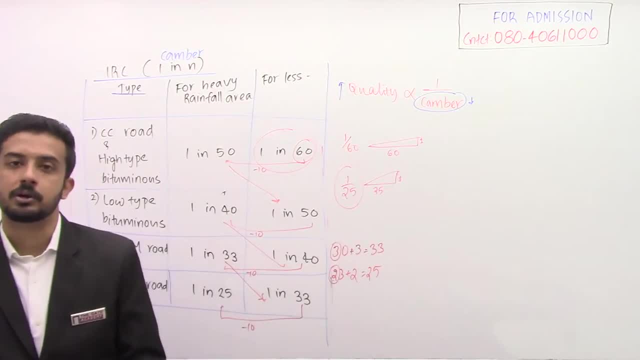 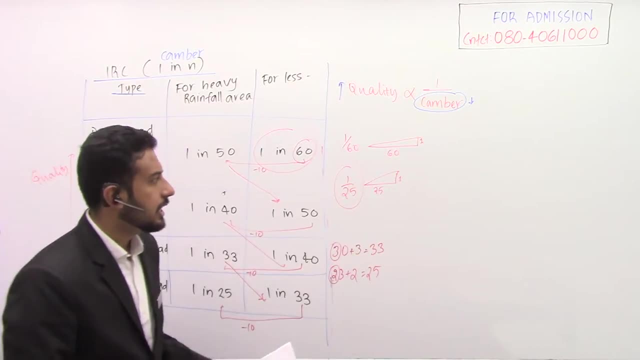 Okay, So just take down a question. I am just going to give a question, You can just take down, Write it. A two lane cement concrete road. a two lane cement concrete road. We can use the short wording is not all. again, Right. 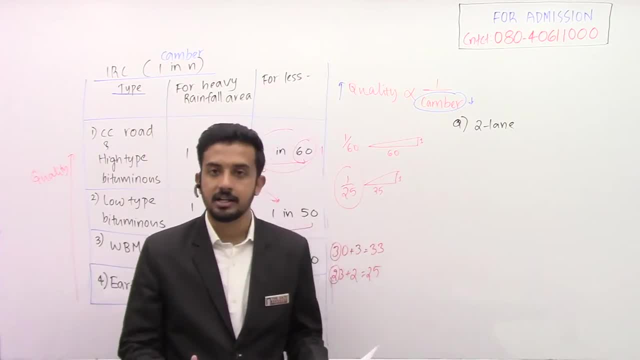 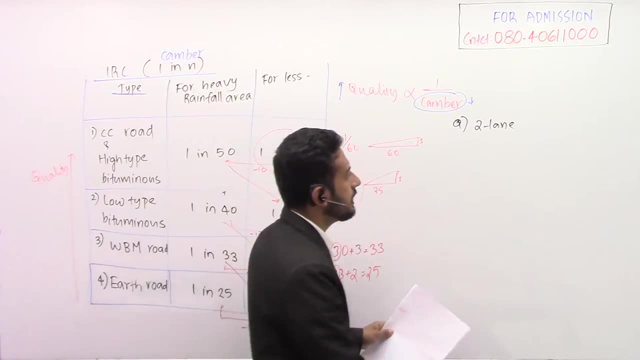 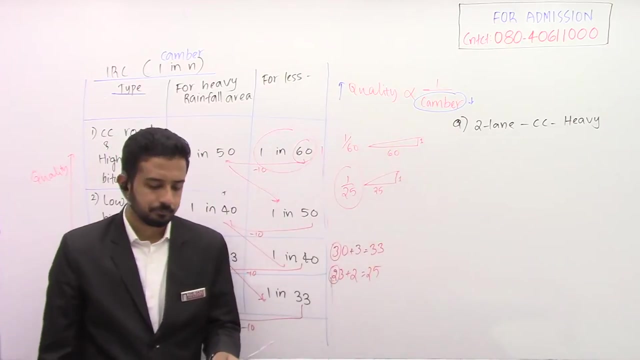 A two lane cement concrete road is to be constructed at a place of. is to be constructed at a place of heavy rainfall. A two lane road, CC pavement. It is going to construct at some heavy rainfall area. Next sentence: What should be the height of crown? 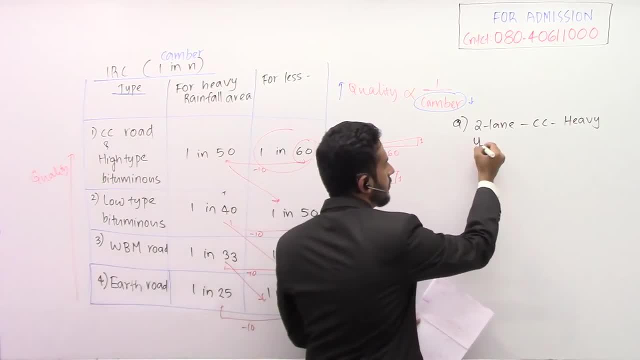 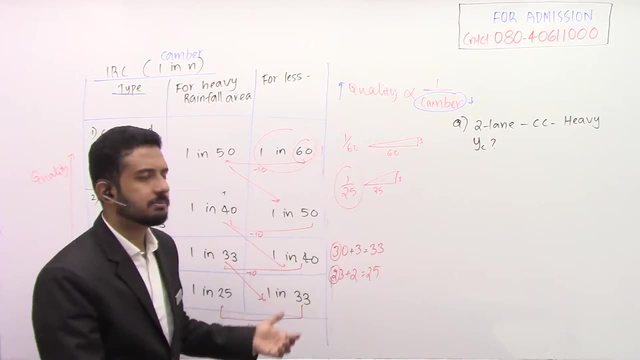 What should be the height of crown? What should be the height of crown with respect to the edge of the pavement? Yes, Same thing: What is the height of the crown with respect to edge of the pavement? Maybe that's why they are going to ask. 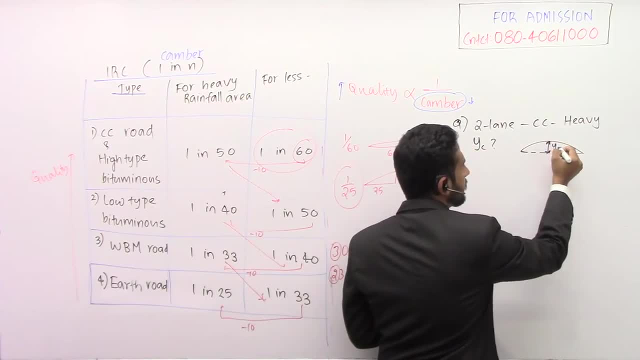 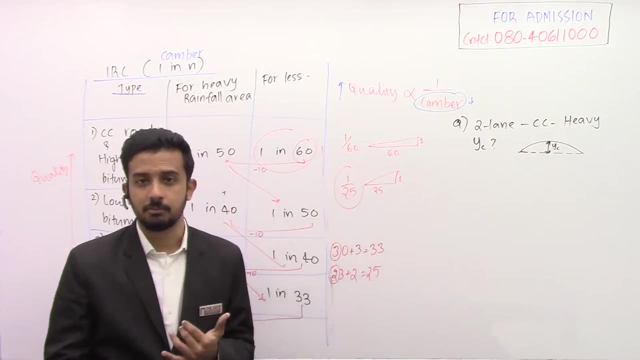 That's how they are going to ask. Height of the crown means what with respect to edge of the pavement? Yes, Calculate what will be W. See, they have not given the value of W, Not given the value of N, If it. 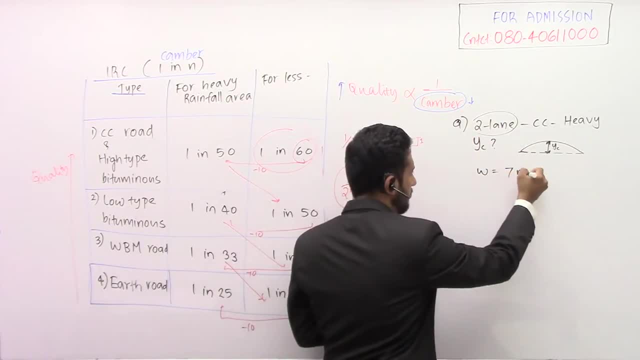 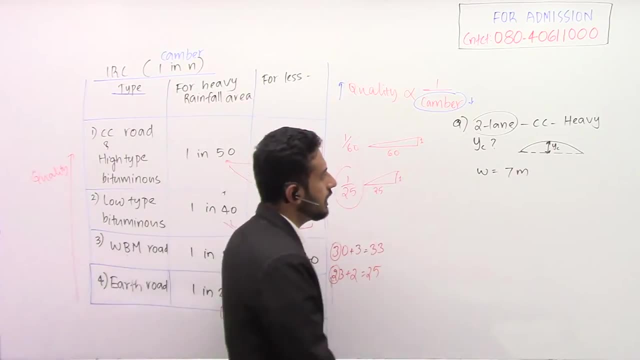 a two-lane road. by default for a two-lane road, w is seven meter right. if it has given that there is a raised camber, then we have to take 7.5 n value. so we know the equation is w by 2n, so w. 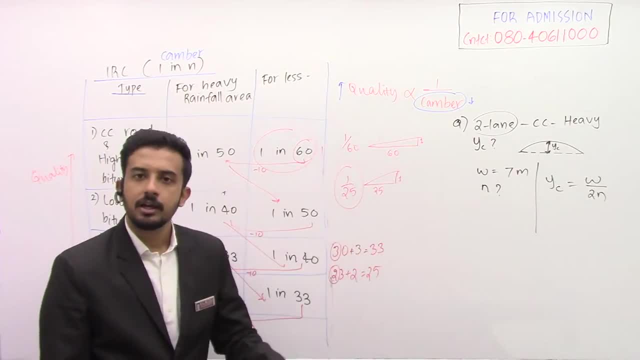 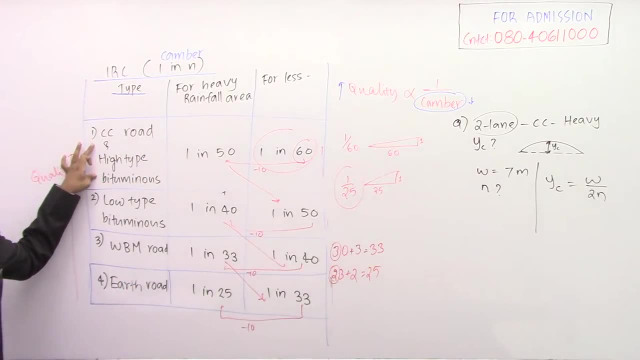 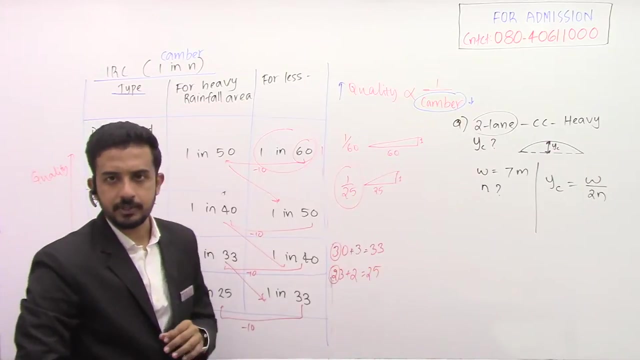 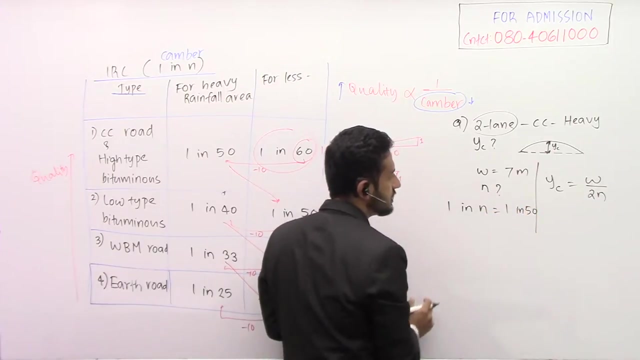 we already know: 7 meter. n means what in the one in n. what is that n value? it's a cement, concrete road, which means the first one, and it is having heavy rainfall area, which means camber is 1 in 50. camber means what? 1 in n? 1 in n is 1 in 50. then what is your n value? your n value is nothing but. 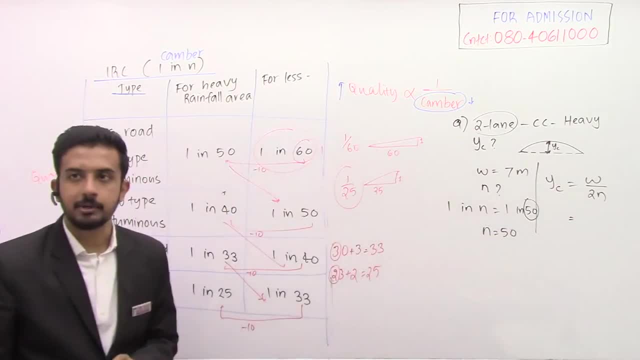 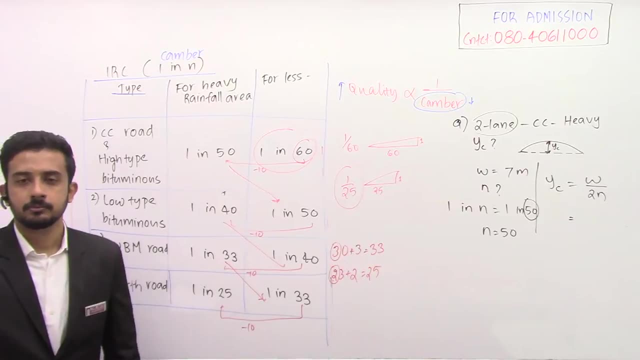 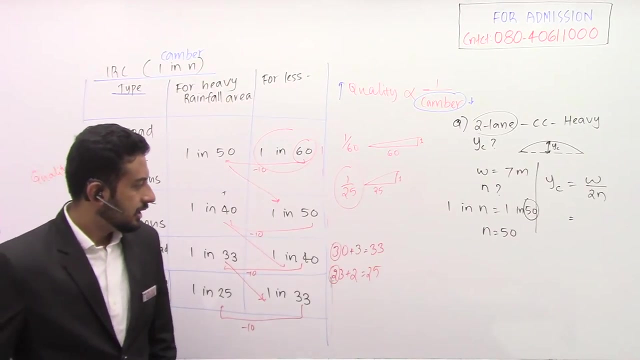 50.. so substitute how much you are getting tell me very good uptal. so substitute how much you are getting s abhishek correct. only for the proper drainage it is necessary to do that and if some erosion, if it is going to affect the road, we will be taking this other. 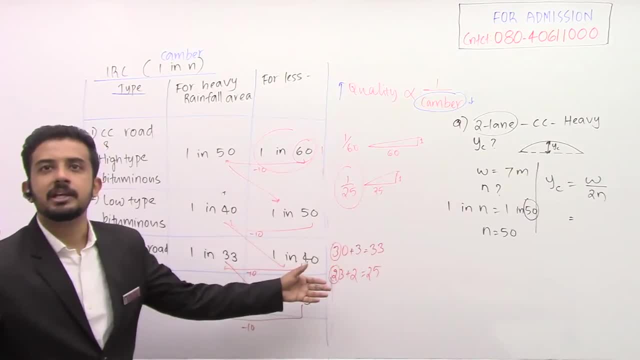 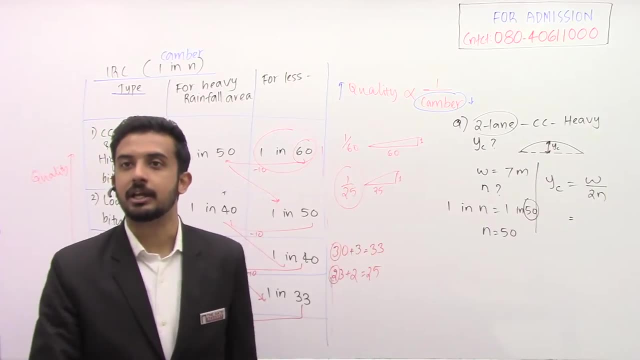 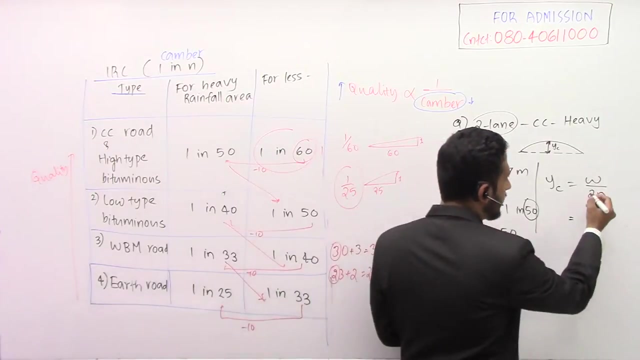 preventive measures also. so give me the answer, others please. what will be the value, so that i'll be, uh, understanding whether you are getting the concept or not? so so the unit also you have to take care. so this is 7 meter divided by 2 into 50.. see in whatever. 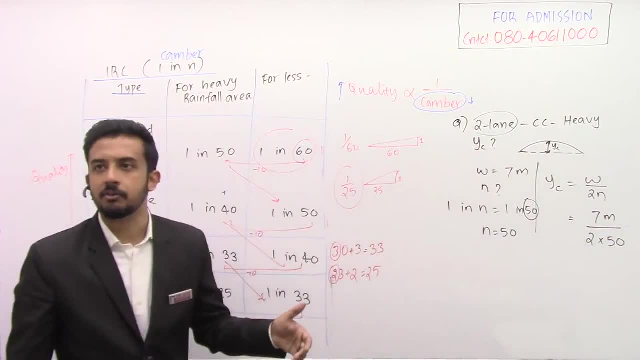 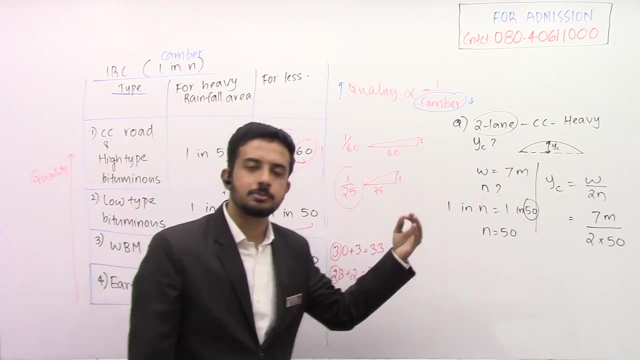 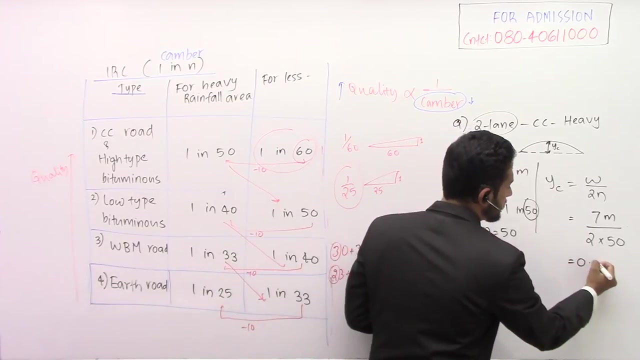 unit: yeah, very good, very good, very good. others also giving: yeah, very good, very good, good. so whatever unit you are going to substitute the width of the road in same unit, you are going to get it because these two are having no unit now, so this will be 0.07 meter, suppose the question is. 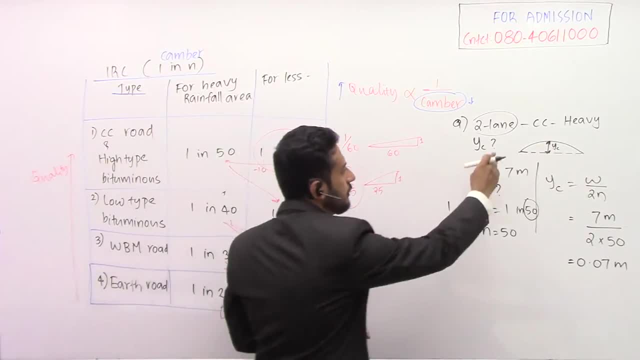 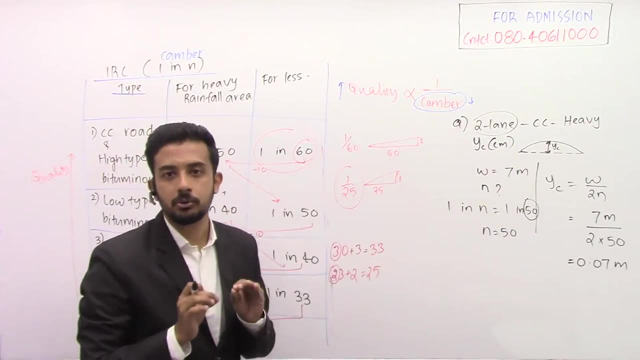 what is the height of crown to the road in centimeter? so in transportation, this is the one of the important thing you need to have to take care. like anything, they can ask you a variety of questions, but the thing is in bracket. they will put the unit also, so in case, if it is a numerical answer type question, you are not getting the 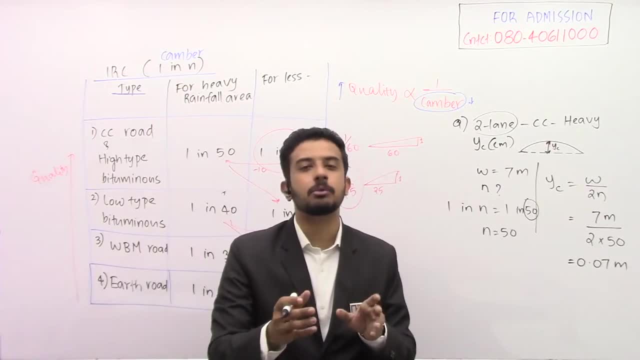 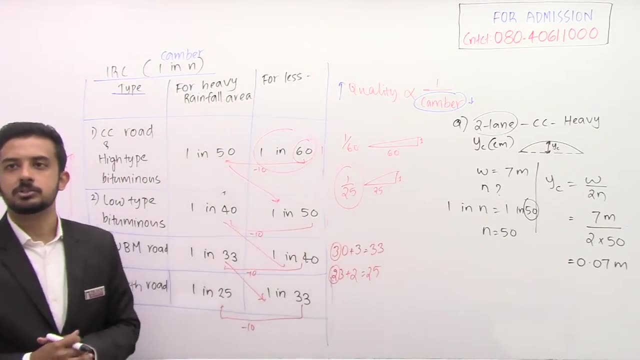 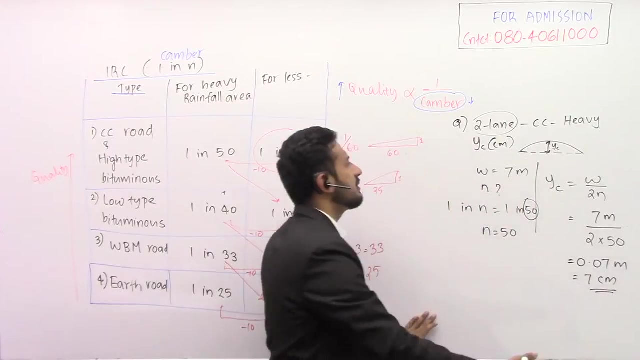 options so you will not be realizing that you are entering some wrong answers. so, especially for numerical answer type, always take care of the units. yeah, very good, very good, manjita, the very much is good. so 0.7 meter, nothing but 7 centimeter, okay, so in whatever unit they are asking, 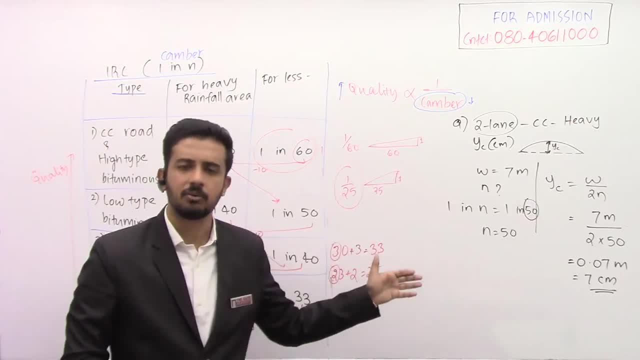 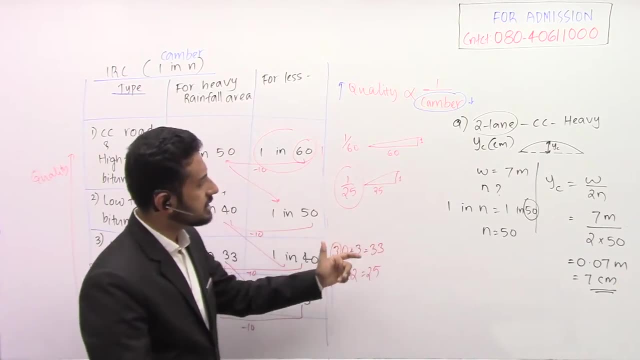 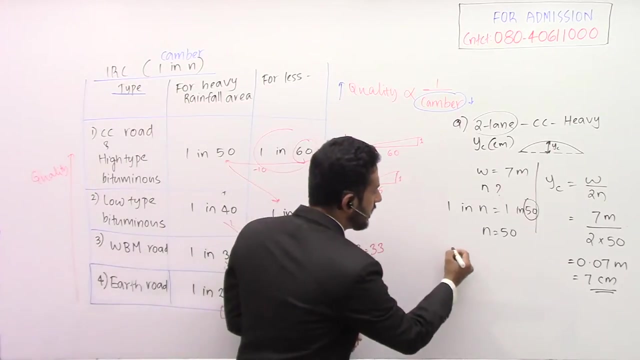 accordingly. you substitute here. i have not given the units, okay, whatever it is, so, 0.7 meter, understanding how we are going to substitute. uh, suppose the same question? i'm just giving you another question from the same question. instead of heavy rainfall, let the same data do it for. 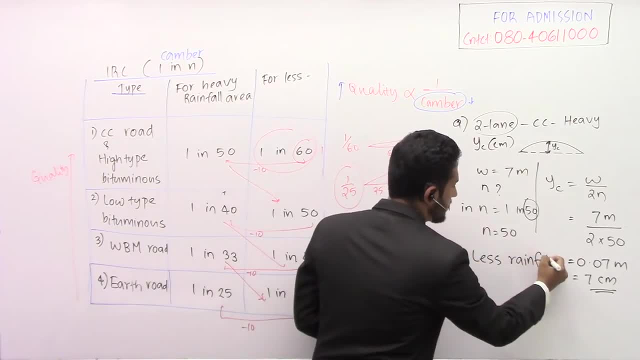 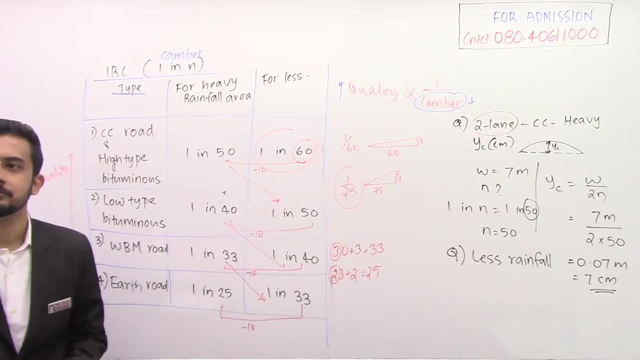 less rainfall area. suppose the area is a less rainfall area. do the same and check what value you are going to get. yeah, very good, in all the subjects. units are very important, okay, but generally they used to make twist in transportation. yes, as abhishek is telling, for hydrology irrigation. 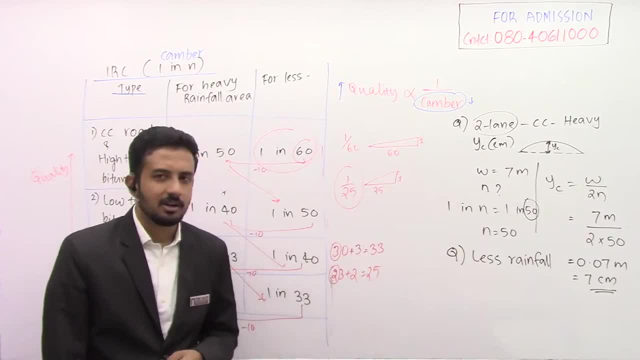 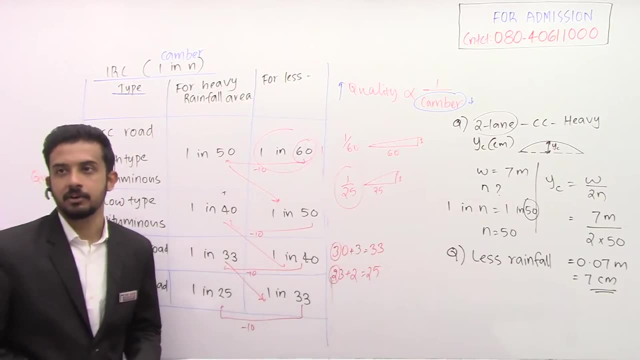 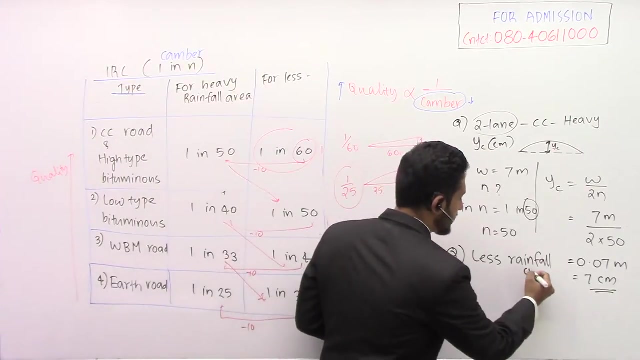 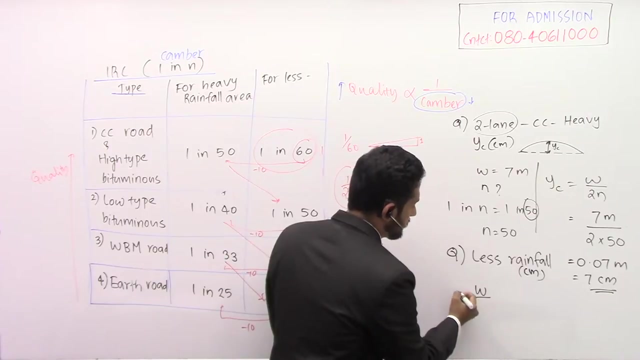 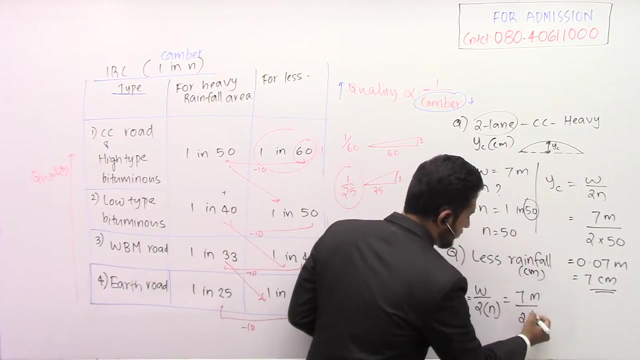 also they used to make twist in the units. okay, whatever be the subject, always take care of the units and then you can make twist in the units. okay, but generally they used to make twist in the units, so they will consider the Algried practiced for this result. therefore, if they are irregular. 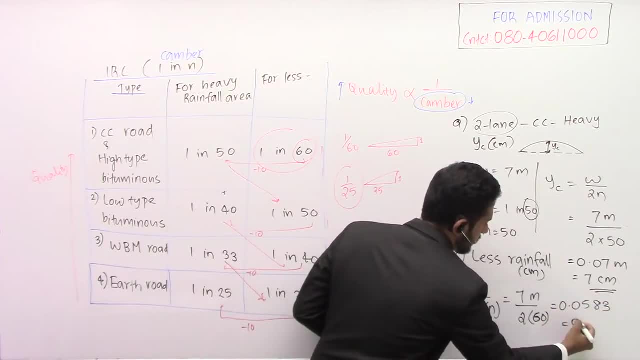 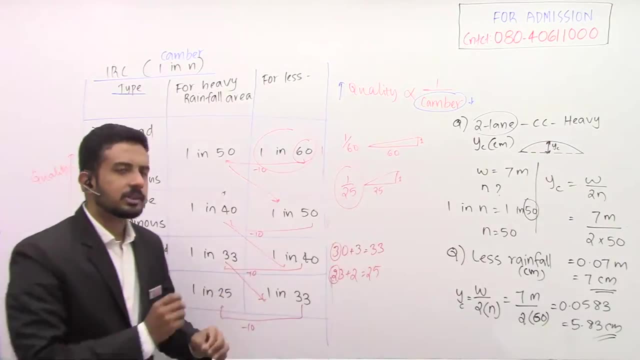 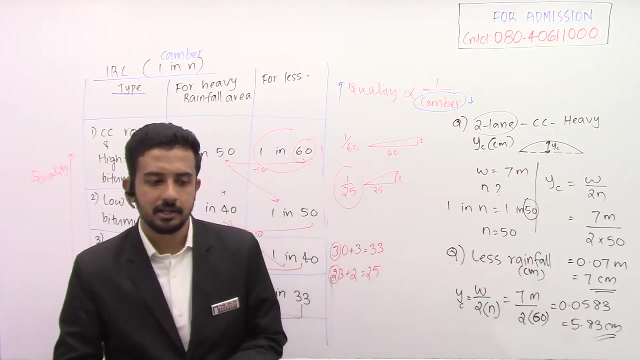 values. actually they could be useful, 5.83 something, i guess. so 5.83 centimeter getting very good, 5.8. see one more thing i'm telling you. uh, generally for gate examination, apart from the unit they will be giving in bracket round off to: 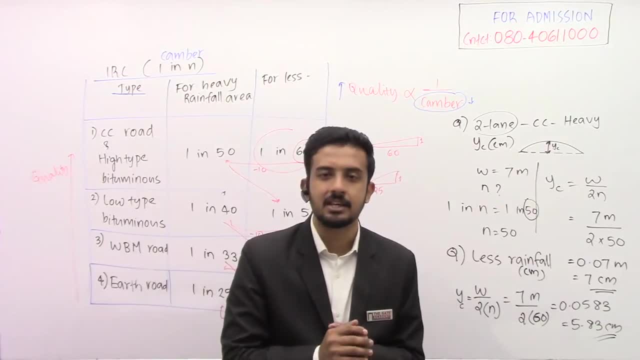 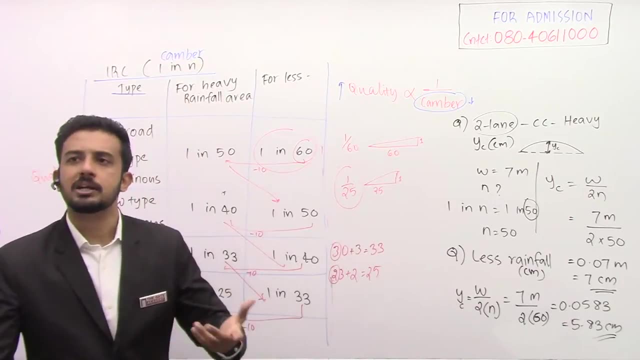 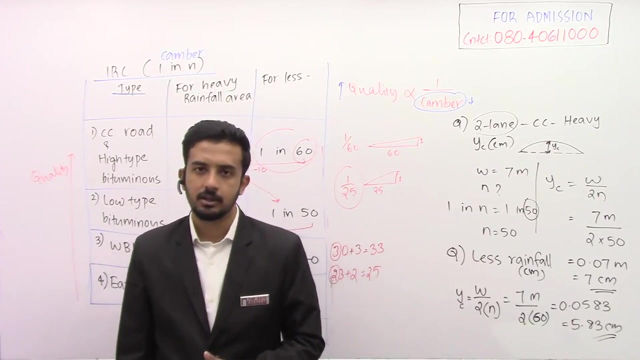 one integer place, one round off to two decimal places, round off to one decimal places like that. okay, so always take the values very accurately and whatever they are going to give, you suppose in this question they are giving round off to one decimal, which means it is 5.8. okay, suppose you are. 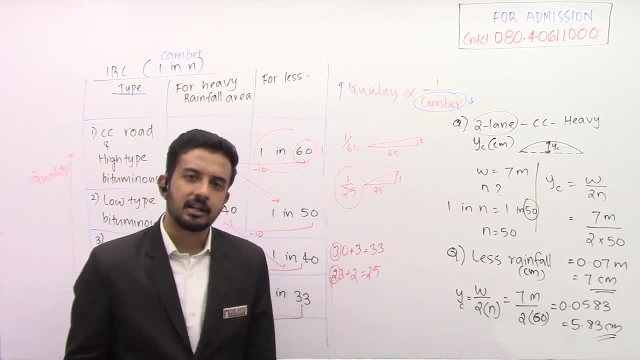 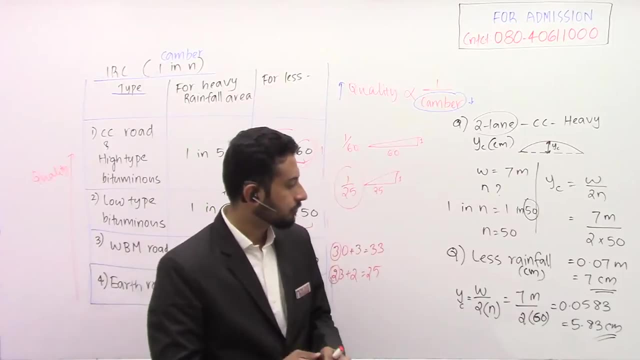 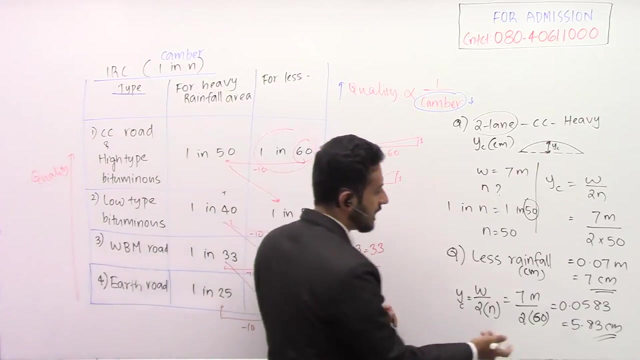 getting some 6.97. you can either write it as 5.9 or 6.0. the range may be something like that. so proper range they are going to give. okay, so in this question, 5.83. in case the question was round off to one decimal, which means after the decimal point there should be one. okay, they will. 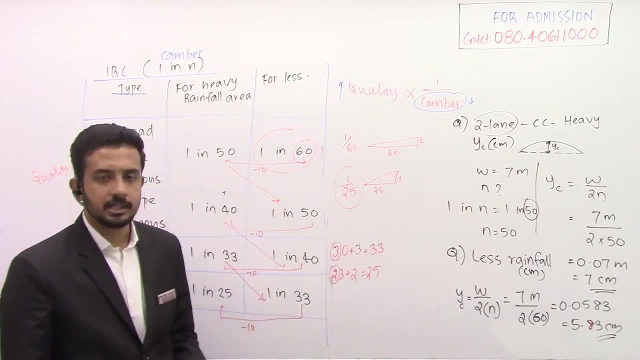 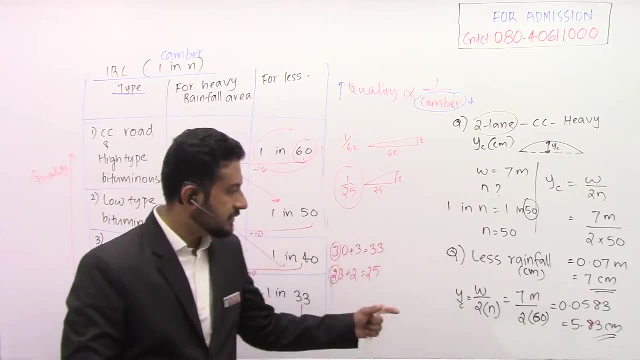 give a range, so 5.8, like that. okay, so always check. uh, sometimes they will give round off to the nearest integer. take care of those things, okay, if it is round off to the nearest integer, which means it is six, so maybe in the range they are going to give some five to six or something. okay, depends, okay may. 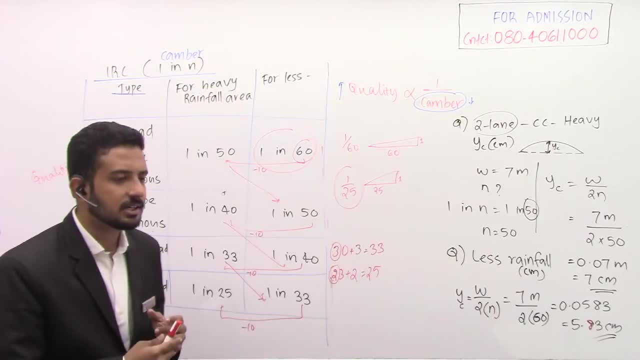 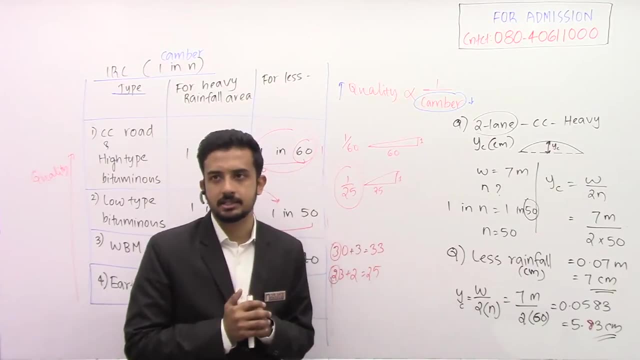 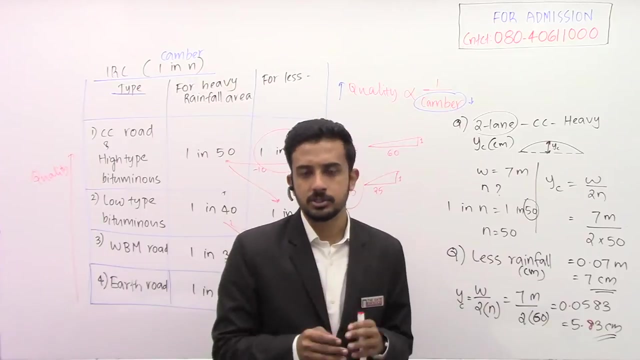 not be for this question. i'm telling in general: okay, always check in which unit they are asking the question and up to what decimal we have to write the we have to enter the answer. that is numerical answer type, where the options are not available if it is a multiple choice question. 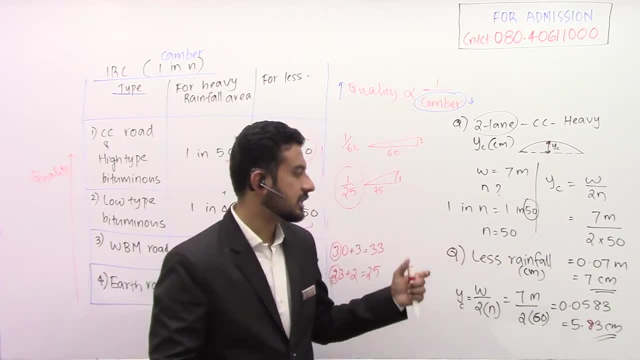 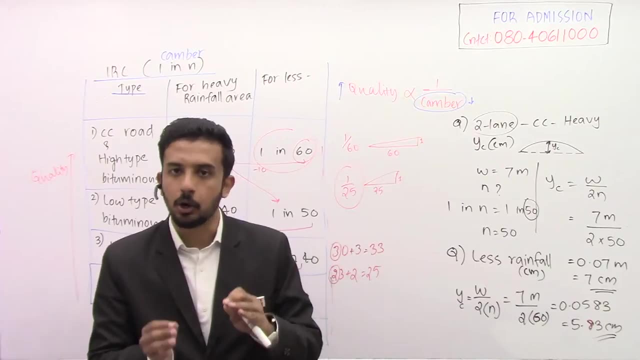 in which you are having the options, then no need to take care of those things. but unit, you have to check it. sometimes they will give the values in meters as well as in centimeters in the in the options. so always check in which unit they are going to ask the question. okay, so understood. 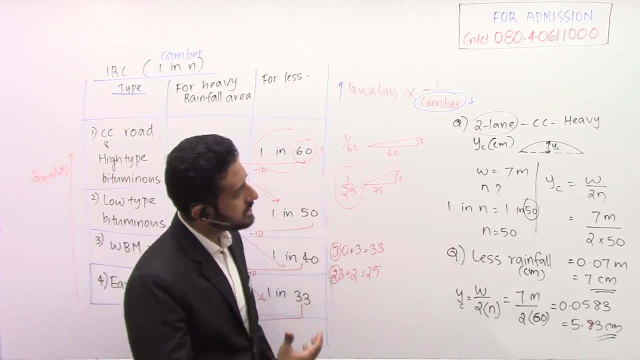 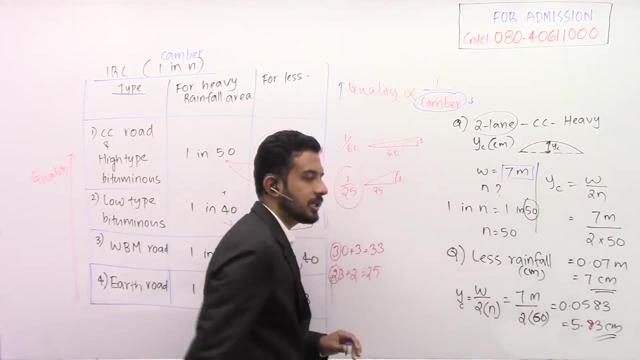 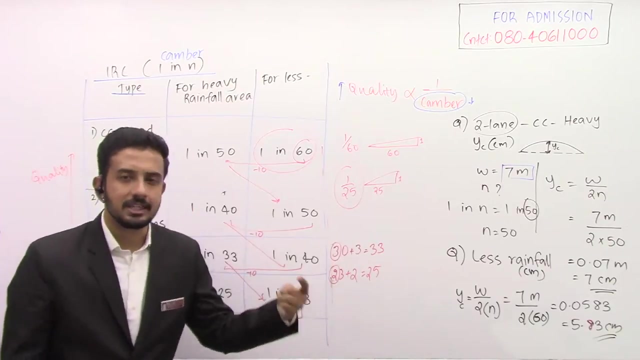 how to calculate the height of crown. sometimes they may be giving you the value directly. see one more thing here. we have taken seven meter. right why we have taken seven meter? because in the question w is not given. that's why, suppose in the question w is given, then we have to take as it is, whatever the value given whenever we are. 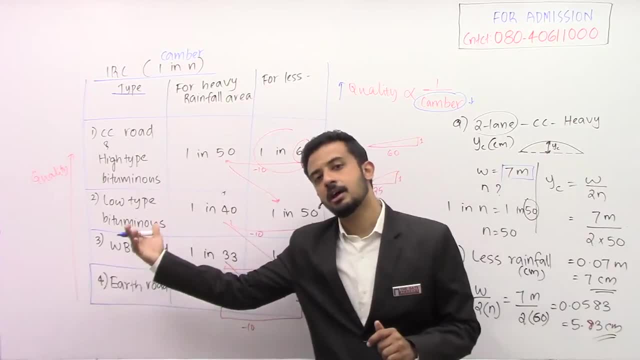 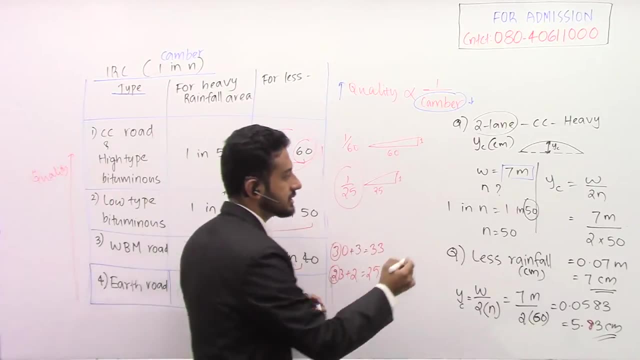 not having a particular data, then who is going to help us? irc is going to help us. to take some standard values, suppose in the same question, they are giving the camber see, instead of this, 1 in 15.. they are telling that the camber is 1 in 55.. 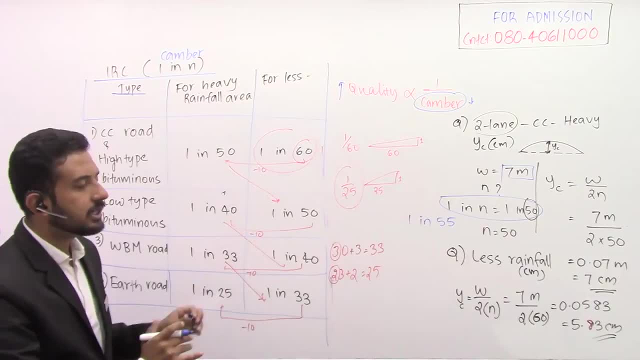 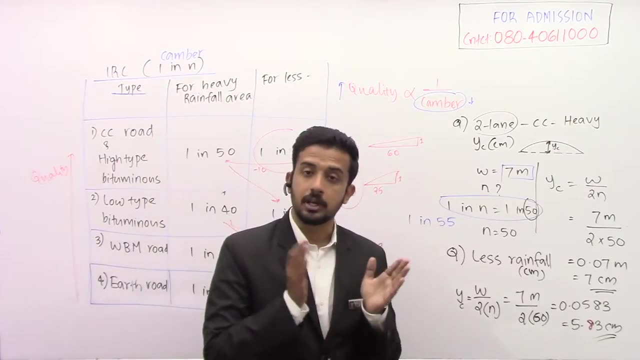 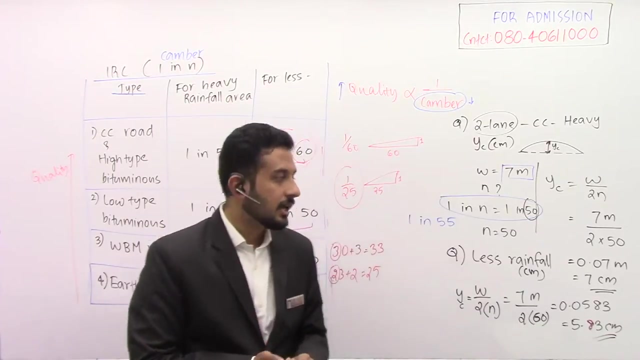 Then you have to substitute 55 only. whatever they are giving, take asset is. sometimes they will give some other subjects, see acceleration due to gravity. if they are not giving, we will take 9.81. suppose they are giving the value as 10, then you have to take it as 10, right, and also we. 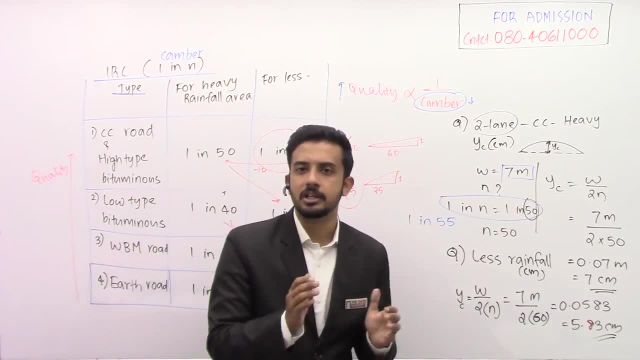 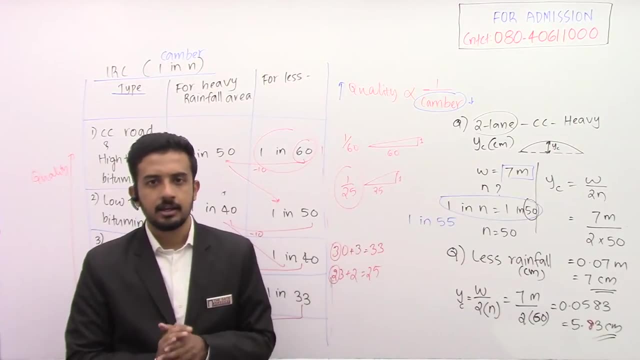 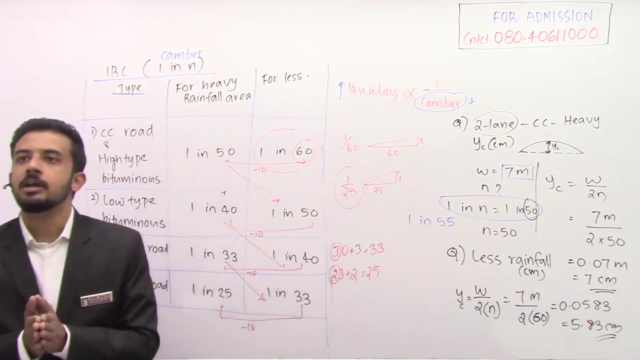 have studied the coefficient of friction 0.35-0.4 and lateral friction 0.15. it is the standard values for design. Then question: if they're giving some other value, we have to take the given value. okay, yeah, that's what. so and the difference between wbm? see, we are having so many roads. 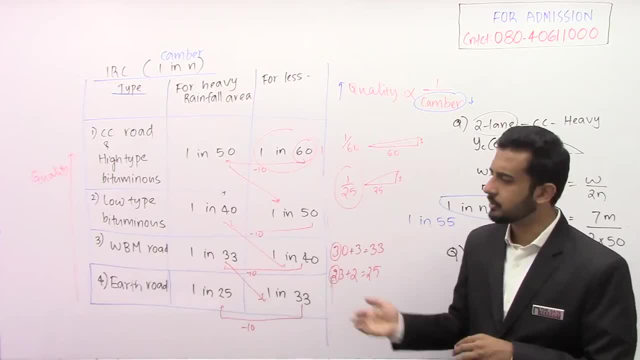 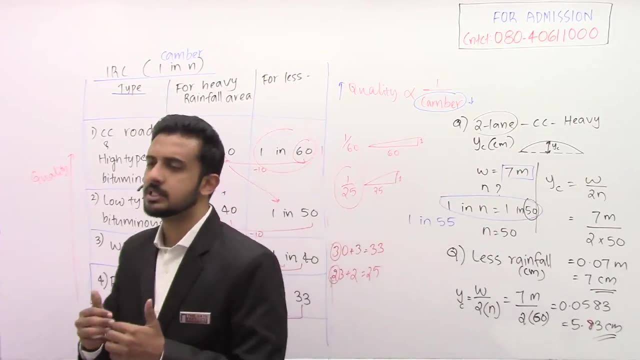 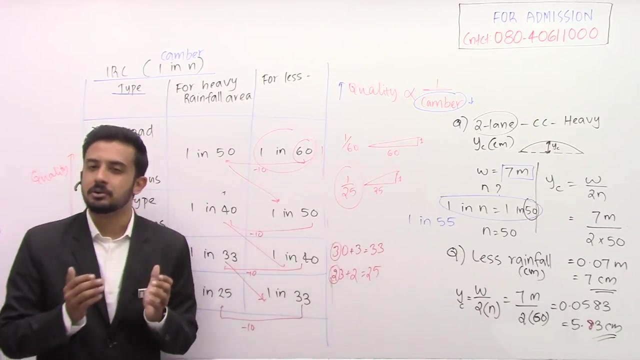 water-bound meccan road. wet mix meccan road. so many things are there not required for gate examination: okay, for bituminous payment. we are using so many param in like course. aggregate- we'll be using fine aggregate. we're having so many mixes and all so in detail we don't require. 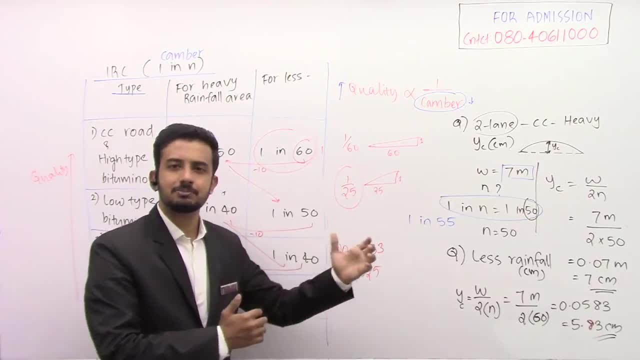 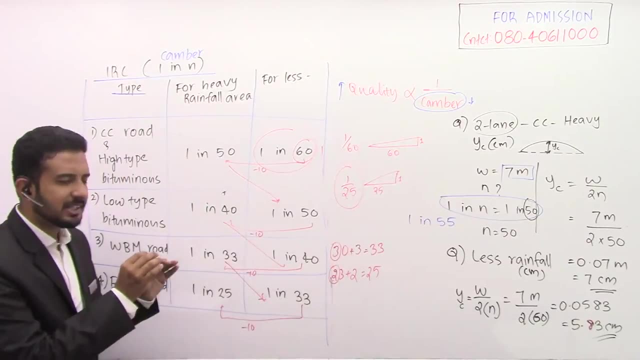 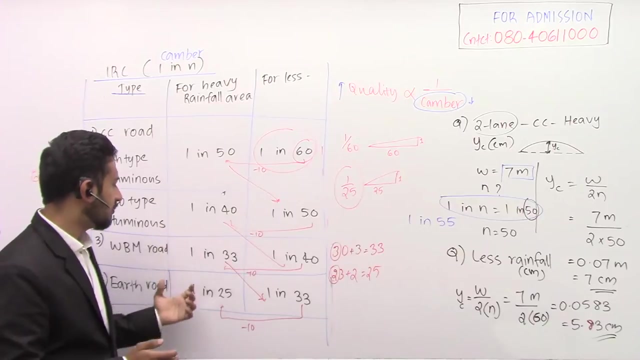 for this particular concept when we are going into the payment materials, payment design. still, if you want to know that, definitely we'll be discussing there. okay, so but always check what all things are actually required here. we don't require those things actually also for gate examination. we don't require what are the construction methods for these things, if you. 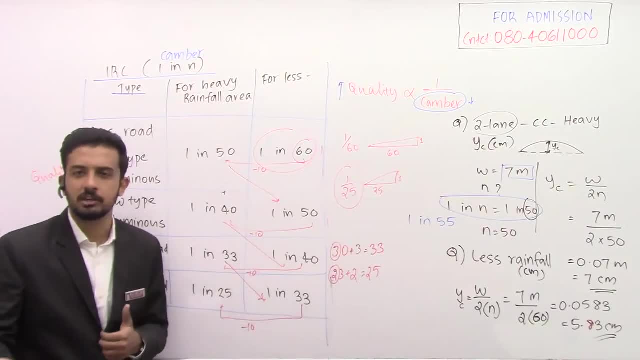 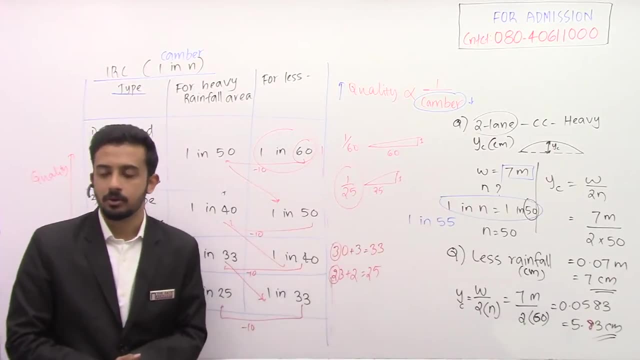 really wanted to know. i will give you my mail id and all you can ask me. i will give you the reply, don't worry. or whenever we are doing the payment, design sessions and all we can discuss there, no problem, okay, so i hope you understood how to calculate the camber and all. so that is. 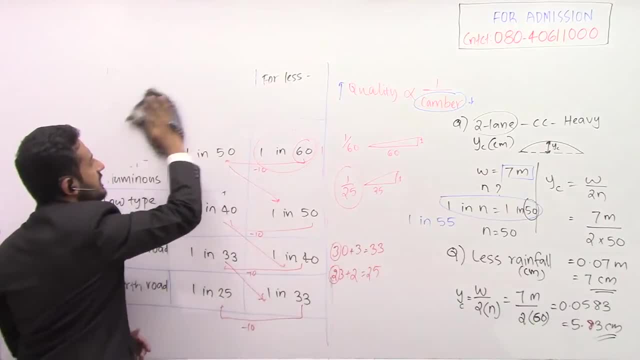 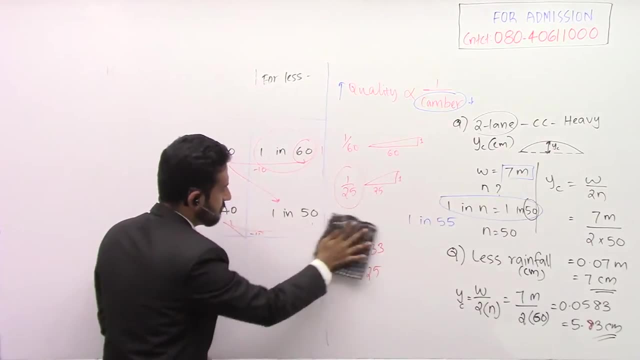 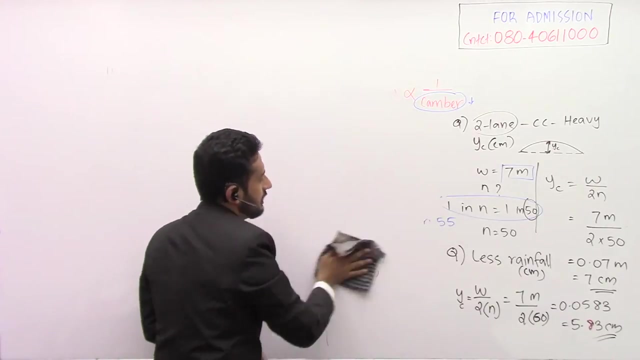 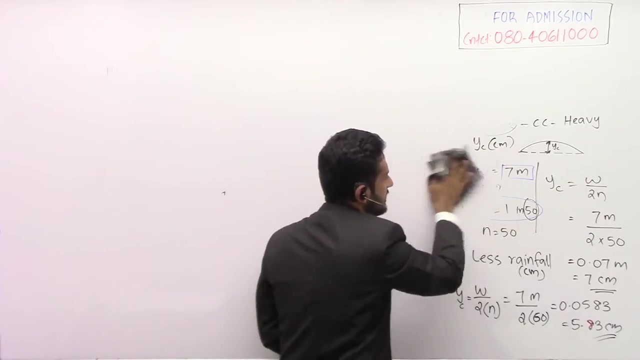 one of the important parameters while considering the cross-sectional elements, and we are having some other cross-sectional elements also, such as median and all uh, not that much important for gate examination. now i am going into the site: distance, okay, one of the important thing, i will, but before that i will 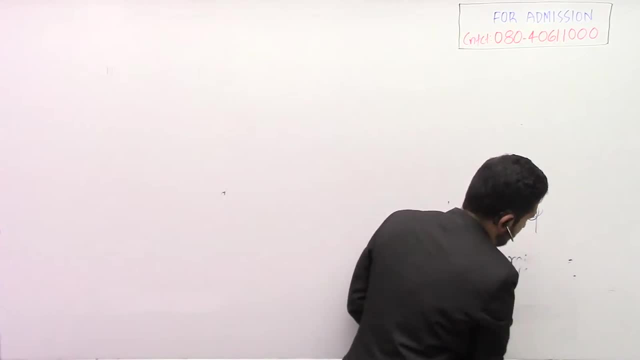 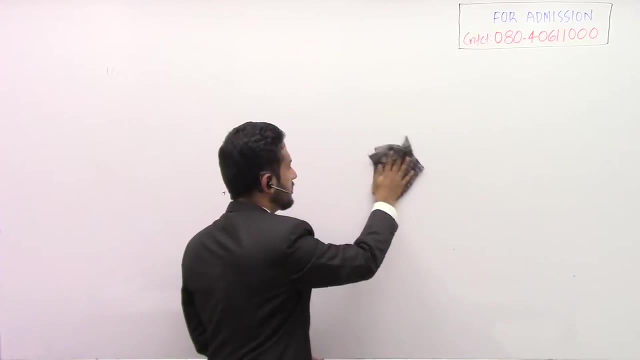 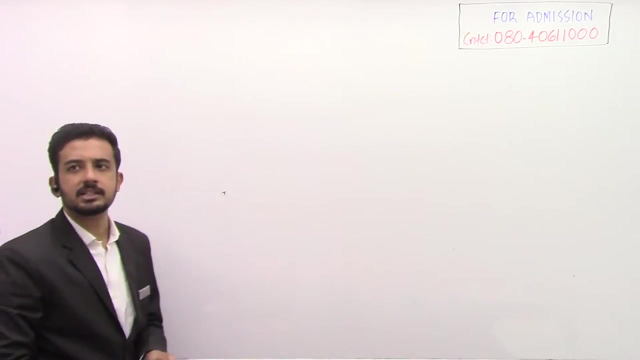 just list out what are the other cross-sectional elements, not that much important. whatever we have discussed will be sufficient, will be more than sufficient, to get a one mark or two marks from the cross-sectional element portion. okay, so there are some other parameters also, such as the next one. you can write it as median: 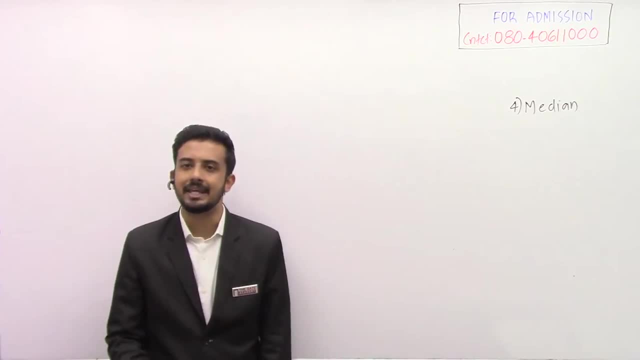 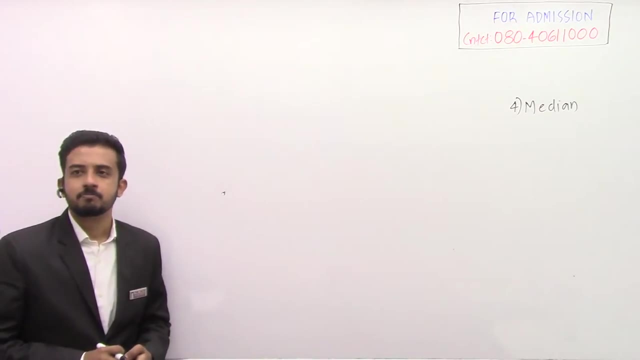 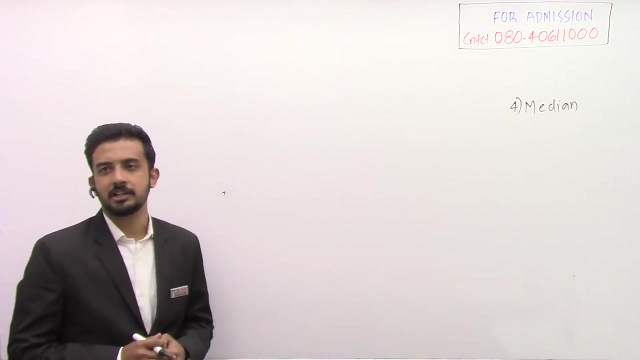 what do you mean by median? just tell me what is mean by median. everything is very much related to our day-to-day life, right? what do you mean by median? why to use median? what is the purpose of using a median road separator? ah, very good, i will be giving you the exact thing, see, suppose. 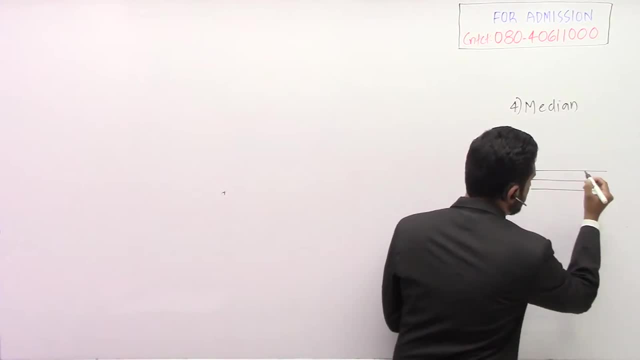 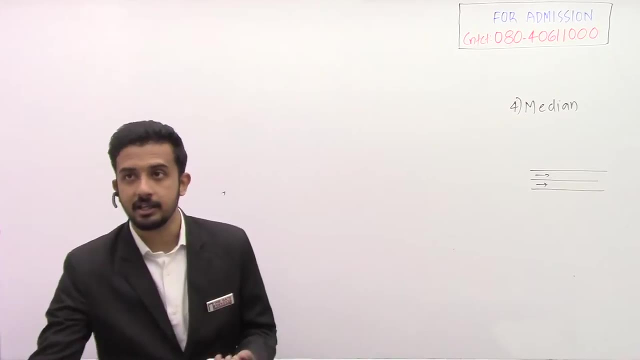 there is a thing, there is a. there are two roads or there are two lanes, both are going in the same direction- whether we will be using a median here. what do you mean by median? yes, road separator is actually correct, which means we are going to construct something here, right? so if both are of 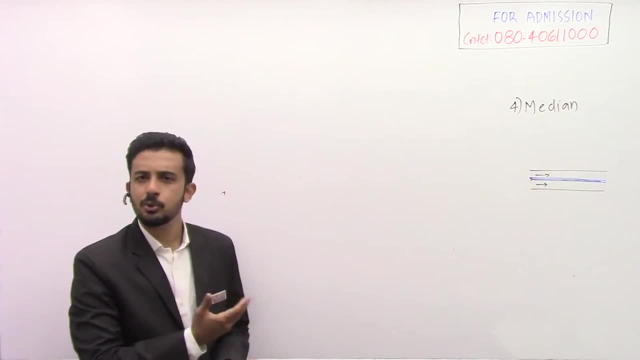 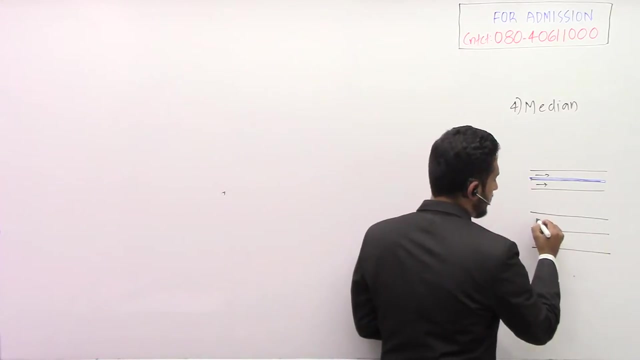 the same line, same direction, will we use a median? no, we are not going to use a median whenever we are having two different directions. yeah, very good, manju, if you are having two different directions. suppose these two are two lane roads, so in this road it is going in this direction. 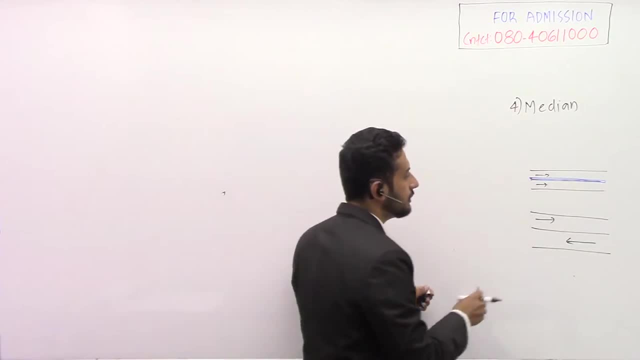 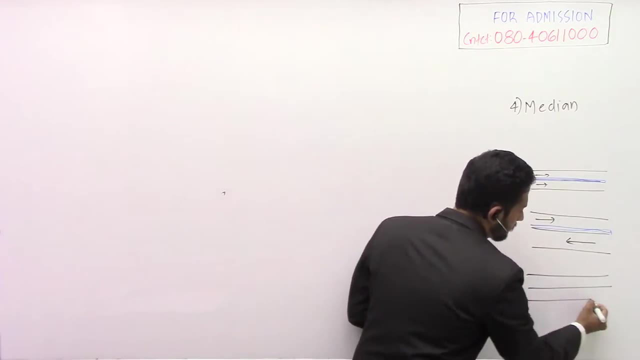 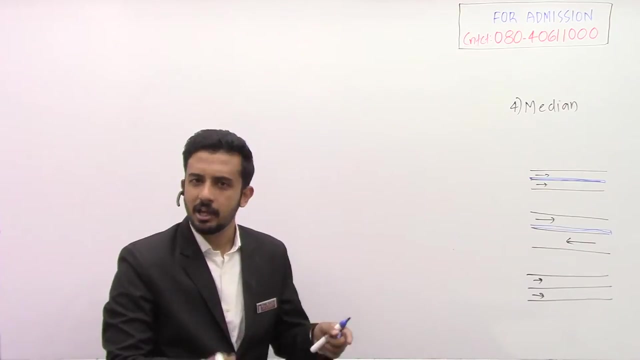 here it is coming in this direction, then we are going to use a median or, if it is a four-lane road, generally for a four-lane road, how the directions will be. here it will be having in the consecutive two lanes it will be having same direction and on the third line it will be having this direction. 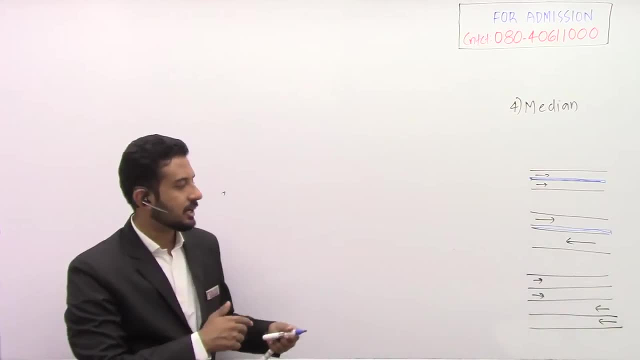 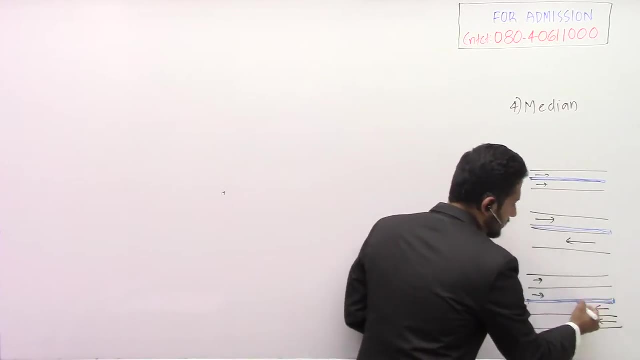 fourth line. it will be having this direction. so generally, this is what a four-lane road is right. so for a four-lane road, we will be having a median here, just to avoid that head-on collisions. that's why we are using median. so what is actually median? 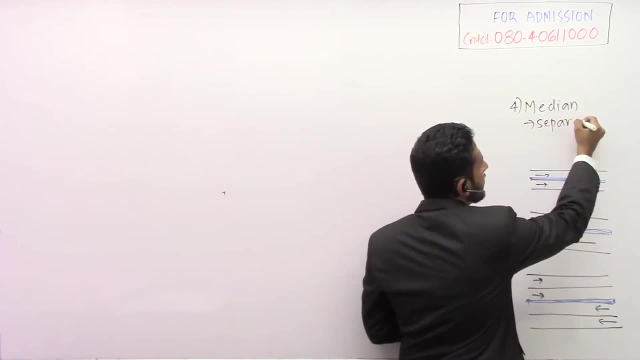 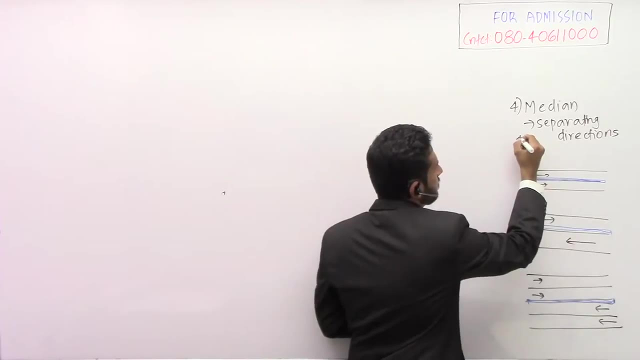 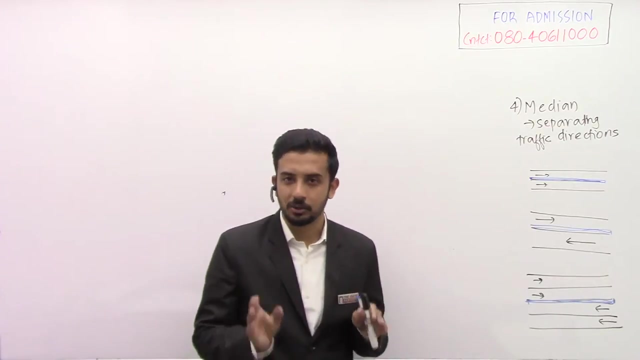 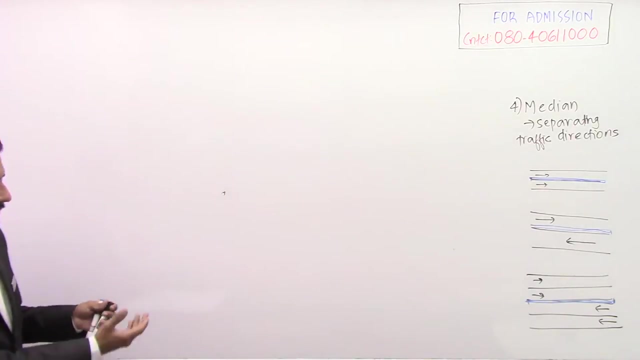 we are, you, we are separating the traffic directions actually. okay, we are separating the traffic direction. so that's what i. i told we know it is used for separating the road, but it's not actually the road, it's. we are just separating the traffic directions. okay, yeah, good, so we are using it to separate the roads, very good. 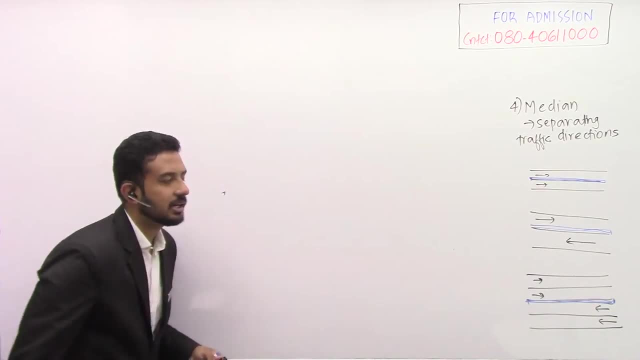 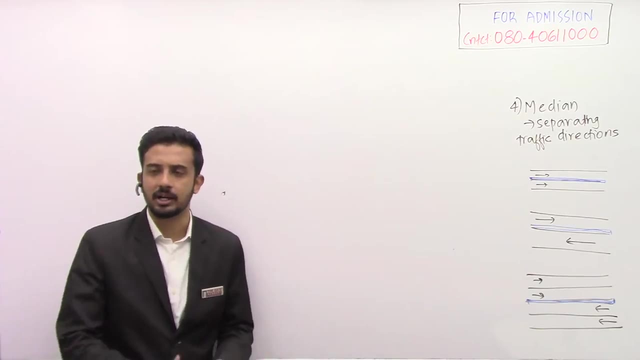 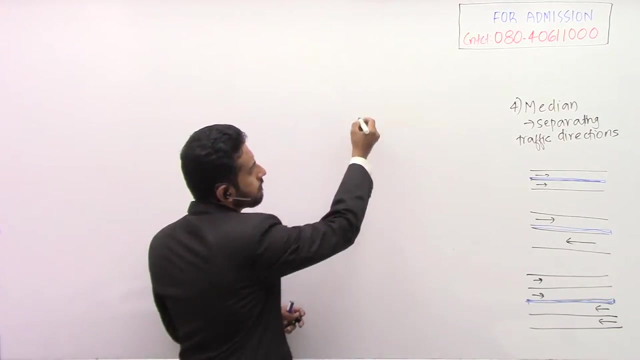 it is also correct, but technically, more precisely, it is for traffic directions, okay, and that is median, then curb. we have already seen what is the curb width of the road. we have already seen that also. then i can tell you: yeah, um, shoulder, is there shoulder? what do you mean by shoulder? 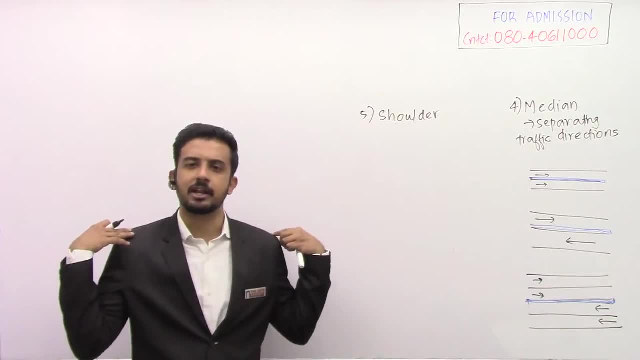 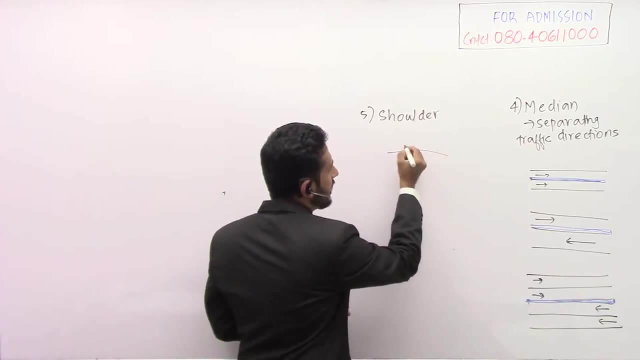 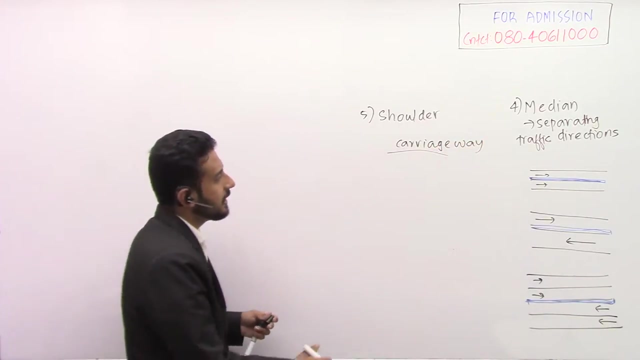 it's nothing, but something like this: on both side we are having shoulders, we are having the head, here we are having the shoulder, exactly like that. suppose this is the carriageway. what do you mean by a carriageway? nothing but where the vehicle is moving, our road, only okay carriageway, and after. 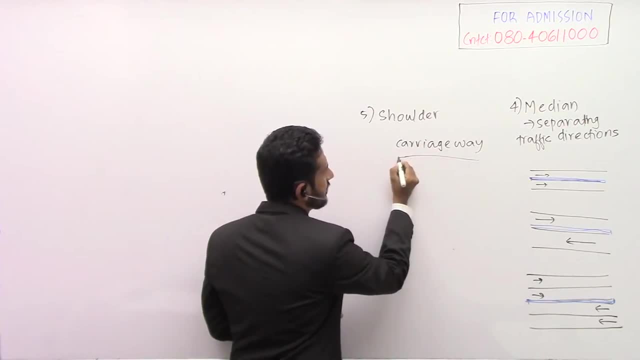 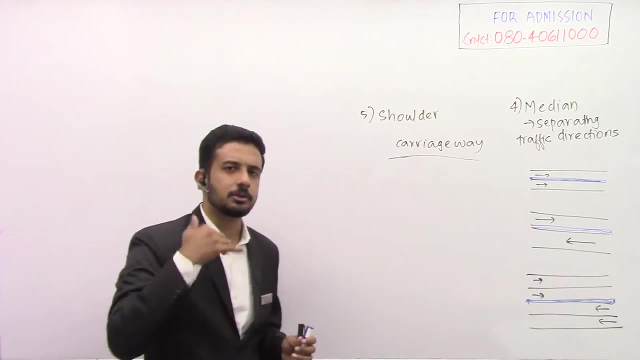 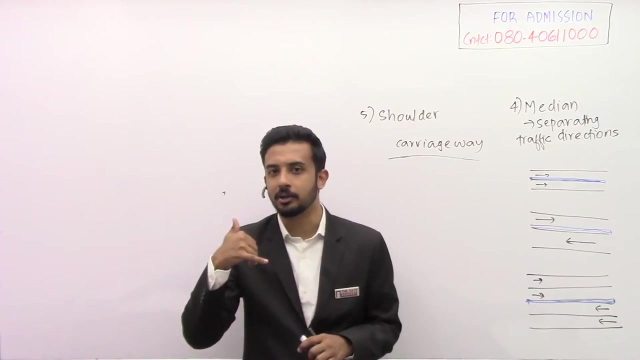 this road. we will be having some portions here, right, some portions- why we are using that portions just for temporary parking. suppose you got a call while driving what you will do most probably you may be slowing down the vehicle and keep on moving while talking. don't do that. you have to park in, uh, on the 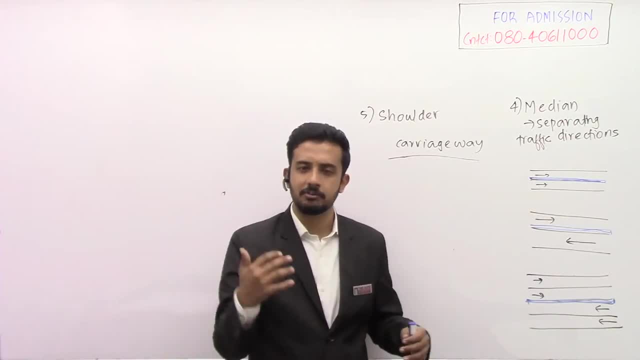 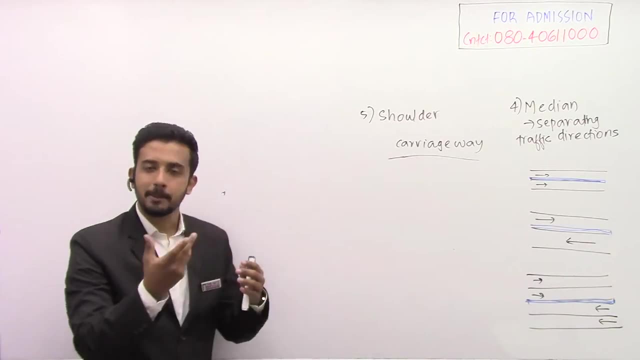 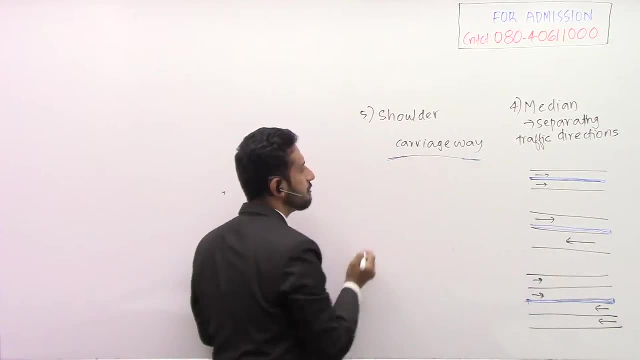 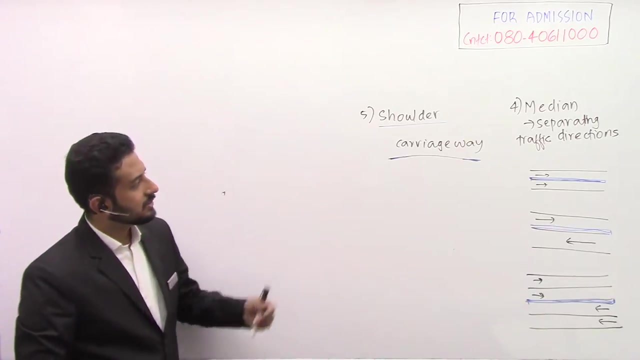 what we require. we require some space here on both side of the road. if you are moving in this direction, you have to park here. if someone is coming from the other direction, you have to park here. so this portion we call it as shoulder. okay, very good, so it is called as shoulder. so this is. 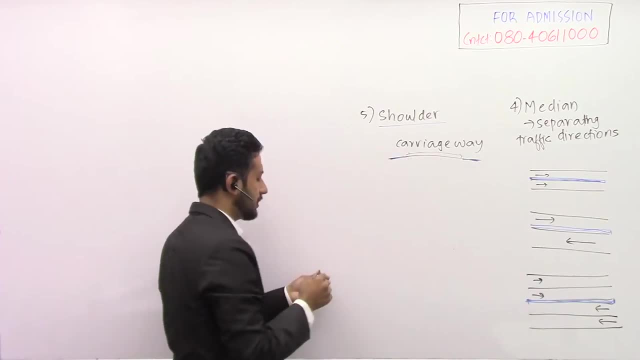 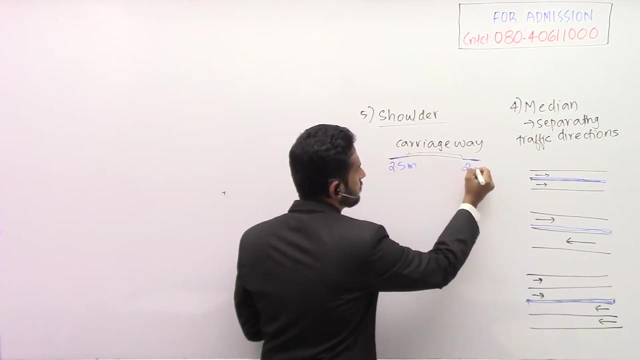 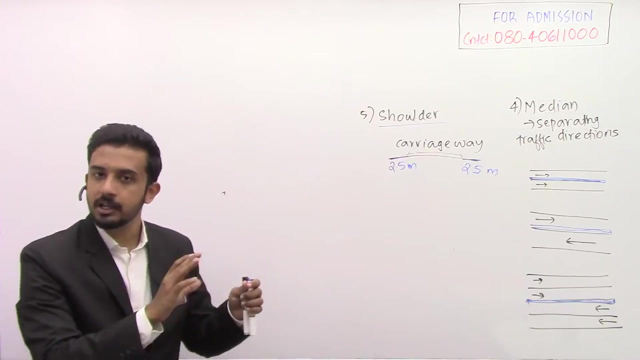 carriageway. this portion is carriageway and this blue portion is called as shoulder. there is actually a minimum width of this carriageway. there should be 2.5 meter, those things you can remember. see why it is 2.5: as per indian. see this value is as per irc indian road. 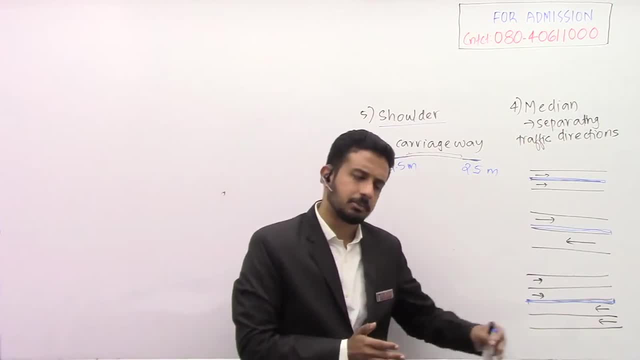 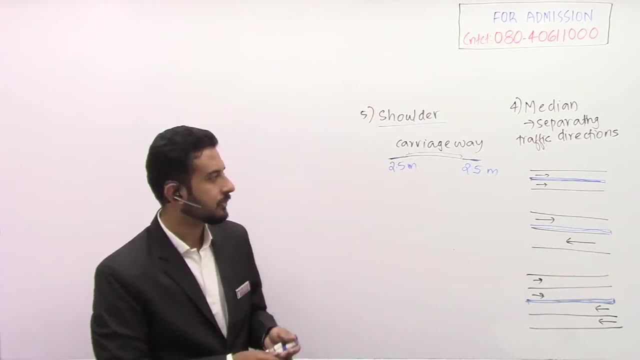 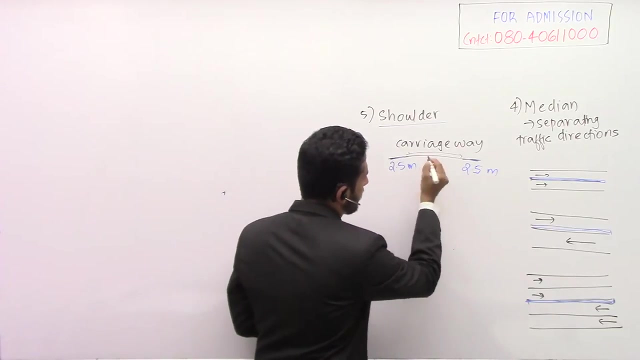 congress. so practically it may not be exactly 2.5, sometimes it may be more than that, sometimes it may be less than that. if it is less than 2.5, it is going to affect our traffic. okay, see why it is 2.5. i'm just giving you for your better knowledge, suppose so? okay, so this is our carriageway there. 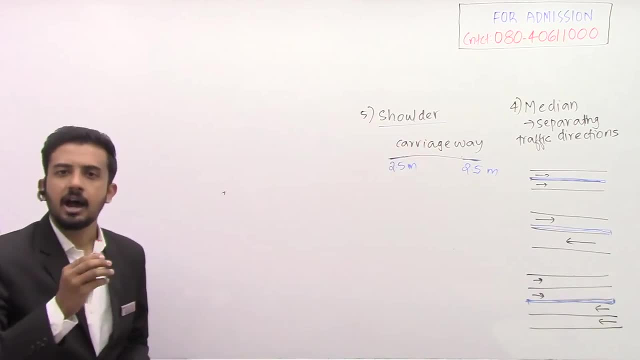 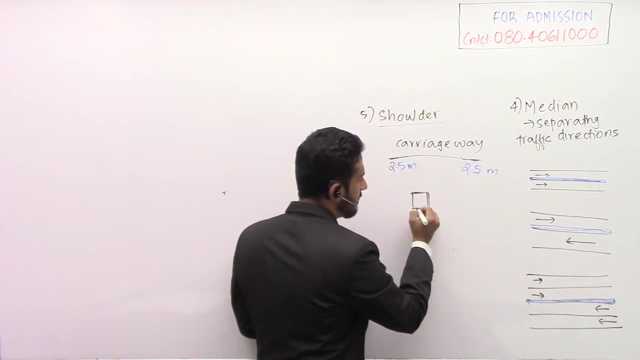 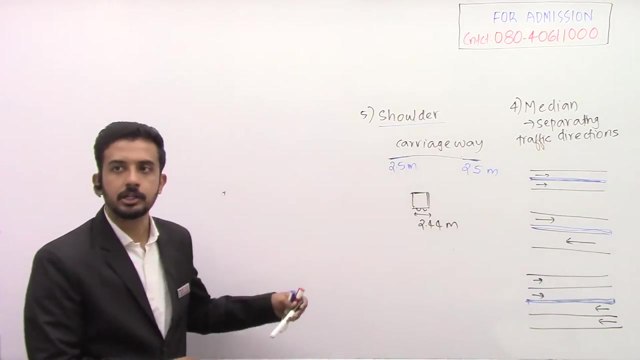 should be some 2.5. now, as per irc the maximum width of a vehicle should be: suppose this is the back side of a vehicle, this maximum width can be 2.44 meter. only note down those things for your better knowledge and for other competitive exams also. these things may help. you see, a lot of exams are there, so yes, 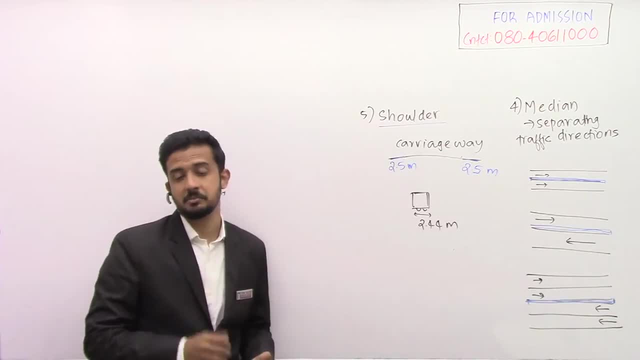 gate exam? is there? rrb exam? is there ssc exam? is there? israel exam may be there. so these things may live. yes, students, ah, for gr c, um and also for reference educational courses, they will be there. if they are getting good scores, many of them may be getting nice scores for. 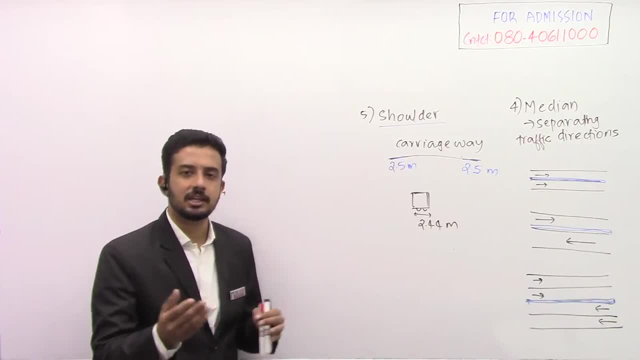 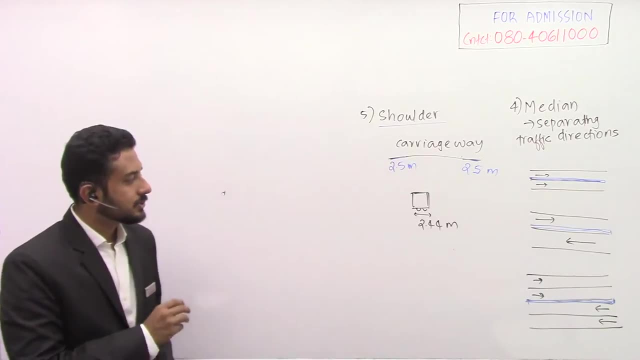 they have got good scores as more students. not only that, if you are getting some good score, you may be getting call for the psus. for psus also, they will be asking some questions: interviewers. interviews will be there, so during the interviews they may be asking such things. 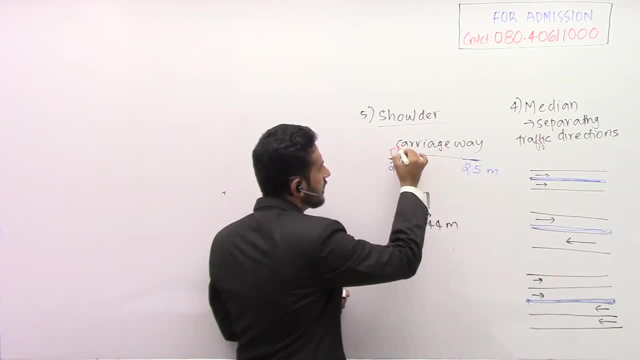 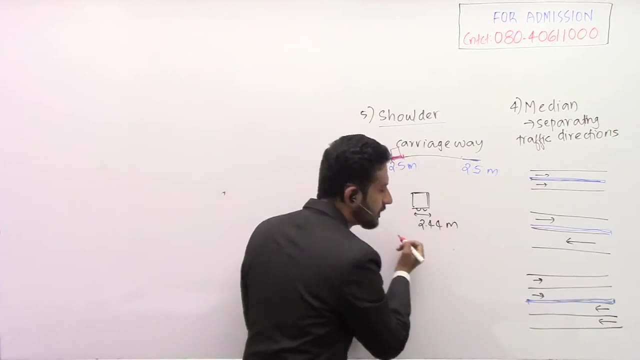 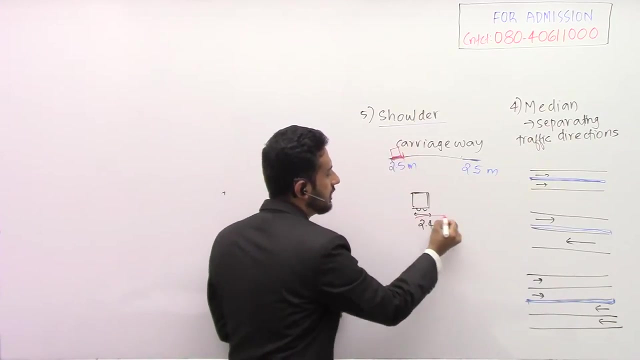 okay. so 2.44 meter is the maximum width of a vehicle as per irc. so a vehicle has to park here so that maybe the maximum width is 2.44 meter. so at least if sir than this, then only we can park it right. so if it is a 2.5 meter, then we can easily park our 2.44. 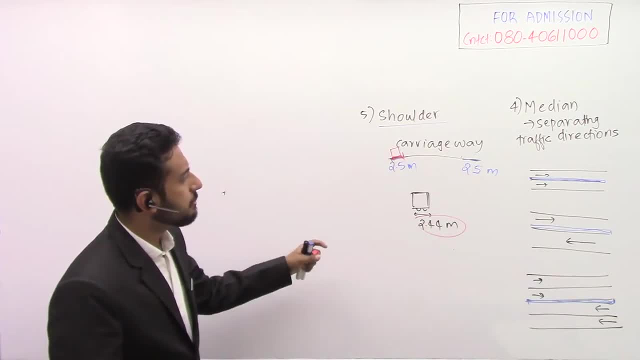 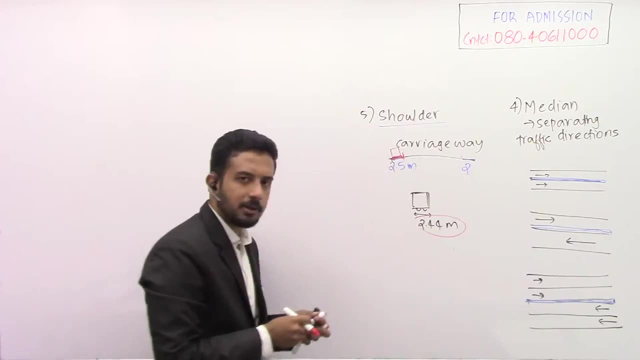 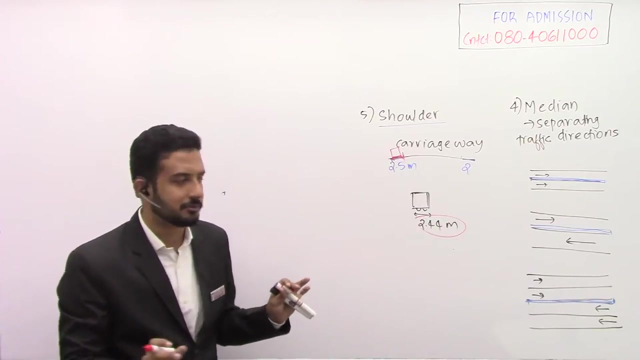 meter with the vehicle. that is a maximum value. suppose we are not having that much, we are giving some two meter only. let it be, we are giving only two meter. what is the problem? suppose some big vehicle has came, some truck or something having very wide. maximum value will be 2.44. so suppose 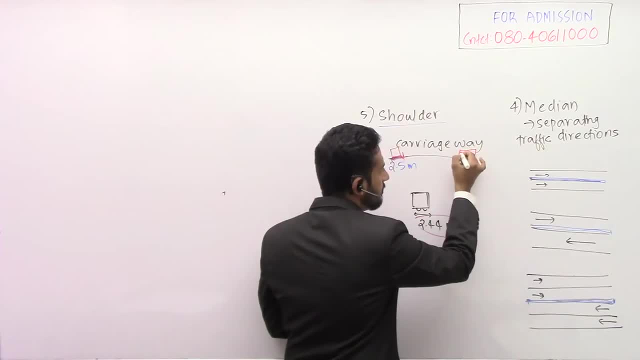 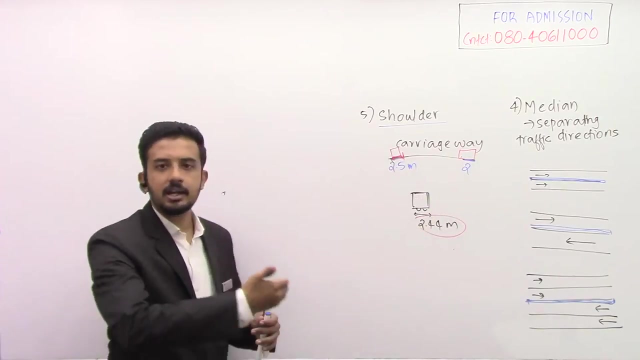 i am giving four, two only. what is the problem? it will be parking something like this. see this thing definitely you might have experienced in your day-to-day life. the shoulder is still here only, but the vehicle width is more than the shoulder width, so that the vehicle will be using. 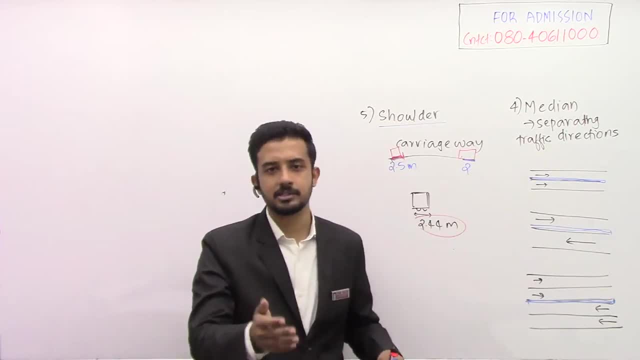 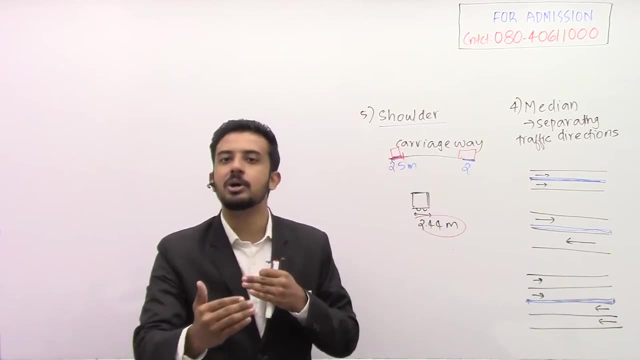 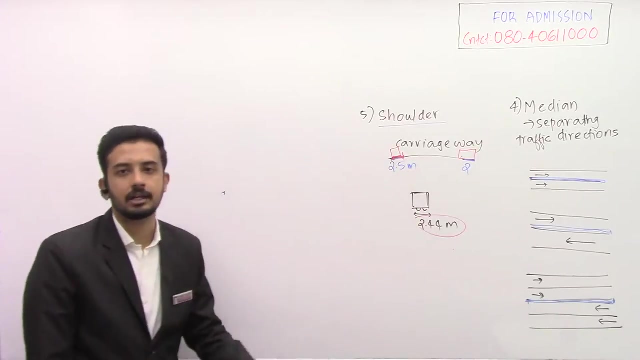 some part of your road. so while you are driving you can see some parked vehicle may be there. so you have to slow down and you have to take the deviation and go. the parked vehicles are going to affect your motor vehicle which are going on the road. that's why irc is telling some minimum 2.5 meter is required. 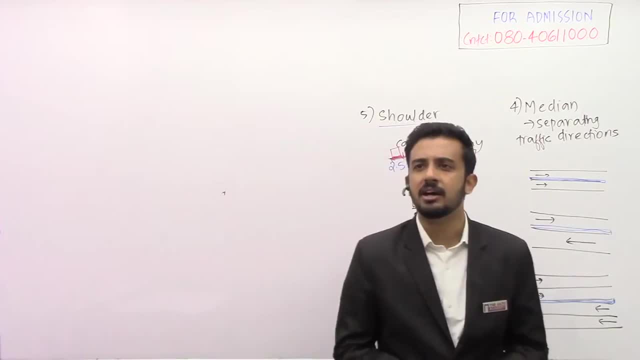 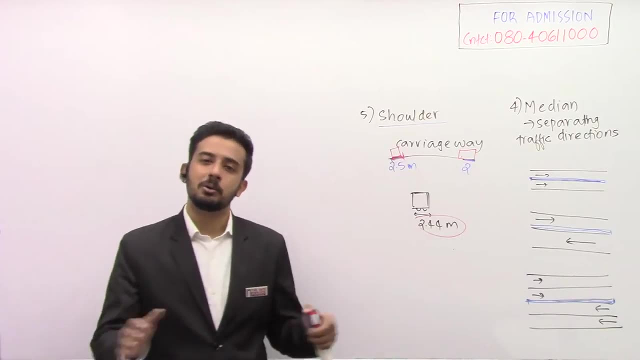 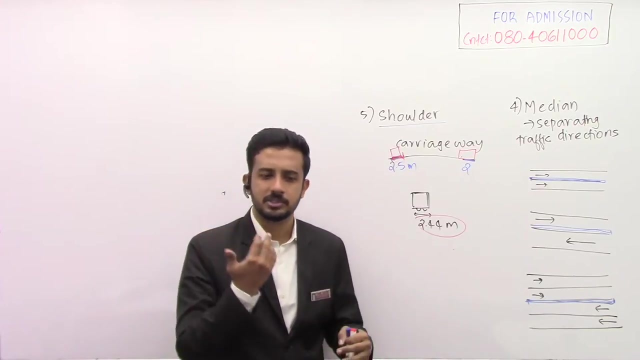 practically may not be possible, because in india everything is congested right. we are not having that much land space. yes, we are having huge land, but the thing is, almost all the land is occupied. we are not having vacant land right so near to the road we'll be having all the shops on the 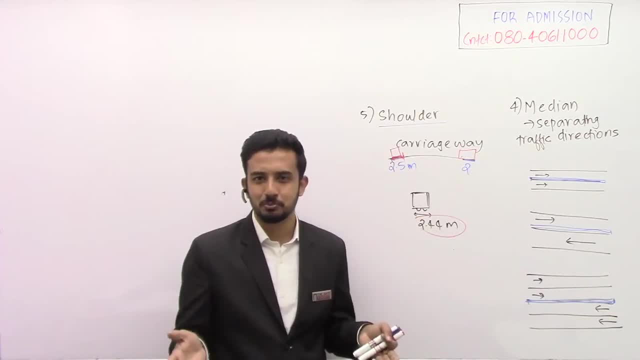 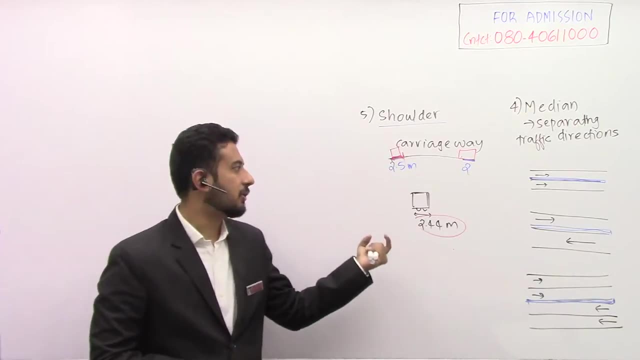 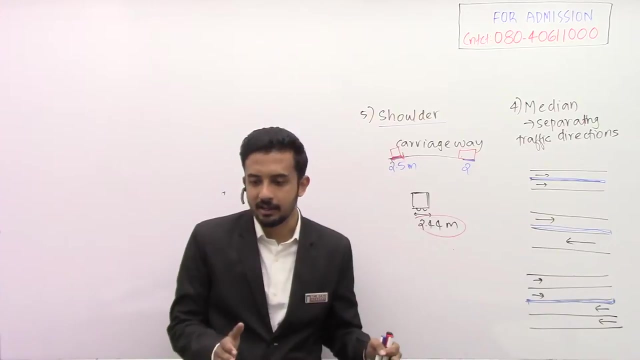 footpath itself. some shops may be there, so we are not having much space. so because of the site constructions, site constraints, practically it may not be able to provide 2.5. that's why we are seeing some parked vehicles, some the the right wheel of the vehicle will be on the road left. 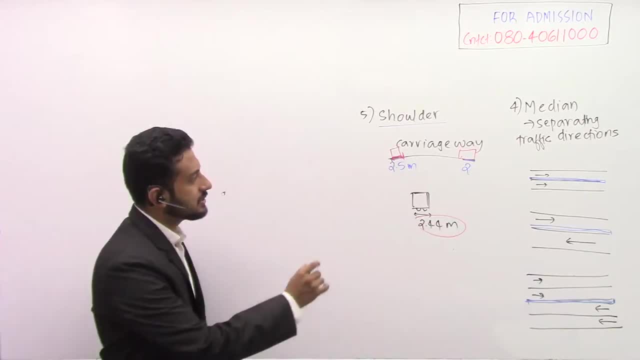 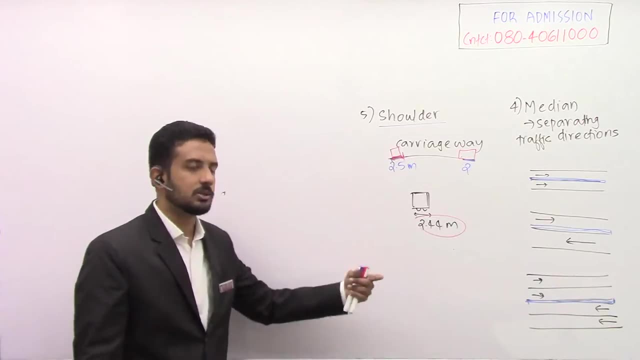 wheel will be on the shoulder like that. okay, so that's why irc is recommending some minimum value of 2.5 meters. so remember that it may help you. these values, everything may help you, not only in grade exam, but also for other interviews, other competitive examinations. 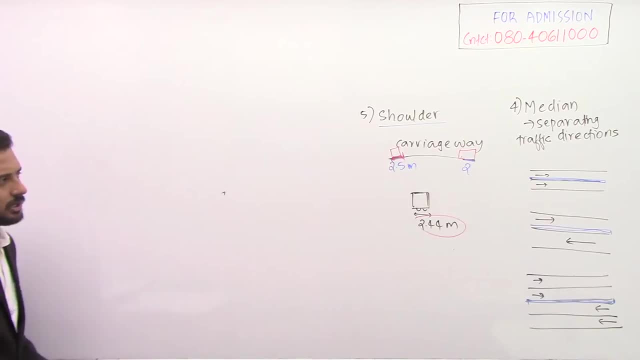 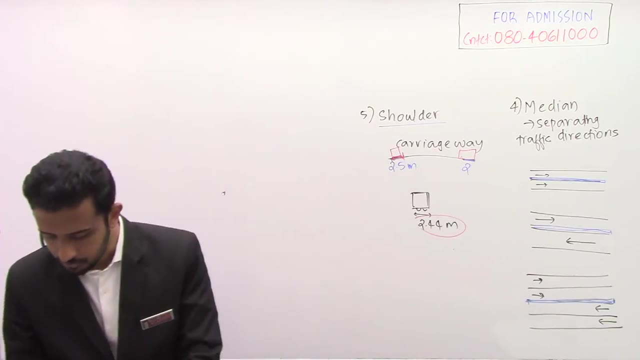 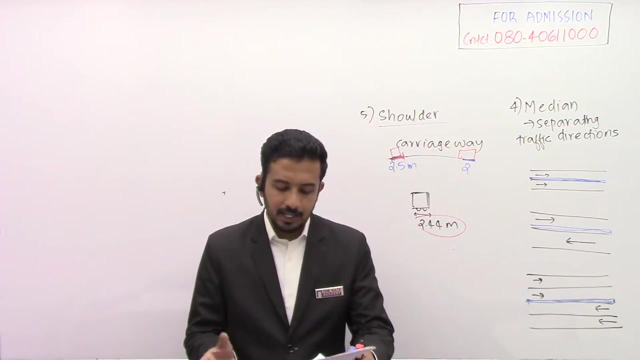 also okay. so that is shoulder. so remember those cross-sectional elements so you can expect a one more question from here. many times they have asked you ask the questions. so yeah, let me. let me simply read some gate questions, theory questions. okay, the value of lateral friction is how much? tell me? 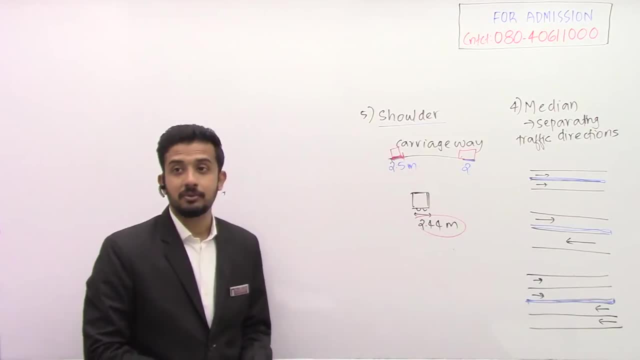 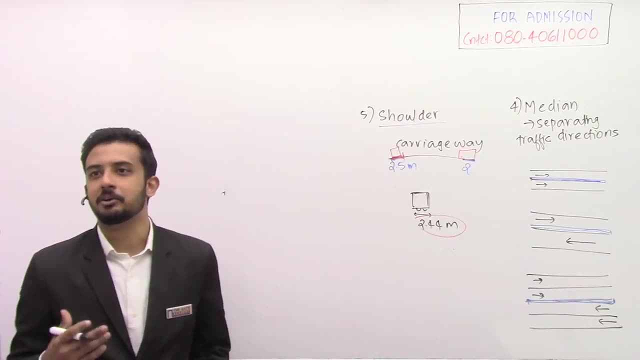 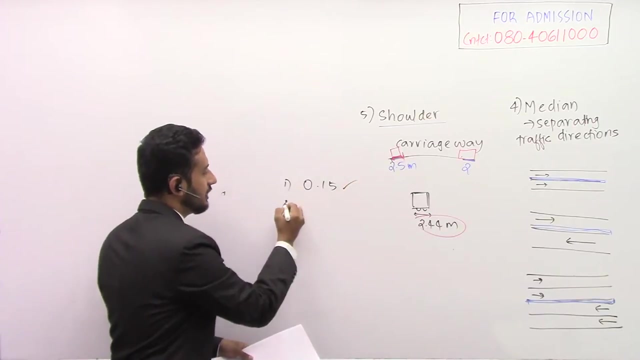 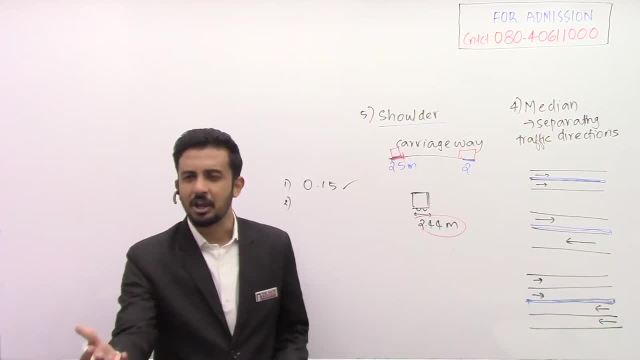 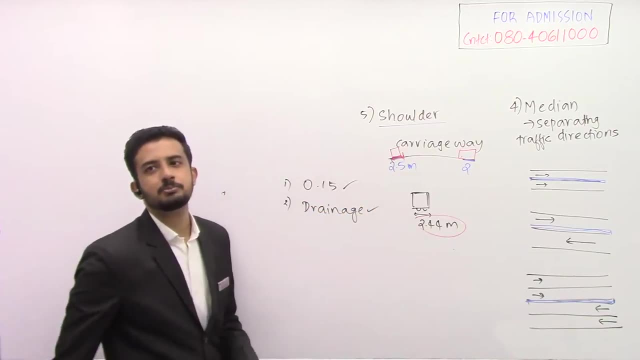 stopping side distance of tracking centrifugal force? you have already given me the reply, right. so why we are giving the drain, why you are giving the camber for drainage purpose, right? so another one more question that is also asked. you ask the question why you are giving the camber for drainage. 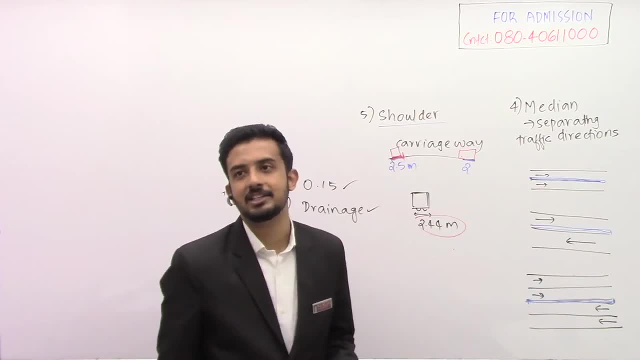 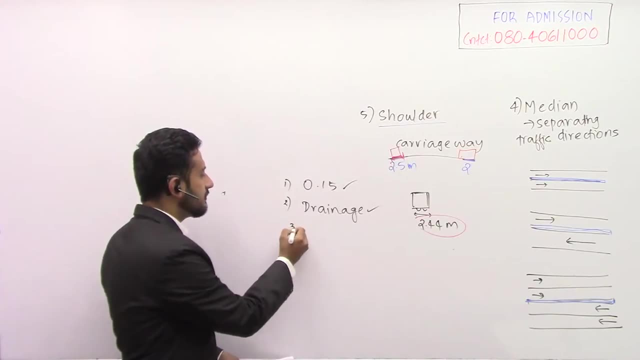 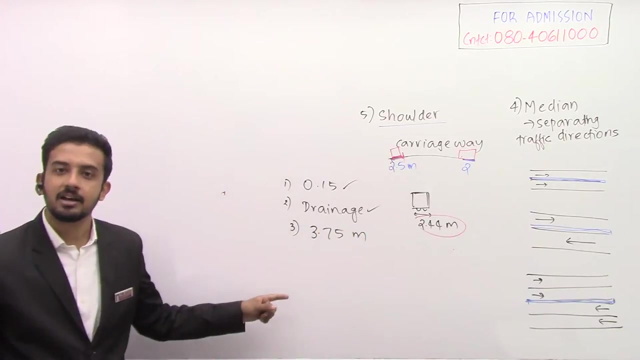 what is the width of a single lane carriageway? yeah, very good drainage. you have already replied while i was taking the class. that's why i didn't ask you again. what is the width of a single lane carriageway? 3.75, very good, this is a single lane. this has already asked for one mark. okay, so always. 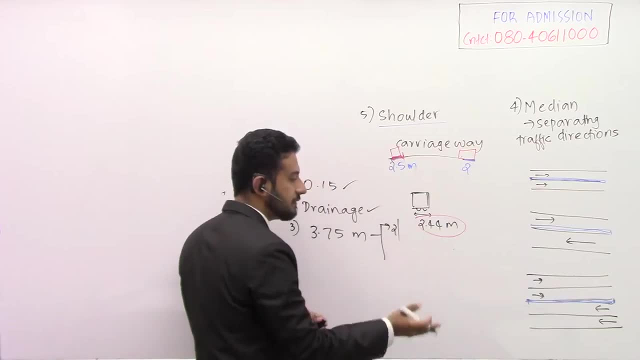 remember the twist. what are the twist for two lane, if it is a raised curve, then it is not seven, it is 7.5. and for n term is there intermediate and intermediate and intermediate? is the intermediate and intermediate for intermediate carriageway 5.5. in all other parameters, whatever be the number of lanes. 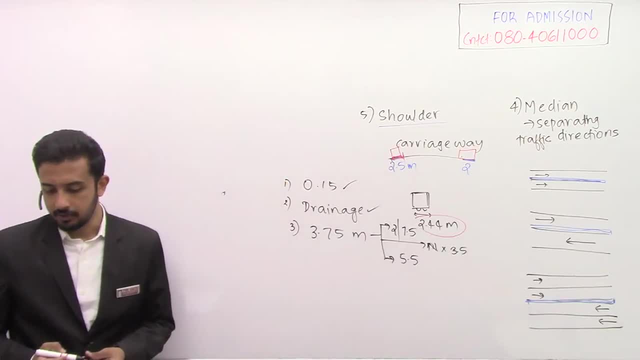 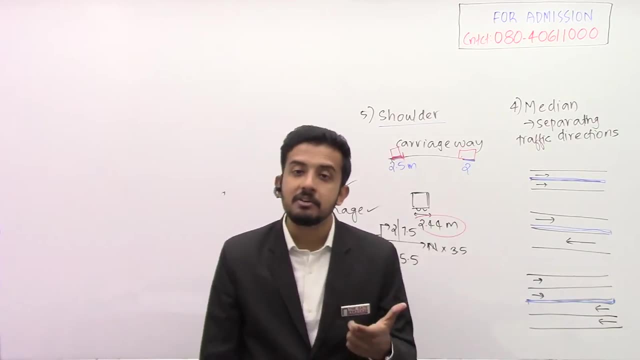 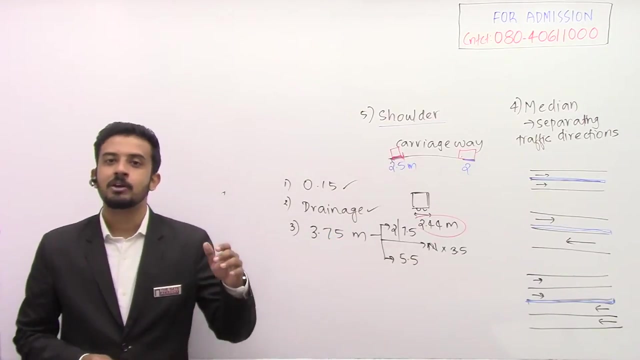 into 3.5. okay, very good. so remember those things. that's it. see that value of camber for cc payment for heavy rainfall area. that is also a previous gate question. see how simply they are going to give you the marks. what is the camber value for cement concrete for heavy rainfall area they have? 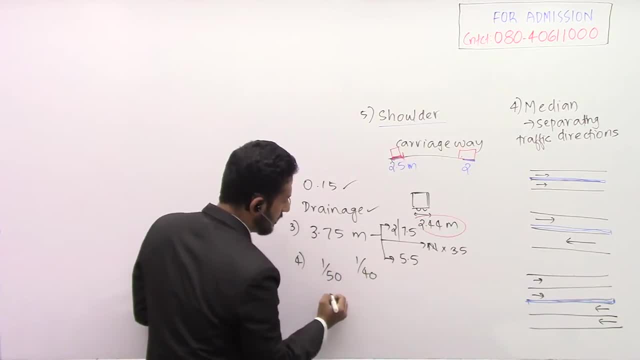 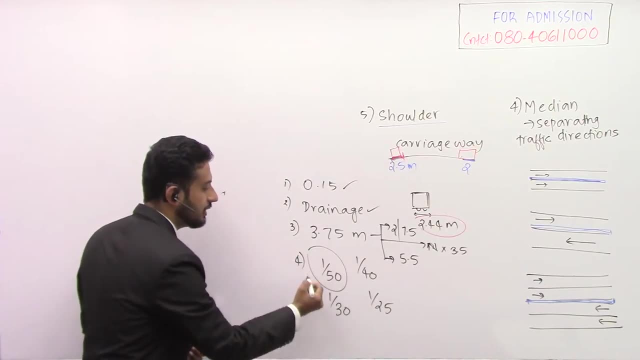 given the options 1 by 50, 1 by 40, 1 by 30, 1 by 25, what is the value for cement, concrete area, cement the concrete? yes, very good, 1 by 50, 50. that's why i told you, better study in one in. 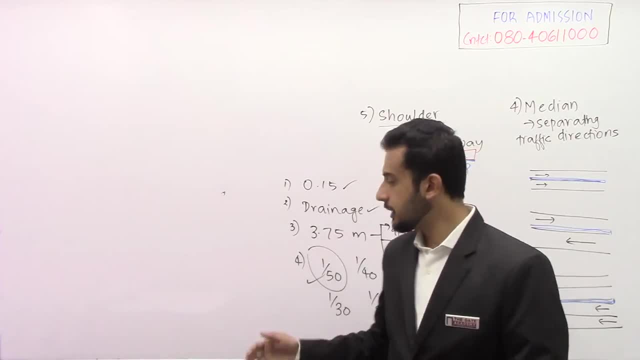 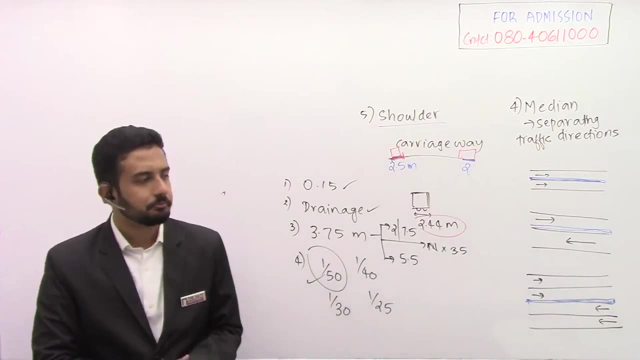 n term, rather than by hurting in percentage. you can by heart this: 1 by 50, like 2.5 percentage, 2 percentage, like that you can remember. 1.8 percentage, okay, 1.25 is there instead of like that you can, you can study. 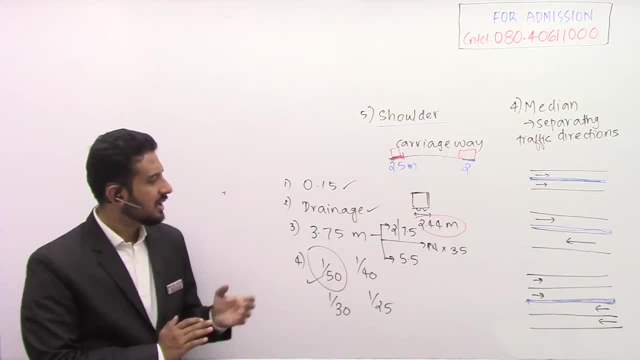 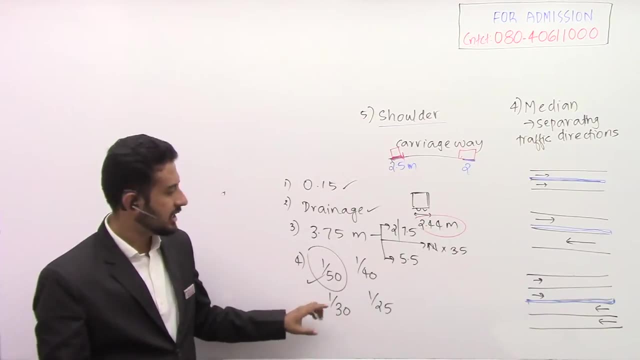 that 1 by 4 mean like that: okay, this much percentage and all. but again, if they are asking such questions, you have to convert like this: if you're studying like this, it's very easy to convert into percentage right: 1 by 50, nothing but 0.02, 2 percentage, that's it okay. and also, if they 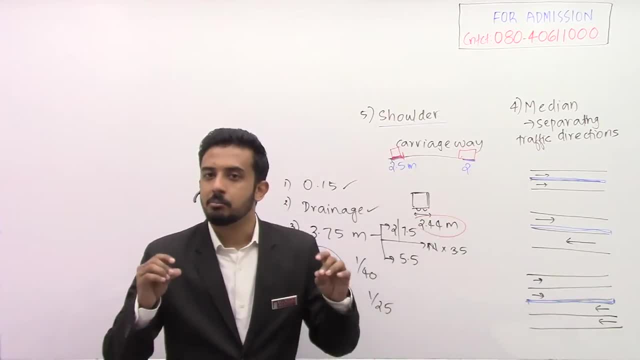 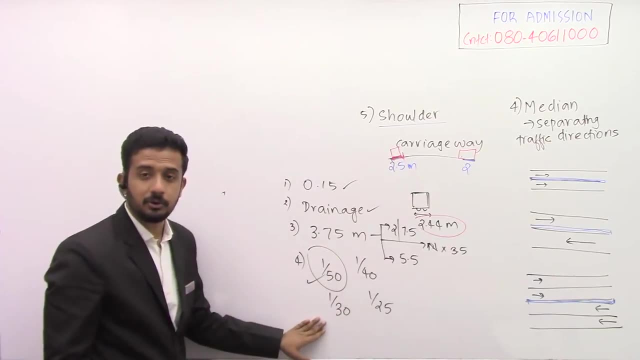 are asking that camber. so far they have not asked that, but anytime they can ask you a question there, because they have already asked a question for w. they have already asked the value for camber. then they are combining it. they have asked for one mark, one mark. if they are combining it, they can ask you. 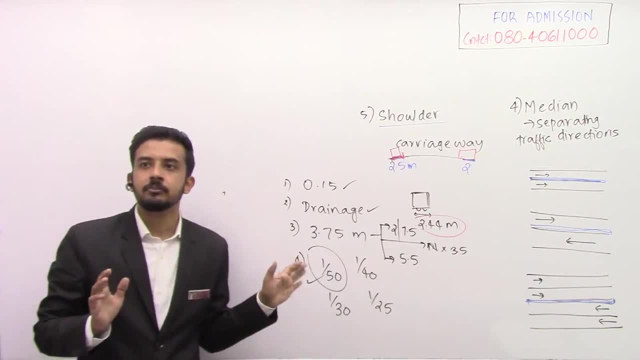 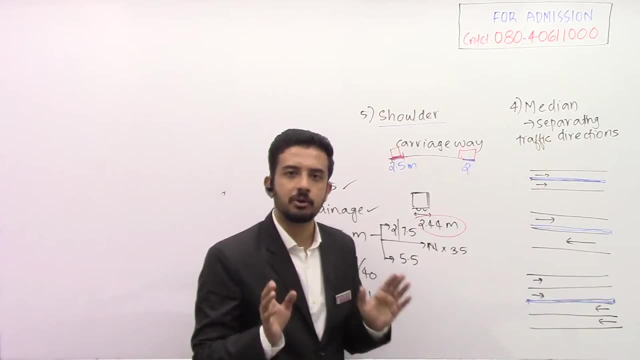 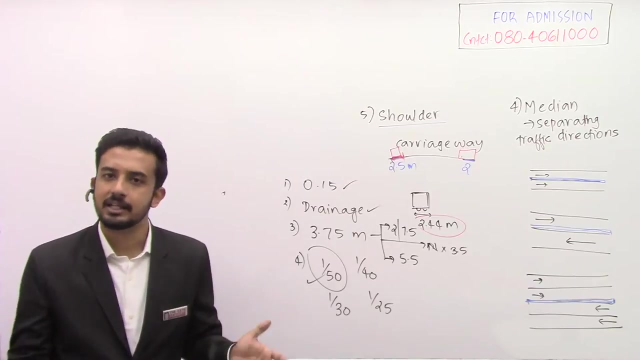 a two marks question that we have already discussed. okay, what is the difference between median and divider? see, divider is nothing but something we are using for dividing. that's it, okay. in general term, median and divider is same. divider we can use for anything. okay, whatever we are, whatever. 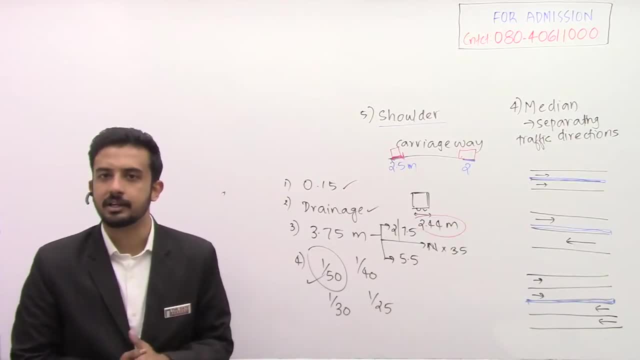 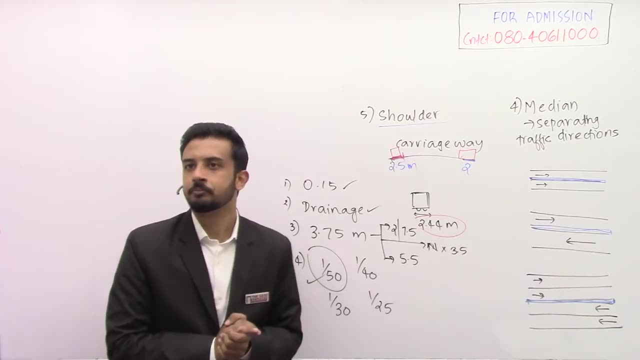 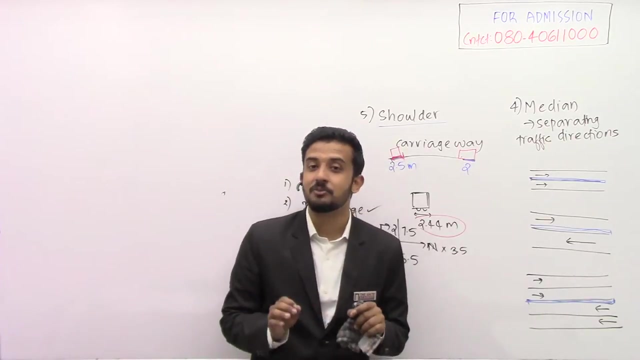 thing you are using for some: deviating the traffic, controlling the traffic, nothing but the divider. so, general sense: divider and median are the same. technically speaking, it is median. okay, so that are the cross-section elements. now we are going to see one of the very, very, very important concepts. 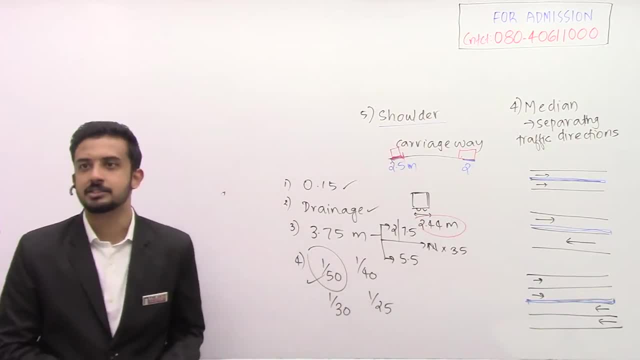 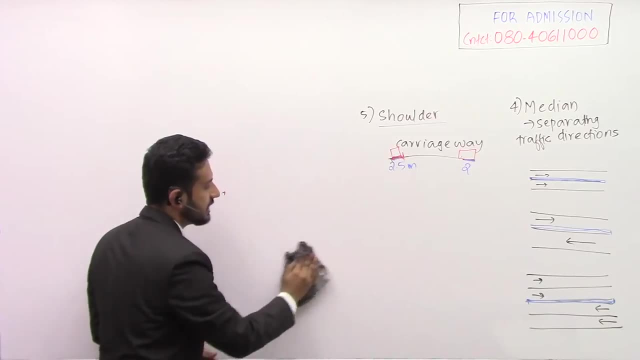 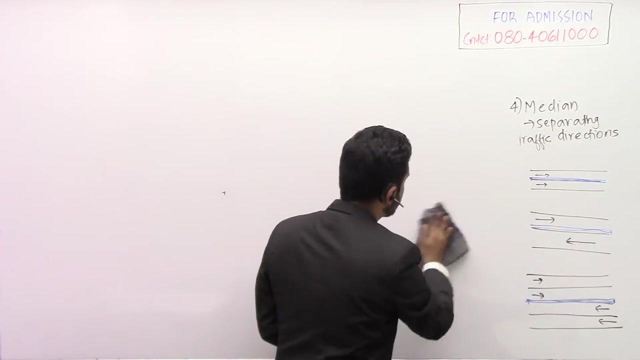 for gate examination. nothing but the sight distance. okay, so i told you we are having two, three types of sight distance. first one is the stopping sight distance. that is the most important sight distance. then comes to the overtaking sight distance. then a small concept is there, called as intermediate sight distance. okay, the numerical portion is there. 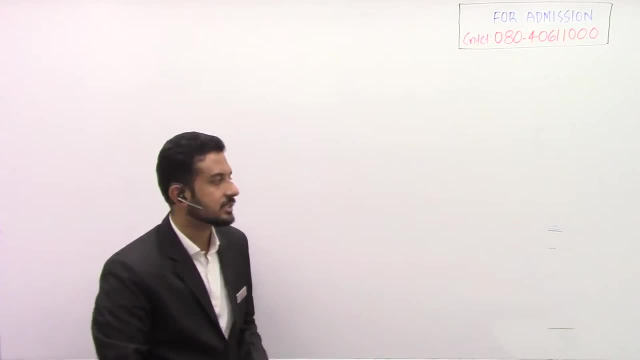 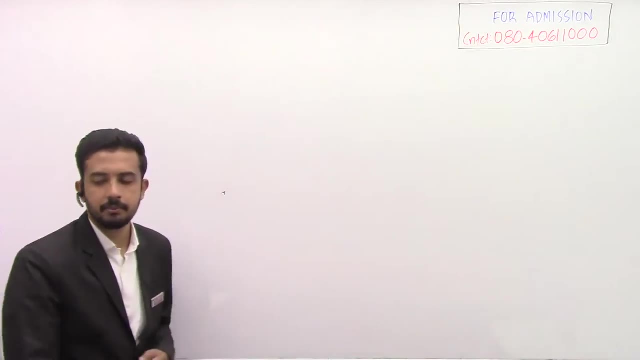 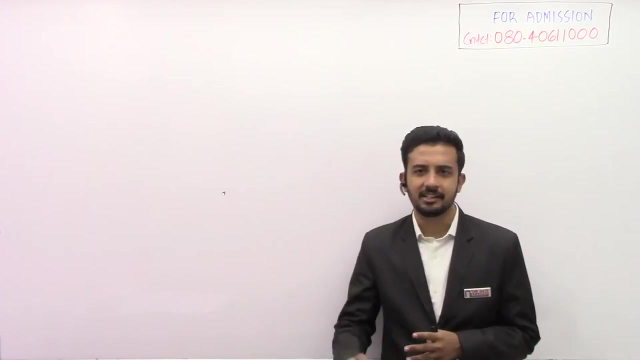 only for stopping sight distance, and the overtaking sight distance and intermediate sight distance is easy. there is no calculations and all one simple theory concept. okay, so what you mean by sight distance? nothing, but no need to study anything extra. whatever we are doing in our day-to-day. 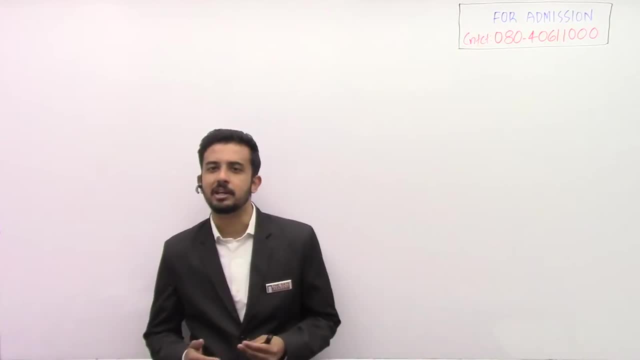 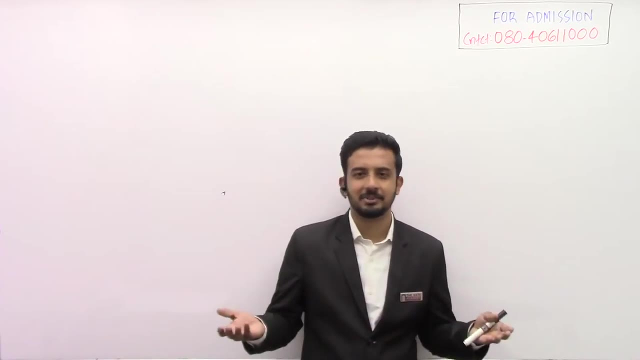 life. you are riding your vehicle, you are riding your bike, you are riding your car. you are riding the vehicle. i hope everyone will be riding the vehicle. either it can be a car, either it can be a bike. whatever it is, or you might have already. uh, no need to tell right, everyone is a road users. 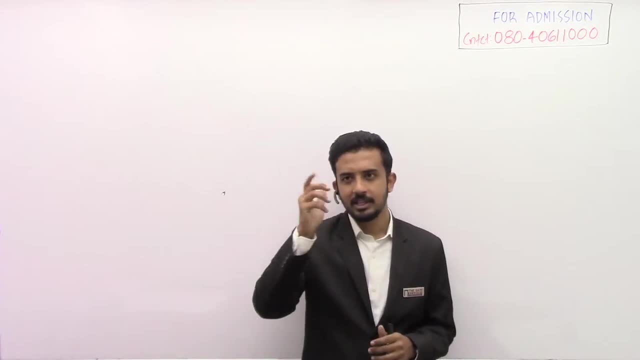 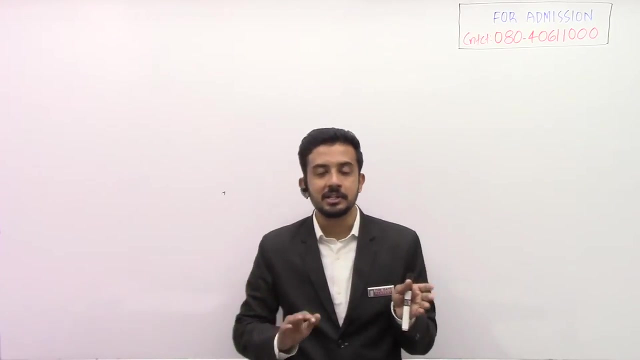 whenever you are riding your vehicle. yes, very good, abhishek. the distance you should see in front of you, the clear distance in front of you, is called a sight distance. okay, why don't listen? lag distance, brake distance- is what? stopping sight distance? actually, we are having different types of sight. 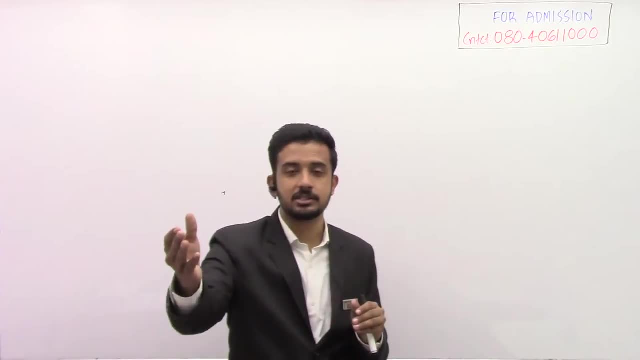 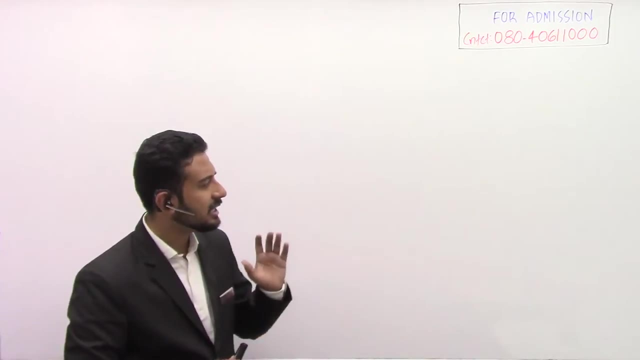 distance. sometimes they can ask you see so for this stopping sight distance. they have already asked you a one more question from the definition of this stopping sight distance. that's what i'm telling. sight distance in the general sense means whatever the clear distance in front of you. that's. 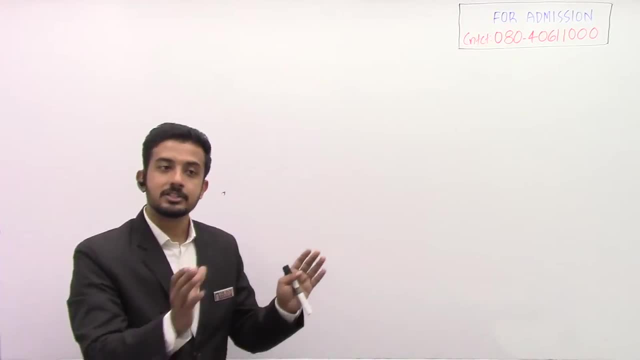 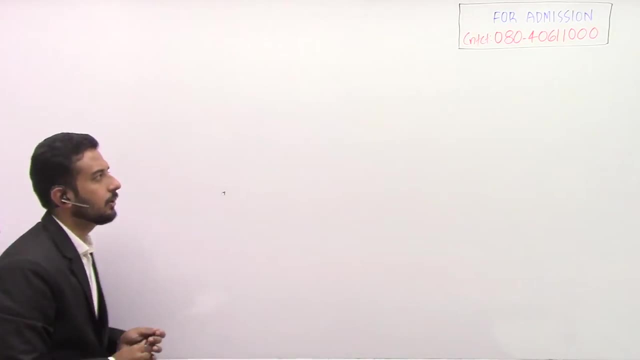 it. if you want to stop the vehicle, that is called stopping sight distance. if you want to overtake, it is called as overtaking sight distance. okay, so we are going to see our first one, this stopping sight distance. so it's a easy concept actually, so you might have already studied in the colleges. 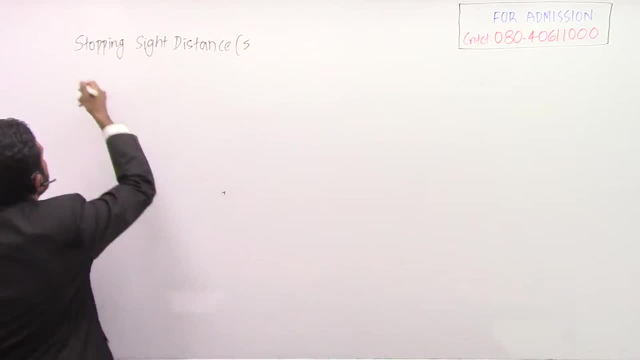 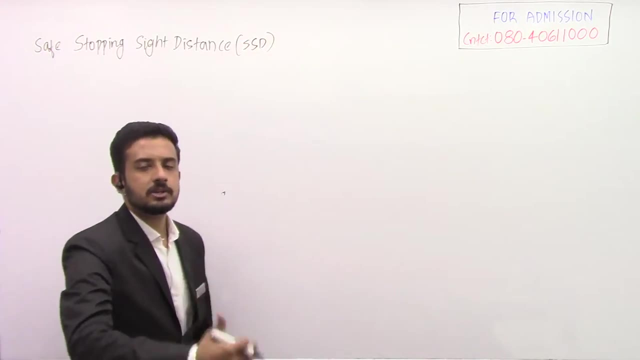 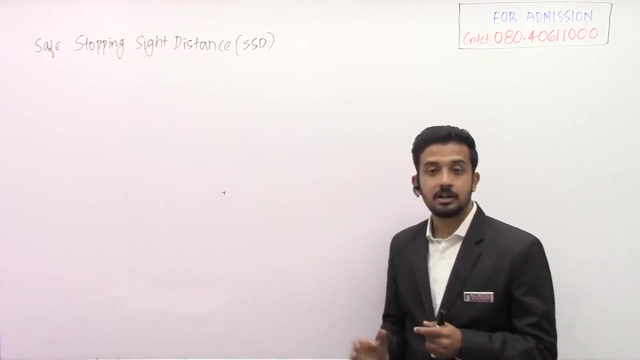 i can tell it as seen. gen actual word is the safe stopping sight distance. okay, but we denote it as ssd only. it is the safe stopping sight distance, so what, it is no need to elaborate a lot. you might have already studied these things. we'll concentrate on numerical problems. okay, that will be better for. 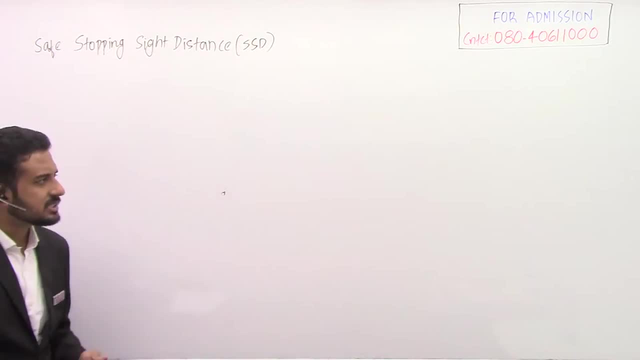 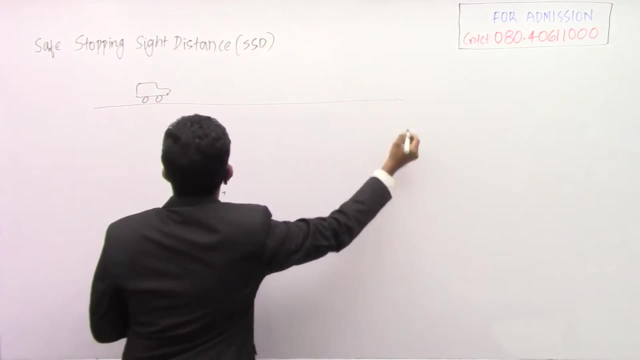 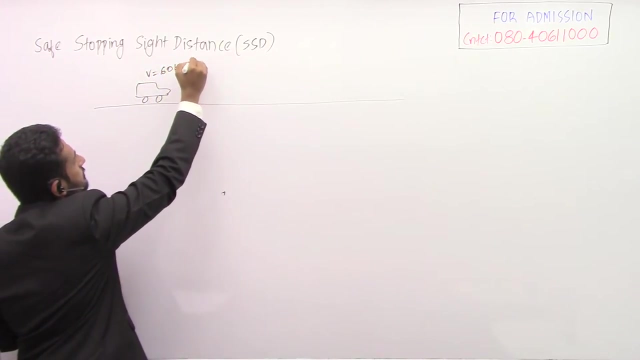 you as you are writing the exams. so what is that? everyone knows. suppose your vehicle. you are riding your vehicle. so again, our car is there, our previous car, we have drawn, so suppose that let it be some 60 k mbs, you are riding your vehicle. okay, so you're riding your vehicle at 60 kmb, as you are. 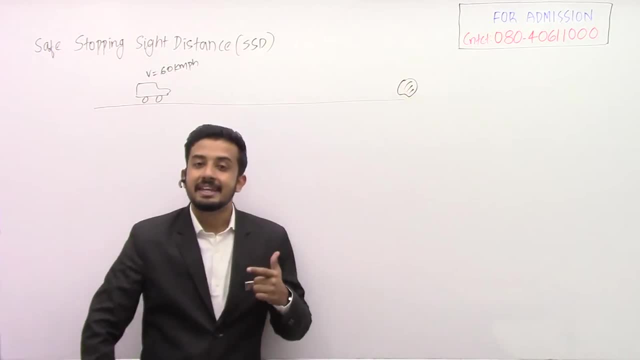 seeing something here. what is that something? it is nothing but an obstruction which can affect you, which can make an accident. so our next example is: you are taking a car and there's a kind of an off-stecker touching something. right, because you are driving the car and you are driving at 60 kmph, you are 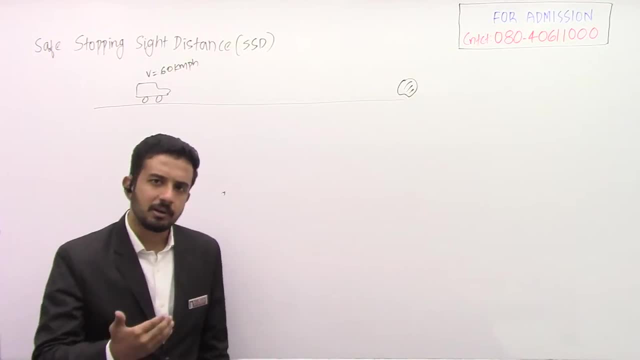 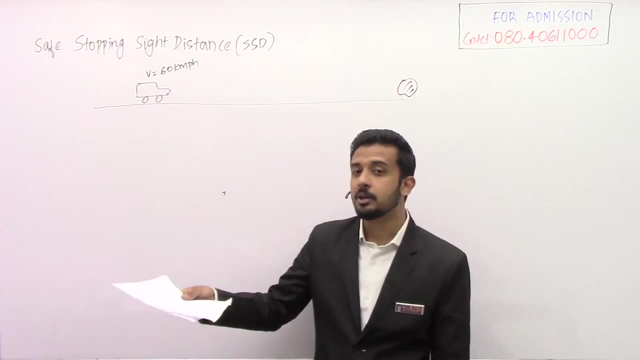 accident? see, whatever you are seeing, will you apply the brake? no, suppose this paper is there on the road? will you apply your brake? definitely not, why. why you are not applying the brake if this paper is there on the road? because you know that this paper is not going to affect you. 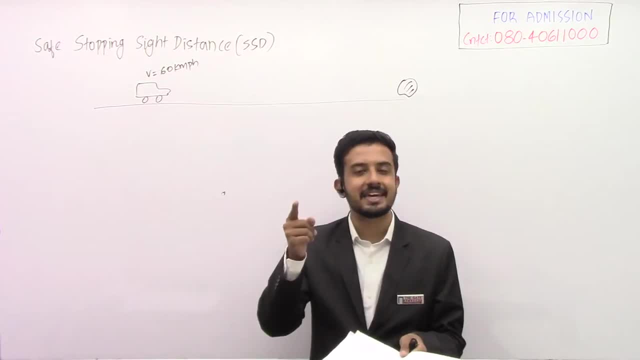 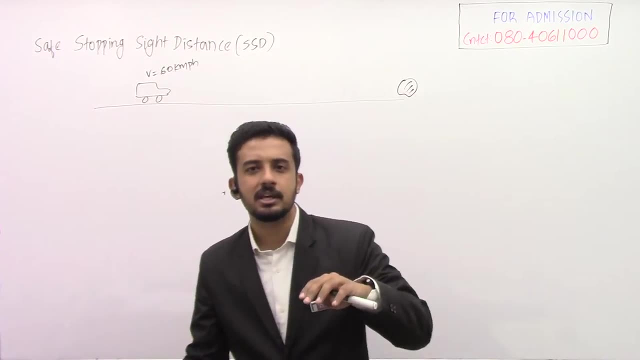 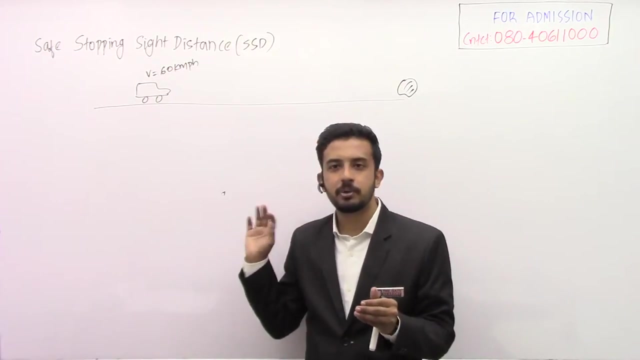 how you know that? because your brain is having the knowledge of the knowledge that this paper is not going to affect. you see, some small babies. they may touch fire and all know why? because they don't know it is going to burn. their brain don't know once they experience that their brain knows. 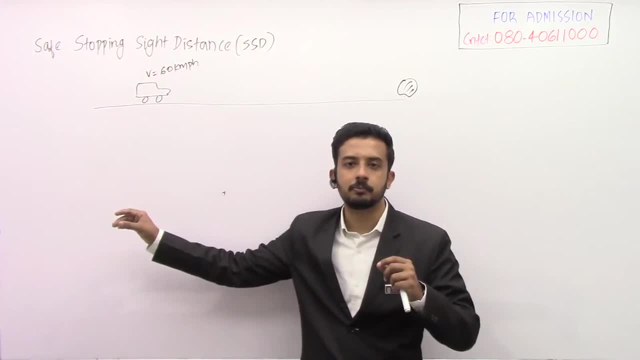 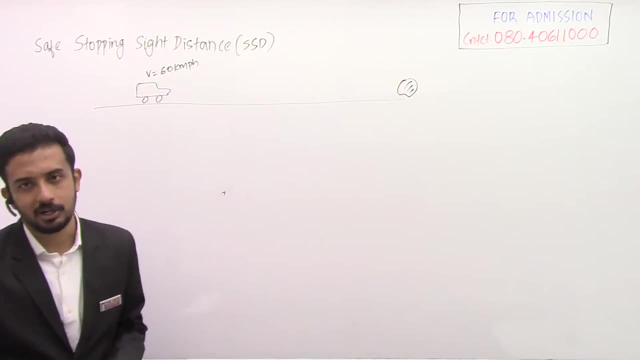 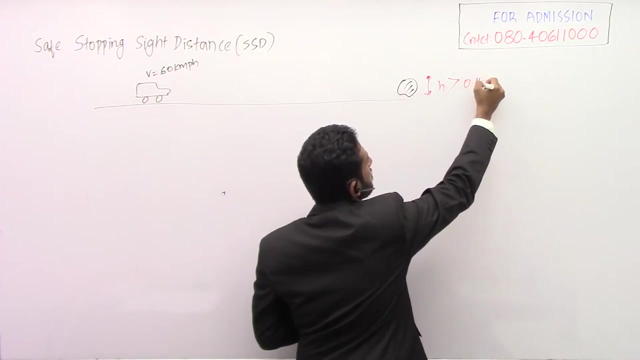 that. okay, next time, if i'm touching, it is going to affect me. so your brain already knows that which all particles are going to affect you and which all things are not going to affect you. irc says that if the height of this object, if it is more than 0.15 meter, 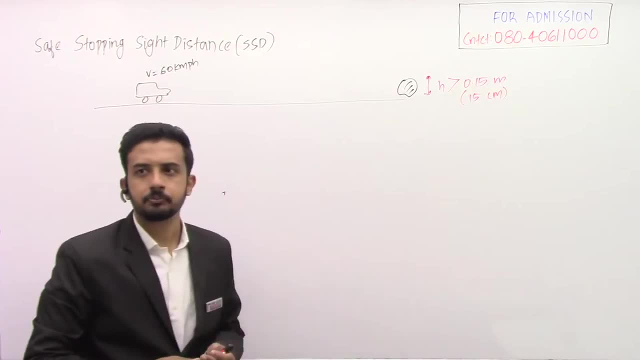 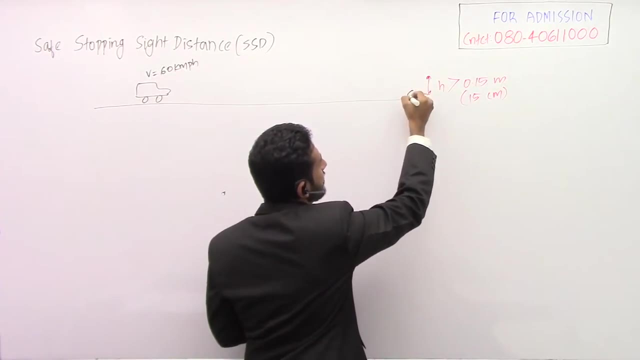 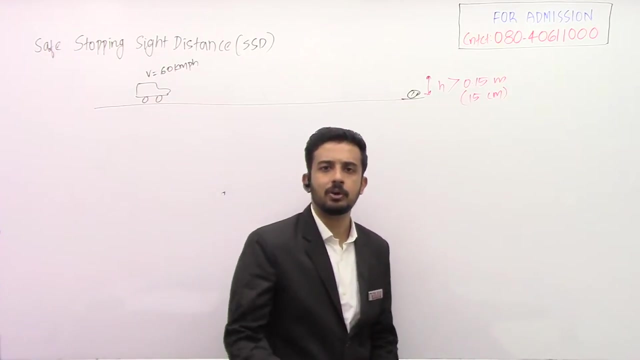 or i can tell it as 15 centimeter, then it is going to affect. you see, the height will not be that much compared to this car. i was simply drawing. something is here, okay, so if the height of the object is more than 15 centimeter, how to remember that value? 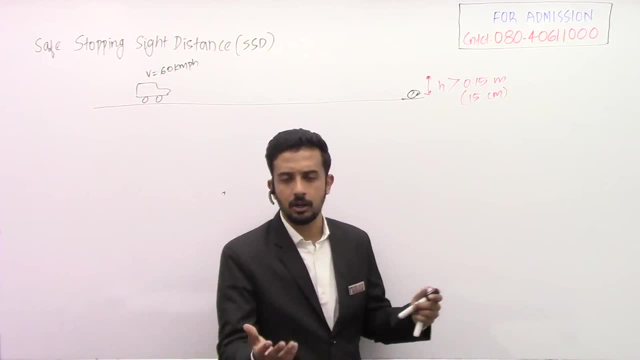 height of a scale, that small scale, 15 centimeter. now, you'll not forget that. okay, so if it is more than that, then only that object is going to affect you. right, say uh, on the road generally you can see the light reflectors. right, some reflectors may be there they are using for 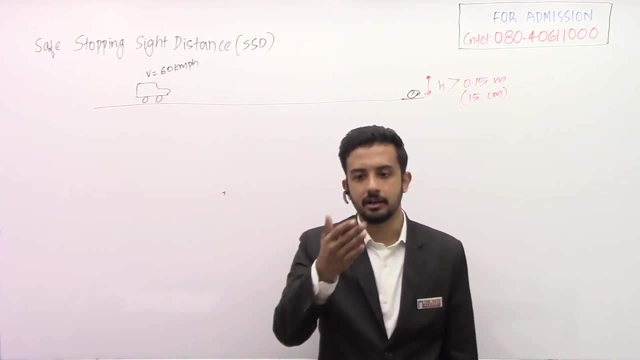 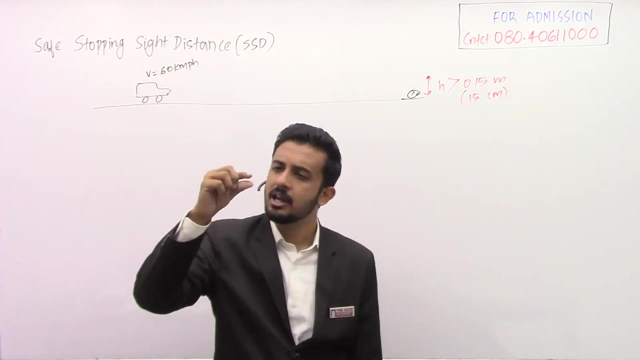 line separation and all okay. see that also a divider right, but it is not a median. something which we are using to divide is called as divider. some right reflectors may be there, having some two centimeter, three centimeters height. that is not going to affect you used to ride the vehicle on. 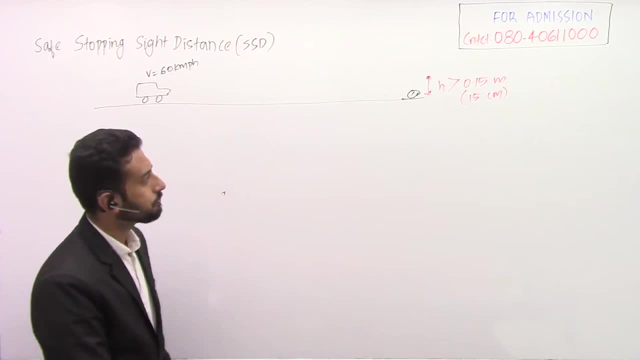 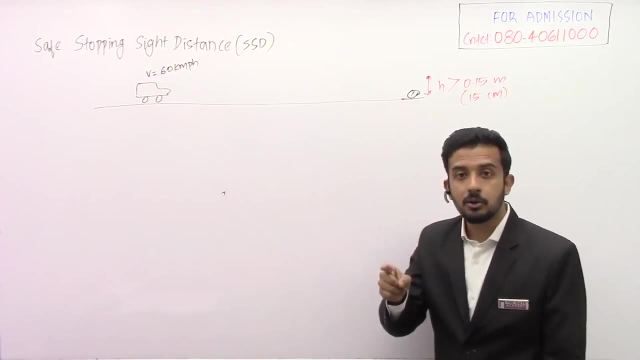 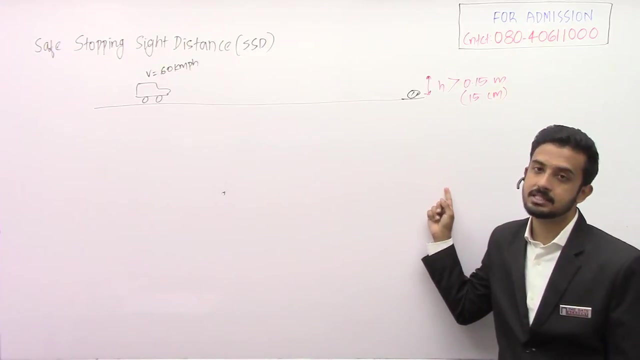 that which is having less than that 15 centimeter. okay, suppose you are having a 15 centimeter object, or more than that. so your brain already knows that it is going to affect you. bro you are going to commit with, you are going to meet an accident, so what you have to do, the brain will tell you. 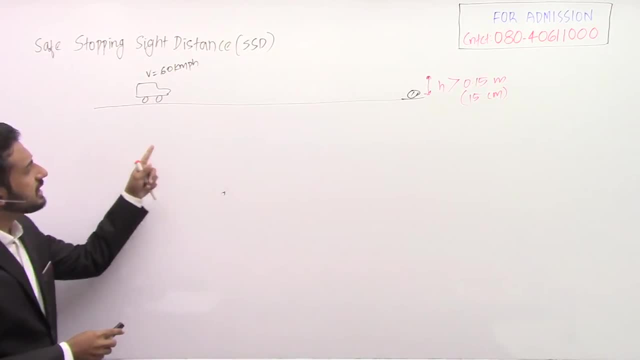 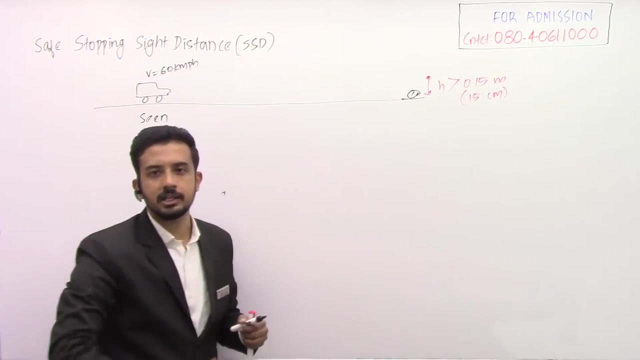 apply the brake right. so you are seeing the obstruction there. let's see what all things actually happening. you are seeing the object. you are seeing the object at the moment. you are seeing the object. your brain will take some few seconds to realize that what it is see. suddenly you see something. you may take some one or two seconds to. 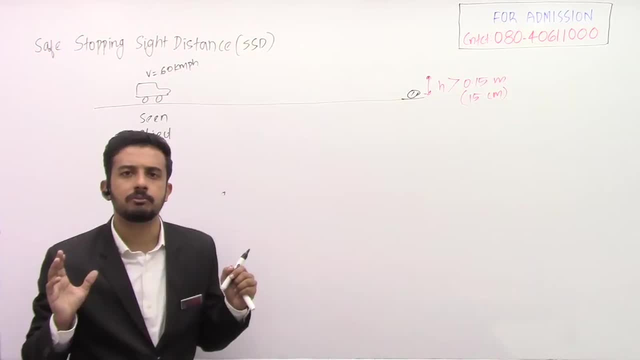 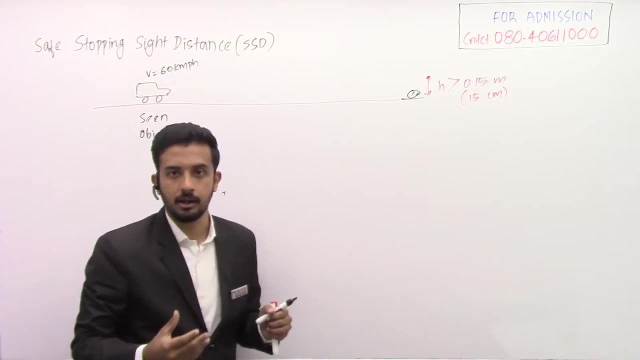 realize that, okay, it's a paper. if it is a paper, it is not going to affect me. i don't have to stop, you have to make a decision. no, suppose that is a see. that can be a breakdown vehicle. right, a breakdown vehicle is there sometimes. so if it is a breakdown vehicle, your brain will make a decision. 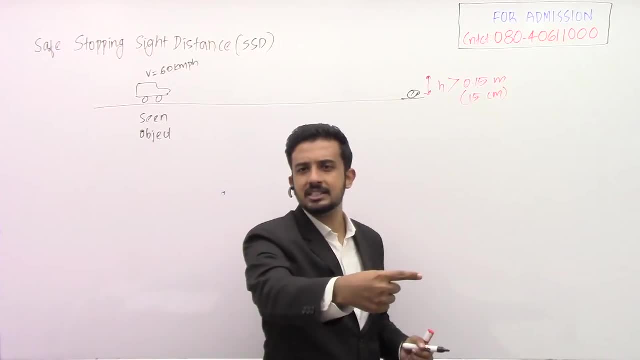 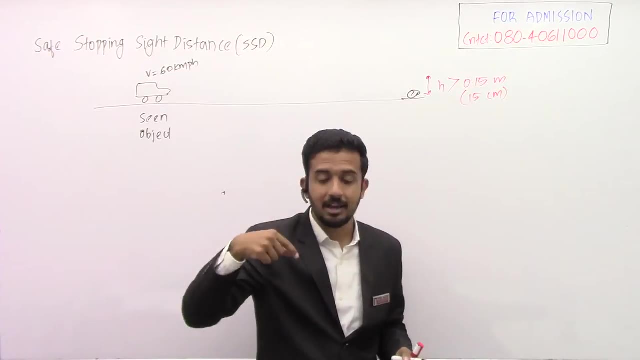 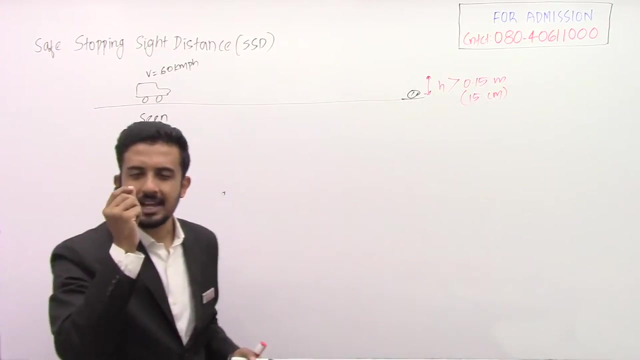 okay, that is a breakdown vehicle. if this guy is going at the same speed of 60, definitely he's going to meet with an accident. so i have to tell this guy to stop the vehicle. the brain will tell you: stop the vehicle. then you are going to apply the brake for that make decision making by the 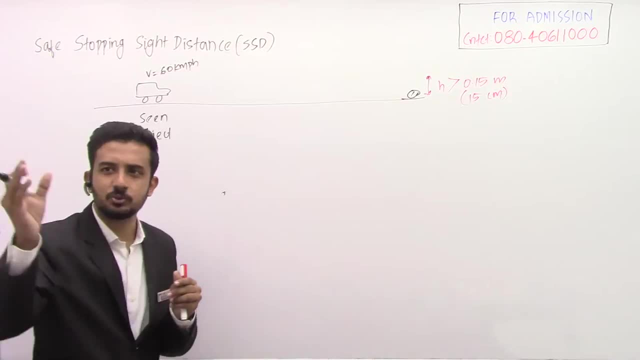 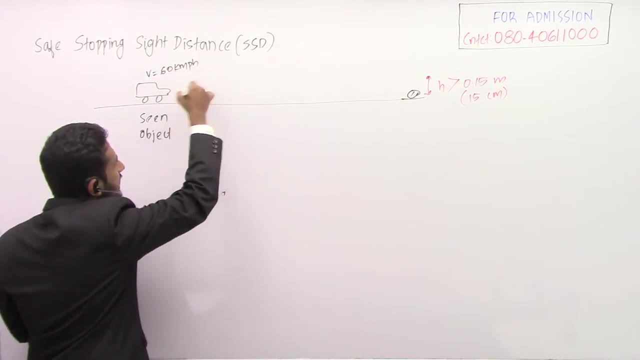 brain. your brain will be taking a few seconds- very good- of shake, as per piev theory. so your brain is taking some few seconds. in that few seconds, your vehicle is moving at the constant speed. so suppose you have reached somewhere here, the same vehicle, okay. so here also, your speed is 60 kmph only. 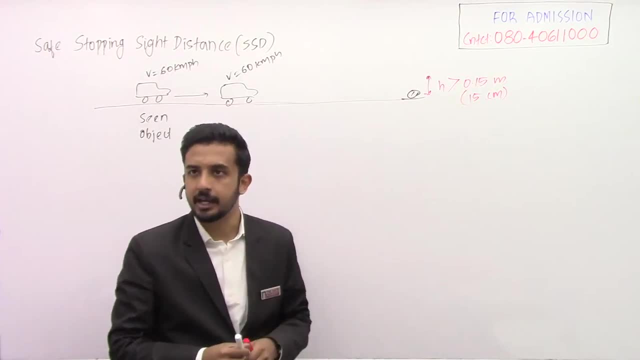 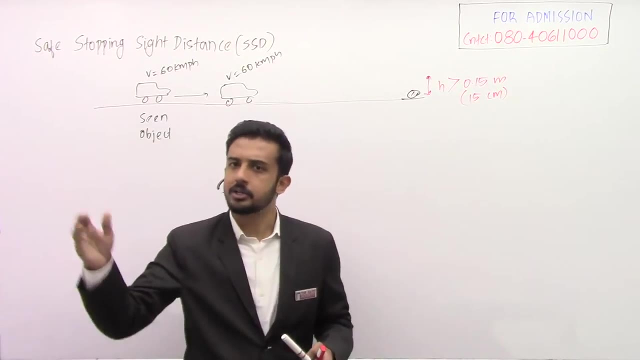 right, because in that time your brain is taking some time. i mean, your brain is taking some time to make the decision whether you have to stop your vehicle or no need to stop, you can continue. your brain is taking some time, right. so at this moment your brain has already. 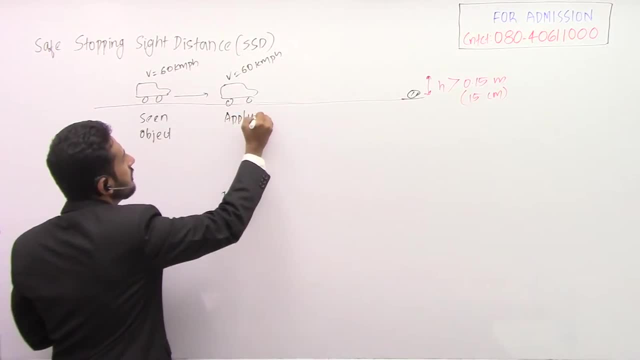 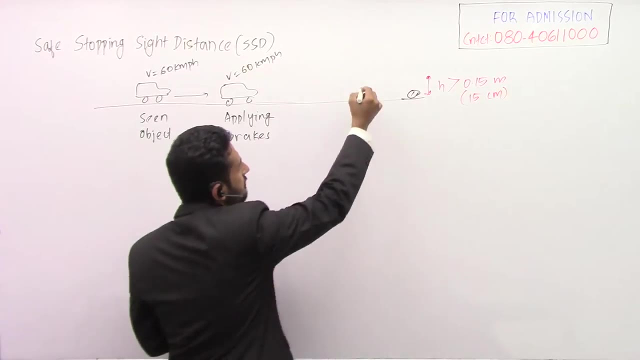 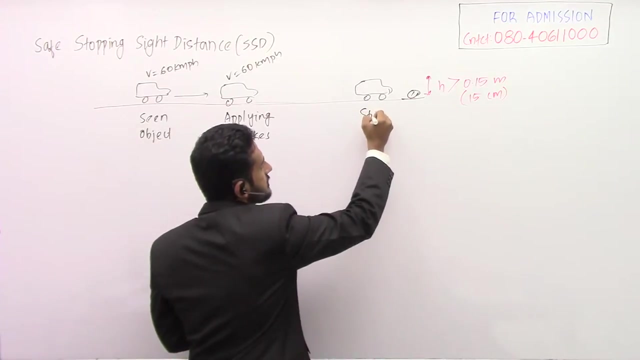 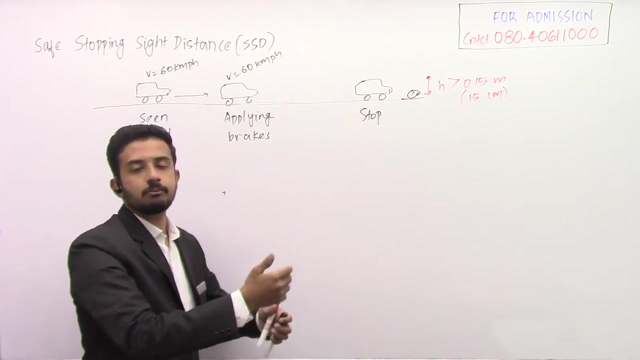 made the decision, what you are going to do now. here we are going to apply the brakes. right here we are applying the brakes. finally, we are going to stop somewhere here so that our vehicle is safe. so we have stopped here. now our vehicle is stopped against some collision with 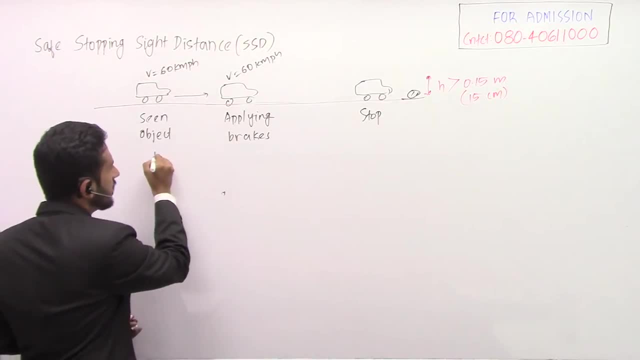 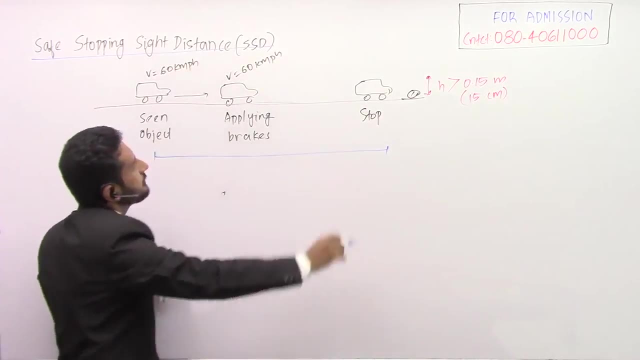 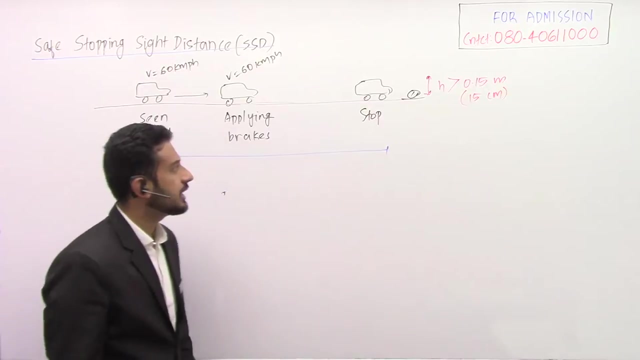 the object. so this distance from this location to this location i can call it as safe stopping site. we denote it as ssd only, stopping sight distance, but the actual word is safe stopping site distance. so i can divide into two parts. see, i hope you know that. uh, prisoners of fire theory. 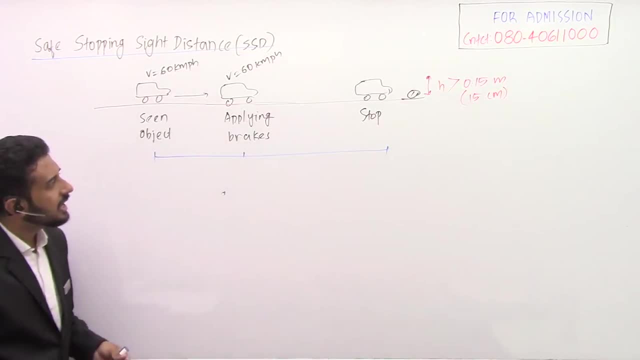 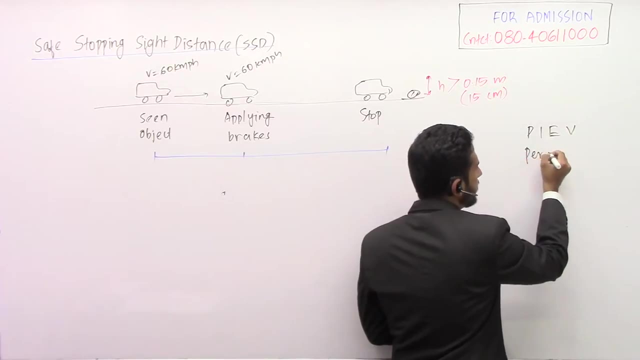 okay, i'm not elaborating that p-i-e-v theory as per irc. p-i-e-v theory: p stands for some perception, nothing but uh, whenever you are seeing something, the signal will be passed to you. whenever the signal will be passed to you, that means the i'm not doing. safe stop and side distance. 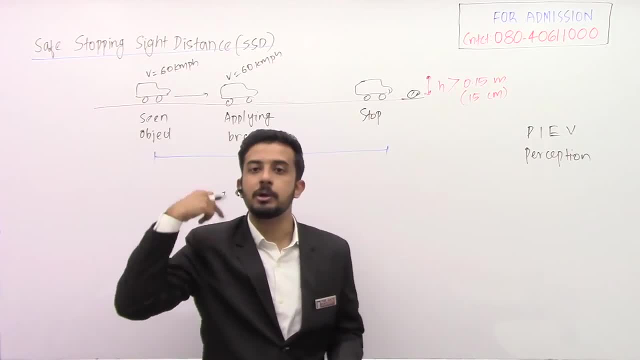 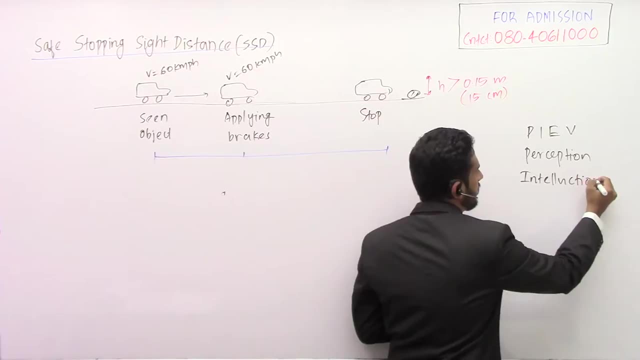 oramos, pastor of radar warning. so we evidently catching your screen. it is safe. your brain- sorry, the signal will be passed. your brain, nothing but perception, intellection. what you mean by intellection? it is nothing. but i told you the baby doesn't know that if it is touching, 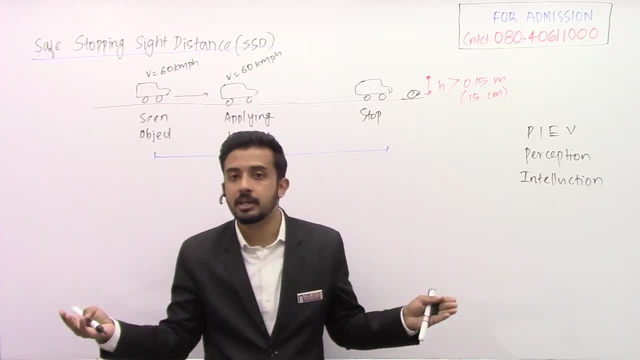 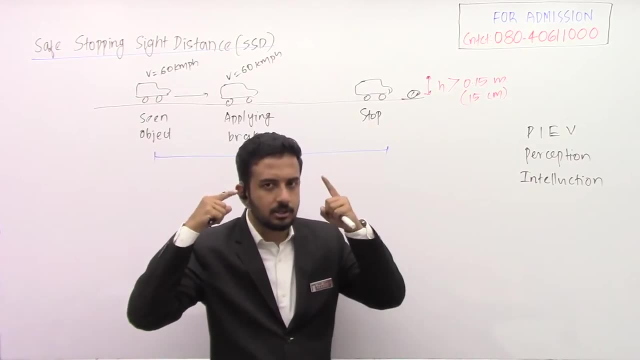 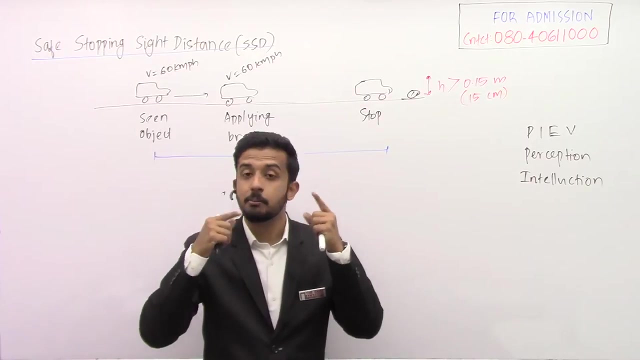 the fire, it will get burned. why? because he is not having any previous experience. his brain, no, don't know that. intellection means from the previous data, from the previous knowledge. whatever you have gained in this 20, 22 years, your brain is going to correlate with the previous experience. 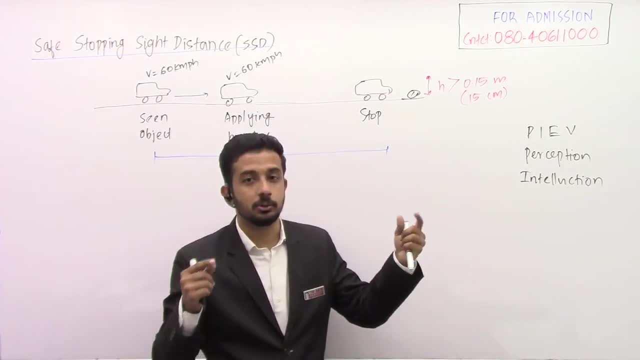 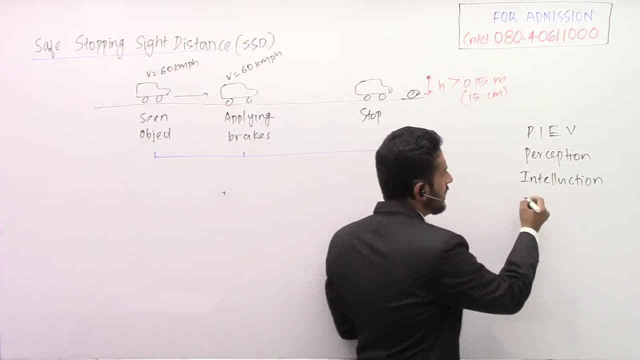 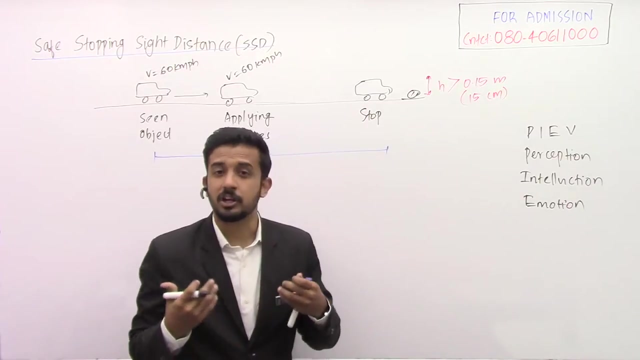 if you're seeing something there, okay, it is going to affect you. it is going to make some decision. nothing but intellection, the comparison of things, emotion. what you mean by emotion, it is not that emotion. it's like you may get feared. if you're a fresh driver, you may be. 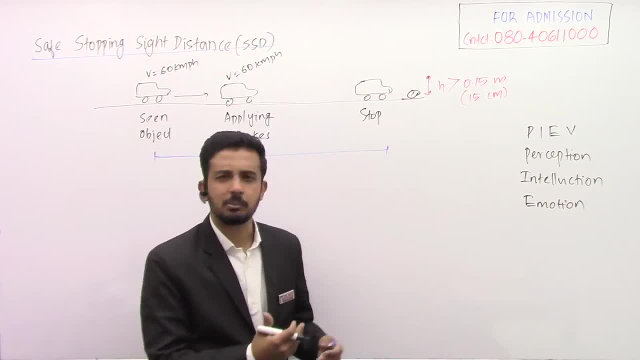 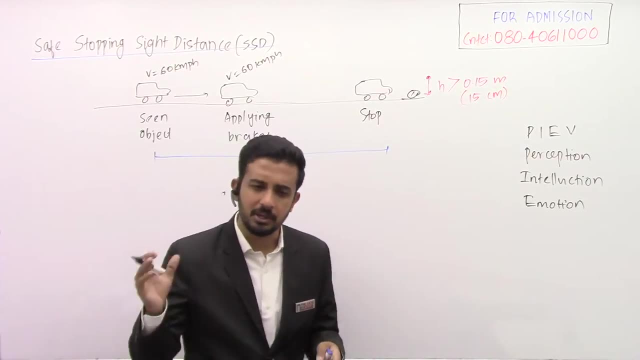 getting shivered and all right. if you're an experienced driver you may be easy with that. you may be experienced a lot of things with that right. so that is nothing but the emotion. maybe you're riding your vehicle having some tension. yes, definitely you may be taking some time to apply the brake, going to affect your time for reaction. making v is nothing. 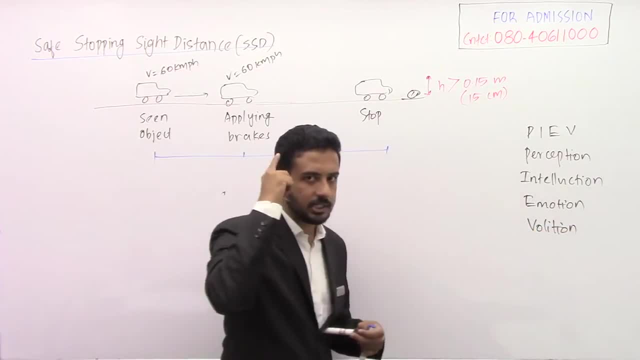 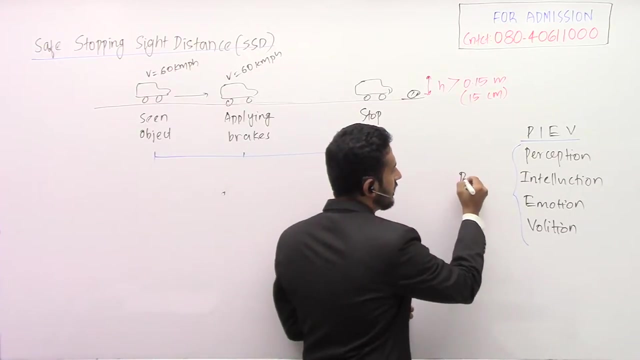 but the volition, nothing. but finally, after making the decision, the brain will tell you: better apply the brake. so you have to apply the brake. that is nothing but p, i, e, v, theory. okay, so for all these things we need some time. that time is called as reaction time. 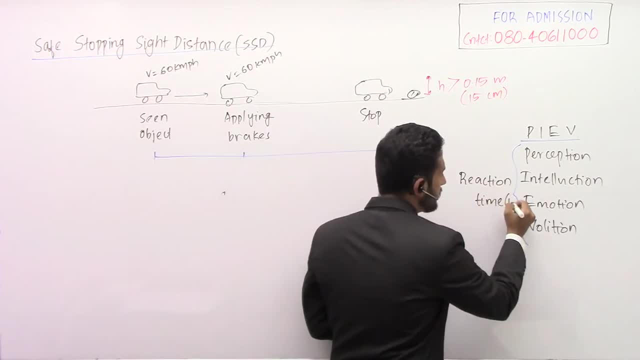 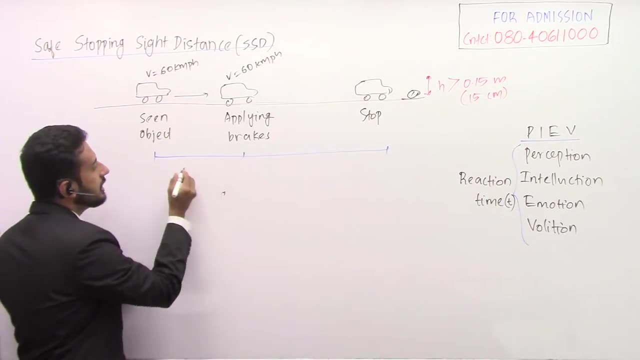 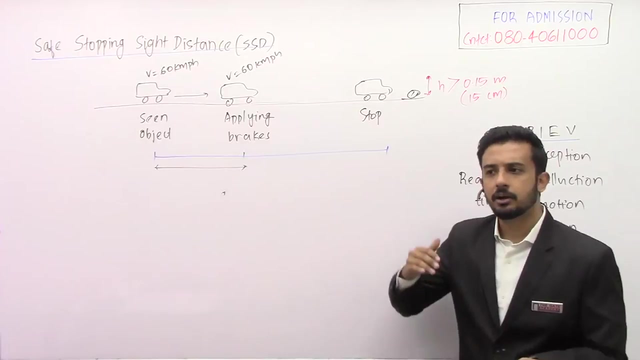 very, very important. generally we represent using small letter t. so what is actually happening in this first part from here to here? the vehicle is moving during the reaction time, so in that reaction time actually we are not applying the brake right, we are simply lagging our brain is. 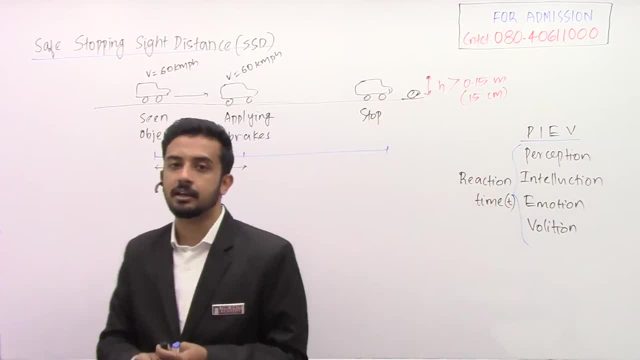 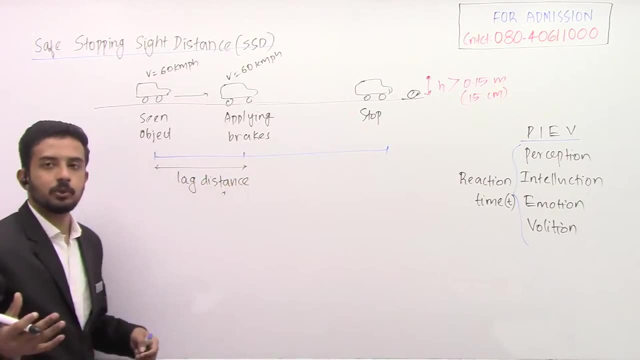 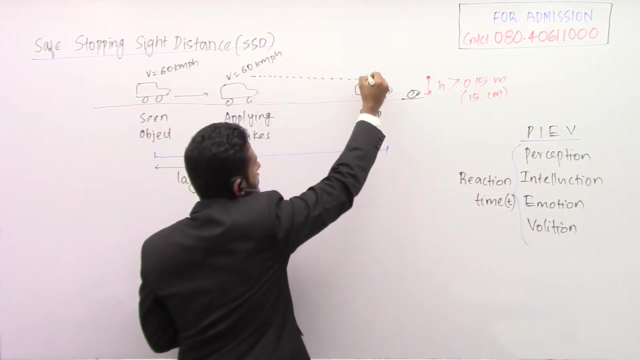 taking some time to make the decision. we're simply lagging, so that that distance is called as lag distance. someone have already replied very good, and here only we are going to apply the brake. so from here we are going to decrease the speed, decrease the speed, decrease the speed. 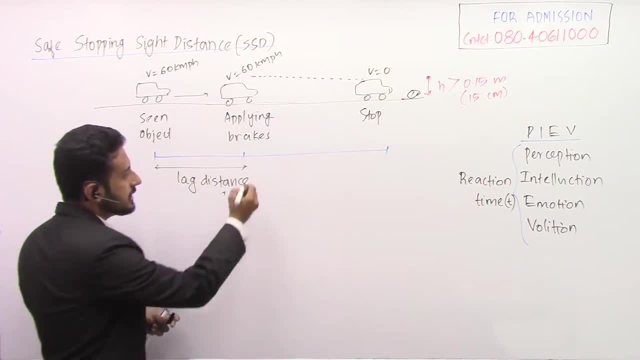 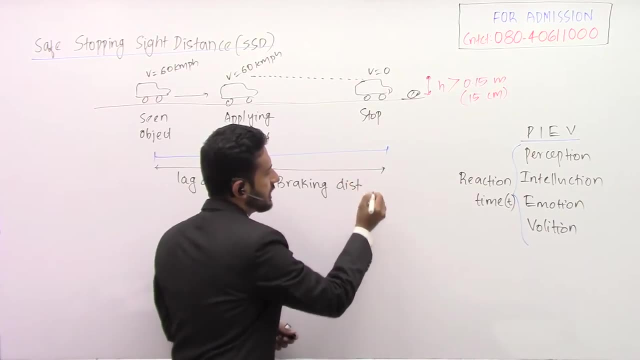 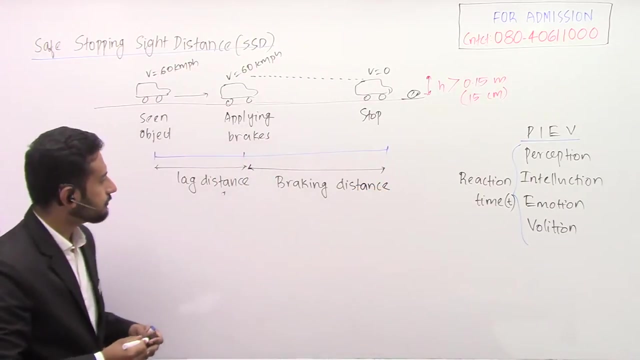 finally, speed will be zero. this distance after applying the brake, we are calling it as braking distance, or sometimes you can see a brake distance and more or less the same. so braking distance and brake distance, everything is same, okay. so lag distance and brake distance. if you're adding this, lag distance plus brake distance. 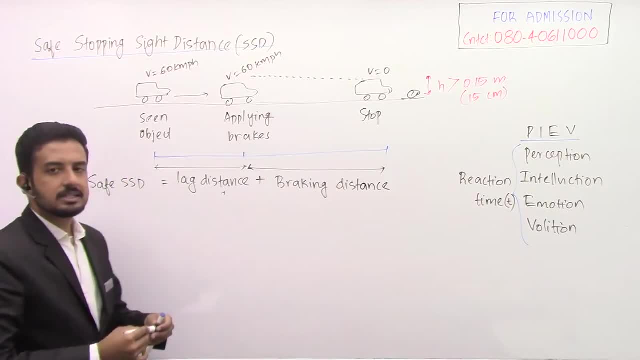 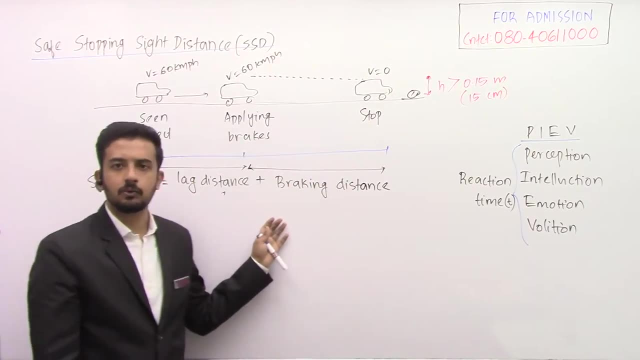 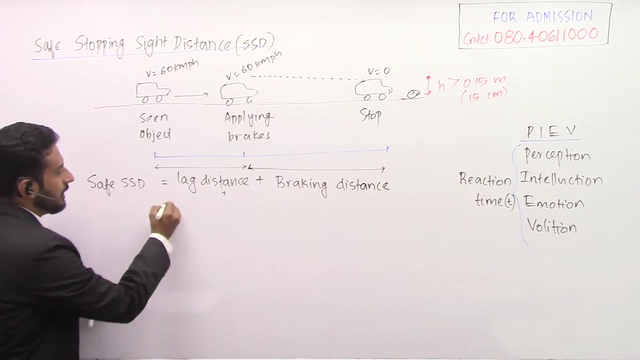 what you're going to get safe stopping sight distance or ssd. simply, both are same. okay, so now we have to see how to calculate this lag distance and how to calculate this braking distance- very important thing. okay, so lag distance and brake distance are the same. so lag distance is nothing. but whatever be the speed here. see, don't simply by heart the equation. 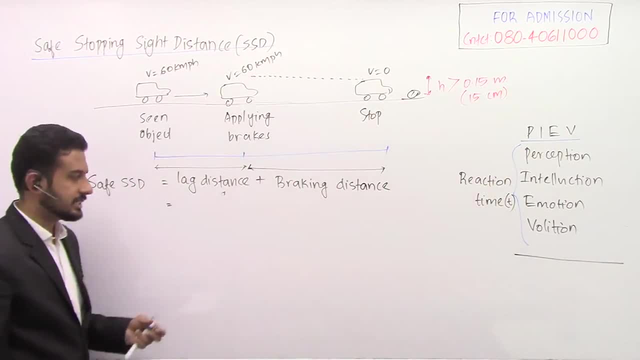 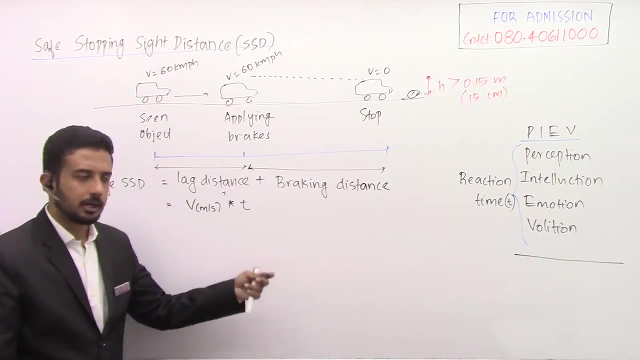 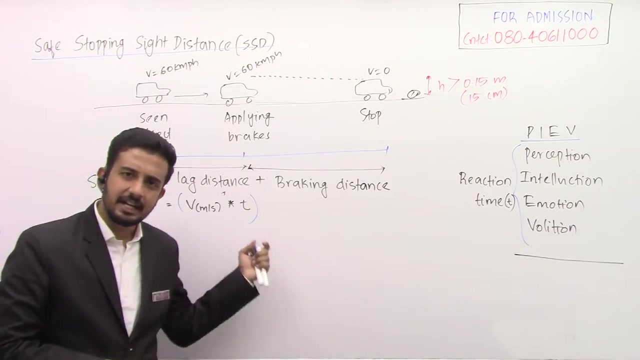 i will tell you how it is coming. and all so lag distance is nothing but speed in meter per second into the reaction time t. so i hope you are parallelly noting down so speed into reaction time t. you might have already studied some value for this reaction time. i will tell you how, when. 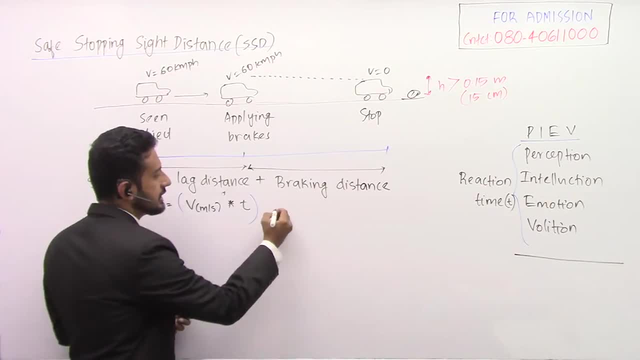 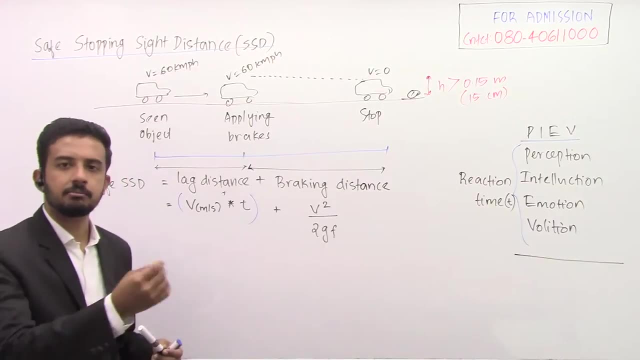 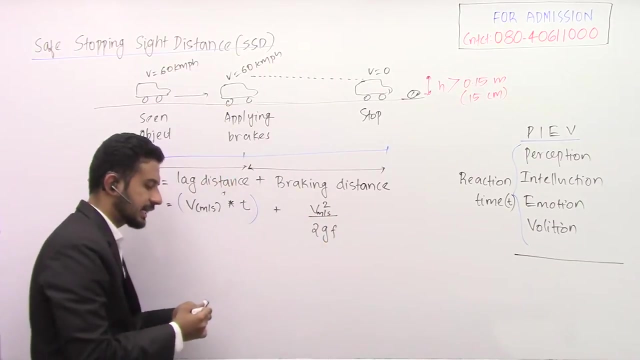 you have to use that. so v into t, the braking distance, is nothing, but v square divided by 2 gf. see, this is the general case. there are some ah special cases also will be giving you there. so here are. so v is in meter per second, g is the acceleration due to gravity, f is nothing, but we are having two frictions. 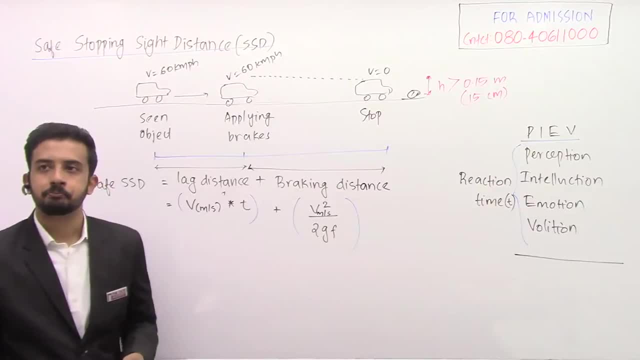 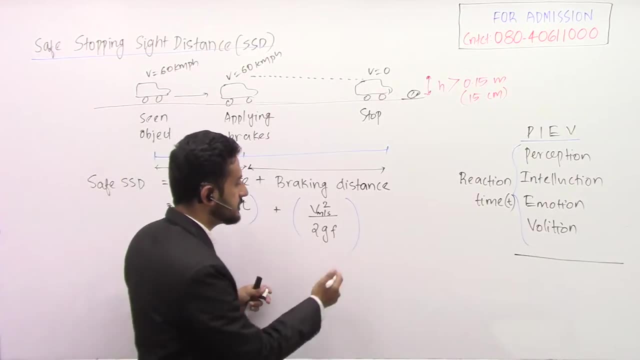 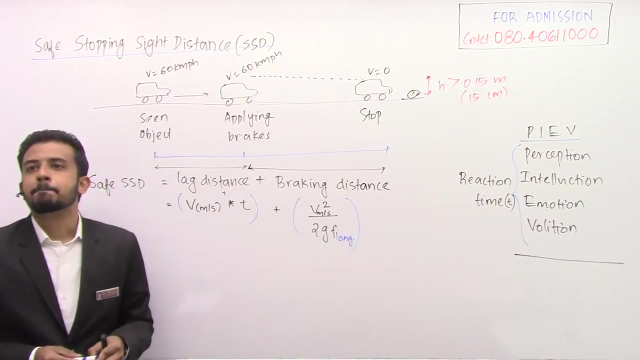 right, coefficient of longitudinal. we are having. coefficient of side friction also we are having. so here we are going to use coefficient of longitudinal friction. why? because our vehicle is moving in the straight road, okay, uh, coefficient of friction, yeah, that's what we have discussed now. very good doubt. so we have to take coefficient of. 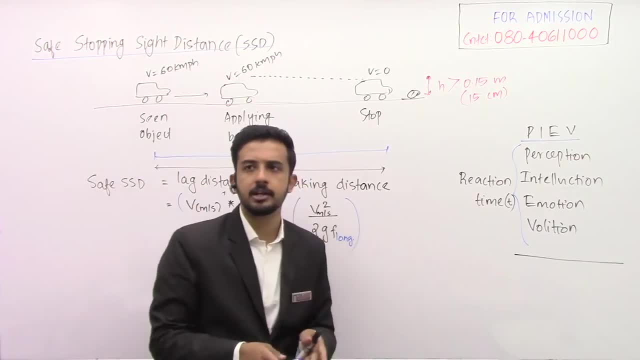 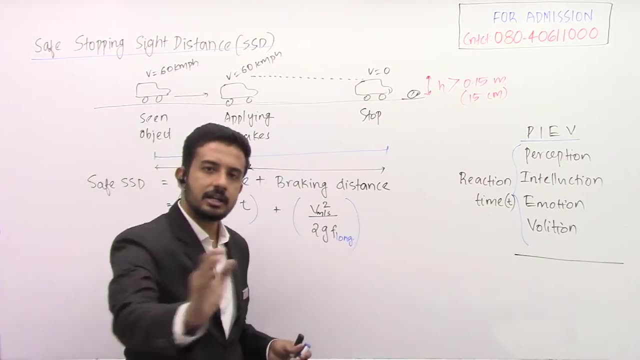 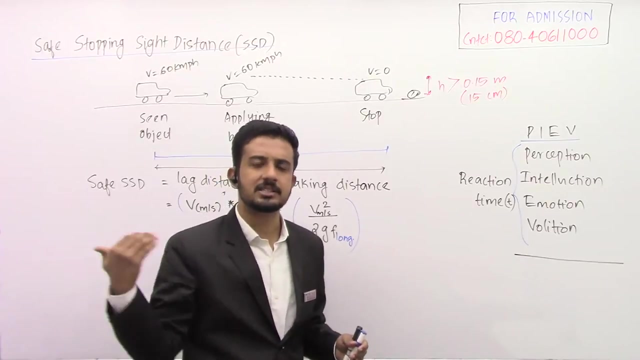 longitudinal friction because we are going in this straight road right whenever we are studying about the horizontal curves. in the coming sessions we will be discussing those things. whenever we are discussing about horizontal curves that we are turning. so when you are having a tendency to go sidewise, so someone is helping you to resist that skidding, then we will take that 0.15 okay. 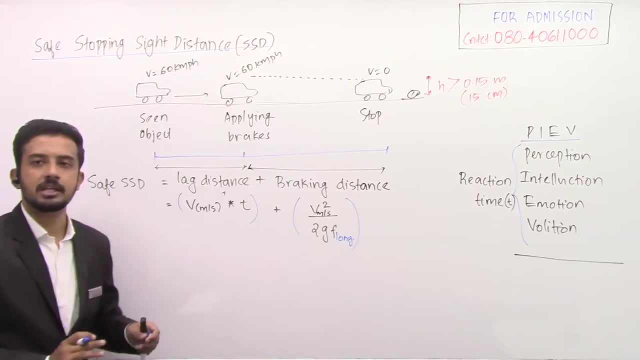 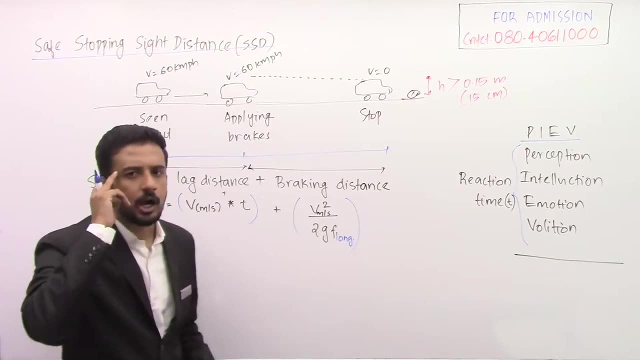 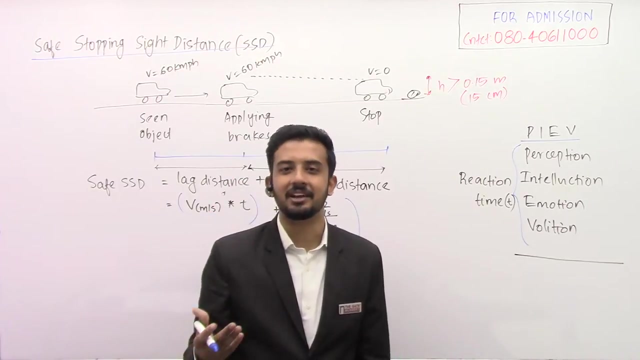 this is also in meter per second. this is also in meter per second. why we have to take meter per second. no need to buy hard these things. see this reaction time: how much time your brain will take. will it take some minutes or hours? if it is taking some hours, definitely you're going to hit and no. 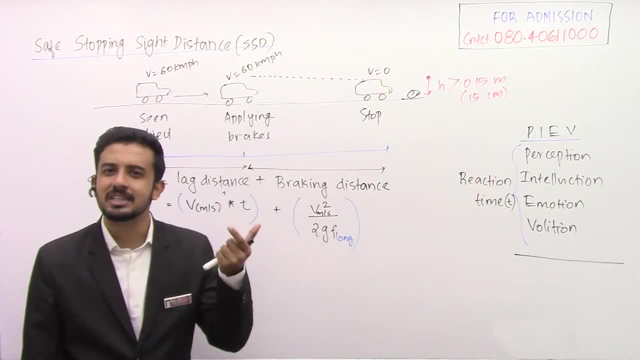 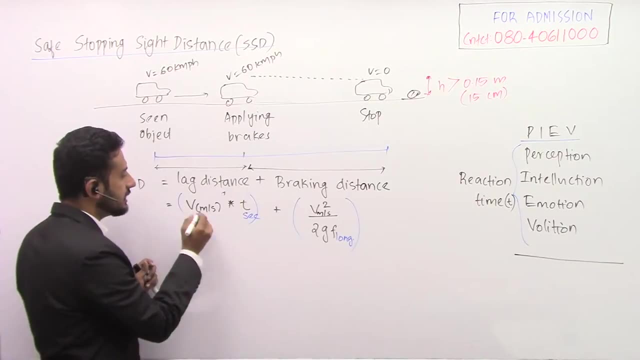 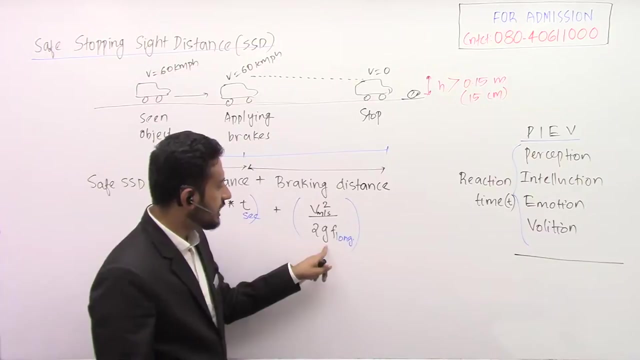 need to calculate the stopping side distance right. definitely it may be some few seconds right. since it is seconds, you need to get some value in meters. then this should be in meter per second. meter per second. this second and second will cancel. then you will get meters right here. what is the acceleration due to gravity? 9.81 meter per second square. 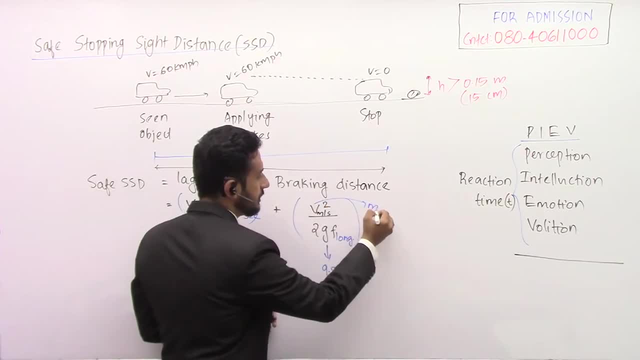 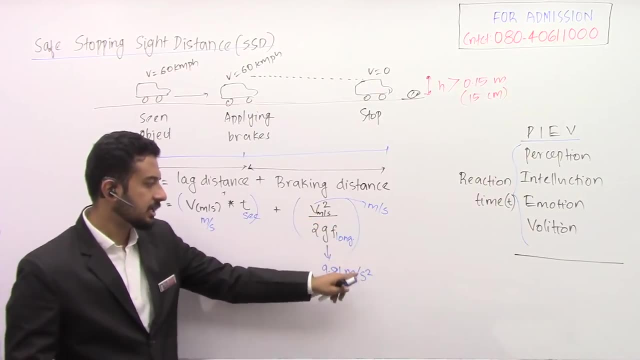 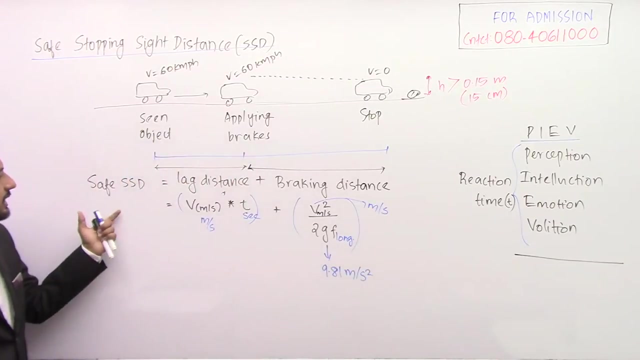 okay, so this is also will be in meter per second. this is not having any unit, it's an empirical formula. Okay, So that should be in meter per second. This also should be in meter per second, So we'll get some value in meters. We'll get some values in meters Then adding those two things. 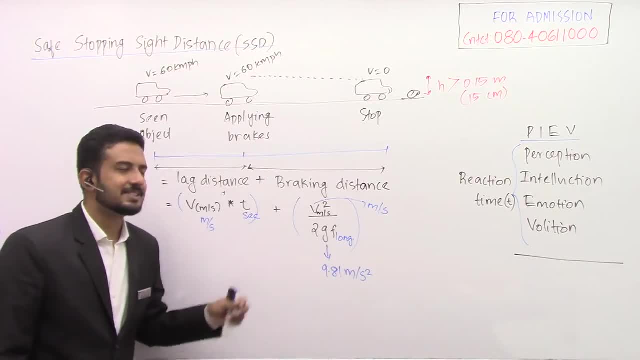 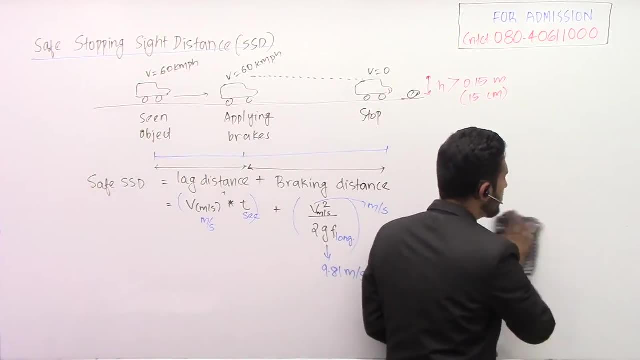 we'll get the safe stopping sighted distance. See this formula you might have already studied in the classes right In college, But I'm going to tell you how these equations are actually coming. Yes, I know, for the gate examination the derivations are not needed, but I'm just 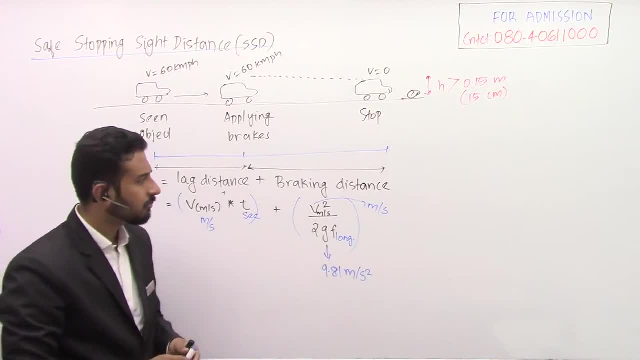 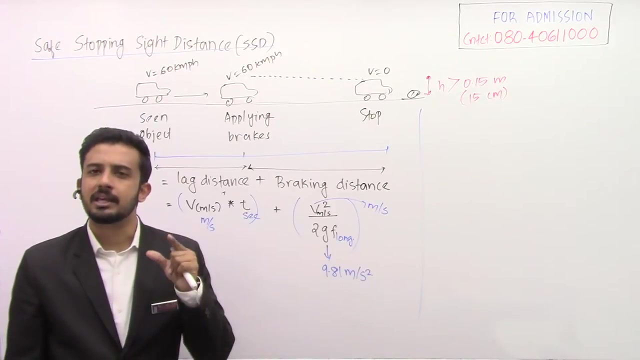 giving you the derivation for this particular concept only. Why? Because since it is a very easy concept- see direct calculation. right, It's like a standard question. You can't expect simple questions every time. Sometimes they can make some twist. So if they are making some twist, 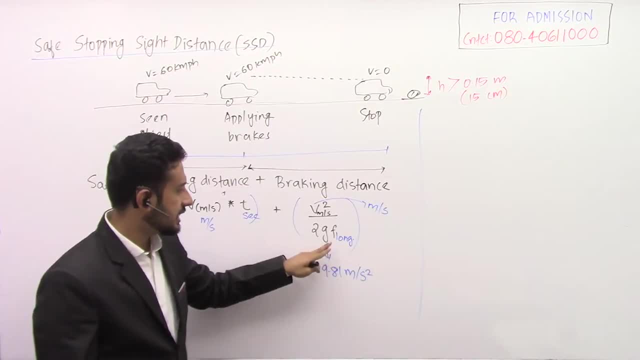 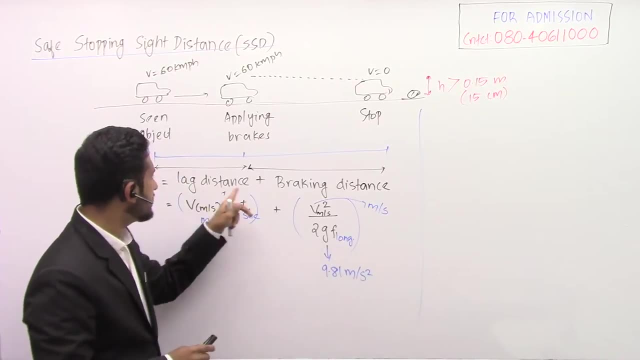 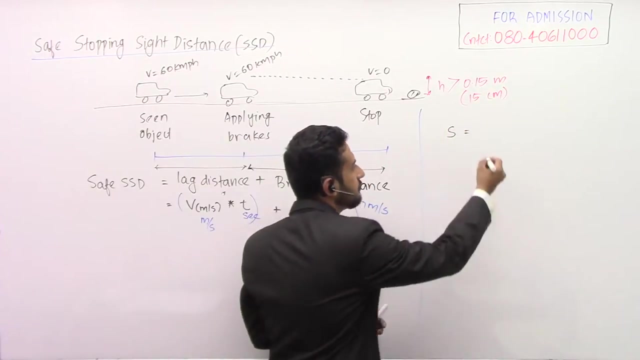 then you have to identify how to make some changes. Yes, If they are giving some gradient and all, there will be a change. I will give you that. Before that, I'm going to give some derivations. See lag Distance. We know in physics we have studied distance is nothing. but what is the equation? 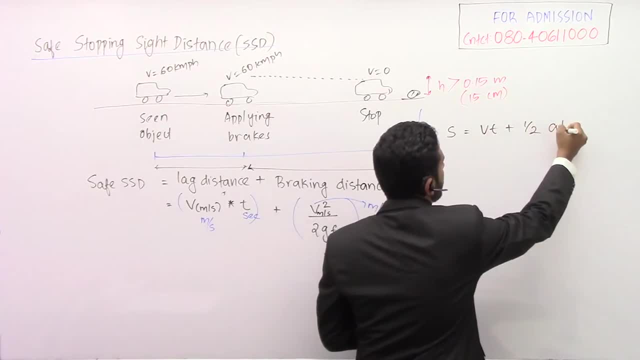 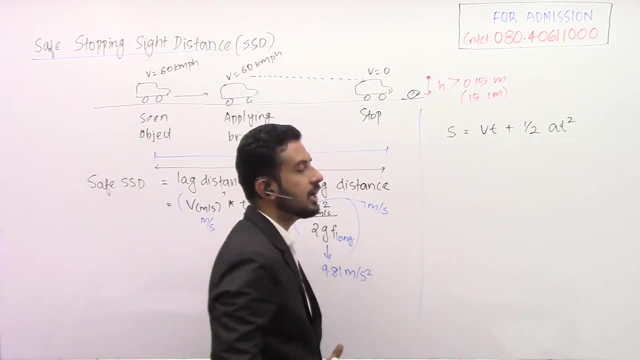 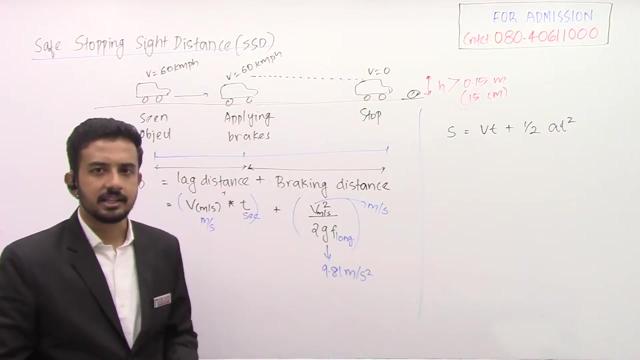 for distance: Vt plus half at square. If an object is moving at an acceleration of a, who is having the initial speed v for a distance t seconds. it is ut or vt plus half at square. We have already studied that. But see here whether it is having any acceleration or deceleration. 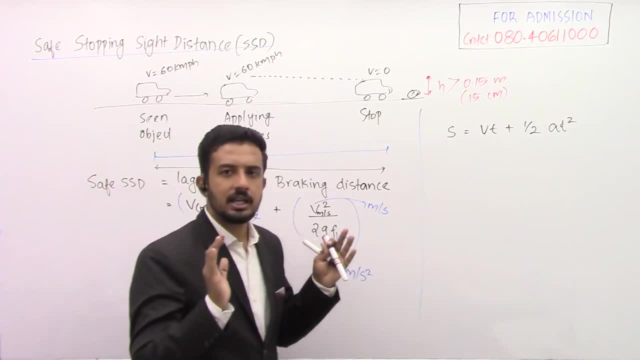 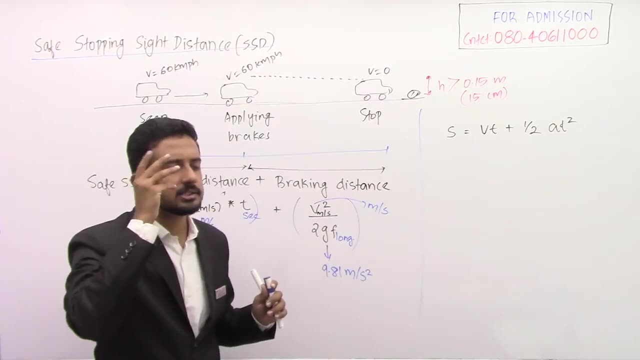 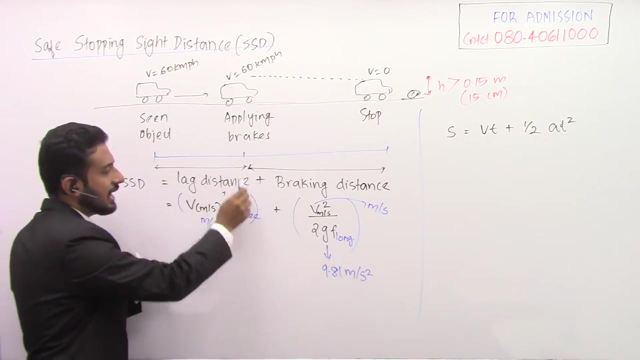 No, In that reaction time you are constantly moving. What is the example? we have taken? Example: we have taken 60. So you are constantly moving at 60. And in that some two seconds or three seconds your brain is going to make a decision. Okay, So in this portion, in this lag, 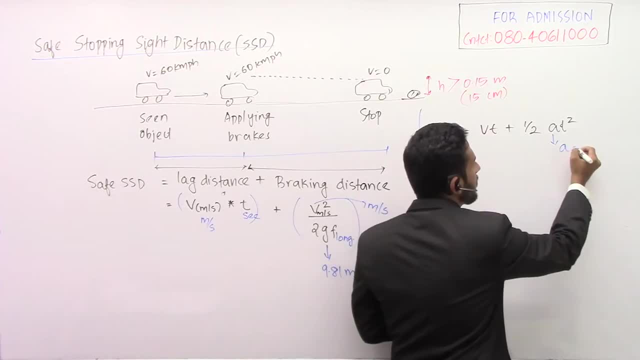 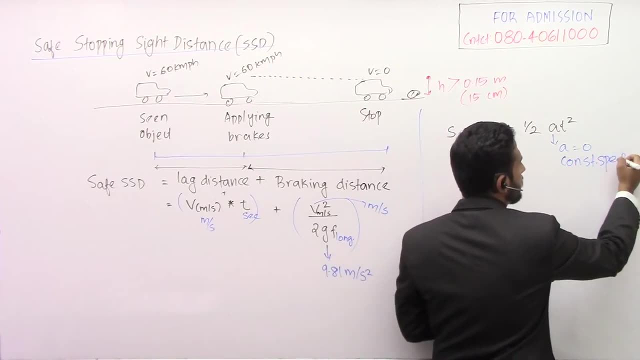 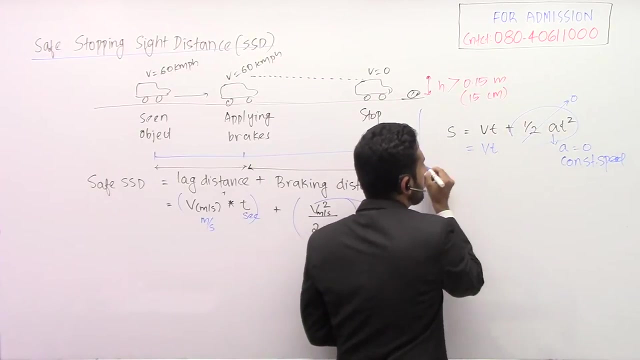 distance. the acceleration is how much? Zero. Why? Because you're moving at constant speed. So if you are going at constant speed, acceleration is zero. So this part is going to be zero. That's why it is coming as v into t. Understand There they. 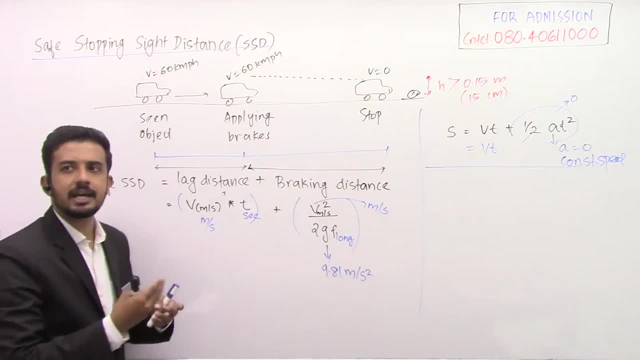 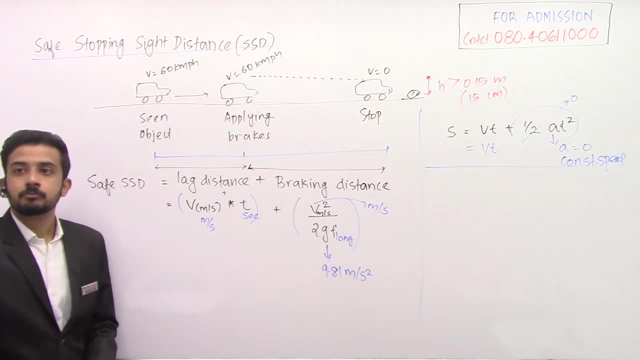 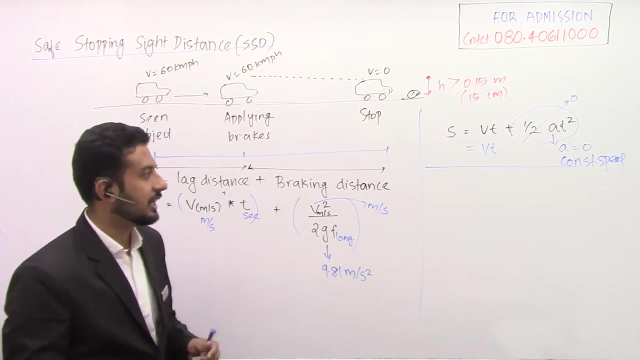 may not be making any twist- Definitely the acceleration will be zero. Okay, Now coming to the breaking distance. If in clearance we are taking curve- but sorry, I will come to that later- One second. So the breaking distance, how we are actually getting this. 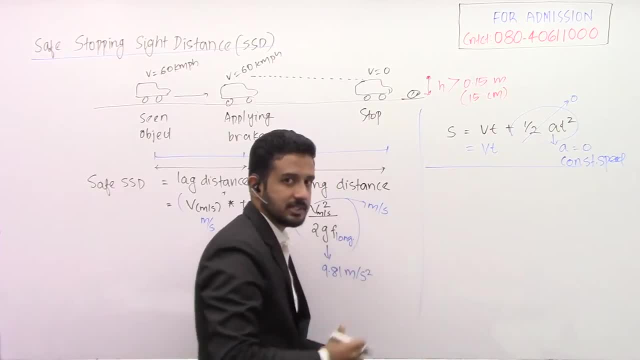 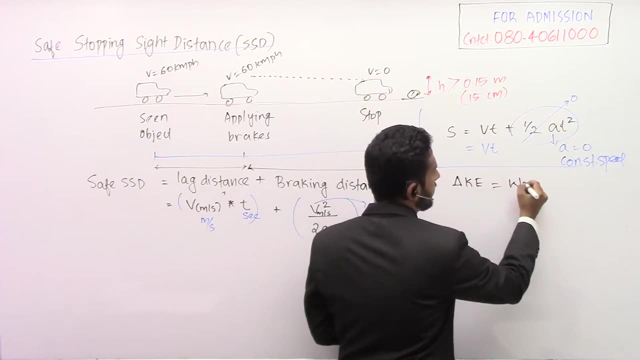 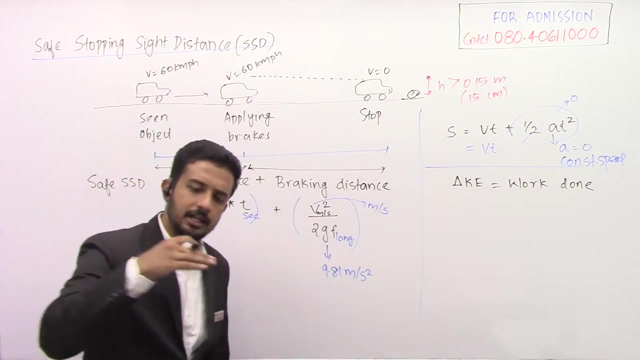 equation You might have already studied, in plus two physics, and all The change in kinetic energy. The change in kinetic energy is what The work done. So what is the work here? Stopping the vehicle? We are applying the brake So finally it is going to stop. Who is helping you to stop? 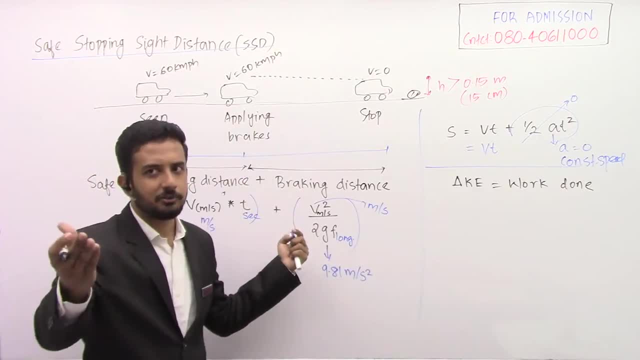 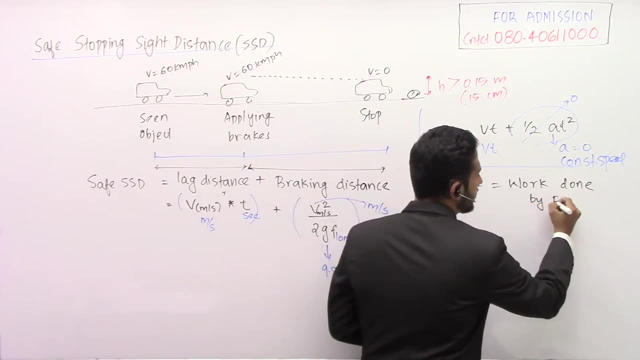 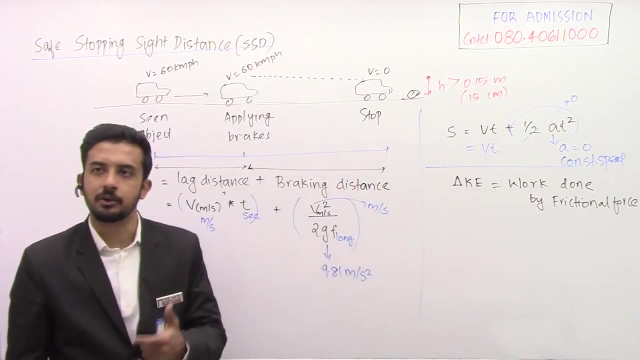 the vehicle. Who is helping you to stop the vehicle? You have already replied before, when we were discussing the cross section elements. This work is done By the frictional force Right. This frictional force is going to do the work Right. Very good. 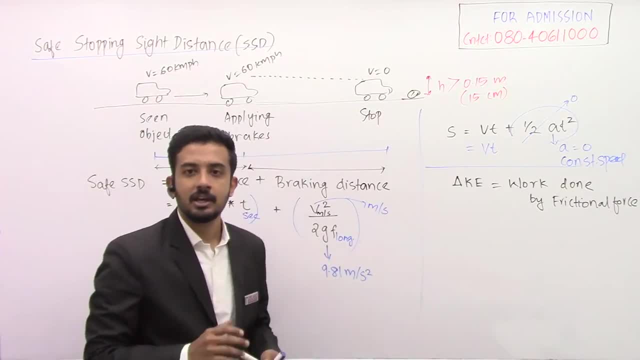 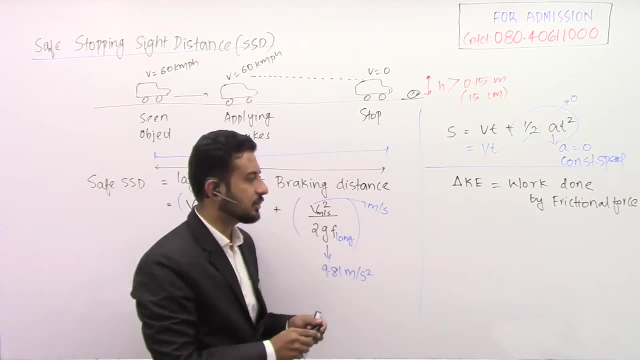 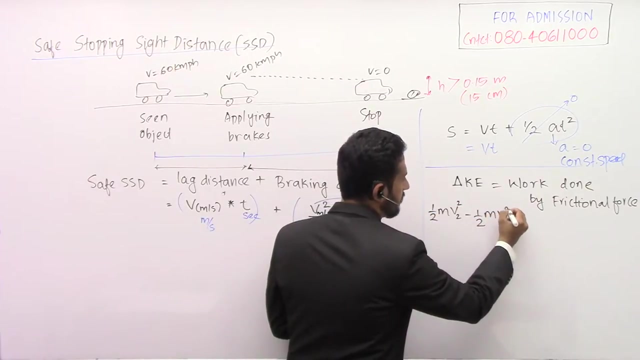 Abhishek. So what is the change in kinetic energy? The final kinetic energy minus initial kinetic energy. So kinetic energy equation: What is the kinetic energy equation? Nothing but half mv2 square minus half mv1 square, The final kinetic energy minus initial kinetic. 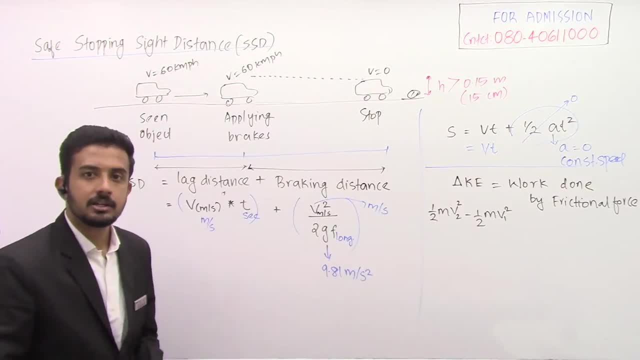 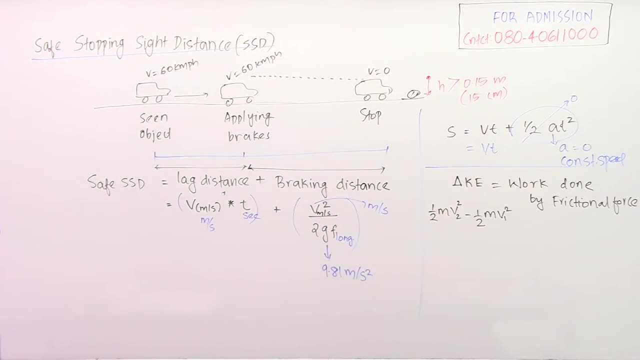 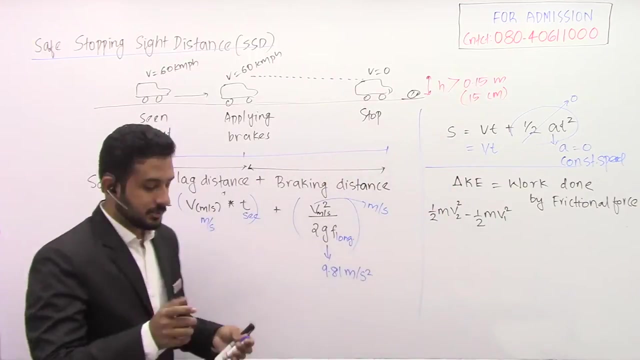 energy. We know the final speed is how much Zero One second. Yeah, Sorry for the interruption. So half mv2 square minus half mv1 square, It is equal to work done, Right? So in this case we know the final speed is how much Zero, So this: 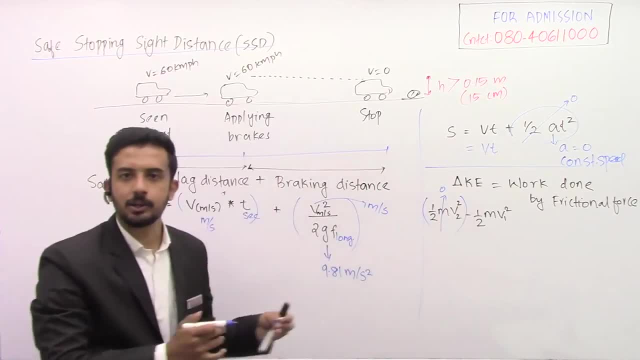 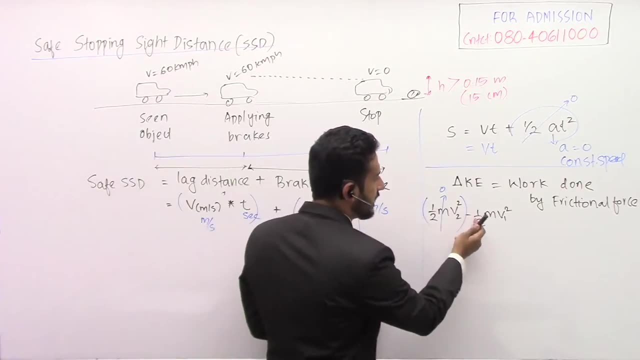 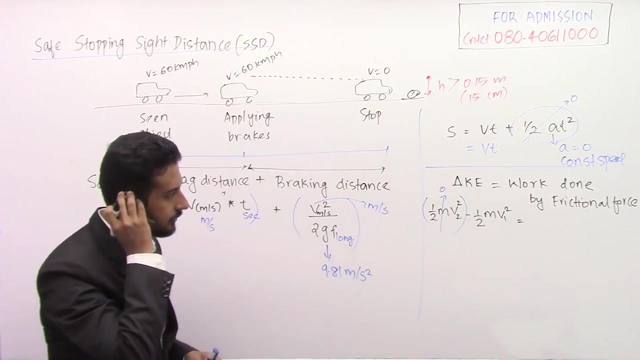 part is going to become zero. So you please note down these things. This is actually required. I will tell you how. Okay, So this part is going to become zero. So remaining part is half mv1 square. So who is doing the work? Who is doing the work? The friction? What will be the work done by a force? 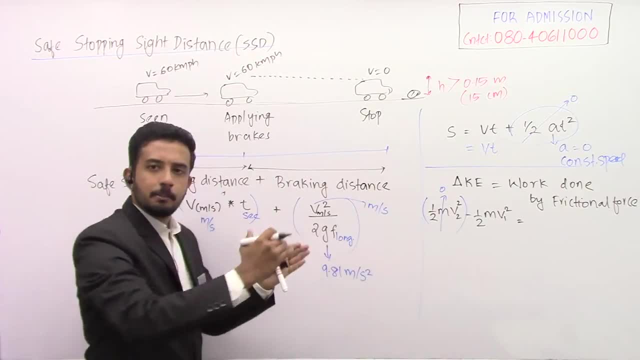 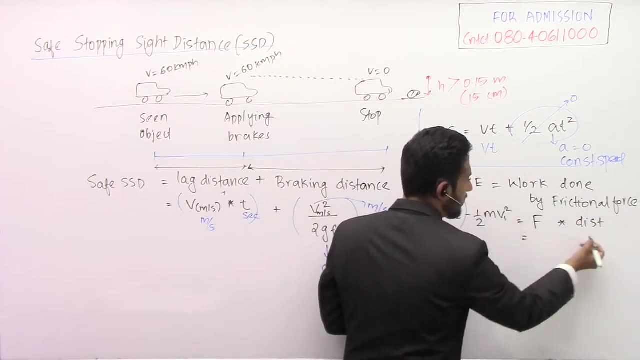 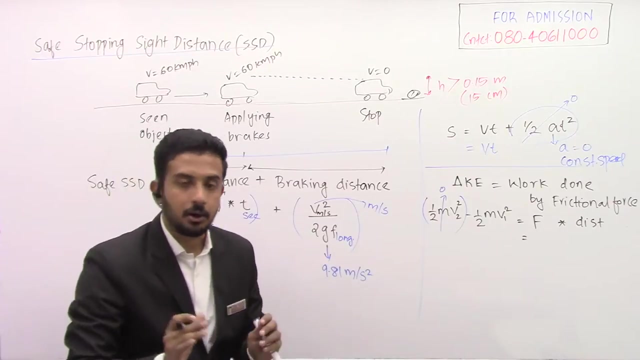 Force into distance. What is our distance? Breaking distance Now, what will be the force? Force into distance. So distance is nothing but the breaking distance. I told you what is the frictional force? Coefficient of friction into the normal reaction. So, coefficient of friction into 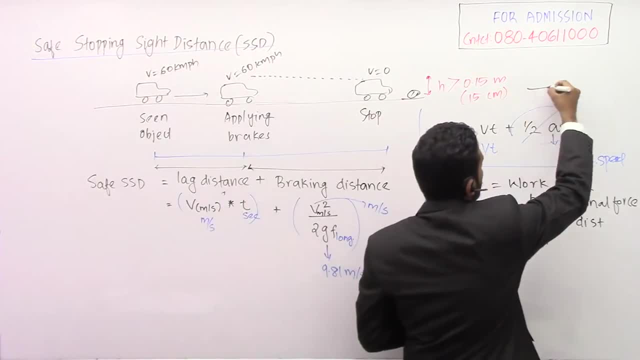 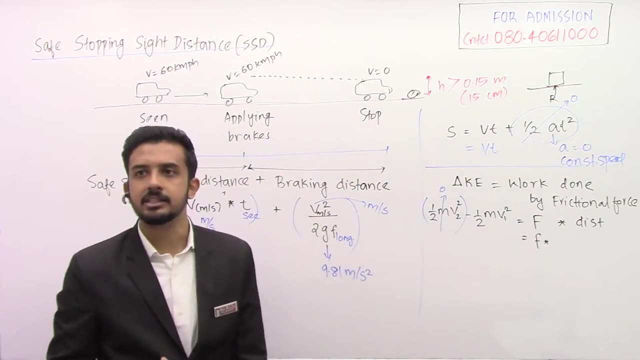 what will be the normal reaction? Whenever an object is there, it will be having a normal reaction R. Maybe you might have already seen this. So it is going to be a normal reaction R. Maybe you might have already studied in engineering mechanics or you might have definitely studied in. 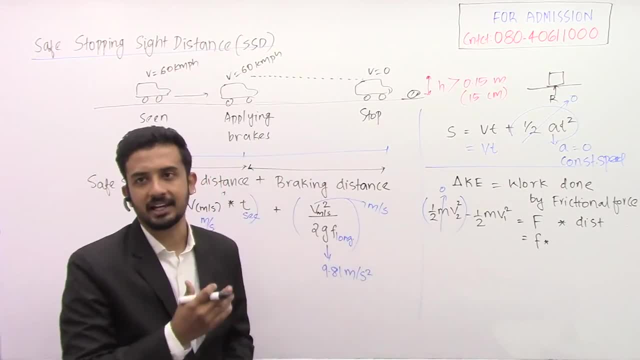 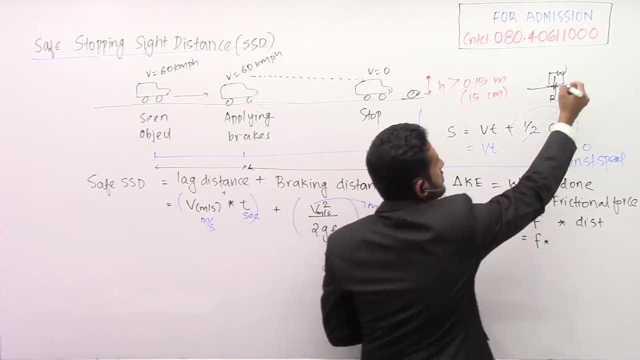 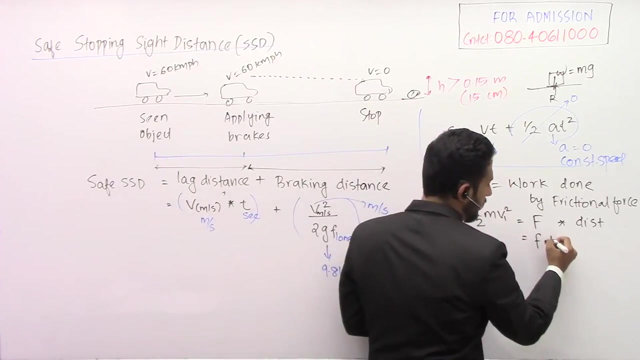 plus two, physics and all, There will be an upward support reaction, normal reaction. It will be equal to the weight of the object, W, Right. So W is nothing but mass into mg, Nothing but weight. So the normal reaction, F into the normal reaction. where I am writing, this normal reaction is: 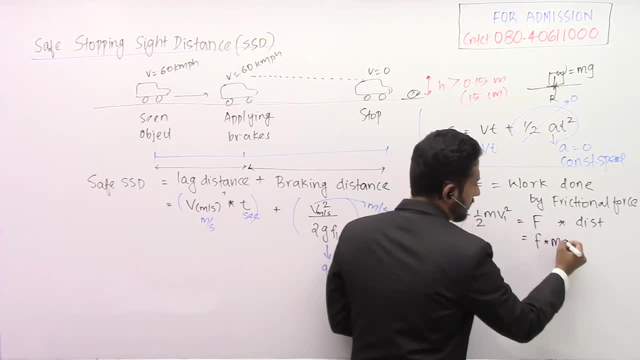 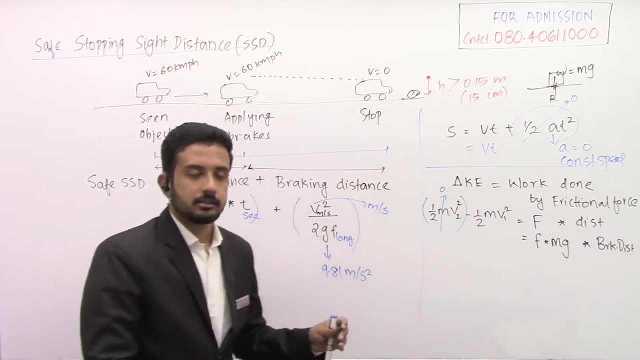 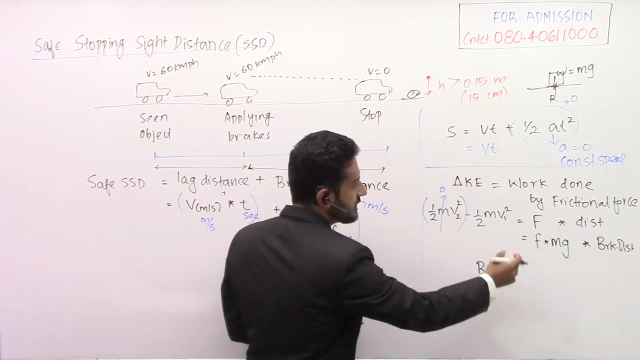 nothing but our weight. Weight is what mg Right F into the breaking distance. Till here it is clear What I require. I require the breaking distance. only Now, what will be the breaking distance, This half mv square divided by F into mg? 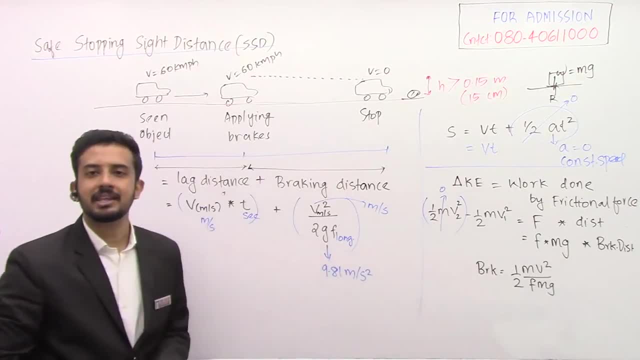 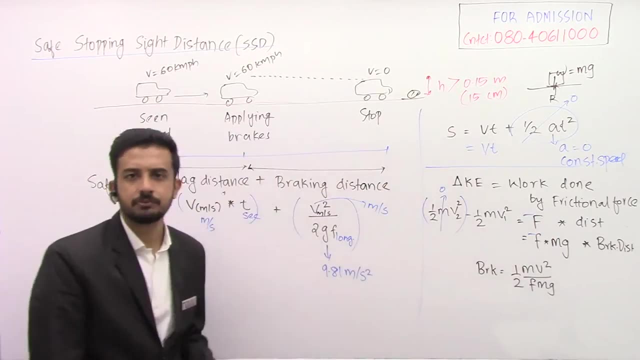 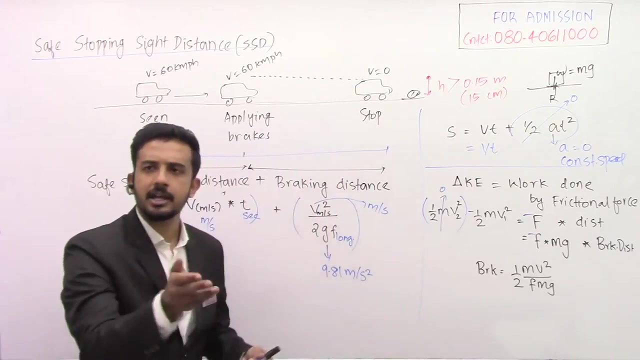 Right. See, the vehicle is moving in that direction and the friction is in the opposite direction, Right. So it is actually minus Friction, Right? It is in the opposite direction. Here we are having a minus, Here also we are having a minus, So that minus minus will get cancelled. Finally, this m and m will cancel. 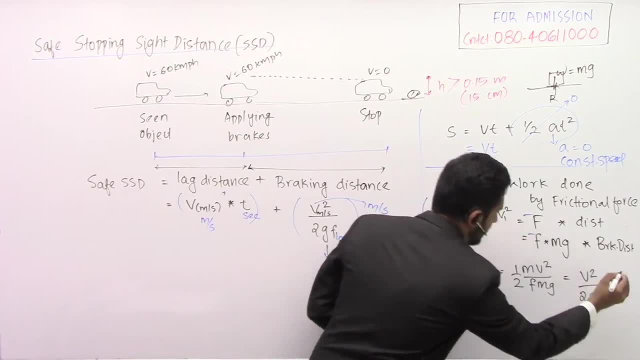 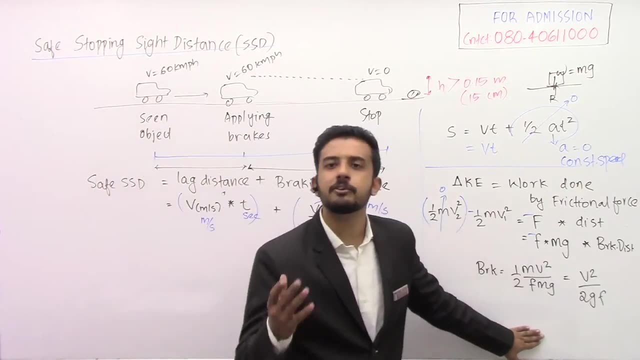 Finally what you are getting: V square by 2gf. That is how this equation is coming Now see. Now you may be wondering why I have given these derivations and all. We require only the final formula. Yes, You require only the final formula. But the thing is, sometimes they can make a twist. 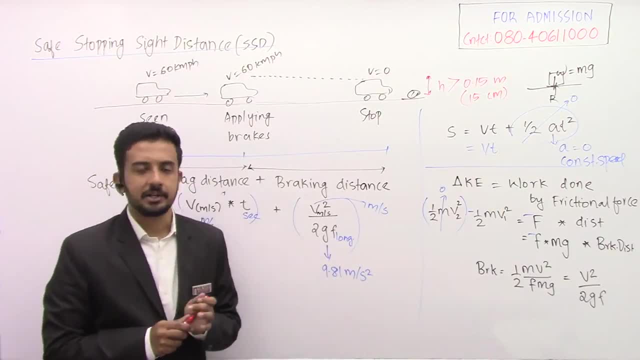 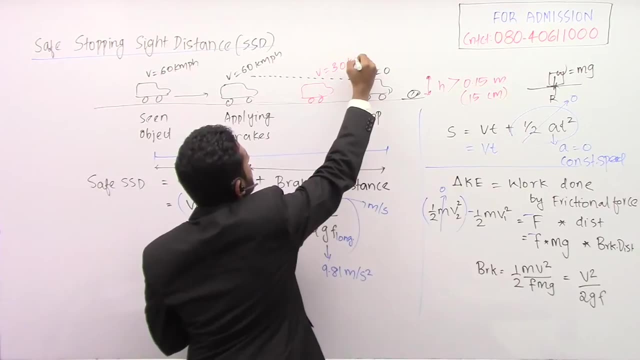 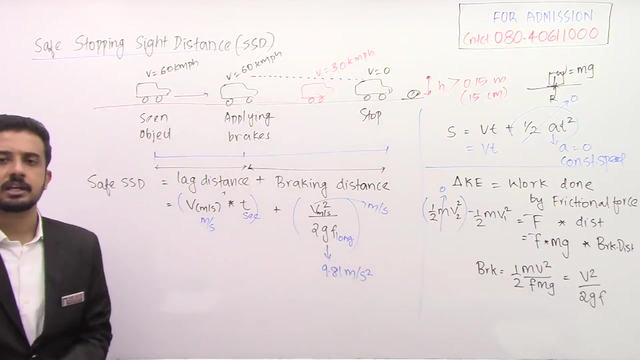 in this question. Suppose They are giving you that at some instant. At some instant the vehicle is having a speed of some 30 kmph. See here we know the speed is going to decrease, decrease, decrease and finally becoming here. Suppose they are giving that in some instant the vehicle is having some speed of 30. 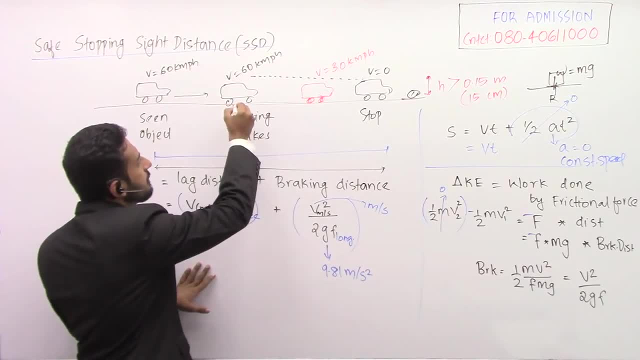 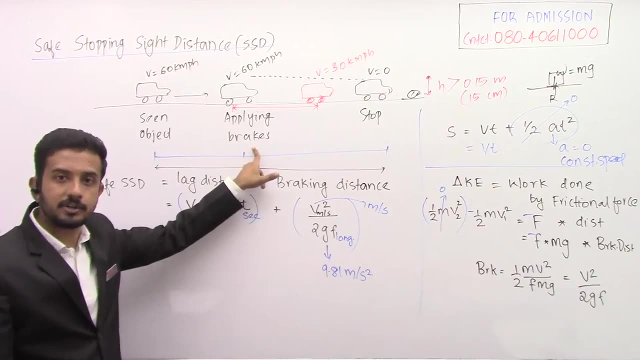 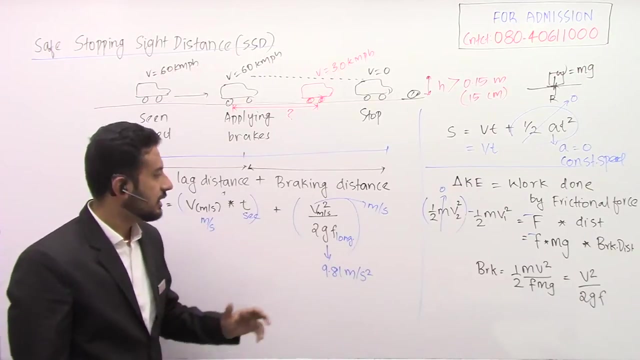 kilometer per hour, Then what may be the distance traveled by this car or vehicle from this point of applying the brake till that point? What is this distance? If they are asking such a question, what you will do If you are using v square by 2gf: you are not going to get the correct answer. 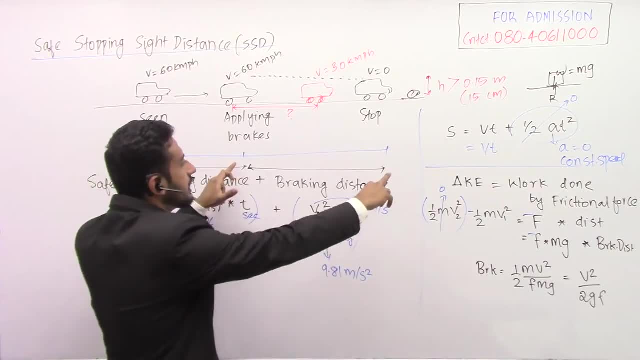 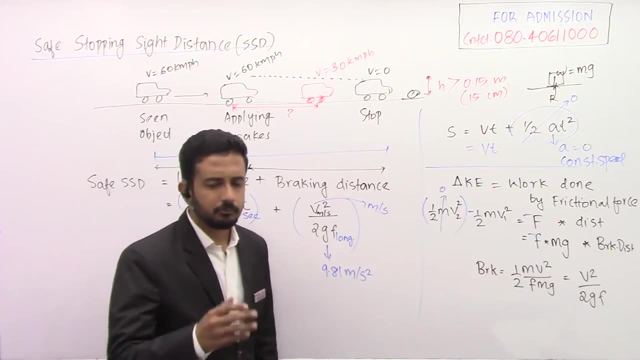 If you are using v square by 2gf, what you are going to get, The complete braking distance, In case, if they are giving some intermediate point and giving you the speed I told you know they can ask the questions like anything. So this is somewhat some level 3 or level 4 type of. 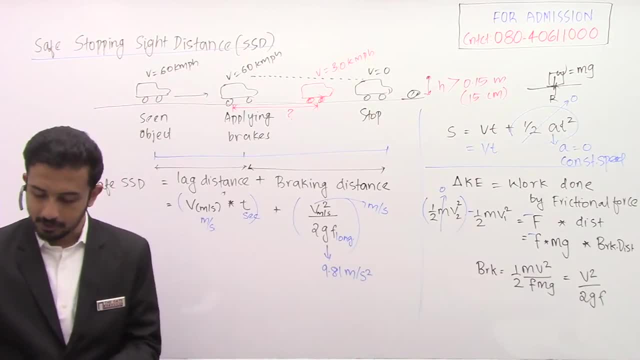 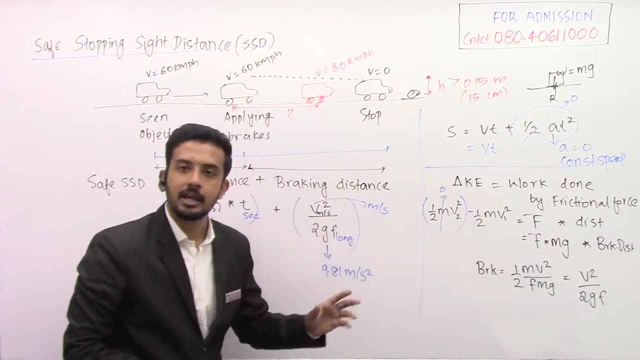 question: Suppose, if they are giving some values like that, What you have to do, What you have to do, Then you have to apply this concept. See, final speed was zero. That's why we got only half mv square. Suppose, if they are giving some concept there like that, Then what you have to do This: 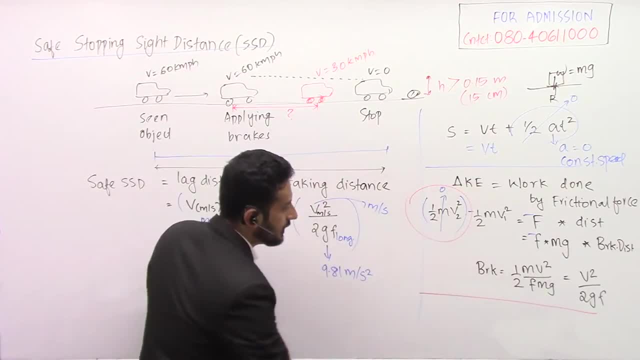 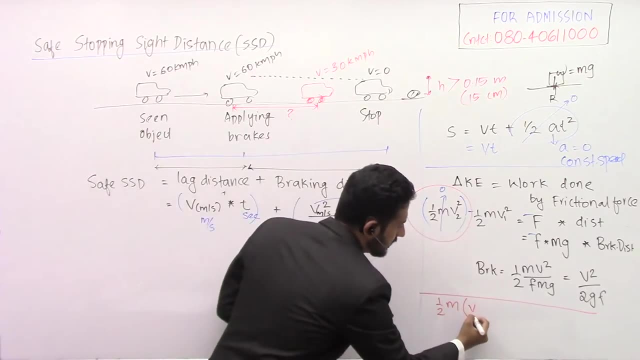 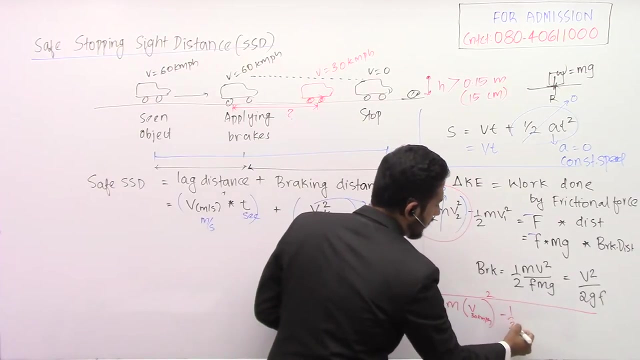 this final speed. not, it will be equal to zero, It will be half into m into See. we have to convert that into meter per second. So correspondingly, this v will be 30 kmph Square half mv square minus half into m into that 60 kmph square See. we have to convert into: 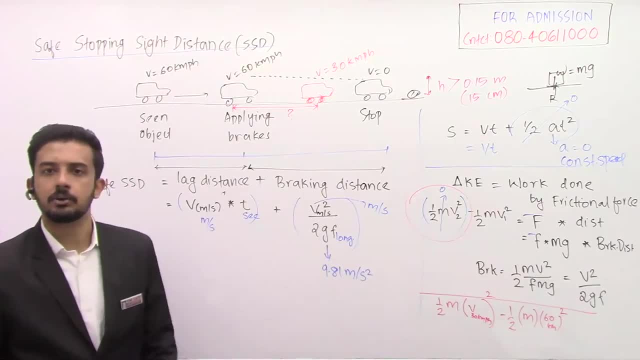 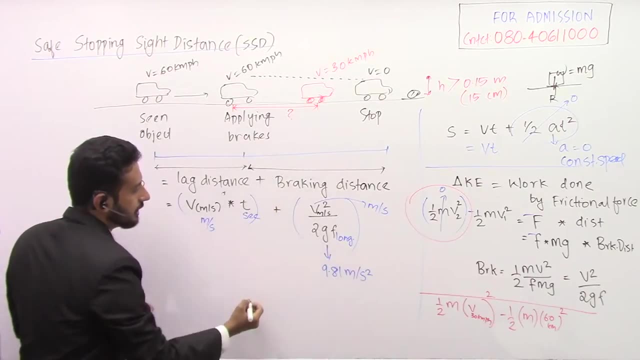 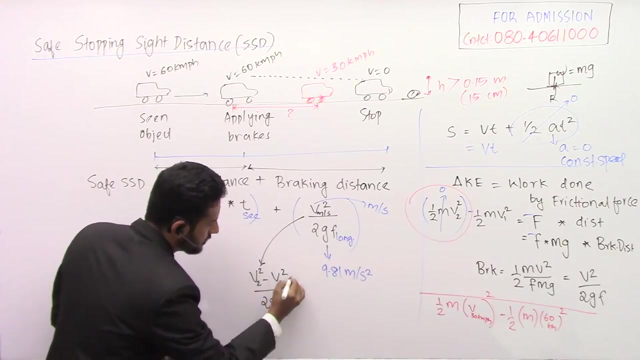 meter per second while calculating. I will give you a question: how to calculate, and not Finally. finally, the equation will become, in case, if they are giving some value like that, or final, this equation will become some v2 square minus v1 square divided by 2gf. 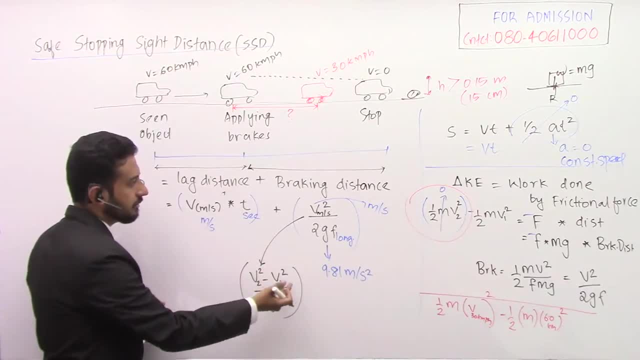 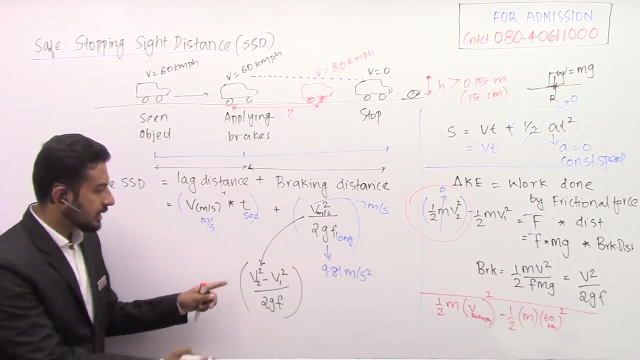 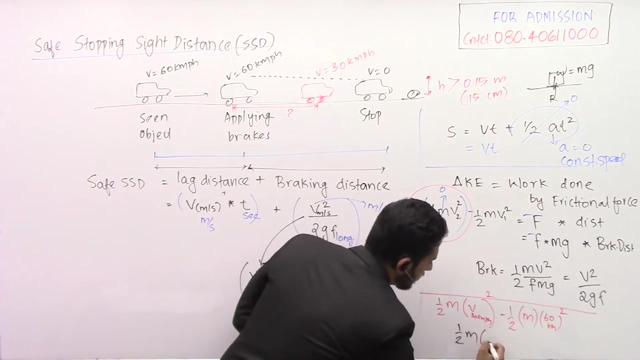 Okay. So whatever you can write- v1 or v2- anything depends on the values. So in case, if they are giving some 30 km, what will be that distance on road? then use both the values, then divided by v, square by 2gf. See, here I can take this half m common. Then I can write v1 square minus v2. 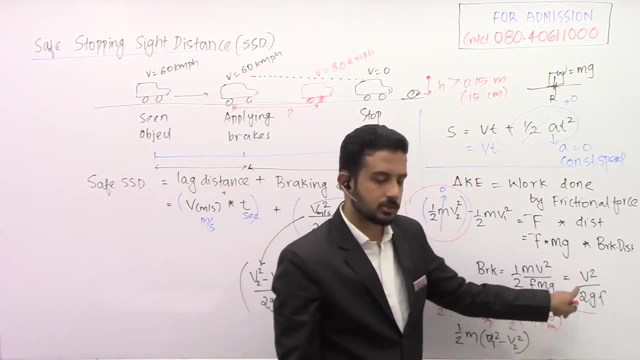 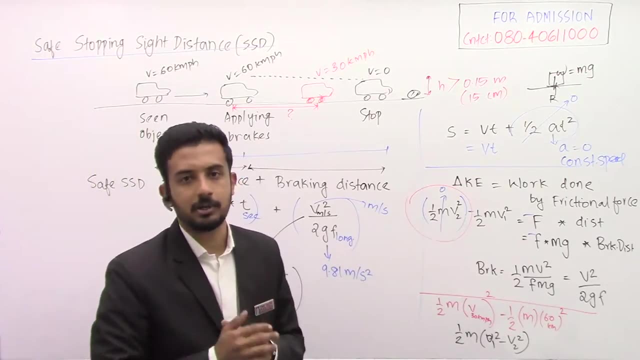 square. So nothing. but instead of simply v? square, we will be getting two terms. Okay. So remember those things in case, if they are making some twist to ask You a two marks question, See in case, whatever question they are going to ask from this numerical 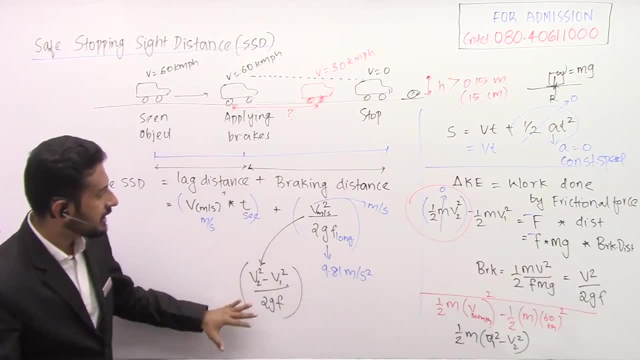 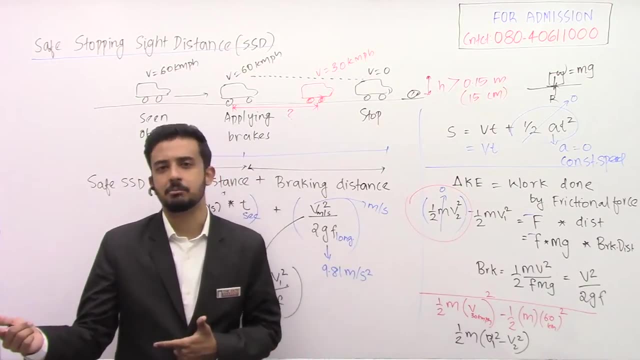 definitely it will be for two marks. Okay, Easily you are going to get. but even if they are making some twist, don't lose your mark by thinking that array, this is stopping side distance. very easy will be easily getting the marks. Don't take it as silly. since it 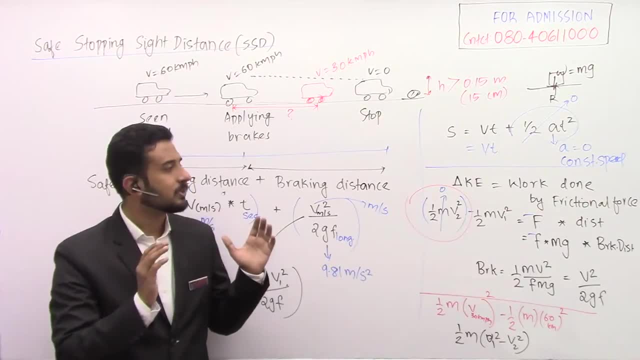 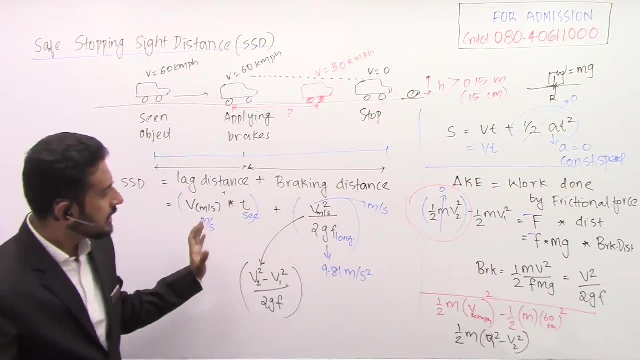 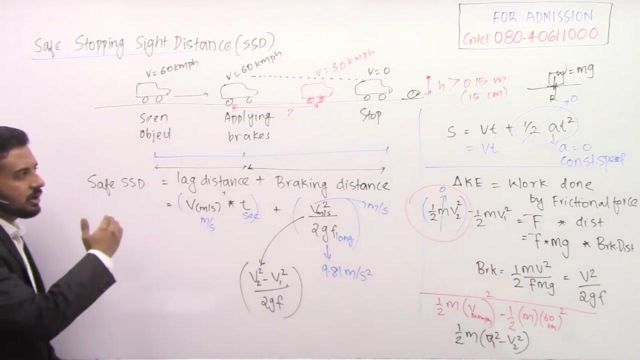 is easy, it is more dangerous. They can twist the question also. So whatever they are asking, easily you can solve. Okay, So this is a level road condition. Okay, So sometimes- yes, sometimes, someone have already mentioned- they can ask you: what is the stopping side distance on. 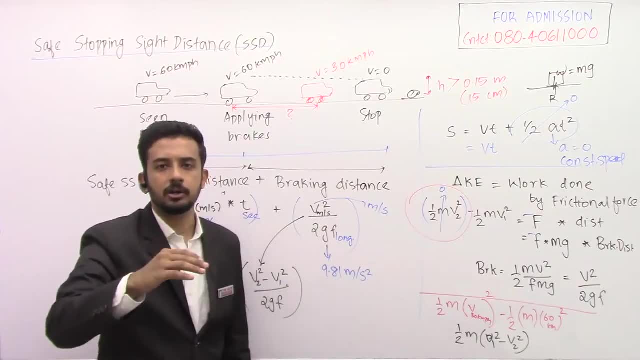 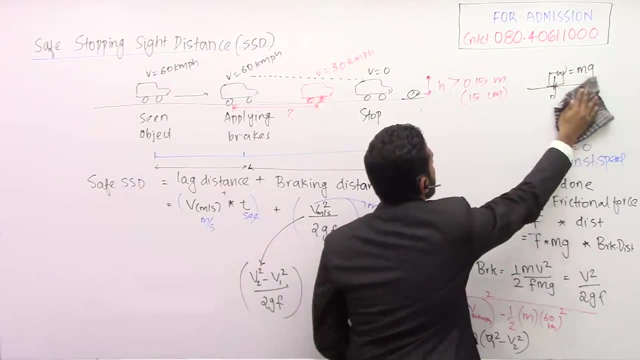 an inclined road if they are giving some inclined road, which means it is having some gradient, that slope, that longitudinal slope. we are calling it as some gradient Right. So I hope you have already note down these things. I'm going to rub this just to write our next case. 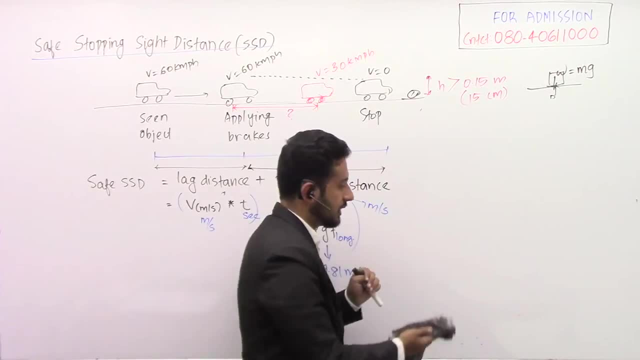 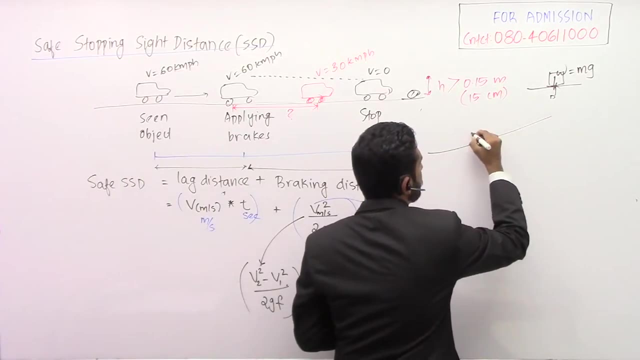 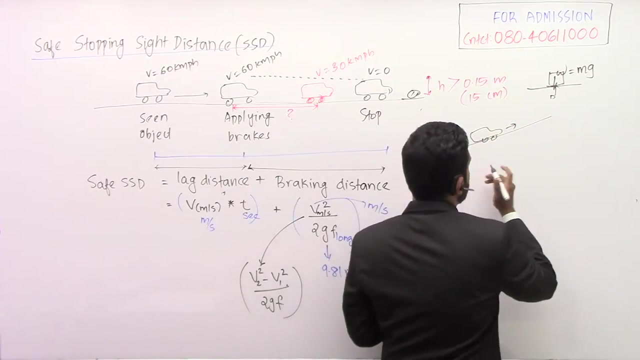 So this is what what we have discussed is a level road. Now suppose, instead of this level road, We are giving some gradient. Okay, So it can be an upward gradient, that is, your vehicle is going something like this, or it can be a downward gradient, which means suppose on. 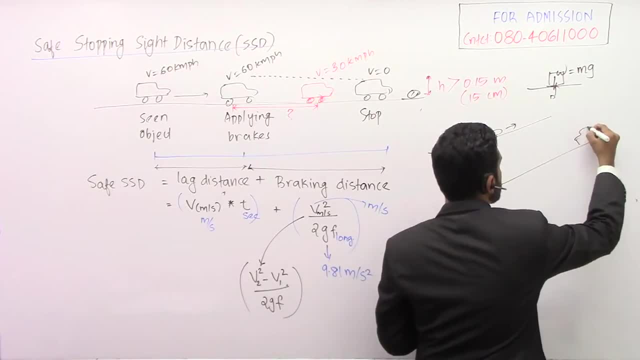 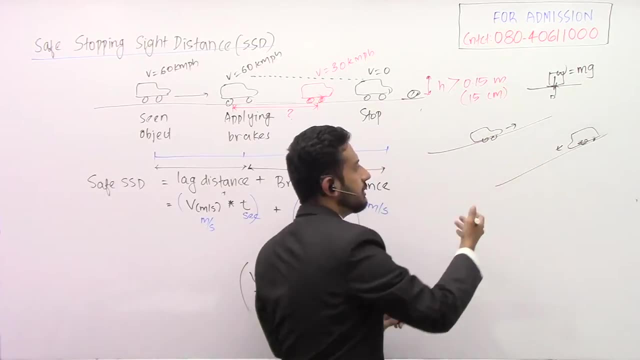 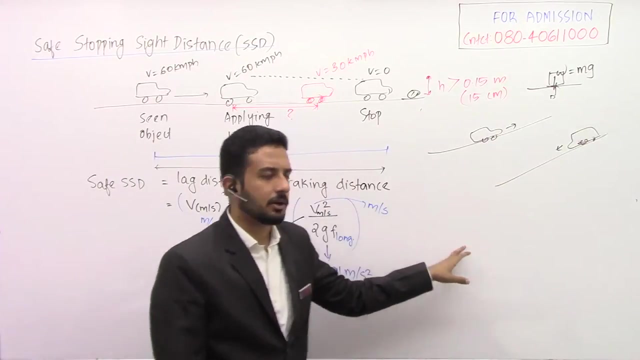 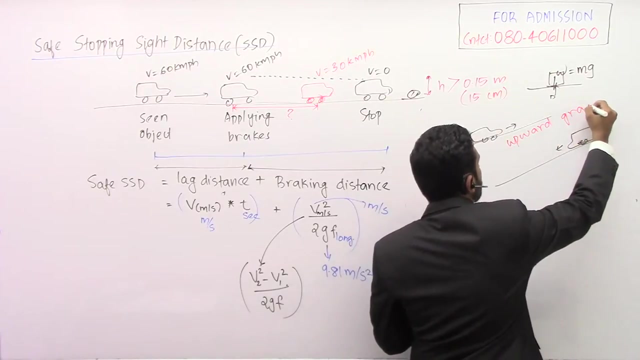 the same gradient. your vehicle is coming in this opposite direction. Sorry, So your vehicle is coming in this opposite direction. Then what will be the stopping side distance? See, will you think if a gradient is there, whether it will change or not. Just tell me. if it is an upward gradient, This is upward gradient. Upward gradient This. 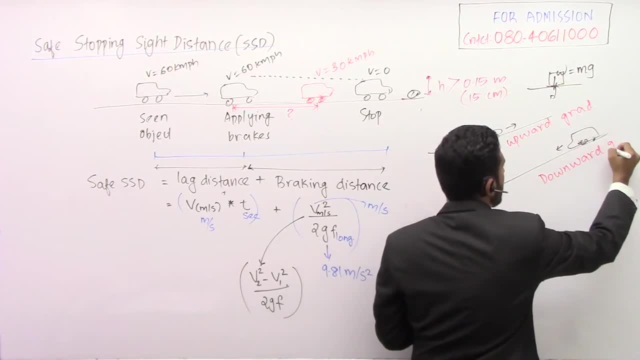 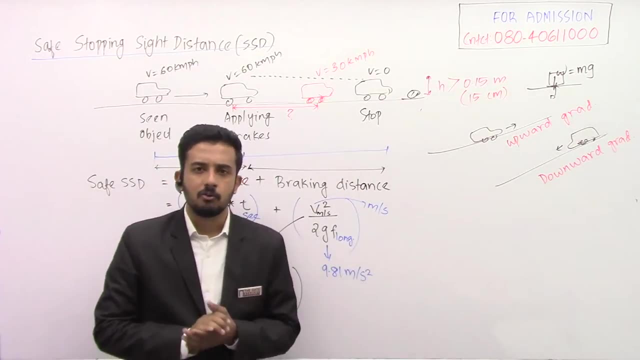 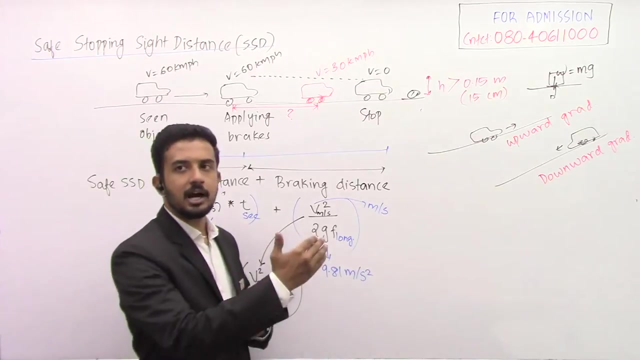 is downward gradient or decreasing gradient. If it is an upward gradient, see from your experience, tell me if you are going up whether you need more distance to stop or less distance to stop. Just tell me from your experience, if you are going up, what will be if you are. 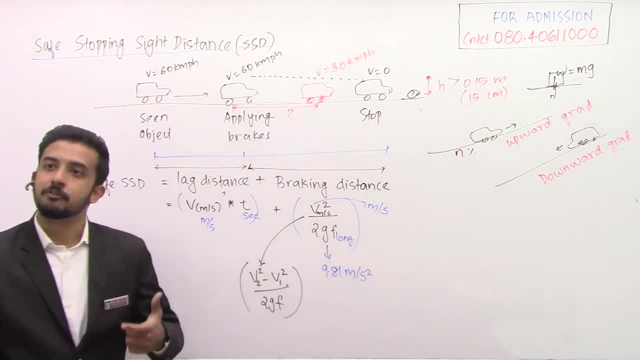 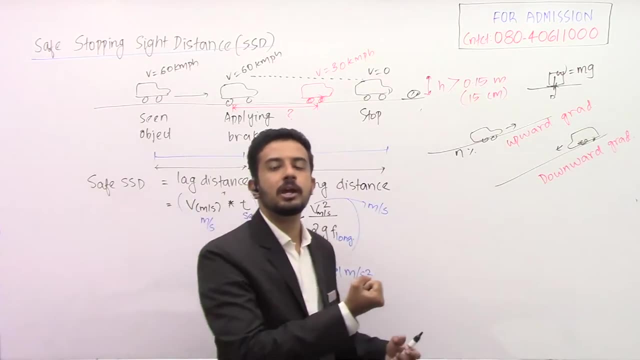 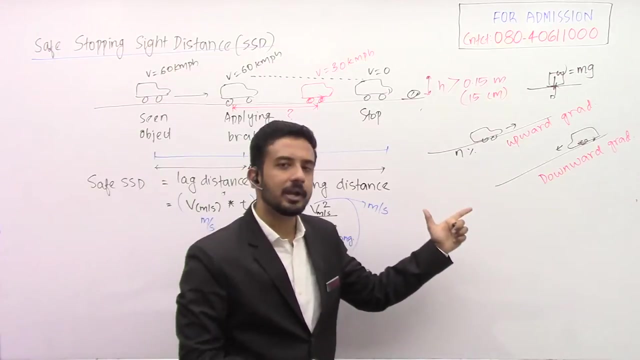 going up, right, Right. So here you need a component of your weight of the vehicle which is trying to pull your vehicle backside, So that much distance you don't require because you are getting some extra pull backside Right. So while going upward, you need some less stopping side distance. So here, actually stopping side. 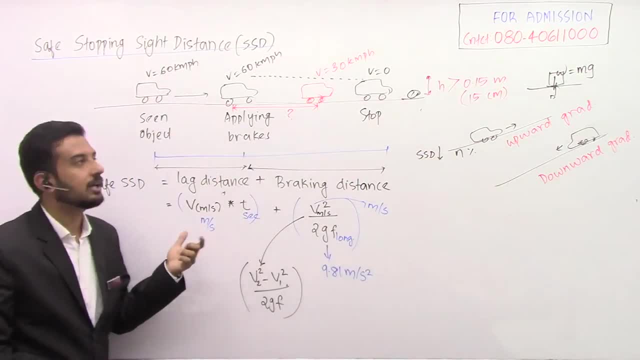 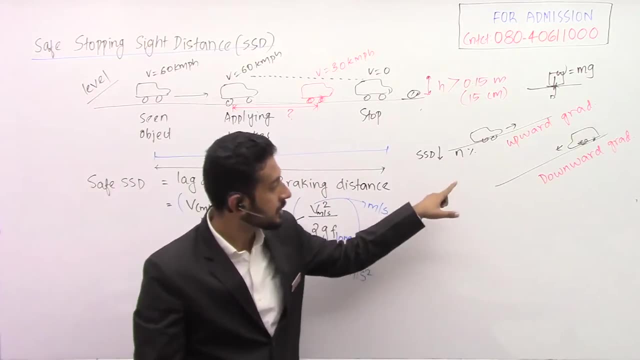 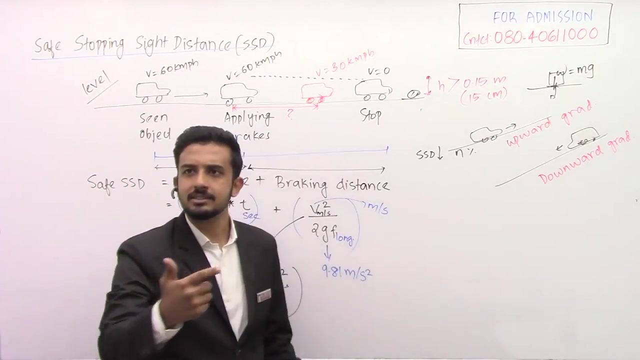 distance is going to decrease compared to our level. So this is nothing but a level road, Right? So Compare to this First case case. in this case, ssd is going to decrease. what about downward gradient? you're coming like something like this? then you need more or less or equal, if you are going downward, what it will be. 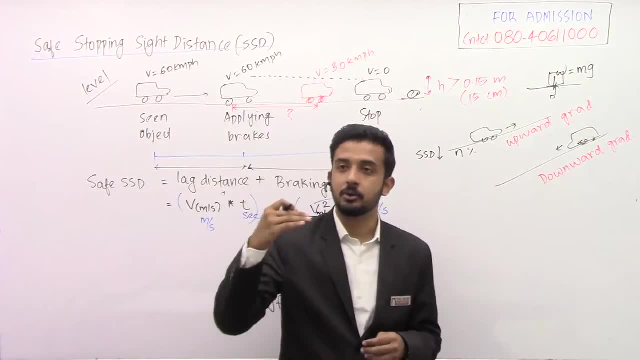 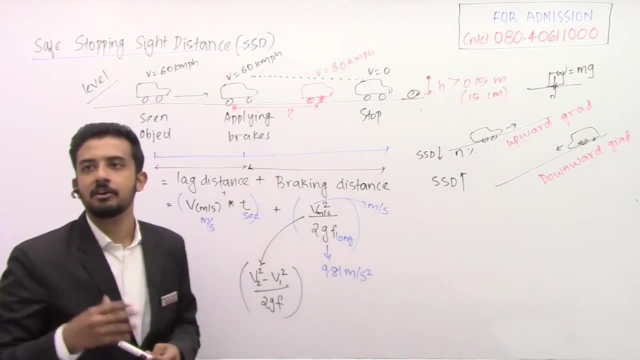 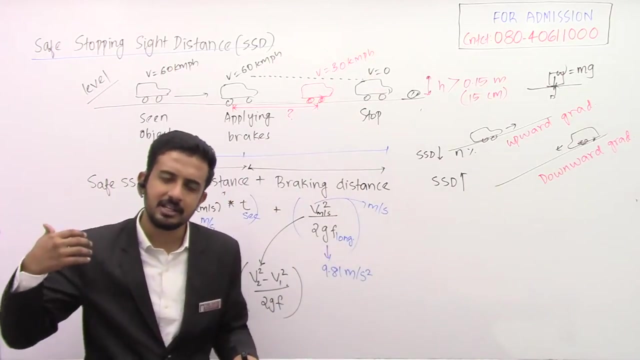 definitely you might have experienced in your day-to-day life. right, if you are going downward, the ssd will be. yeah, ssd is going to increase. right, very good, very good. of course it is more because your weight is in the downward direction. now a component of weight. it is going to pull you. 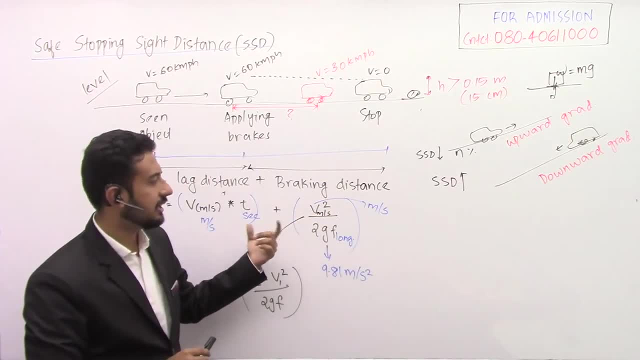 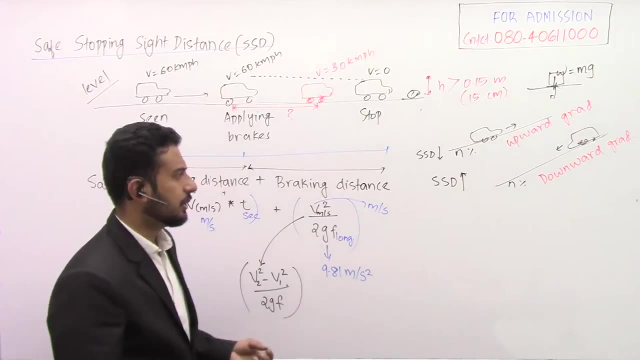 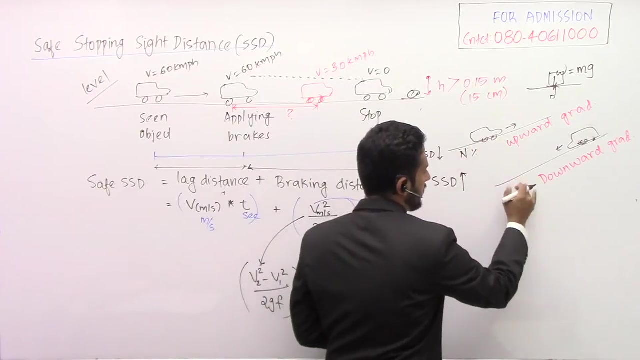 downward. so there is a change in the uh stopping side distance formula. if they are giving some gradient, i'm just denoting it as some n percentage. i told you either i can represent in one, in n or i can represent. i have already used that same letter, small letter n, so i'm just giving some. 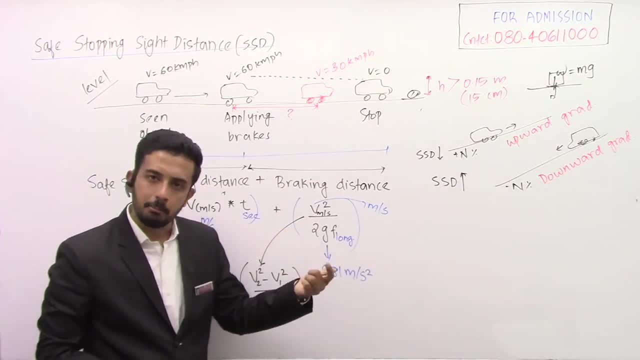 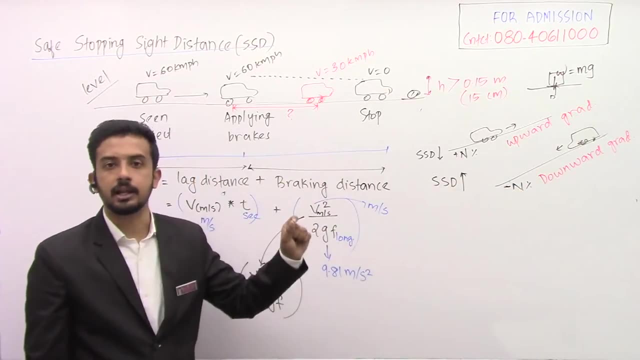 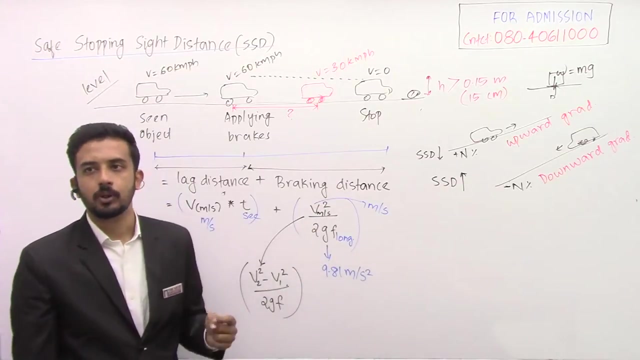 see there is one more notation: plus n percentage, minus n percentage sometimes if they are giving some plus value, which means it's an increasing gradient or upward gradient, or if they are giving some minus three percentage, minus two percentage, which means it is a downward okay. so see that notations also. sometimes they can give like this: 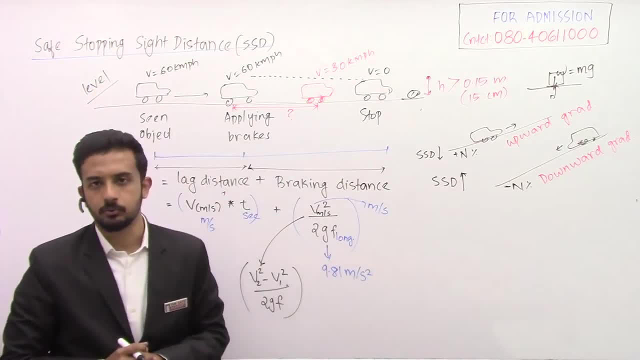 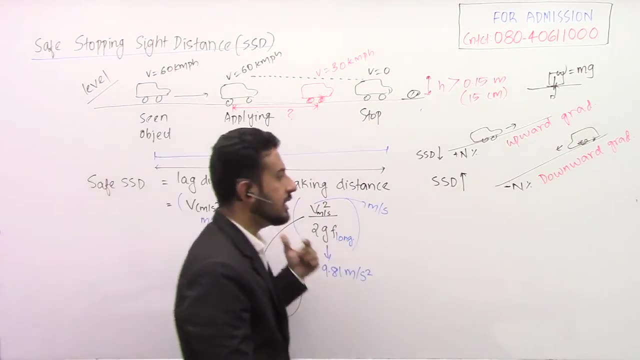 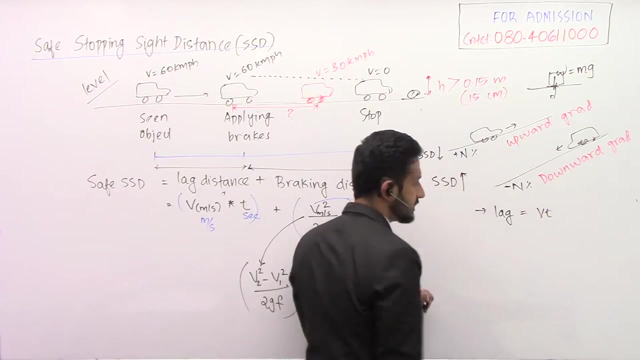 instead of telling you whether it is an upward or downward. okay, so what is the change is going to happen? this is going to affect our breaking distance only, not the lag distance. so write a node, the lag distance will not change. lag distance is v into t itself. 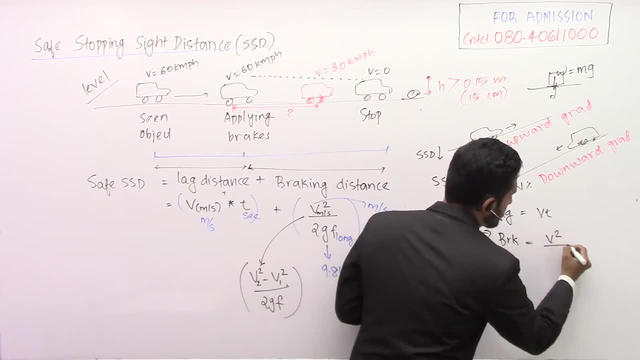 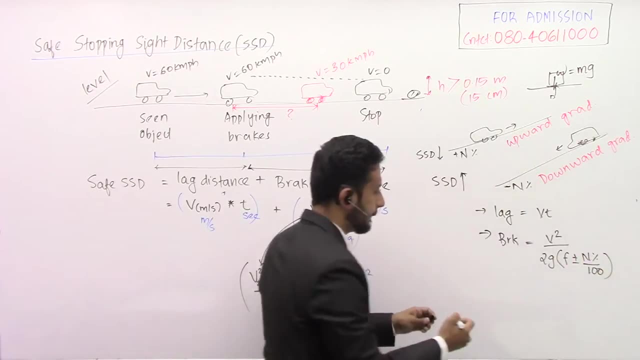 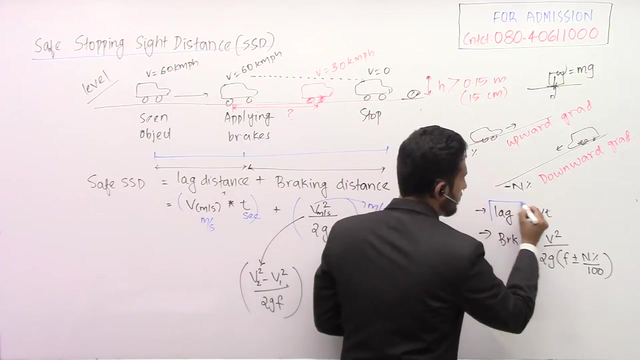 now what will be the breaking distance? it is equal to v square divided by 2g. f plus or minus, n, percentage by 100. why i am writing plus or minus? if it is an upward gradient, we know it is plus, and if it is a downward gradient it will be minus. 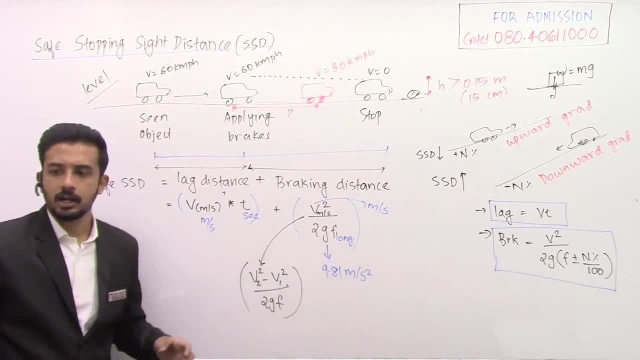 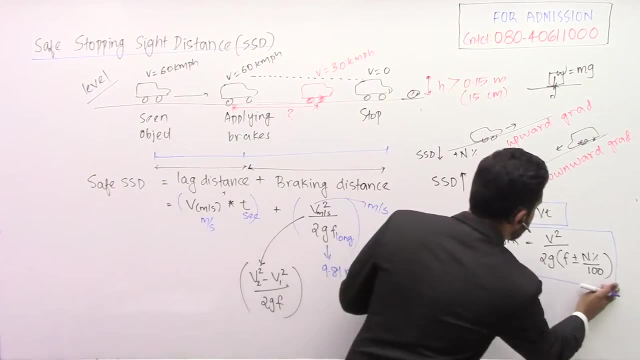 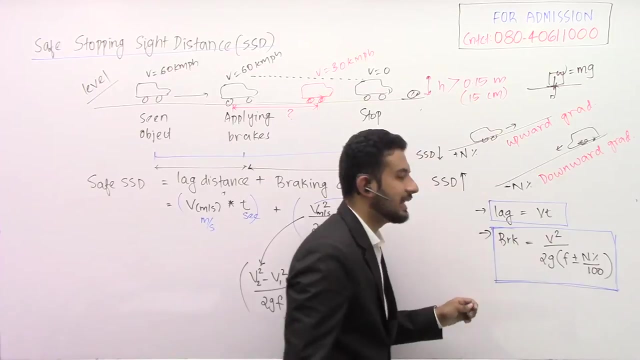 okay, we will do some questions. also how to calculate that? see, uh, why i have written that it is n percentage by 100 and all. why i have written that n percentage by 100 and all? because we have to substitute the values in terms of decimals means. suppose this is given as an example. they. 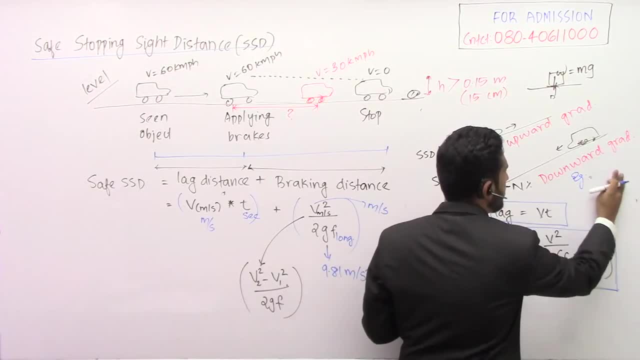 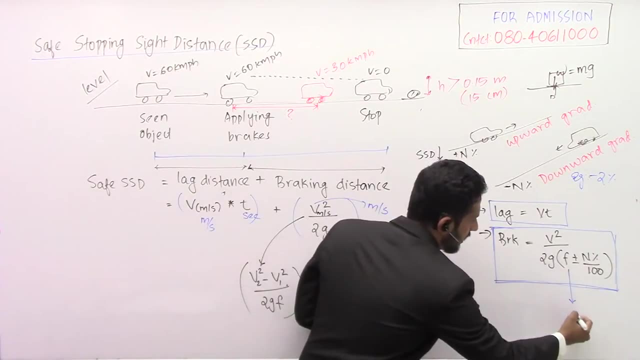 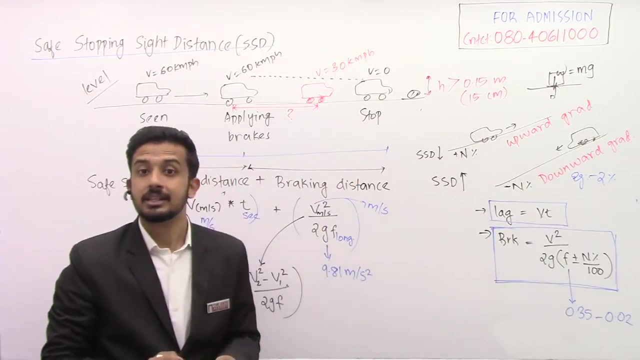 have given some minus four percentage, or let it be some minus two percentage, which means we have to make that. this is our guys, this is how we are multiplying. here is the one thing that we have to do with this: this bölt ke heck, that is going to be this one minus one, which is gonna be a. 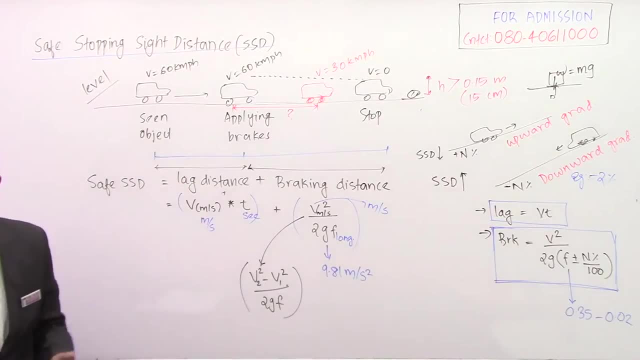 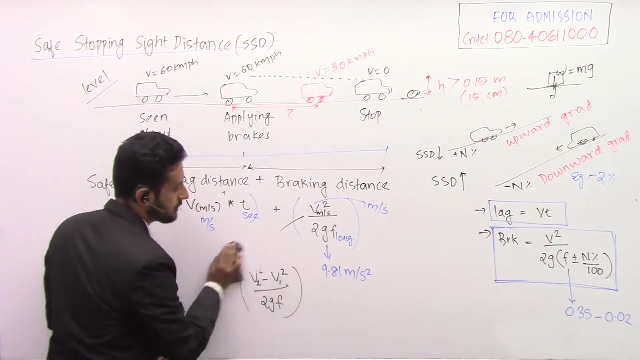 minus zero, point 15 and minus one. ok, so what that means is fordi. that means, while substituting, see what will be the f value. suppose let it be some 0.35 minus 0.32. this point also: v1 square minus v2 square. suppose if they are giving you a term called as breaking, 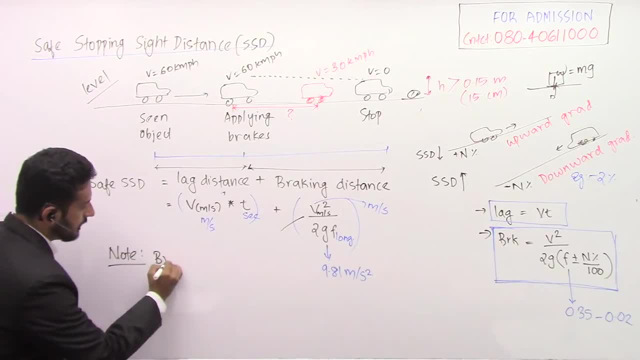 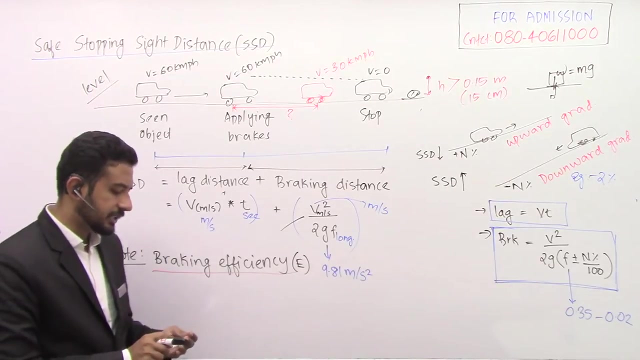 efficiency. you can write it as a note if they are giving some breaking efficiency. see what you mean by this breaking efficiency. i'm just denoting with a letter e, okay, any letter. you can give any notation what you mean by this breaking efficiency. if your brakes are 100 percentage efficient, 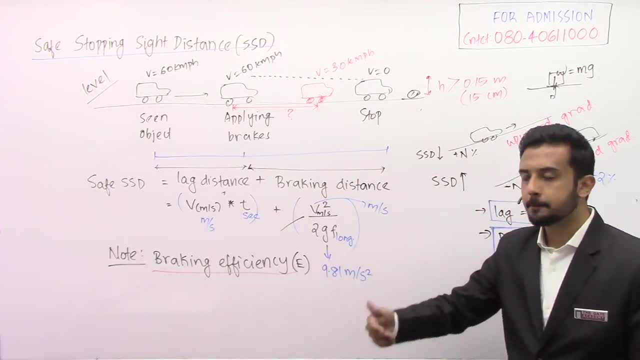 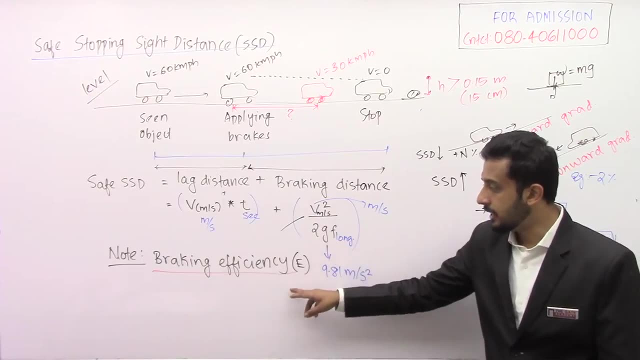 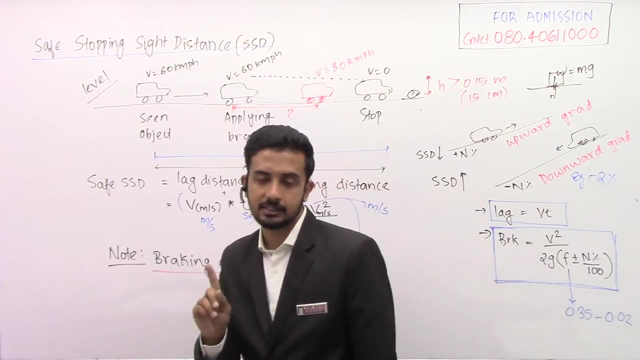 which means if you're applying the brake, your vehicle will stop within the distance of v square by 2 gf. it doesn't mean that braking efficiency is hundred percent, doesn't mean that whenever you're stopping, whenever you're applying the brake, your vehicle will stop. it's not the case. 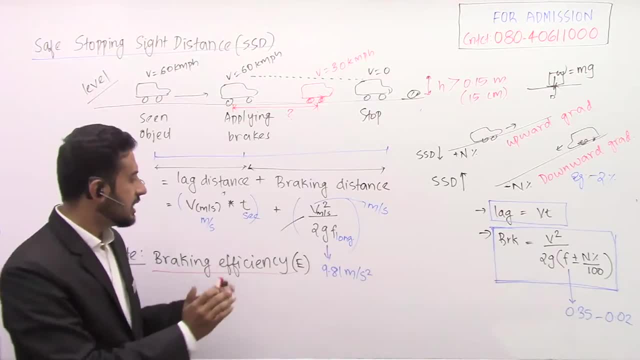 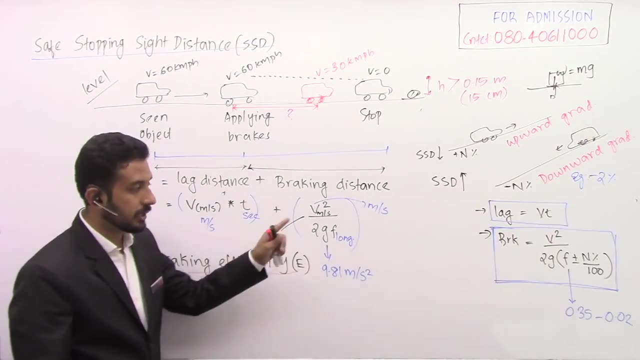 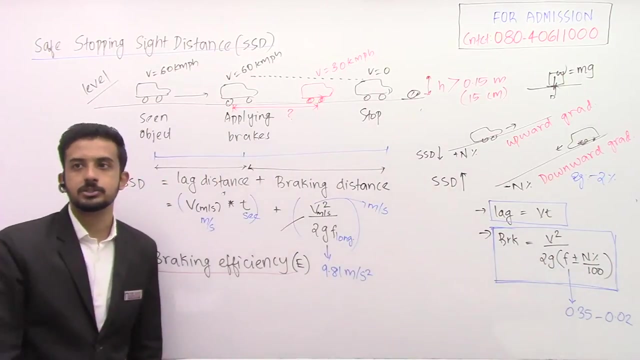 hundred percentage braking efficiency means if you're applying the brake after a distance of v square by 2 gf, your vehicle is going to stop. or if it is a gradient, after a distance of v square by 2 g into f plus or minus n by 100, your vehicle is going to stop. 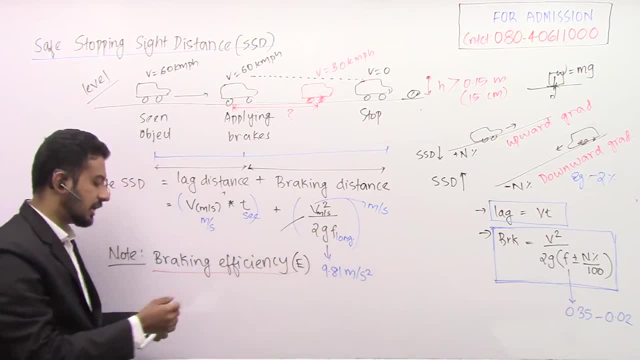 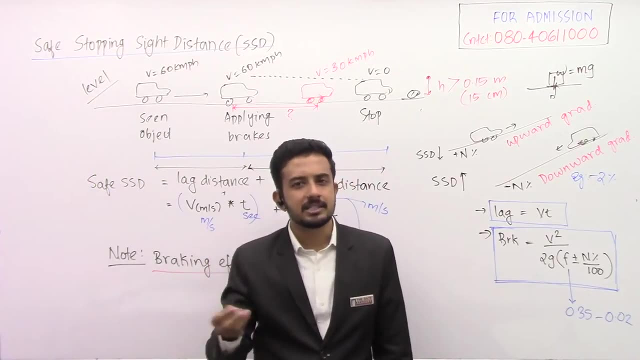 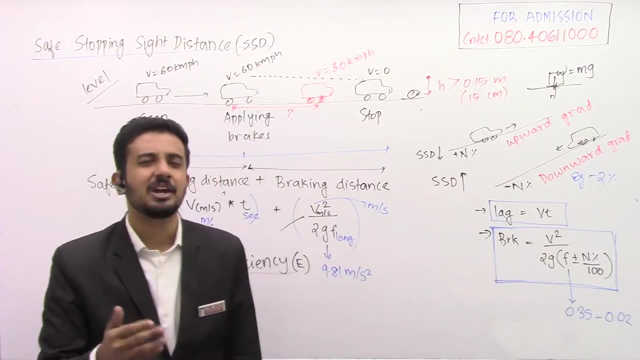 okay, so exact same value you will get if the 100 percentage efficiency is there. see, definitely, if you are using your vehicle, if the brakes are worn out after some period of time, what happens? even if you are applying the brake, your vehicle may be simply going on right. you might have used the. 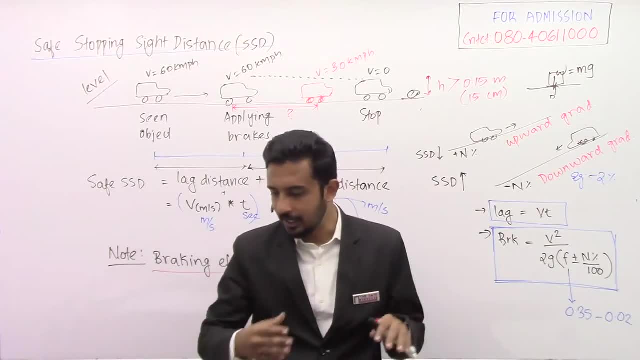 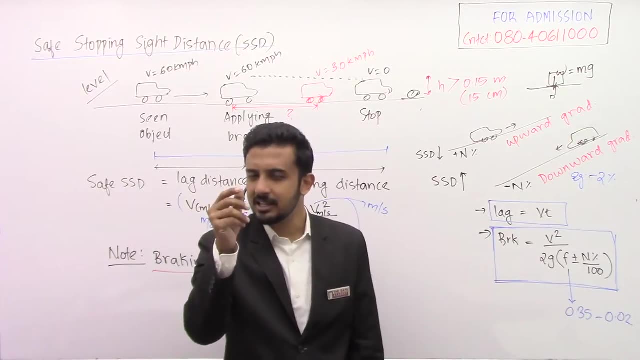 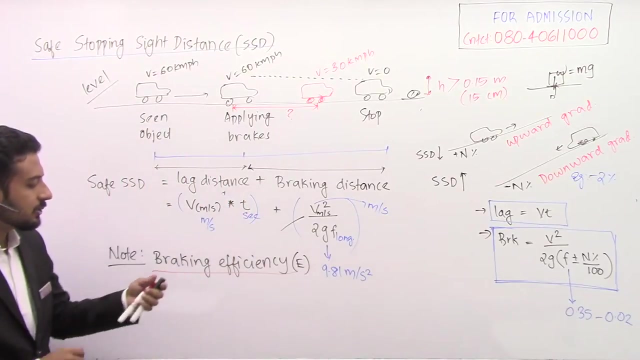 cycles now in childhood. so if you are applying the brake still, your cycle may be moving. why it is happening? because of the brakes. that thing has already gone, which means the braking efficiency is less. if it was efficient, then within some shorter distance it may be stopping. now the 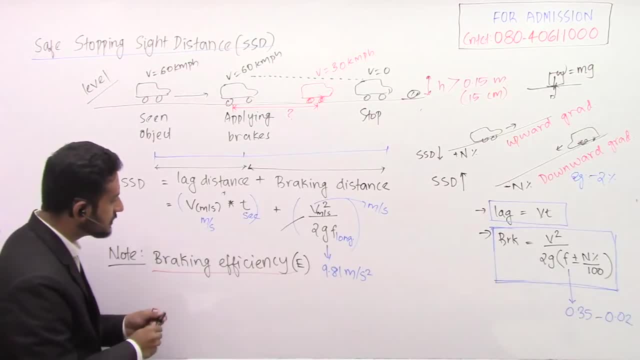 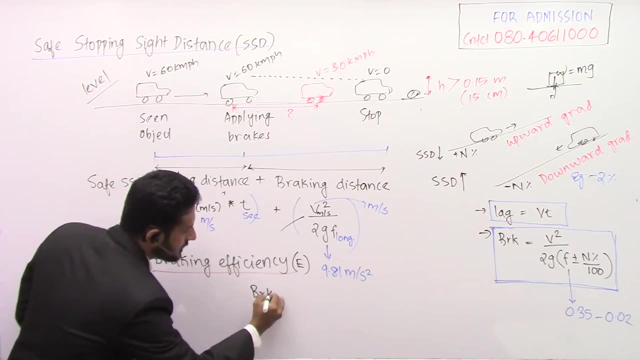 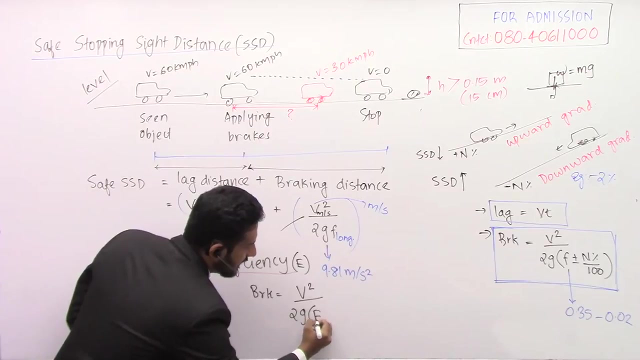 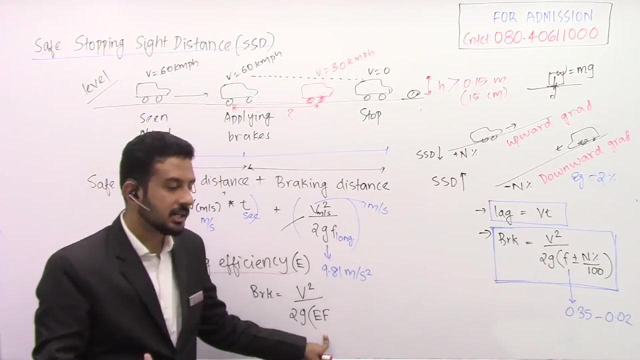 braking efficiency is going to decrease. yeah, very good, abhishek. so if they are giving you some braking efficiency e, the lag distance is same. the brake distance is going to change. what will be that braking distance v square divided by 2 g, into e, f, the frictional value if the freight is the braking diff efficiency is 100 percent. 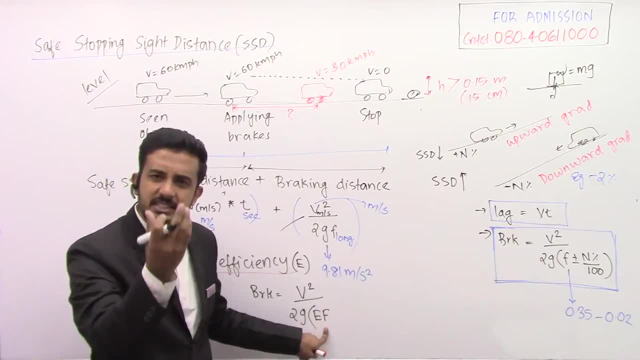 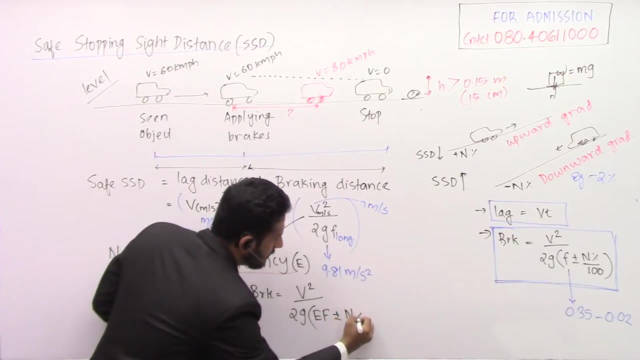 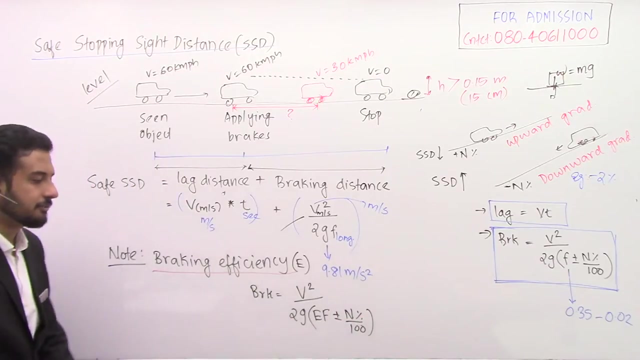 you will get the complete friction. if the braking efficiency is less, that friction that you are going to get is less right. so it is e into f. in general sense, i am writing plus or minus n by 100. if it is a level road, n is 0. so it will be simply e into f. only now, what will be the lag? 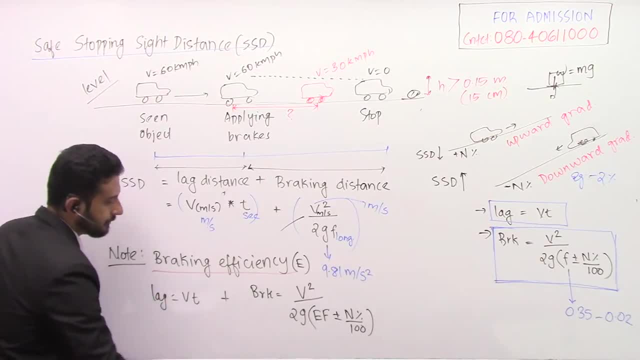 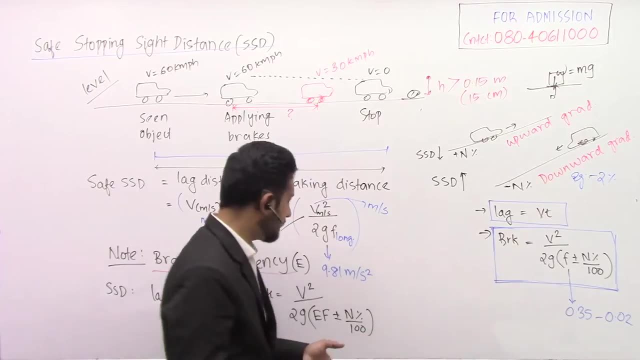 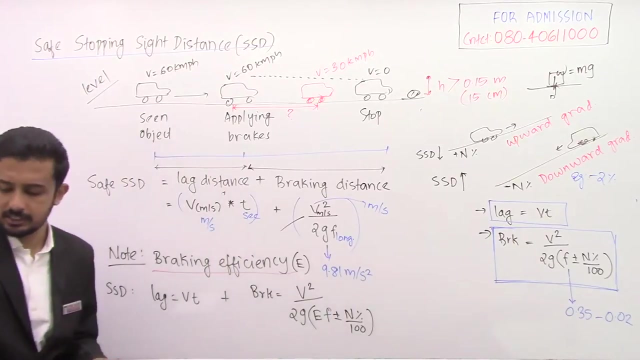 distance. lag distance is same vt, so if you are adding this, i will be getting my stopping sight distance okay. which means, suppose the coefficient of friction- this is not capital f, this is small f- coefficient of friction, capitalist g generally denote for frictional force. okay, see what it. 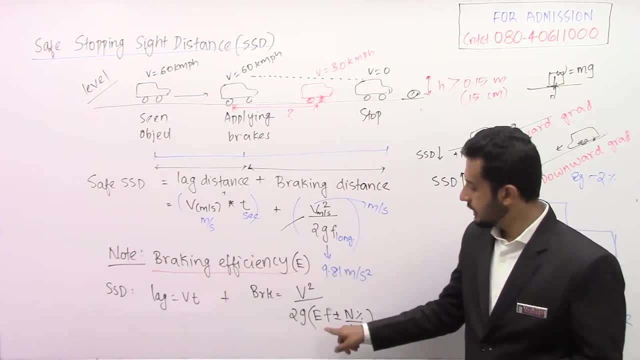 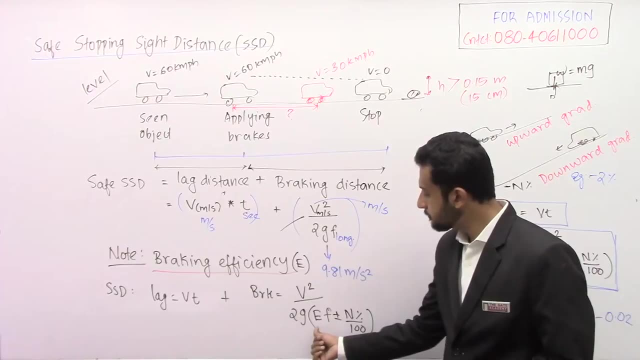 actually means. suppose hundred percentage of friction is equal to the frictional force. okay, so if it is 50 percentage efficiency, the small f value is some 0.4. then if it is 50 percentage efficiency, finally it will be, efficiency is 50 percent means means 0.5. so 0.5 we have to multiply. 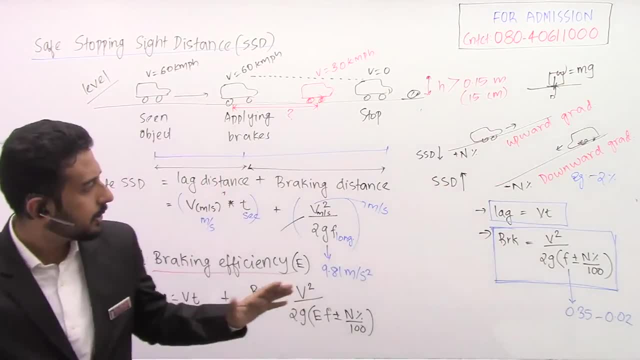 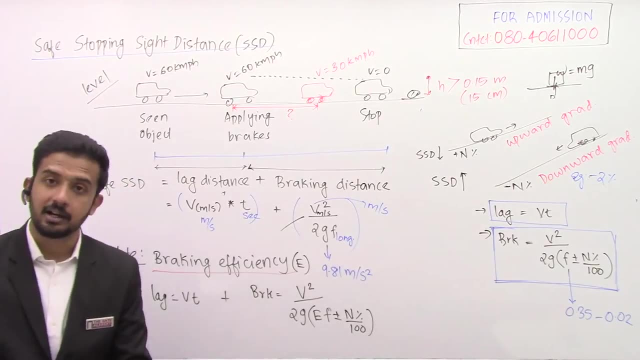 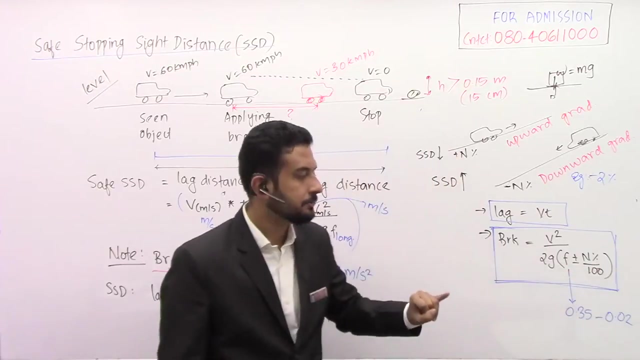 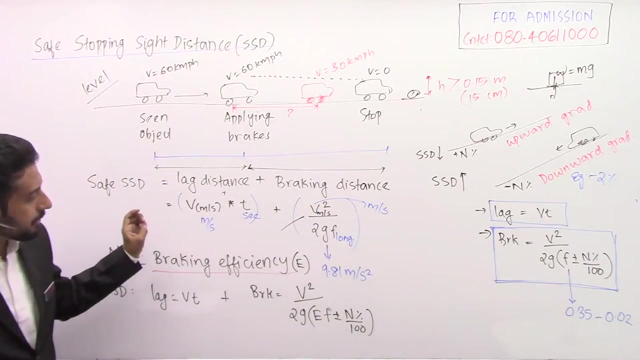 with the coefficient of friction. okay, so i hope you understood those concepts of stopping sight distance. so let's uh, do some questions for the better understanding, okay, so which all points you should remember here you have to substitute in terms of decimal and decimal and decimal. one point. second point, you should substitute the value of speed in meter per second, and the third. 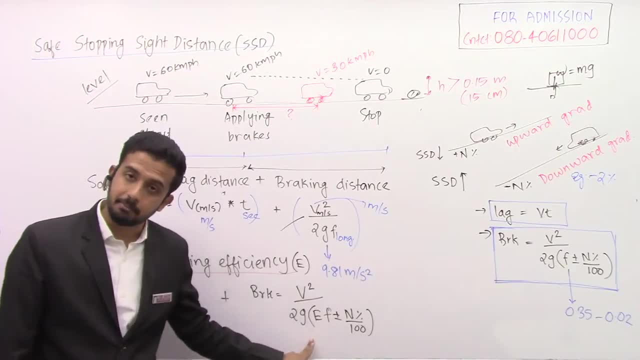 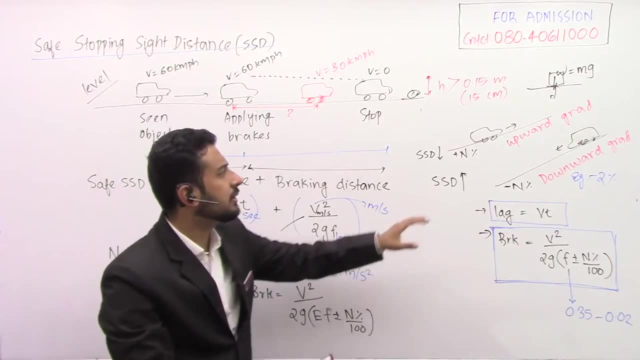 point: if they are giving some efficiency, you have to use multiply the efficiency with the f value. okay, so those are the points you should remember. also remember these things. see, they will not give these conditions under 15 centimeter. that is for your knowledge. i'm telling who has given that. 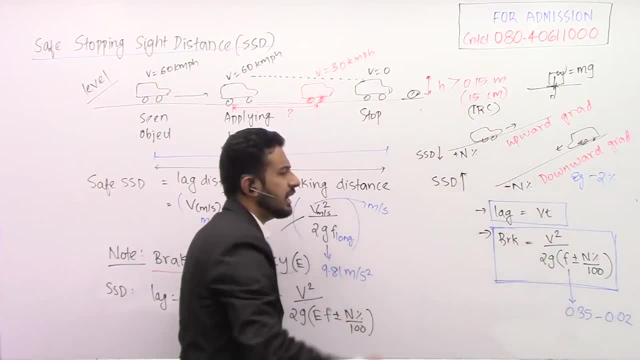 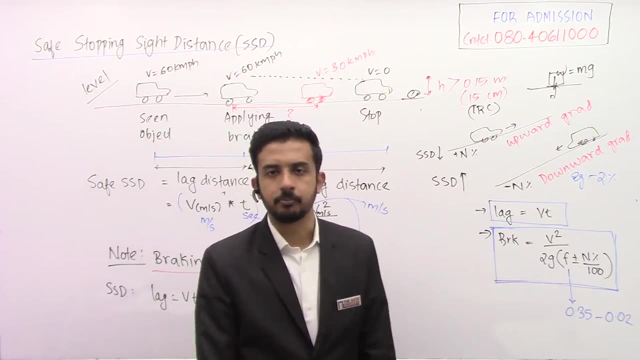 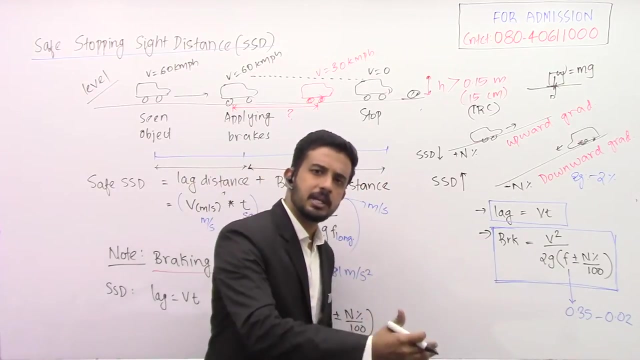 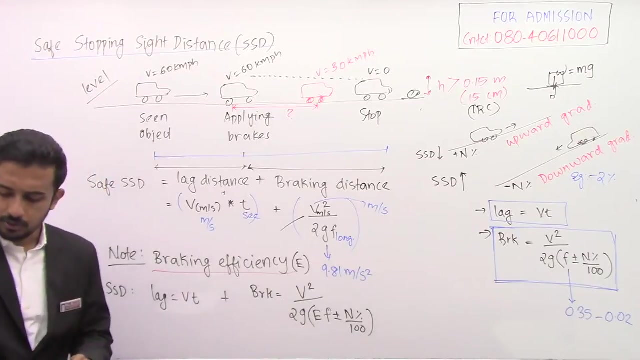 it is given by irc. irc has given one more term. see, just just imagine you're riding your vehicle. your brain is taking some time. will it be the same time my brain is taking? definitely not. maybe some fresh driver is there, maybe some experienced driver is there. definitely, the value of reaction time is going to change, right this part. so they. 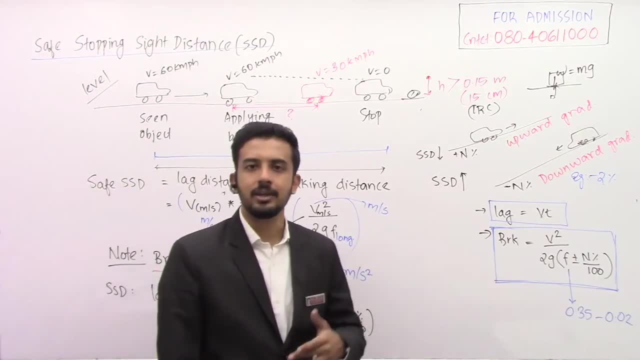 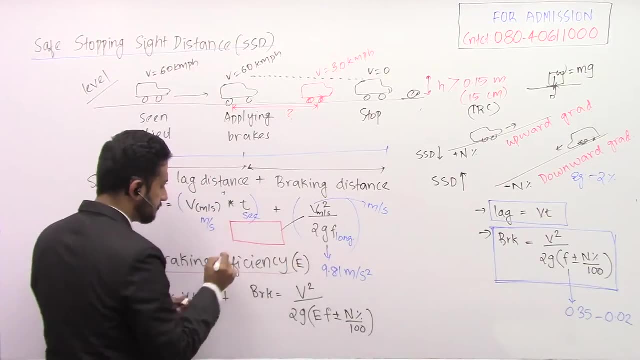 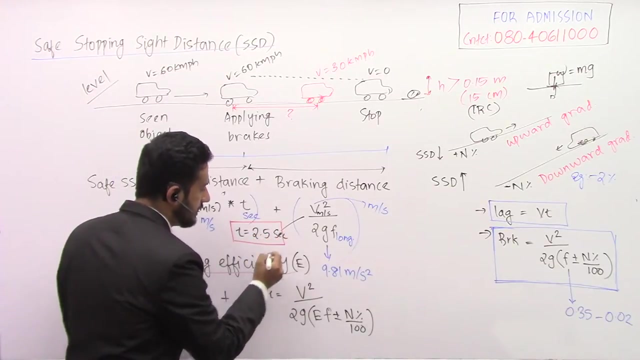 will give some values in the in the question. whatever value they are giving, take as it is in case. if they are not giving, we have to take a value of t. that is the time. t is nothing but 2.5 seconds, as per piev theory. irc has given a reaction time of 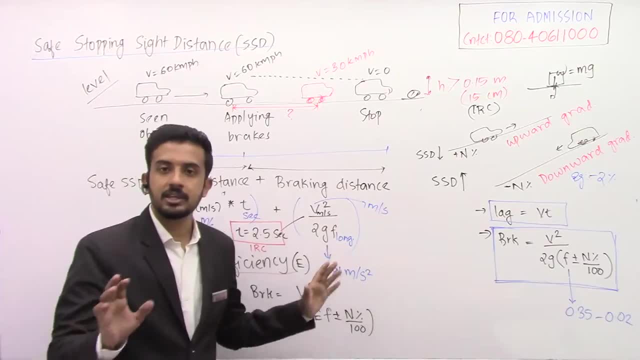 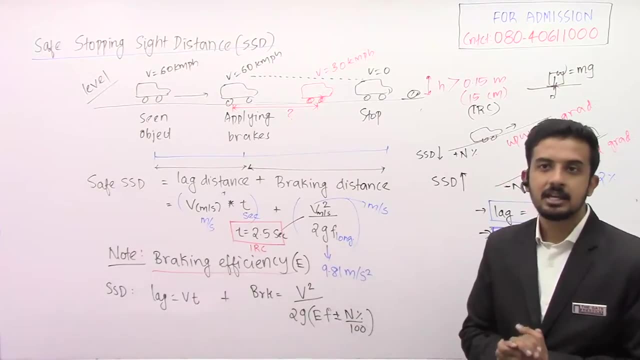 2.5 seconds. same is the case if they are giving some value: 3 seconds, 2 seconds, 2.4 seconds, 2.8 seconds, 5 seconds- take as it is in case. if they are not given, then take 2.5 seconds. this itself. 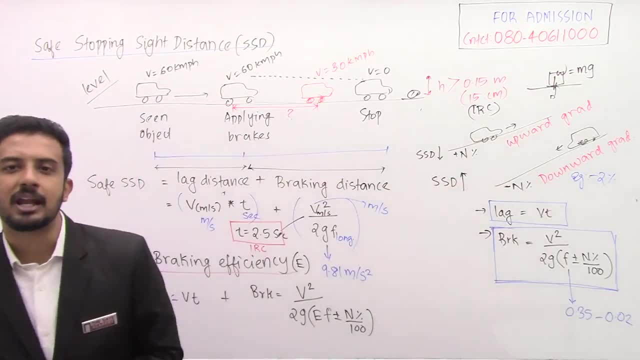 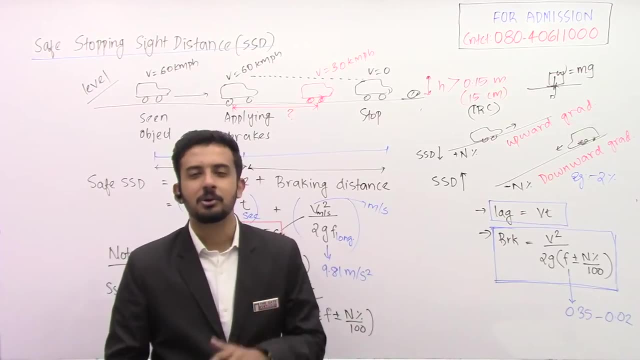 is a previous gate question for one mark. i'm going to tell you that if you are giving a value of t. one more interesting thing: they have asked a two marks question from this concept. you want to know what is that? what is the equation for breaking distance on a gradient? four options were there. 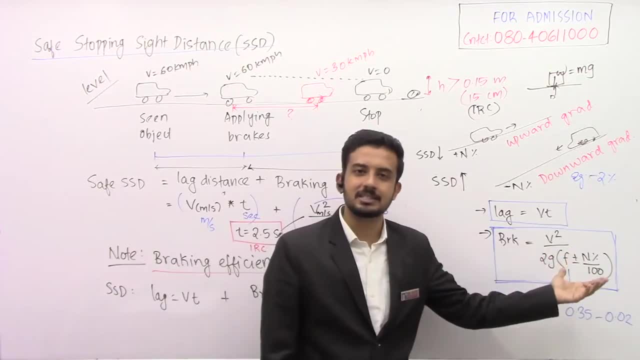 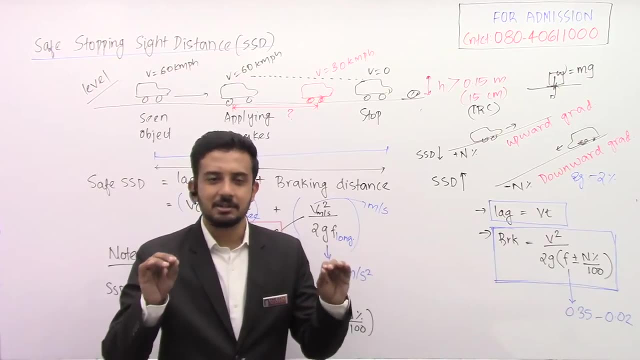 v square by 2 g f. v square by 2 g f plus n by 100. v by 2 g f f, something like that. so some values they have given simply, simply the equation they have given for two marks from this particular thing. okay, so. 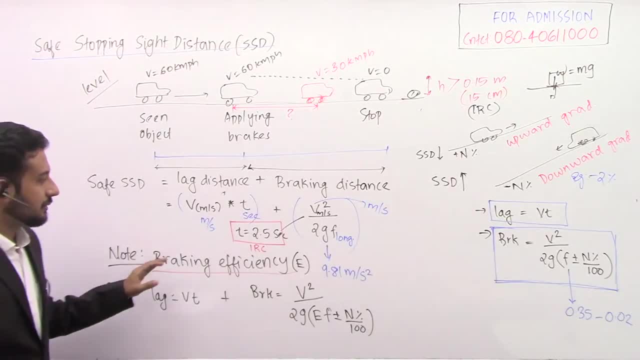 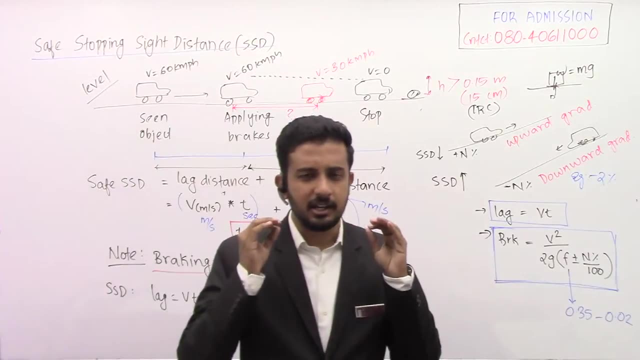 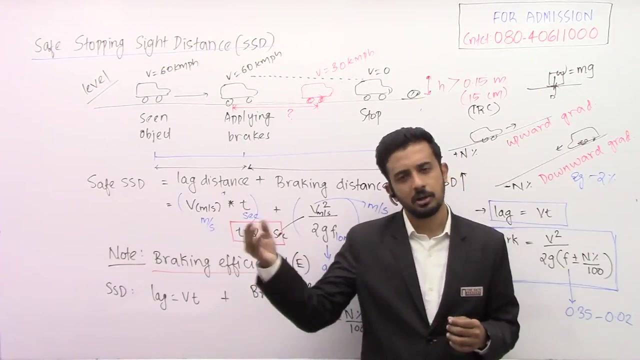 that means right now. any way you can get the value. which one you are asking? which is maximum or minimum? this is, this is actually an average value. if an ideal driver, maybe someone, is having good exp, he may be taking only one seconds or 1.2 seconds or maybe something less than that. 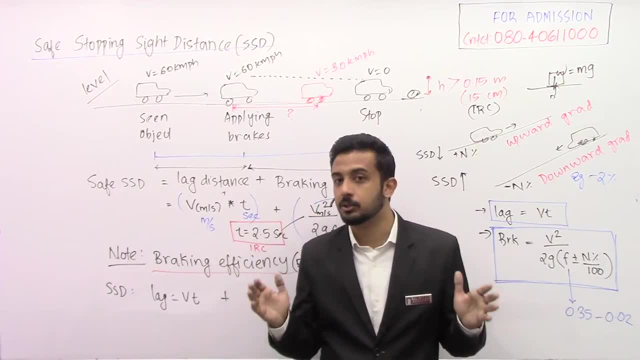 because he or his brain is having enough exp on the road so he can make decisions first. or he is a good driver, means while driving he is concentrating only on driving, suppose some other. if i am driving, i have only 1.2 secs to work. okay, if i amوجienne, i have a speed of 8.5 seconds. when i drive? what happens if i am while driving? honestly, i need to make a good decision. why didn't you do point? because sometimes, when you try doing something and then get lost in the thing, you fit the problem, but this is not possible because the car doesn't do anything. 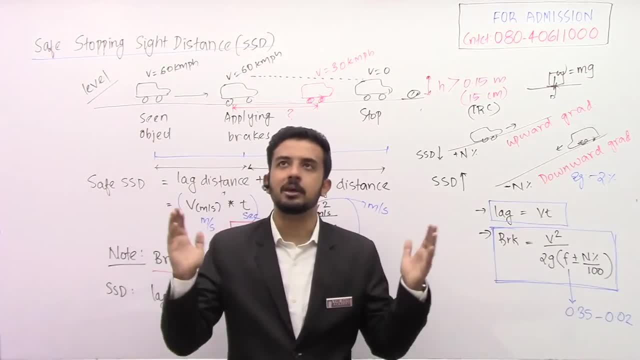 what is happening. so it is nowhere wherever you got your eneghrcam- some other drivers. he's not a good driver. you may be thinking something else. maybe you might have watched some movie. you may be thinking some scenes of the movie and you're driving. definitely is. 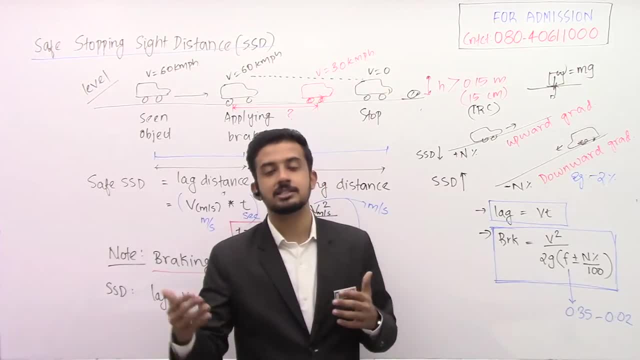 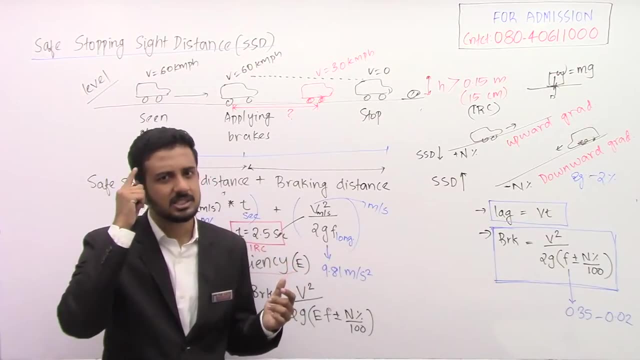 going to affect you, so you'll get some more time. six seconds, seven seconds. see, that's why accidents are happening sometimes. right, the drivers are not able to apply the brakes fast because his brain is taking more time, because he may be thinking something else, he may be tensed, something. okay. 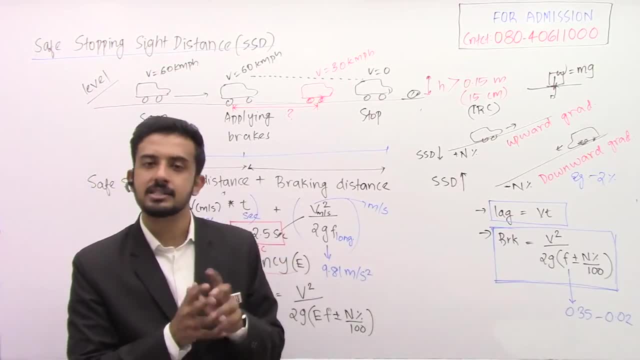 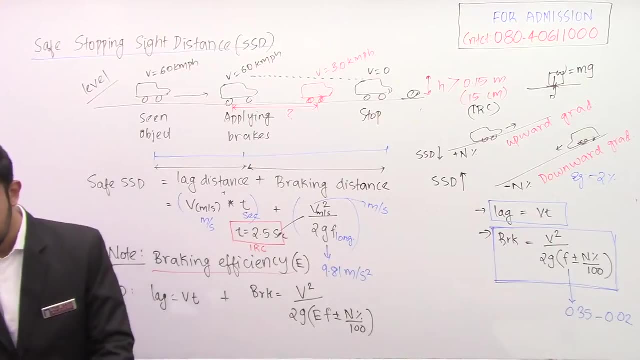 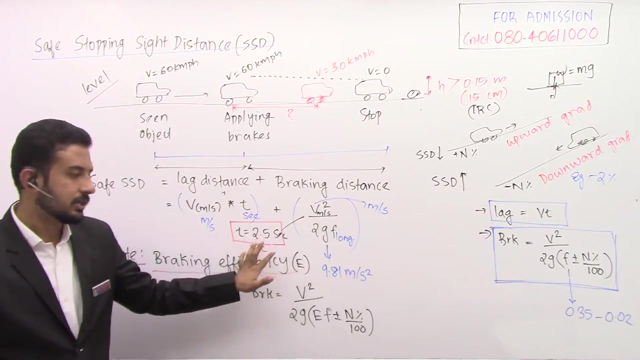 so this is actually an average value: 2.5 seconds as per irc. okay, if not given, then only take. it is: if they are giving some value, take as it is, okay. so i'm going to give you one question. uh, remember this should be in meter per second. if not given, then only 2.5 seconds, and the remaining values 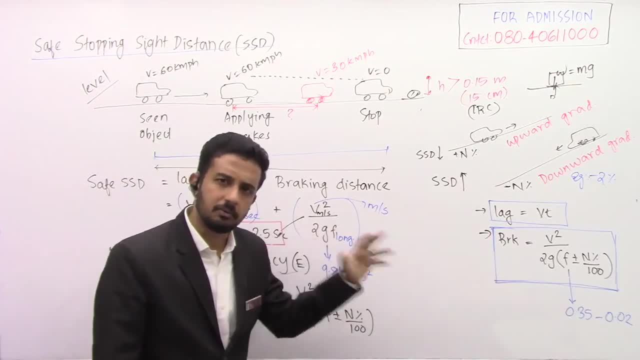 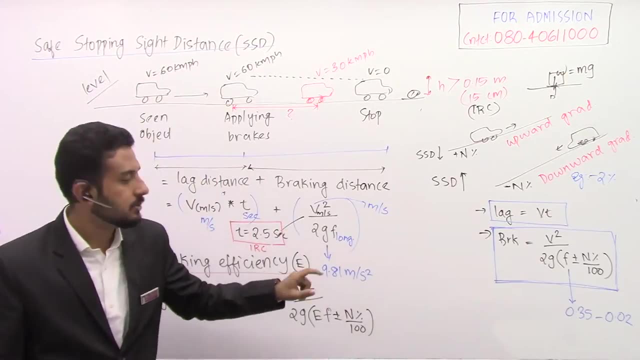 this should be coefficient of longitudinal friction. whatever value they are going to give, take as it is, they will be giving the values. okay, because it is in the range. now there is no per particular value, so they will be giving the range and all. so take down a question i'm going to give. 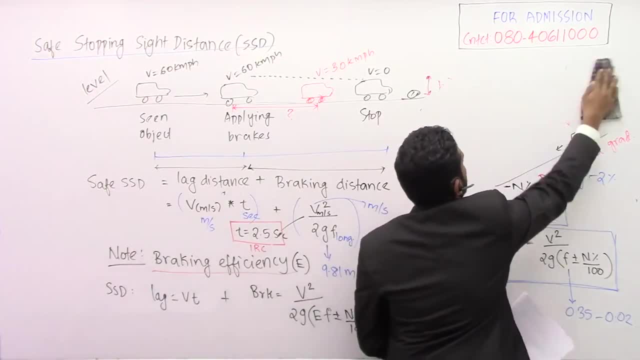 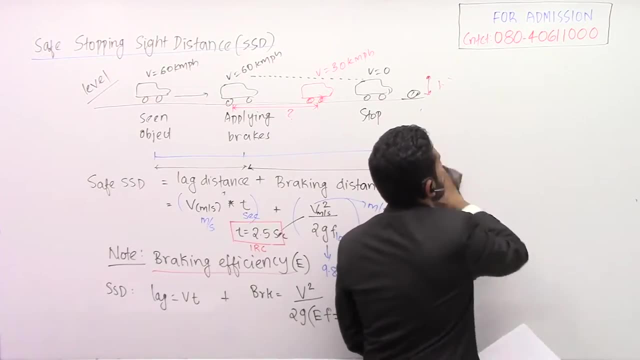 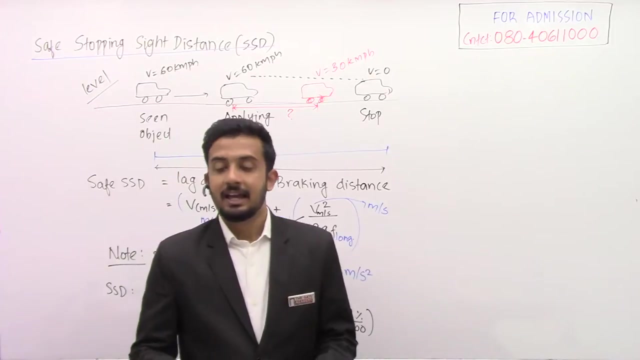 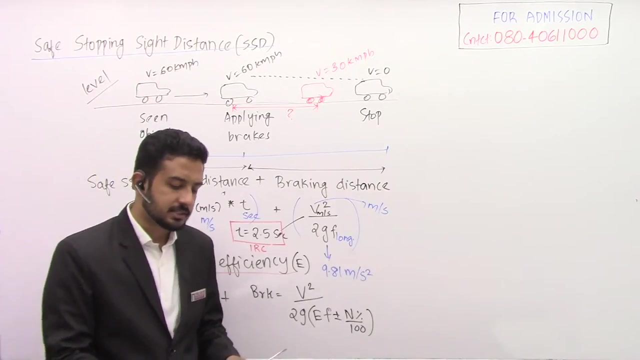 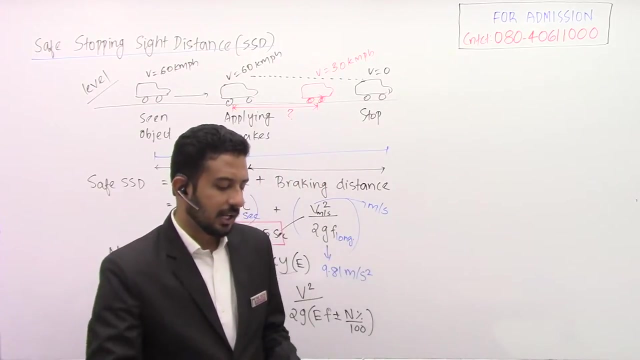 you some question? okay, i'm giving. i'll be writing the things here while i'm reading, right? so yeah, only few minutes. we are having no right, no problem, just write simple, simple questions. take the first question: calculate the safe stopping site data distance on a level road. use some short, short words. only calculate the safe stopping side. 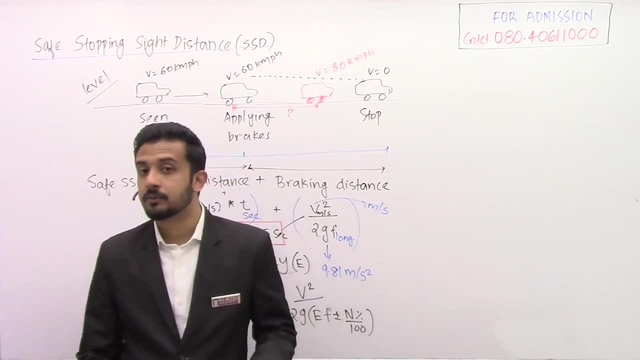 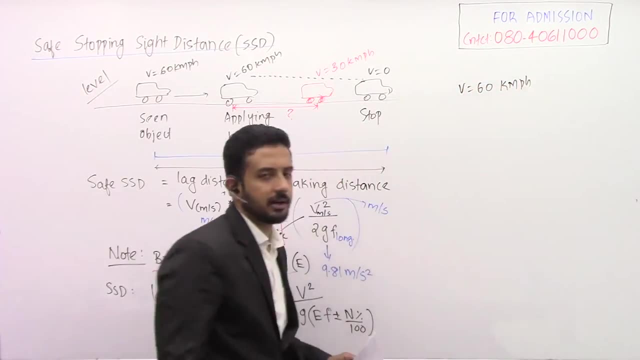 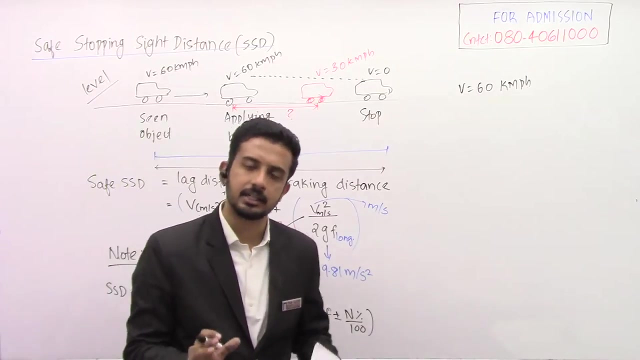 distance on a level road for a design speed of 60 kilometer per hour. for a design speed of 60 kilometer per hour. okay, see what you mean by design speed. design speed is nothing but the speed at which the road is designed. that's it. so the vehicle may be coming at the design speed. 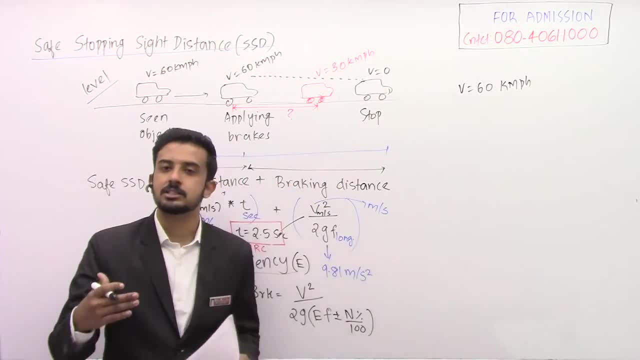 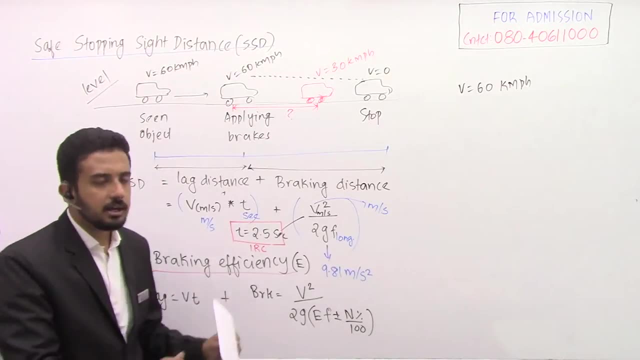 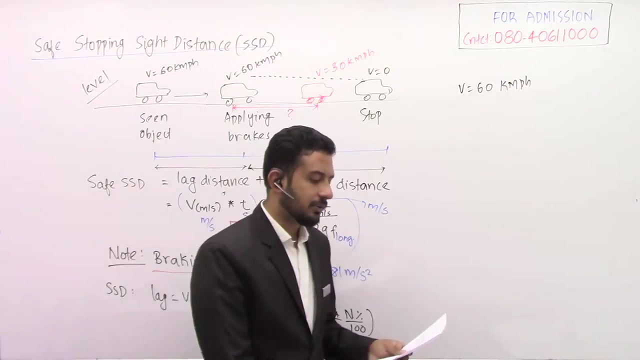 or let's learn that our intention is the vehicles should be coming less than design speed. okay, but simply, if they are giving the design speed instead of giving the speed of the vehicle, we'll be taking as the speed of the vehicle. okay, so design speed is 60, so calculate the SSD on a level road for. 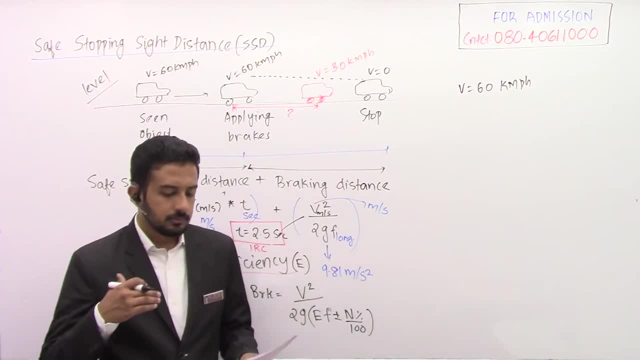 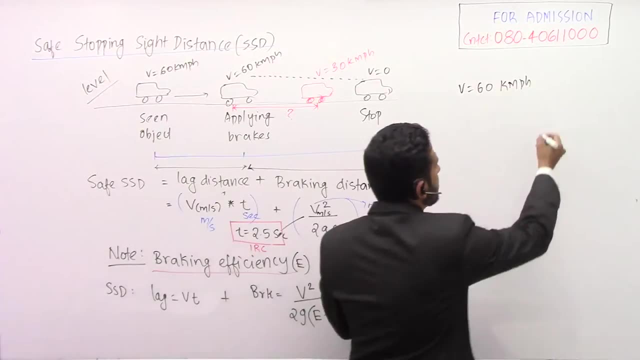 design speed 60 kilometer per hour and mark in the bracket. you can write: assume the coefficient of friction is equal to 0.36. coefficient of friction here as n is equal to 0.36 and 90 liberties is. that value is also the value. 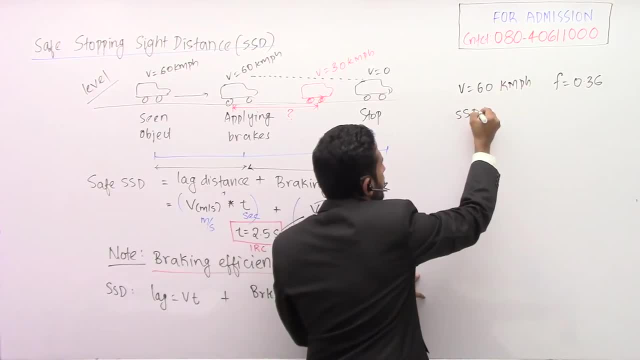 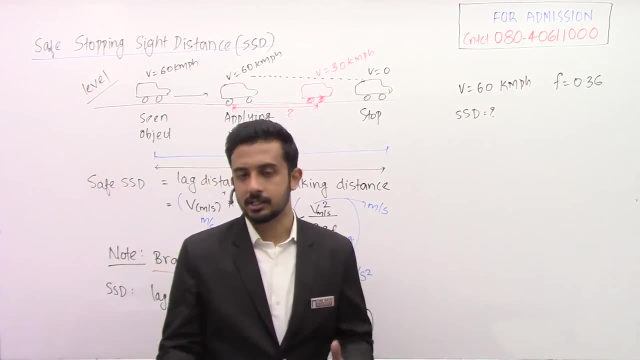 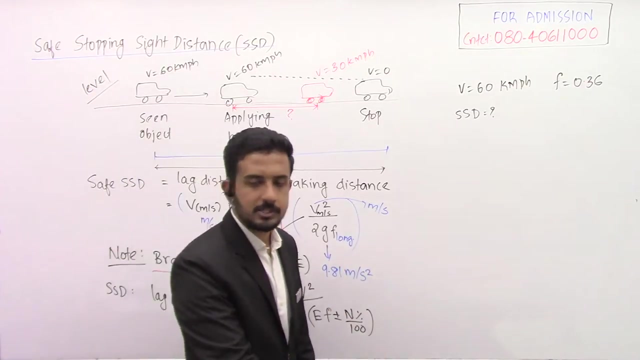 coefficient of friction is 0.36, so calculate the stopping side distance. do fast. if they are asking such a question. definitely it will be for two marks. okay, many times they have asked the question, so you can practice those previous questions also. some questions will be solving here also. 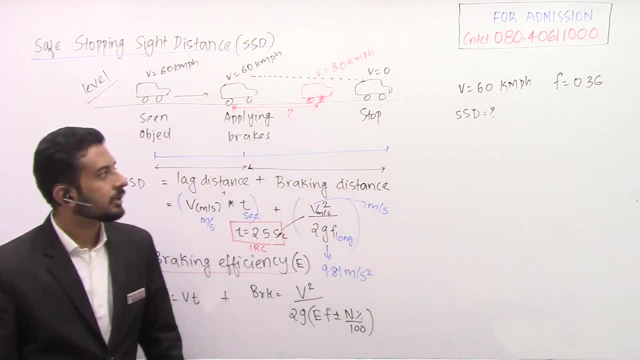 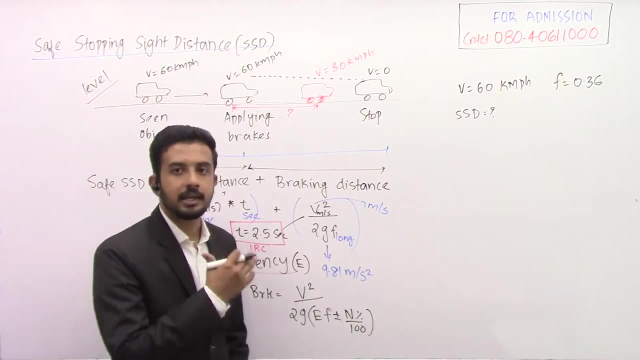 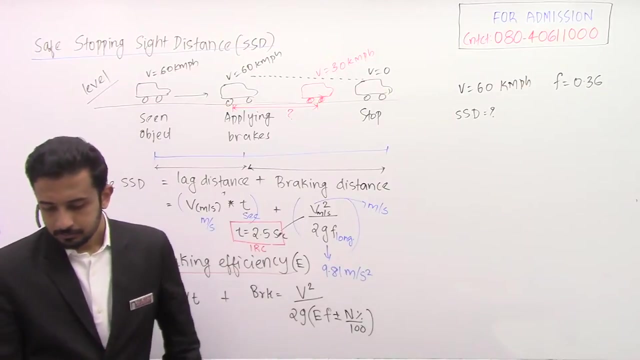 same type of question, they will be asking for two marks. so in this case they have not given the reaction time. then what you have to do, you have to take it as 2.5 seconds, because irc told: if you are not having the value, take this value. very good, devashish that speed is required for us. 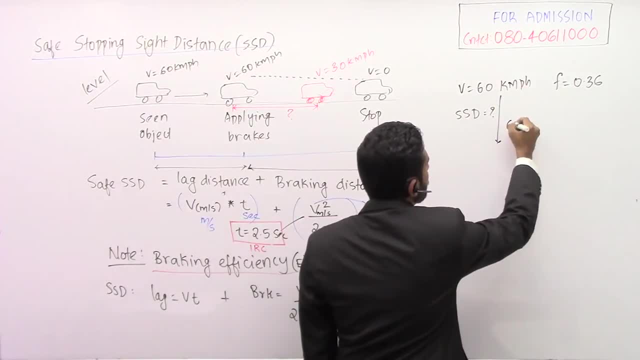 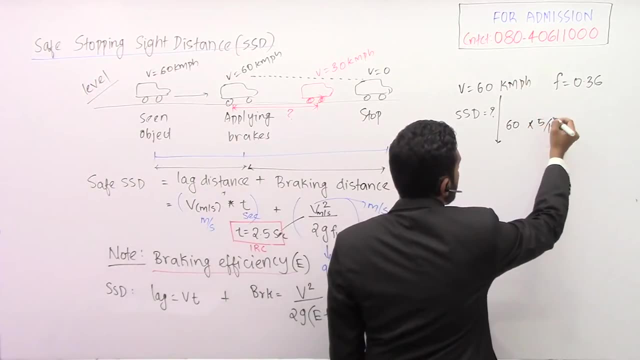 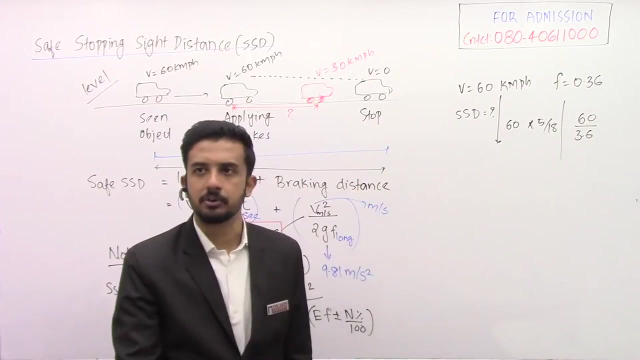 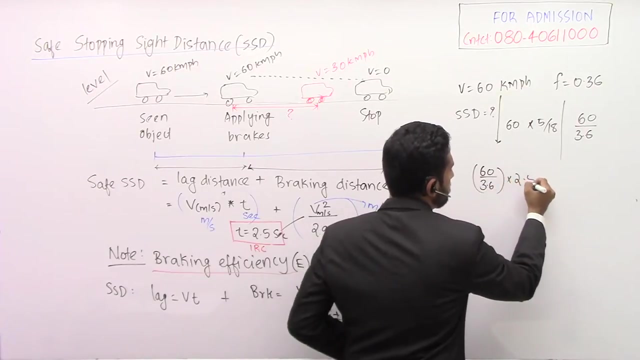 for the gate examination. what i have to do? first, we have to convert into meter per second, how to convert kmph into meter per second? you have to multiply by 5 by 18 or you have to divide by 3.6. this 18 by 5 is nothing but 3.6. so i have to divide by 3.6, so it will be 60 by 3.6 into 2.5 plus 60 by 3.6. 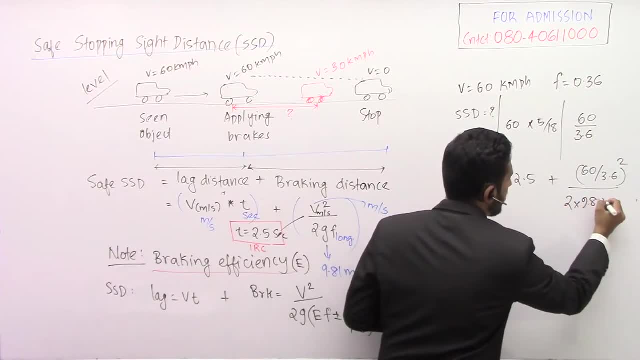 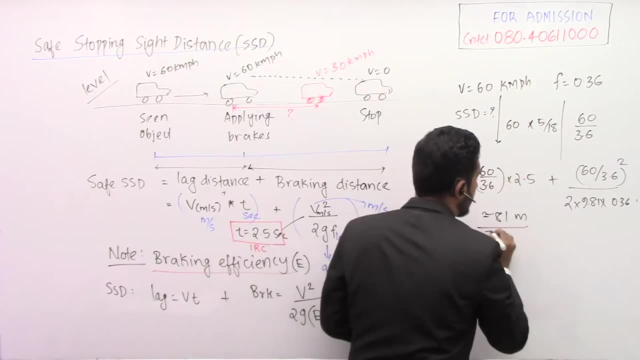 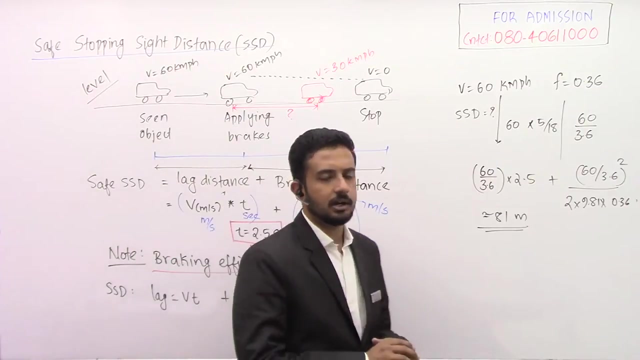 square divided by 2, into 9.81, into 0.36, how much it is? approximately some 81 meter you are getting now. so depends maybe. yeah, very good, very good. so you may be getting uh options sometimes or they will give a round round. 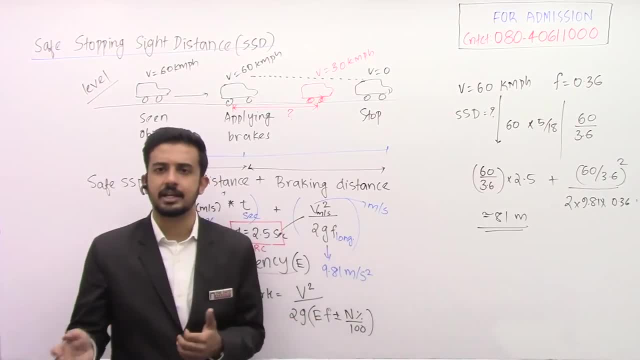 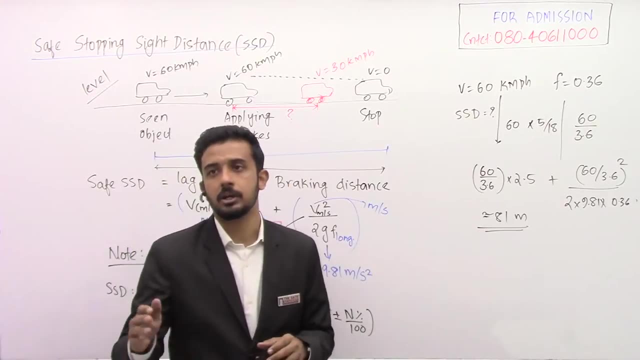 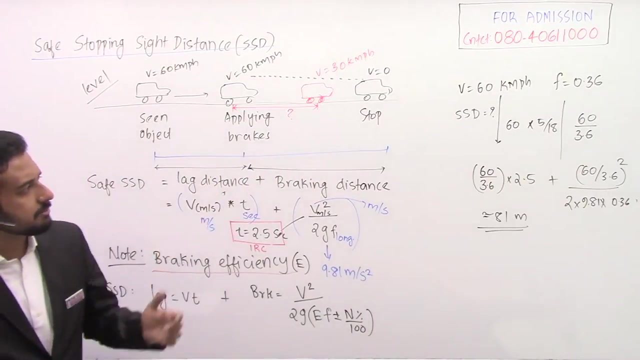 round to one decimal and all. then you can write that, whatever you are exactly getting, there will be some range, some 80.1 to 81.1, something like that they may be giving. no, it is 81 point something you're getting, so accordingly, a proper range they will be giving. okay, very good, so that is a simple. 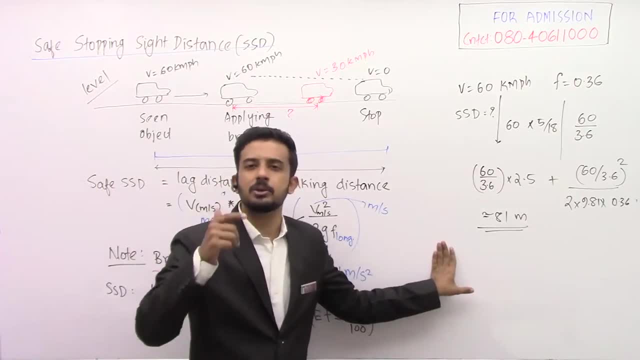 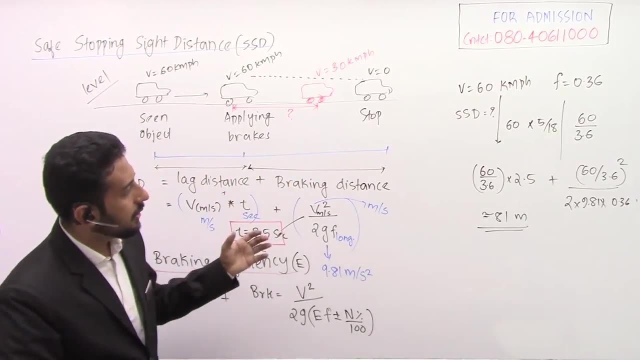 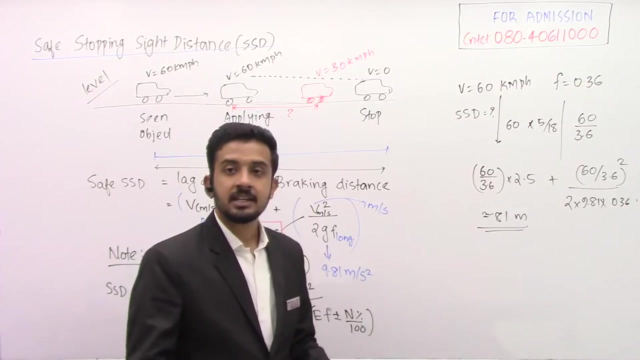 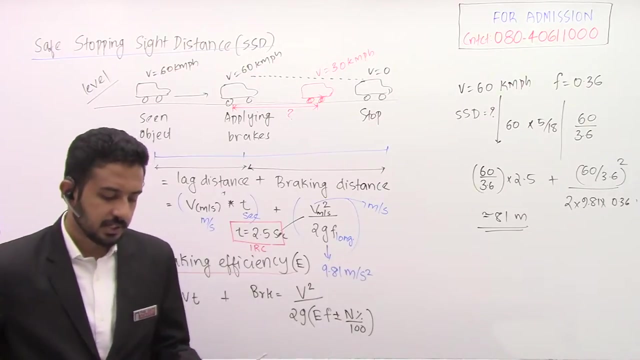 question. many times they are fast, such a very minute, simple question. many times okay, that two for two marks, either for one mark also. sometimes they used to ask: okay, now take the next question right. a decreasing gradient of three percentage. a decreasing gradient of three percentage is present. 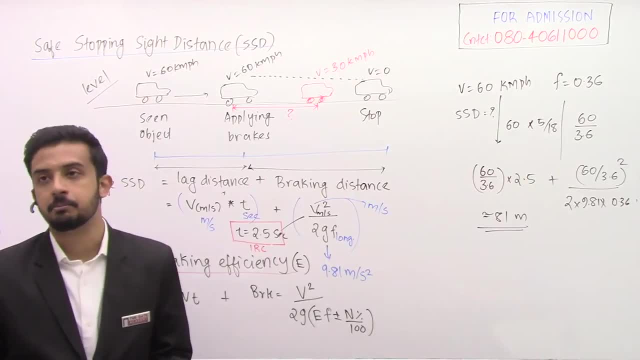 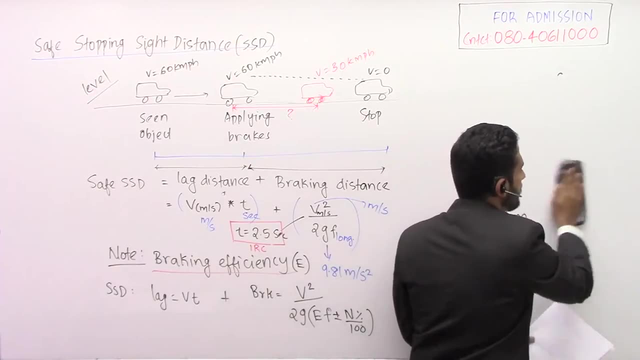 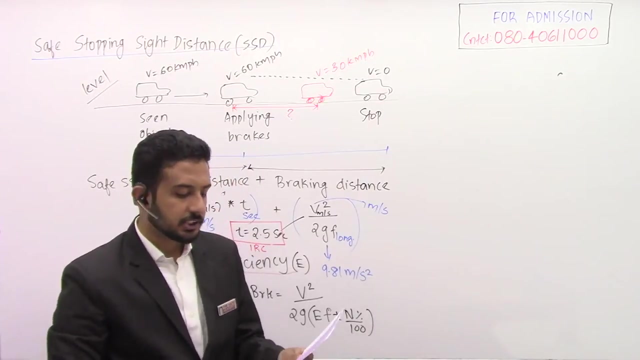 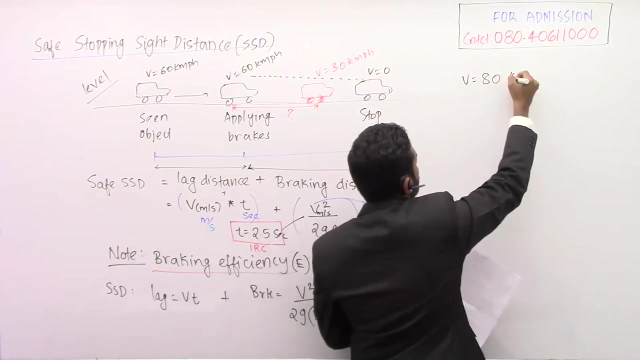 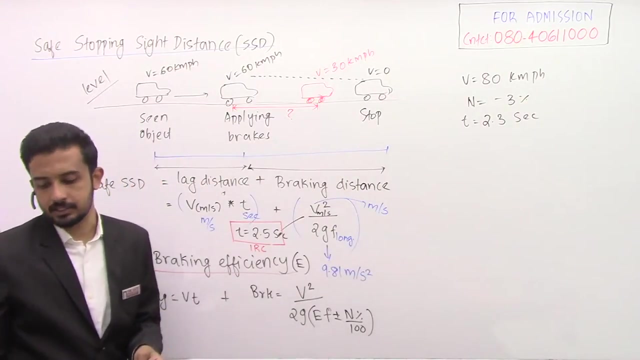 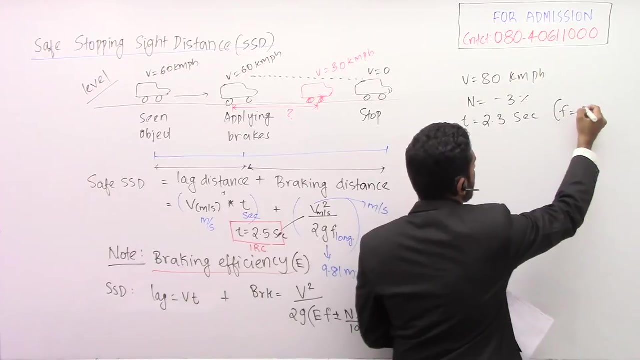 on a road of design speed 80 kmph. a three percentage decreasing gradient is there where speed of the road is 80 kilometer per hour. okay for a driver with reaction rate of 80 kmph. the speed of the road is Fe 2.3 seconds for a driver with a reaction time. 2.3 seconds for a driver with a reaction time. 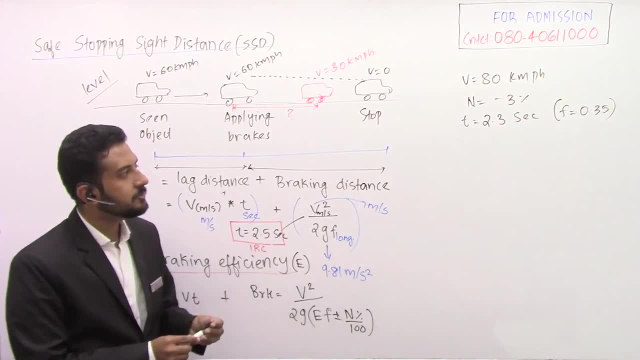 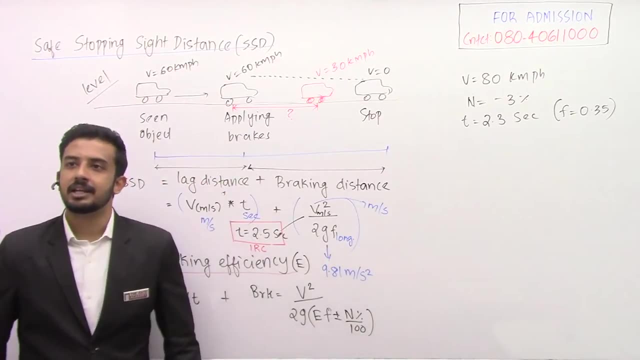 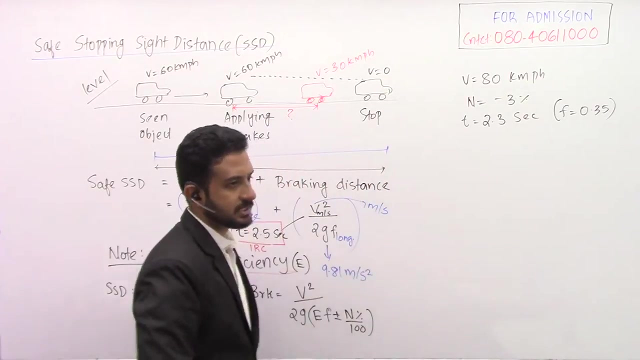 0.35. see what is this? 0.25, it is nothing but coefficient of 0.35. coefficient of longitudinal friction generally. reaction time: 2.5 seconds. yeah, why? because they are not giving the value in the question. in case, if they are giving, take as it is, most of the time they may not be giving because 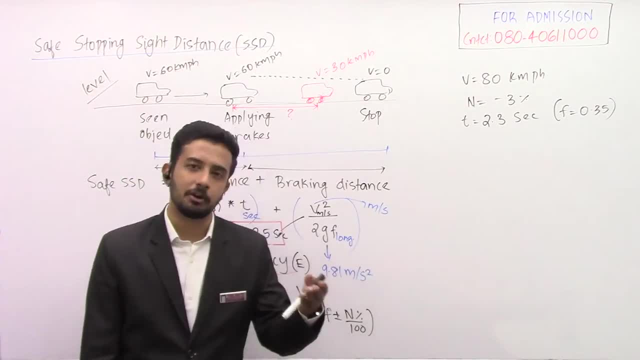 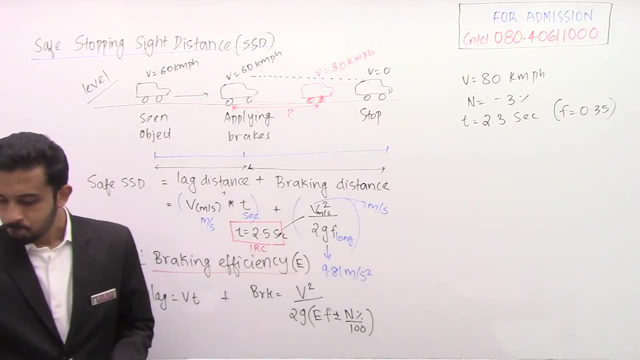 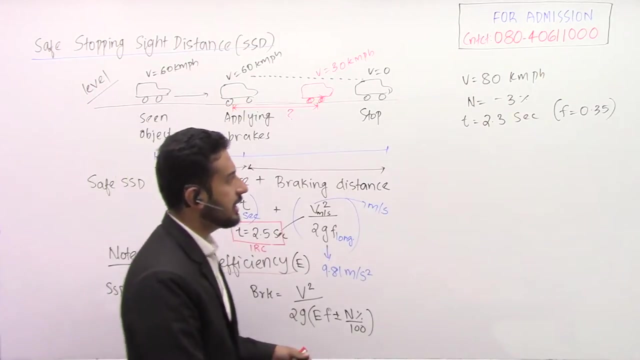 they are giving you two marks for this calculation, so you have to remember that 2.5, just for remembering that 2.5. also, they are giving some marks. that's why, okay, it will be approximately some 130 meter. very good debashish, better take, always take- the accurate value, so it will be vt. 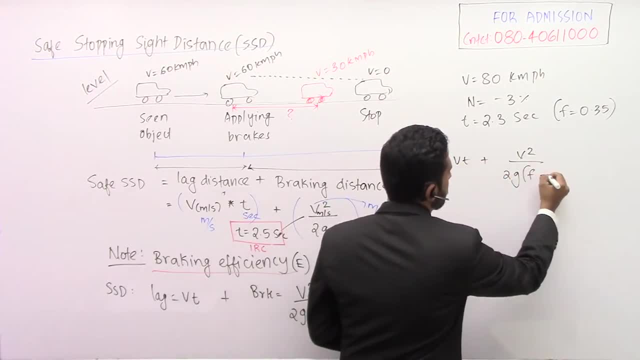 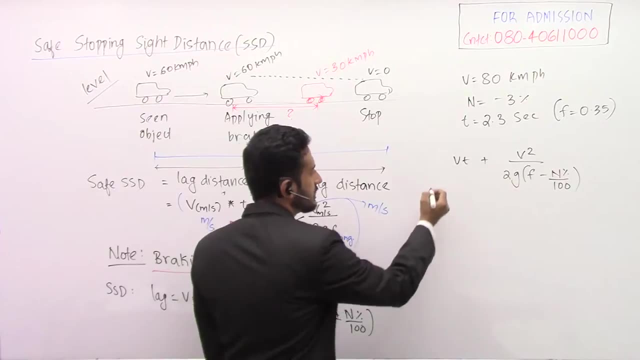 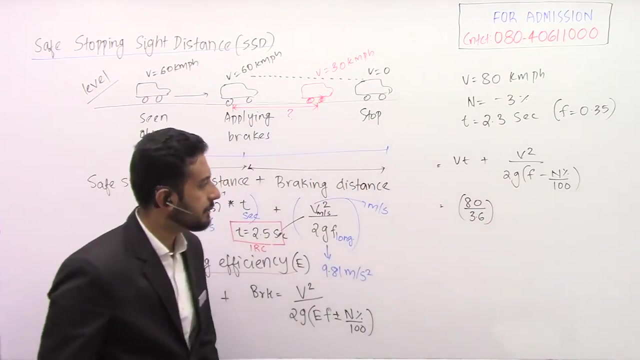 plus v square divided by 2g, f minus n percentage by 100, because it is a decreasing gradient. yeah, everyone do it. do it and tell me the answer. so first you have to calculate into 80 divided by 3.6. see, better, you use this 3.6 because don't try to convert that. see if you are converting 80. 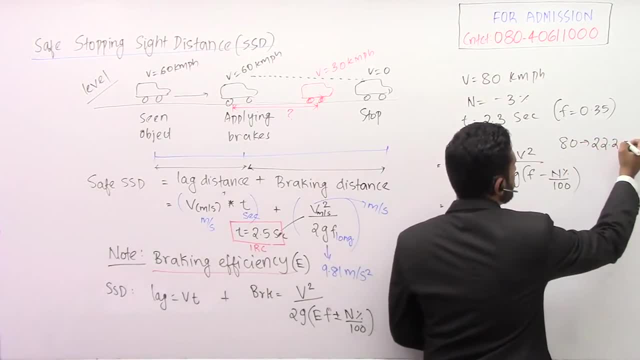 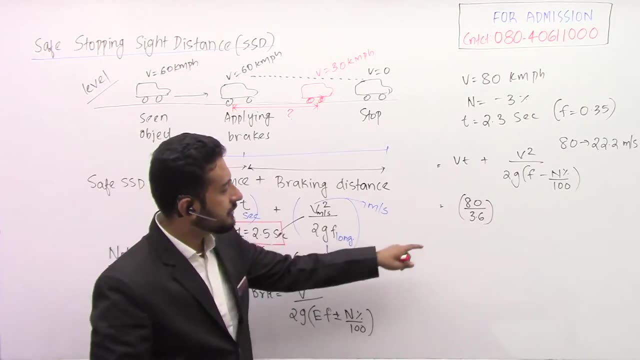 it will be around some 22, i guess some 22.2 meter per second you may be getting. so, if you are taking that simply 22.2 or 22.22, and if, instead of, you are taking 80 by 3.6. 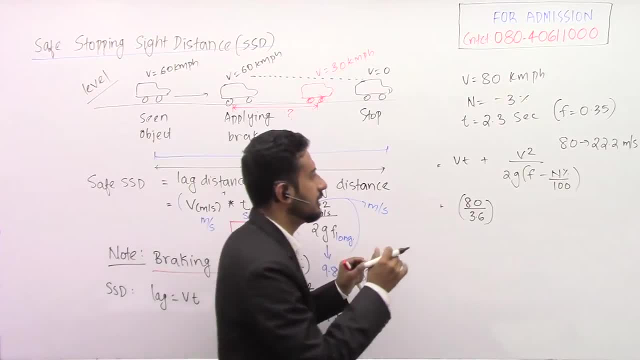 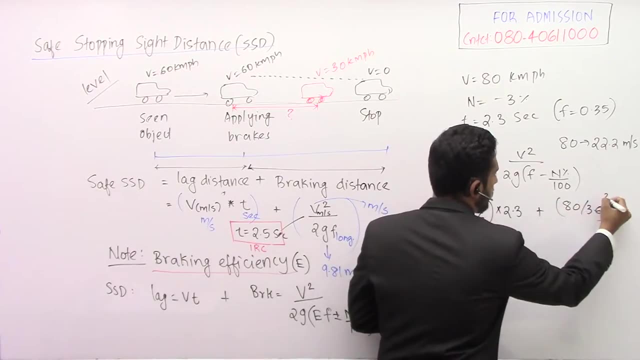 you are going to get the precise value, accurate value you are going to get okay. so better take something like this: so 2.3 plus 80 by 3.6 square, divided by 2 into 9.81, what is the value of f 0.35? so from 0.35 we are going to minus how? 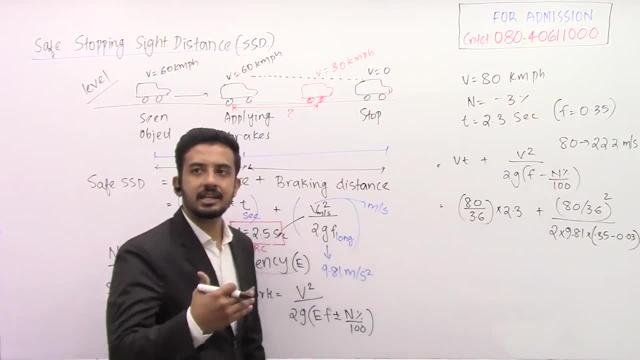 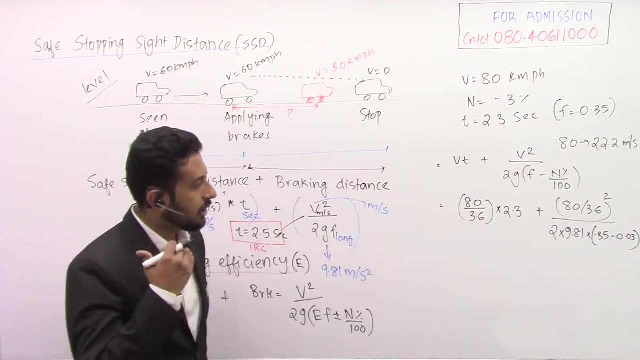 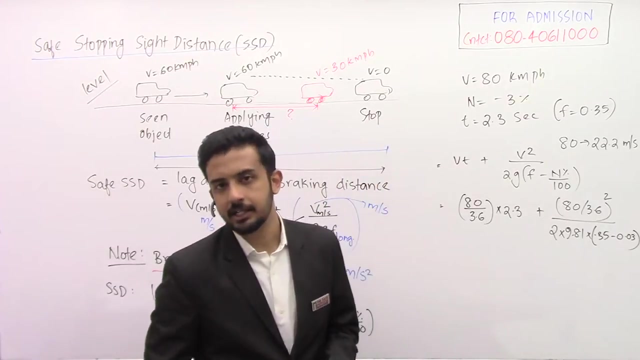 much, 0.03, because they have given it's a decreasing gradient. very good, i ignored the decimal value. better, don't ignore the decimal values. okay, always take the accurate value, because we don't know right what will see. if the options are there, it's fine for numerical answer type question. 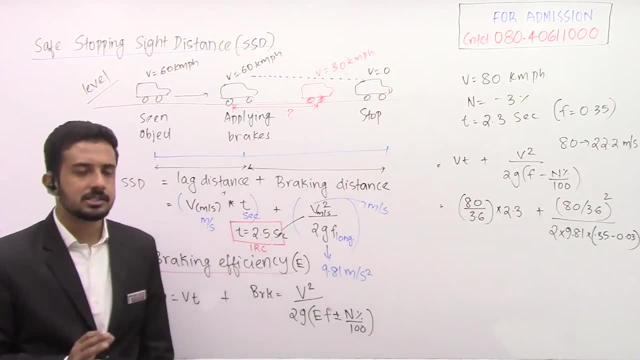 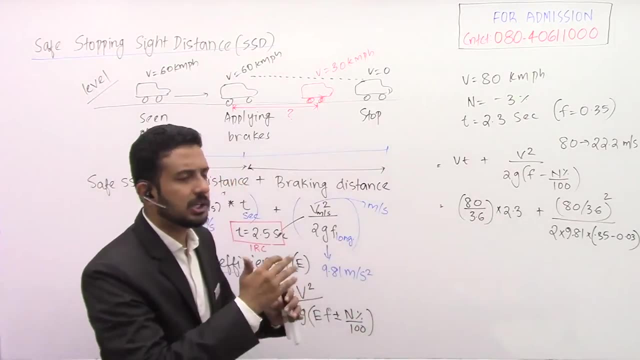 if it is there, better. whatever they are going to ask, um, give as it is. and one more thing: see, if you are taking simply 22 instead of 22.22 and all here, you are going to use it, you are going to square it. so some change. 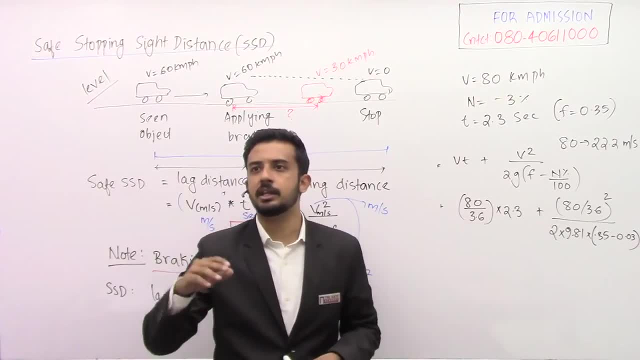 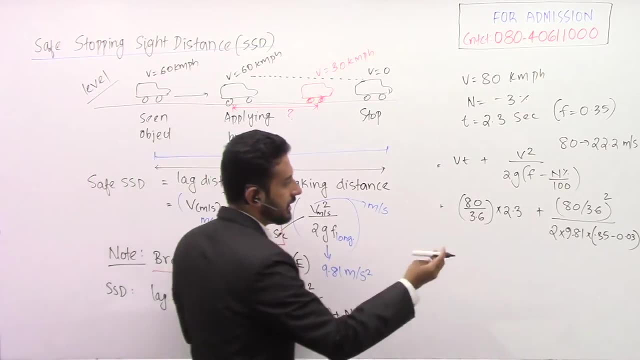 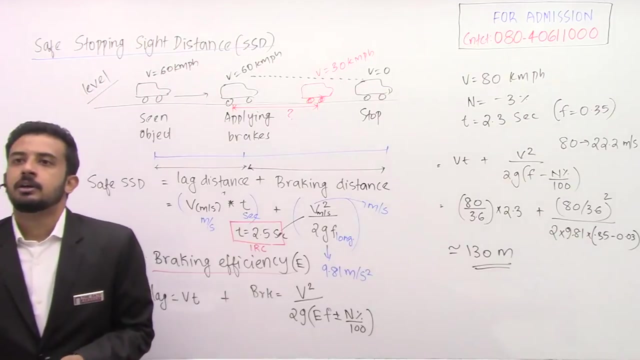 may be happening between 130- 130. someone is getting 129, something like that happen, so you may be getting some 131 point something, so better take accurate value. so, approximately, everyone is getting some 130 meter. approximately. sure, though, it's good class. yeah, thank you, sunil. thank you. 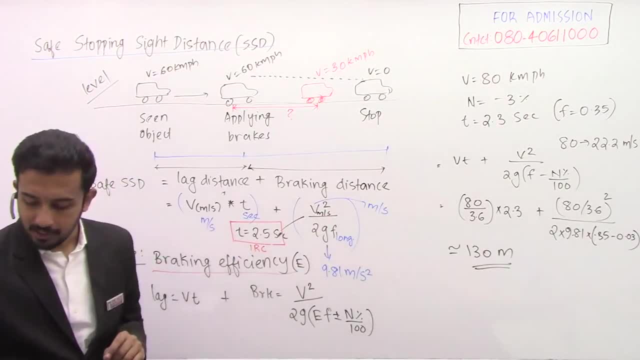 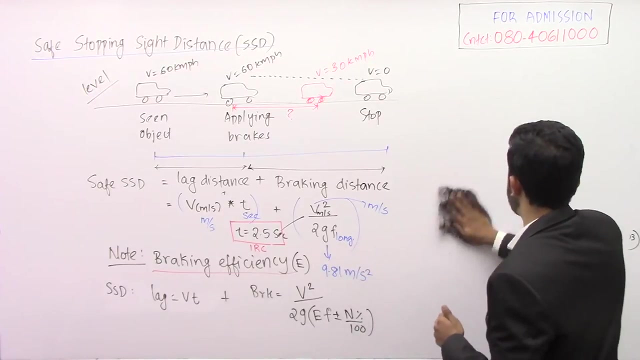 okay, so this is what now, one important parameter. is there one twist they can make? i forgot to tell you that. see, in this case, uh see, okay, i hope you got this answer- 130. see, in this case, in this level road case, or whatever be the case. 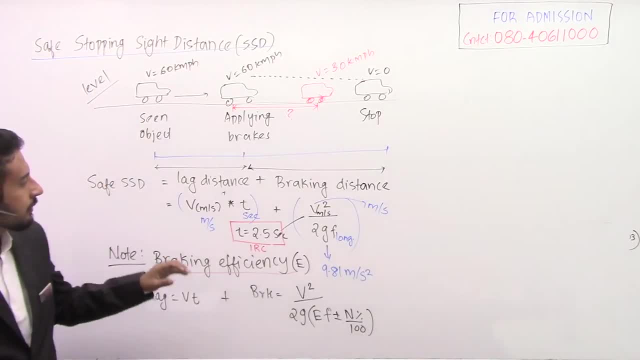 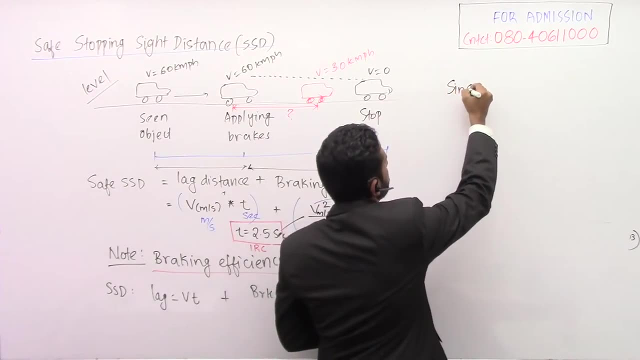 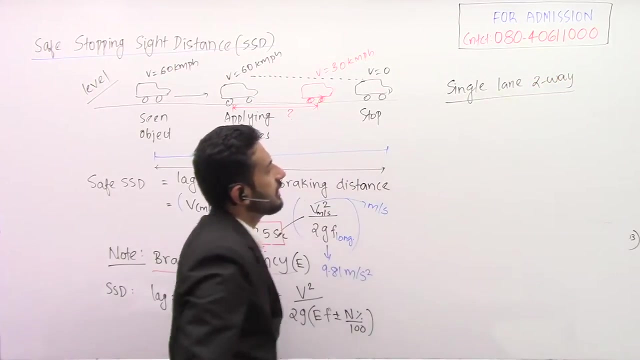 suppose. uh, generally for level road case. only that is there. see, this is in one direction, right, there is a special case of a single lane, two-way road. for a single lane, two-way road. okay, for a single lane, two-way road. what is actually happening? see, you are going to stop. 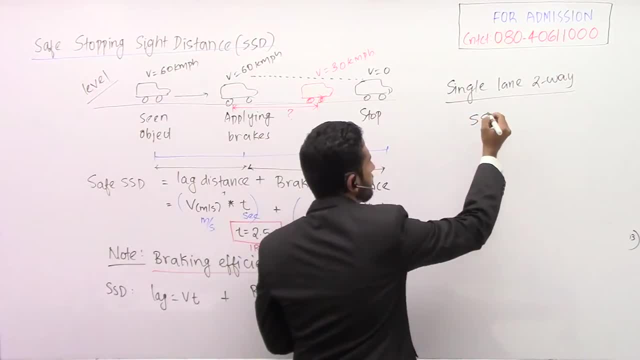 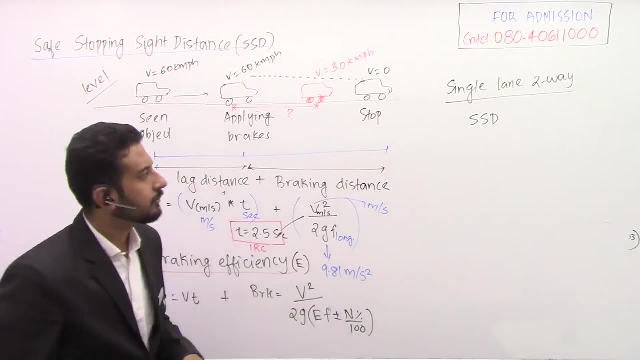 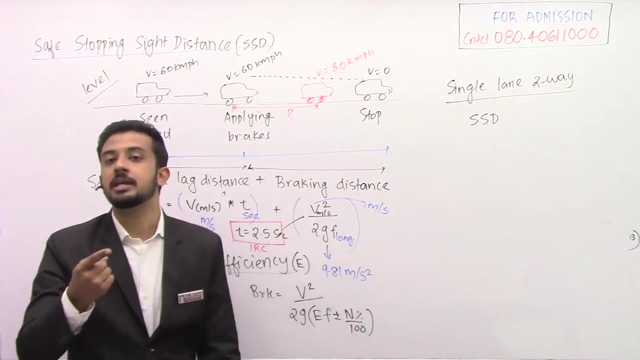 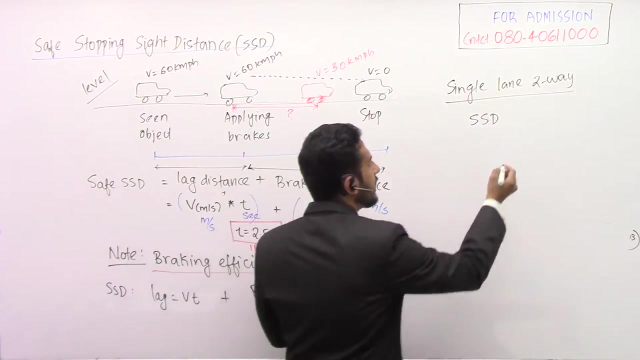 your vehicle, which means you need some ssd, single lane, two-way what it means? a vehicle is coming in the opposite direction also. so for that guy, if he is not able to stop here, what happens? he is going to come and hit you right. very good, so he is going to come and hit you then. to be safe you require. 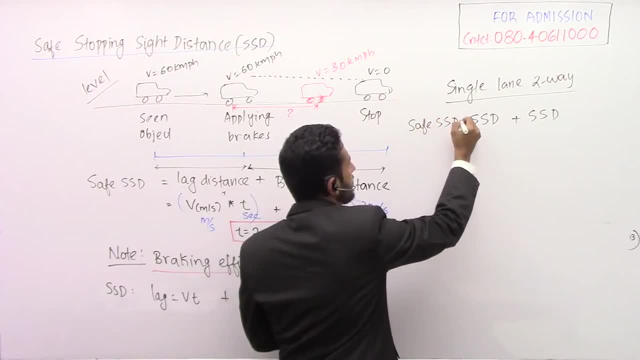 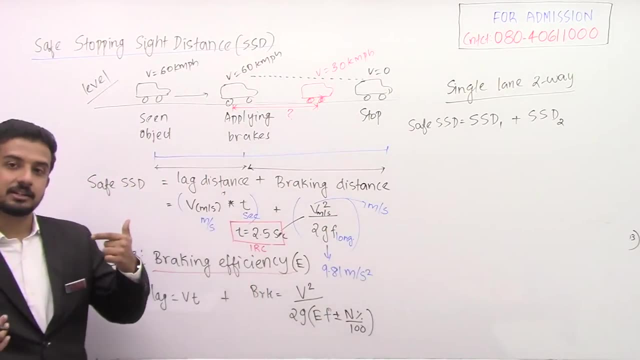 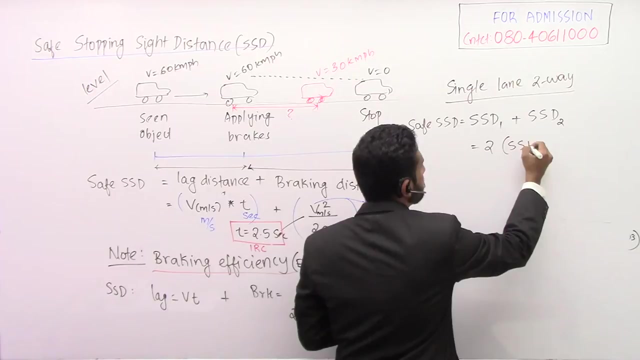 one more. so actually, the safe stopping sight distance is what ssd1 plus ssd2 a vehicle is coming in the next from the from the opposite direction also. so for a single lane, two-way road we generally take it as two times stopping sighted distance. why is two times stopping sighted? 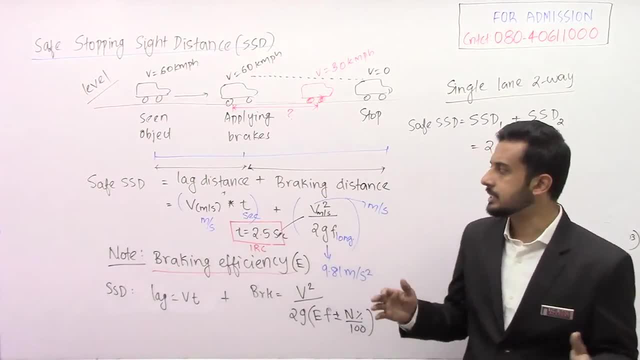 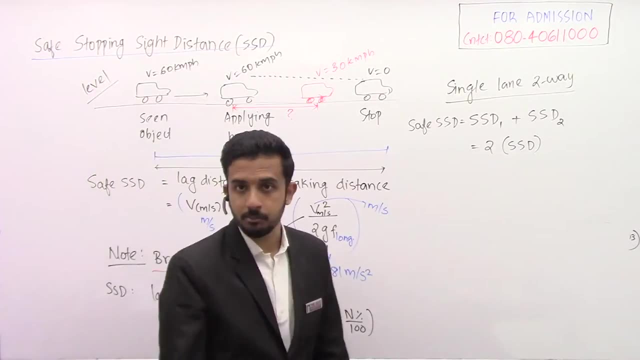 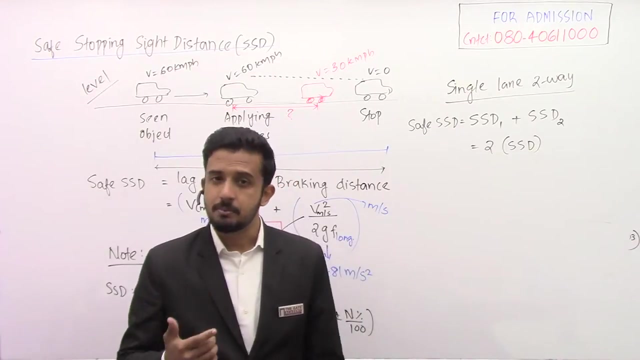 distance? why? because you need some particular distance. see, what was the value of that first question: some 81 meter. you got, no, approximately some 81 meter. so if you are having some 81 meter, yes, you are safe, you can stop and you will be safe. suppose that is a two-lane road. 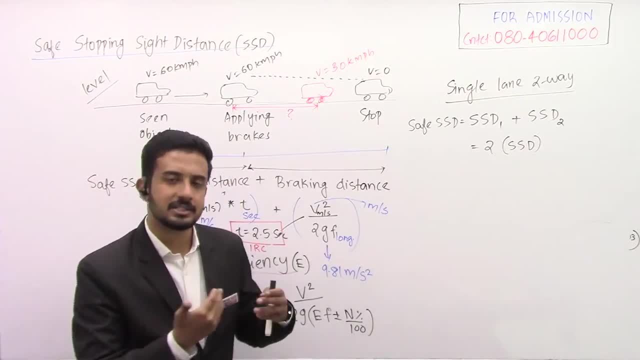 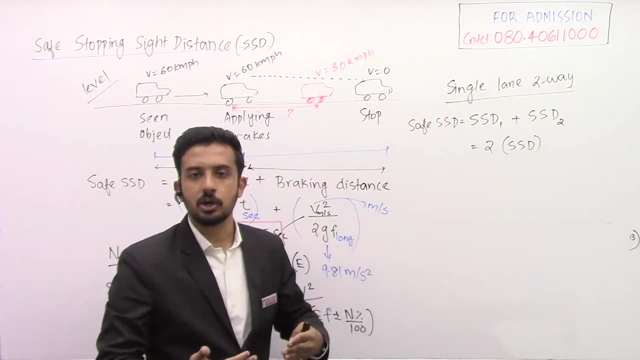 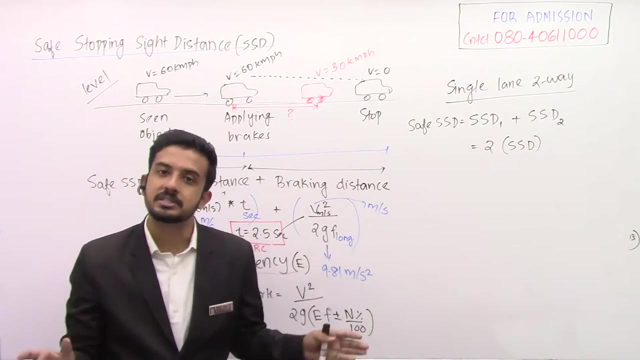 means another guy is also coming. we are assuming same speed. another guy is also coming from the opposite side. what if? if that guy is not stopping, you are stopping before obstruction, but he is coming and hitting you. are you safe? are you safe? absolutely not to be safe. how much distance you'd 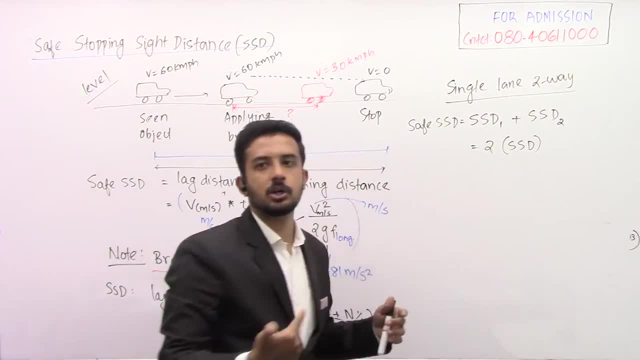 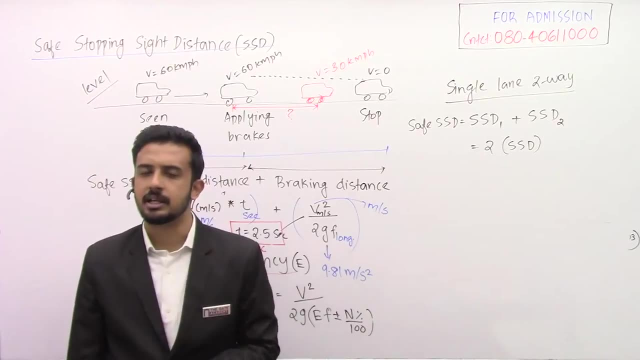 need your stopping sight distance plus that guy's stopping sight distance. so finally, you are safe, you can stop and you will be safe. suppose that is a two-lane road means what will be the value of stopping sight distance two times ssd? understanding you take the first. 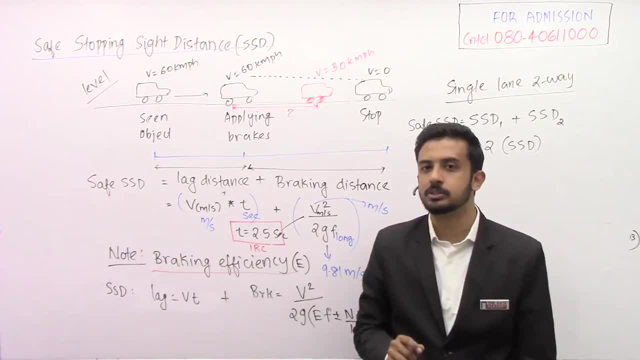 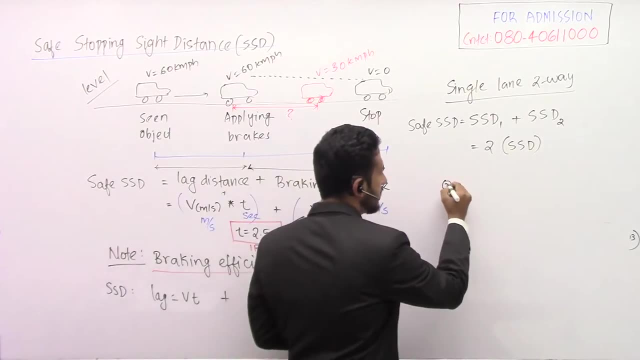 question and from the same data i am asking you one more question. suppose that was a single lane, two-way traffic for the first question. suppose i'm giving you as another question in the question three- is what in the first question, question one, suppose it was a single lane, two-way traffic. 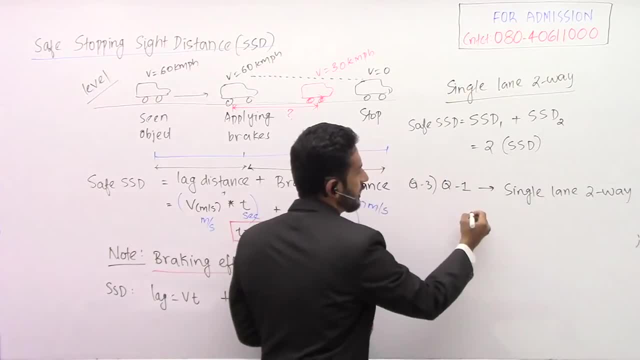 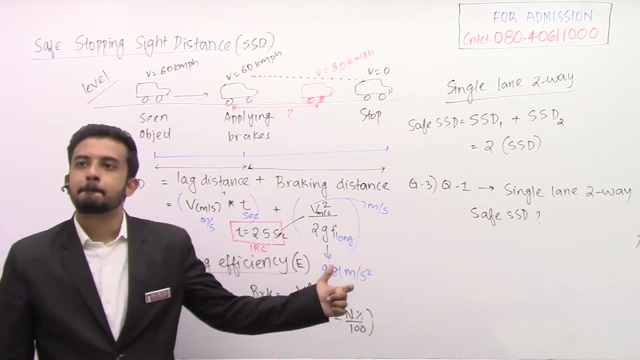 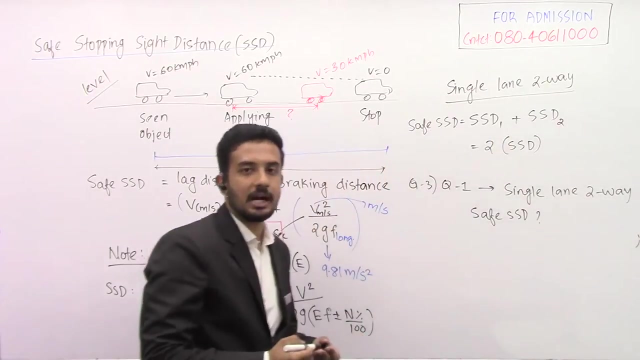 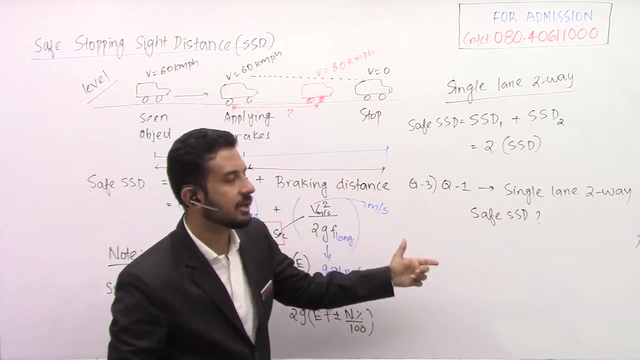 single lane, two-way traffic, what will be the safe ssd? or simply, if they are asking, stopping sight distance also same, okay, yeah, that's why i have written ssd1 plus ssd2 actually speaking. but if they are giving some value of the other vehicle, then we have to calculate ssd1 plus ssd2. but most of the time 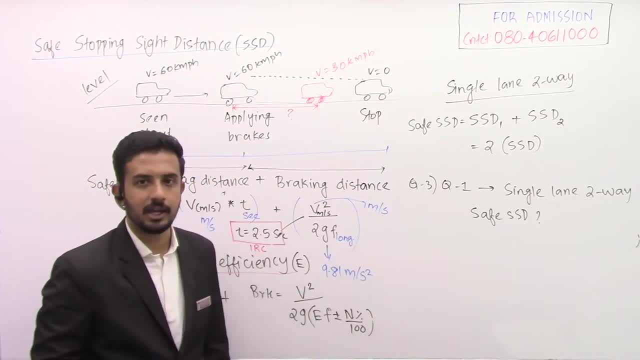 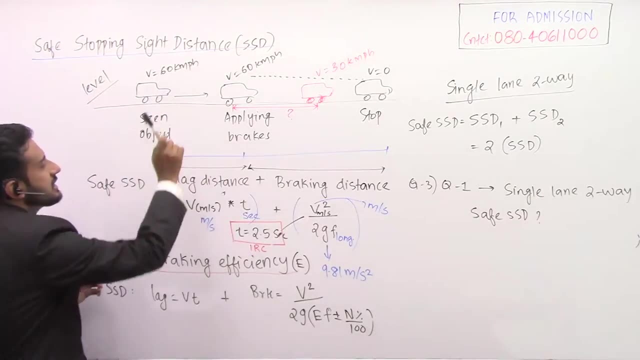 if this is the, if this is the condition of the vehicle, then we have to calculate ssd1 plus ssd2. condition: single lane, two-way. they will not give the other vehicle's value. we have to assume both are same, because we are assuming that this is coming at design speed, 80 kilometer per what was? 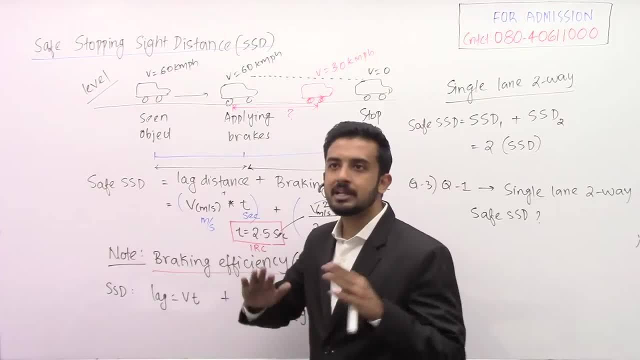 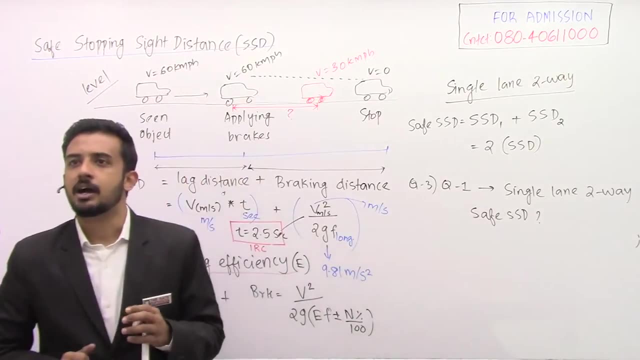 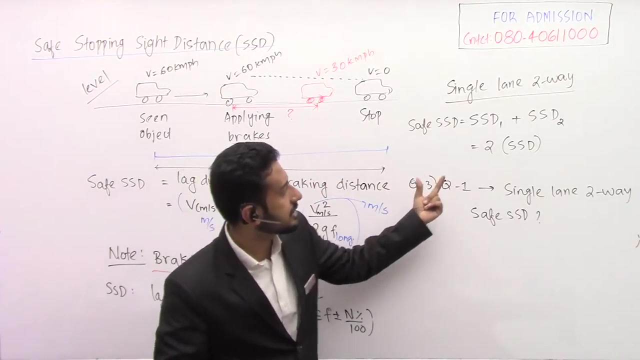 the speed first case: 60 kmph. design speed means our maximum speed, so maximum that much in the worst case we are going to come in that maximum speed only. okay, understood. that's why we are taking it as two into ssd. if they are giving separated values, then calculate ssd. 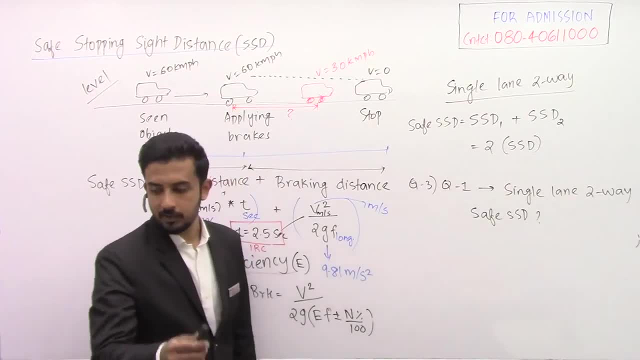 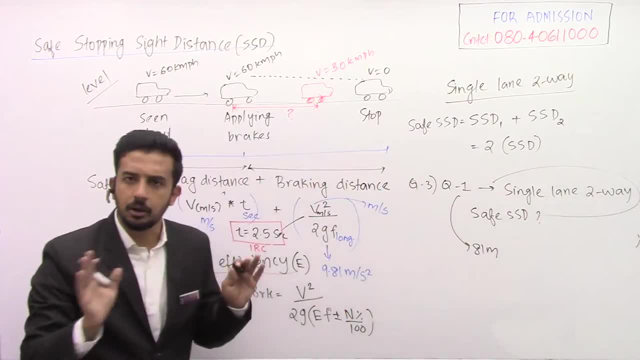 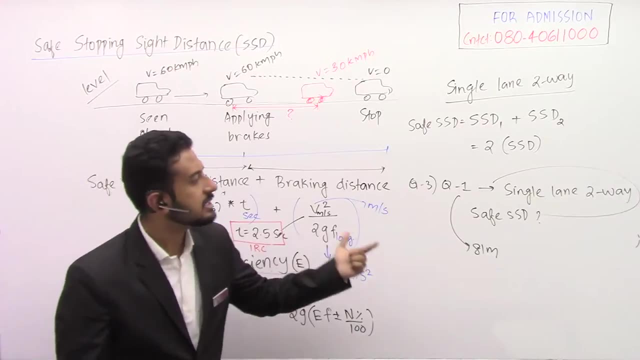 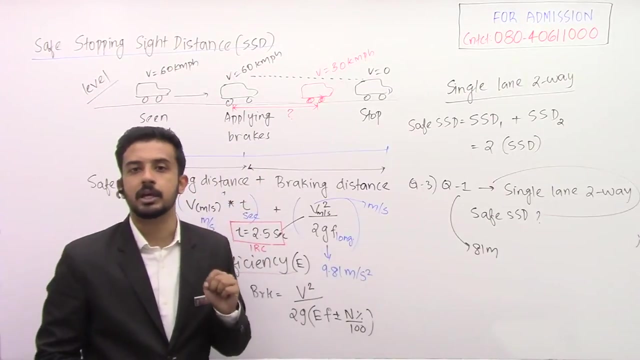 so in in by default. if they are not telling anything regarding number of lanes, directions by default. it's our general case: 81 meter. in case, if they are giving something like this, don't make mistake, don't get deviated: see 81 meter. also, they may be giving in the options. 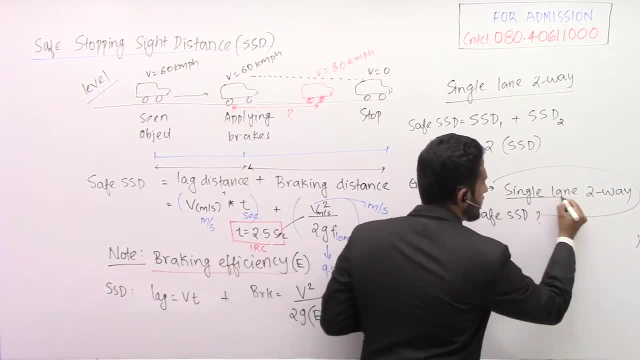 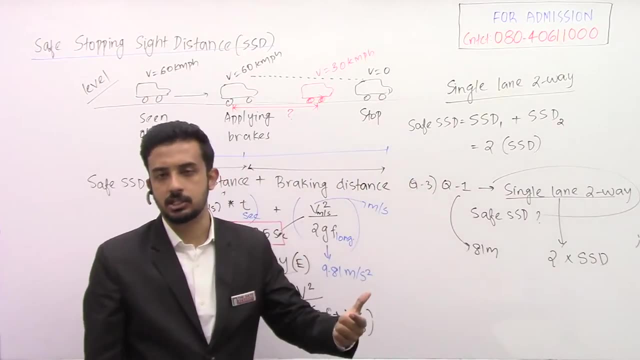 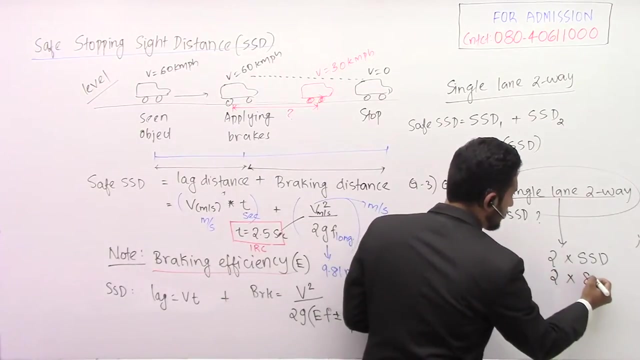 so here we got 81 meter. so if it is a single lane, two way, we know we have to take two into ssd. actually it is ssd1 plus ssd2, but since they are not giving any other data, we are assuming it is same value of speed and all. so 2 into 81 162. 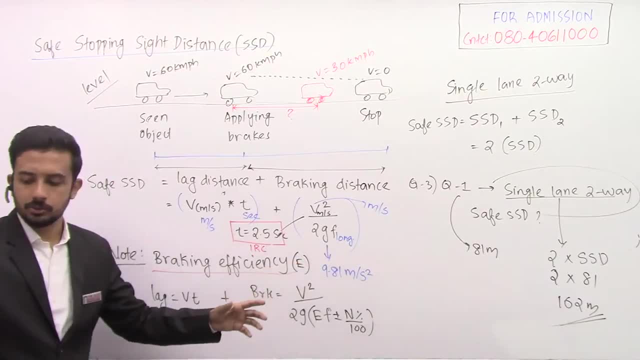 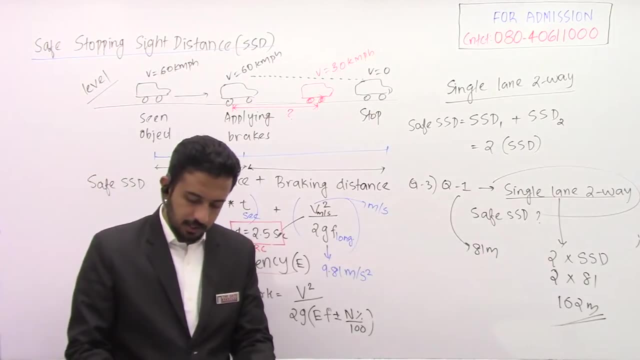 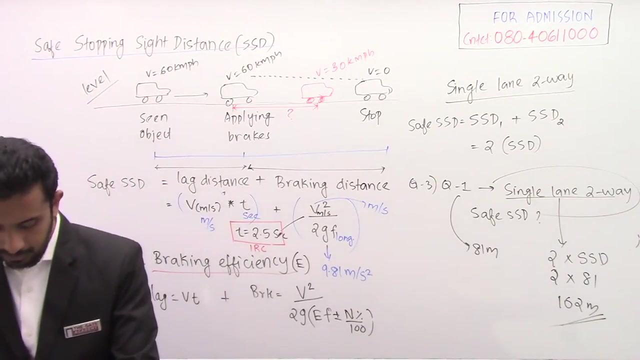 meter. okay, so i hope you understood that twist. also, in case, if they are making some twist, don't make any mistake. okay, so can i give you another question within some limited time? i'm going to give you another question, uh, okay, so i told you know some suppose this case. 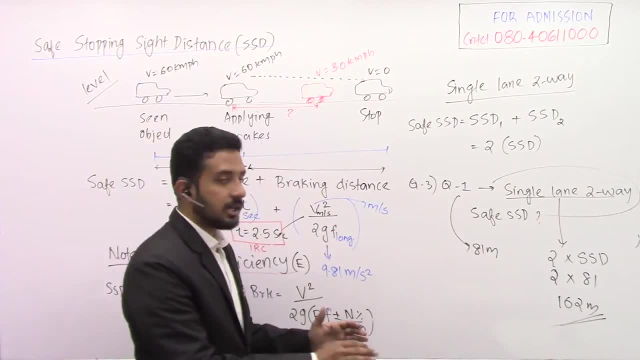 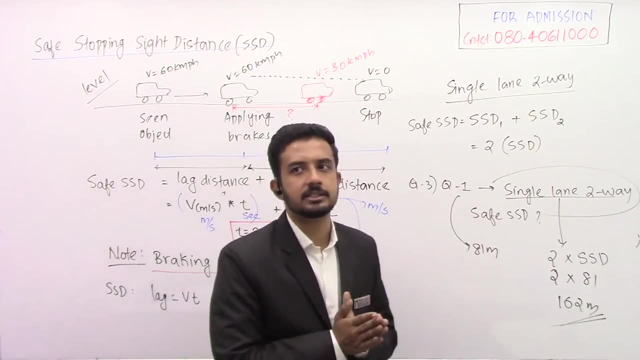 some intermediate that i'm going to give you. okay, see, always listen, always read the question carefully. uh, it may not be always. they are asking you the stopping side distance, sometimes they can ask you what is the lag distance, or sometimes they can ask you what is the braking distance. 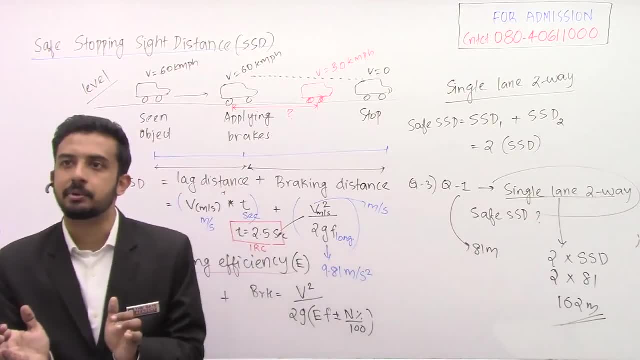 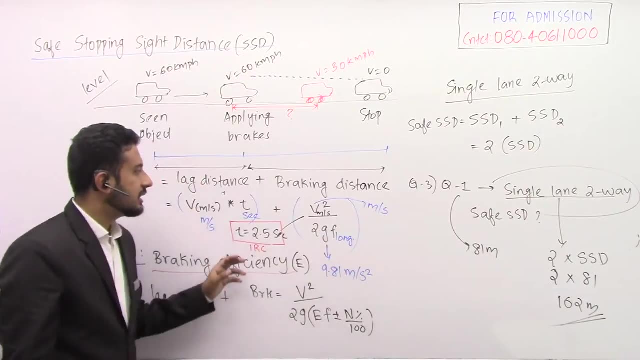 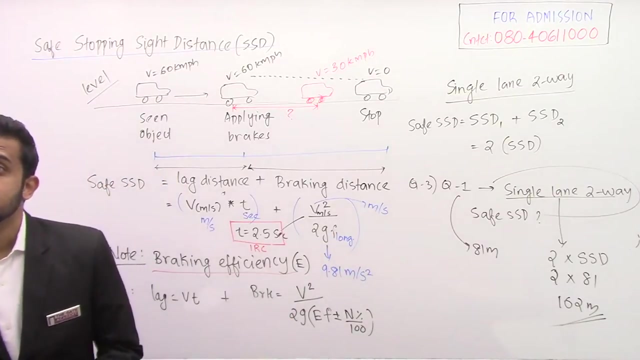 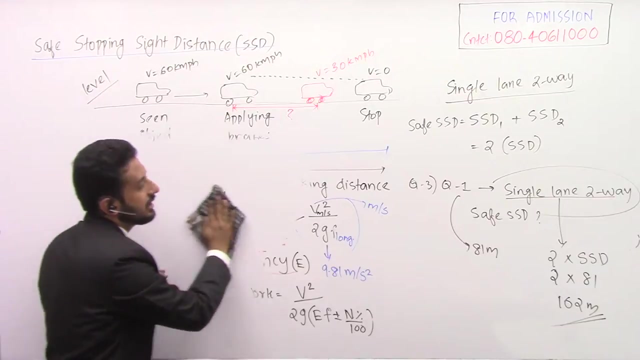 okay. so whatever they have asked, calculated separately, then uh, take the values. okay, if they are asking stopping side distance, then only add it. suppose they are asking only breaking distance. we need only v square by 2, gf, like that. okay. yeah for admission, and all you can call to that number. i have written a number there you can call. 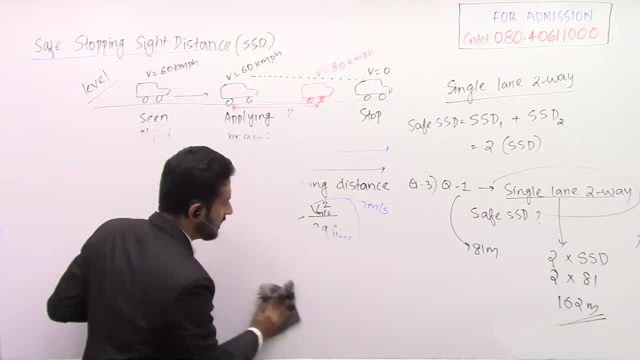 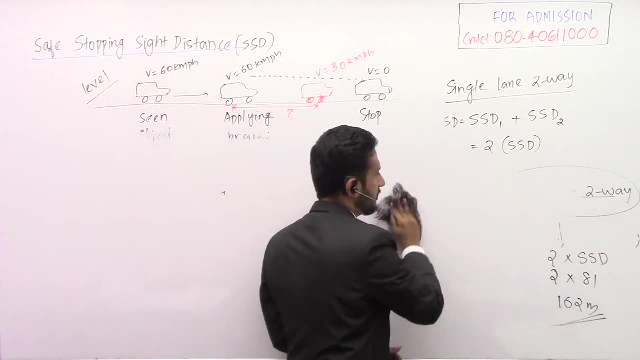 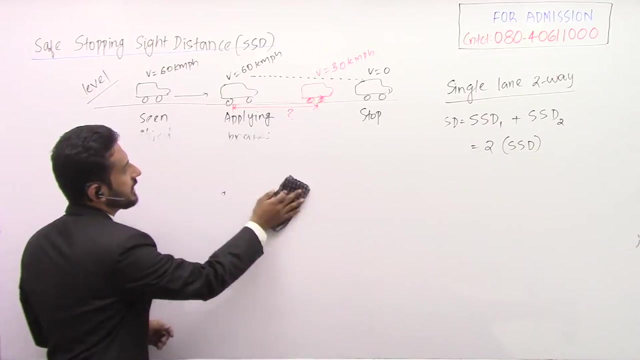 the online, offline, whatever all the classes are available. you will be getting offline classes. you will be getting physical classes. you will be getting physical classes. you can just call to that number and ask your queries. okay, and regarding other subjects, time table: also, you can contact and ask them, fine, so i'm just going to give you a question. 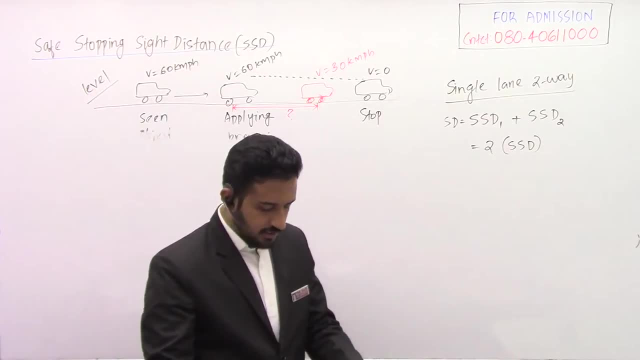 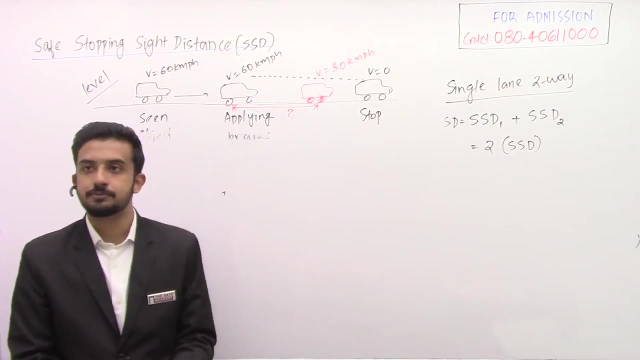 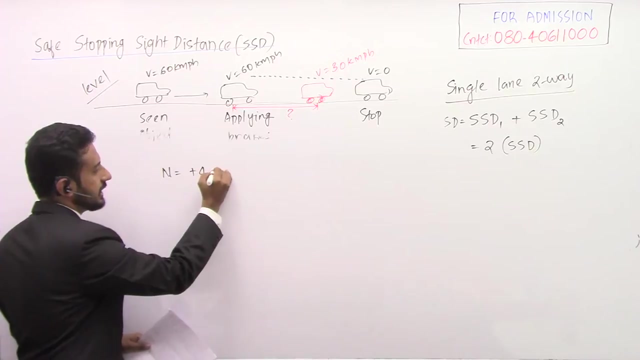 something like this. if they are making some twist, don't make mistake, so write a question. a vehicle is moving on a road of gradient plus four percent dates. a vehicle is moving on a gradient of plus 4 percentage. what it indicates it's an upward gradient. okay, at a speed of 20 meter per second. 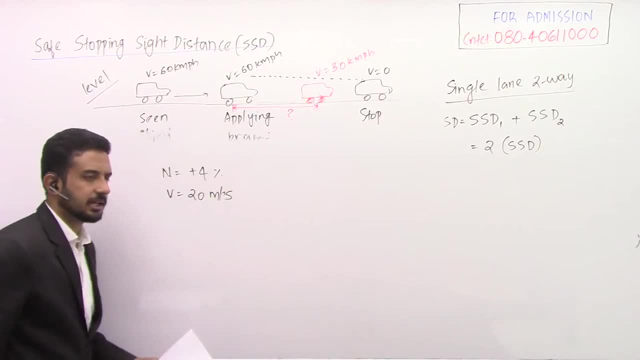 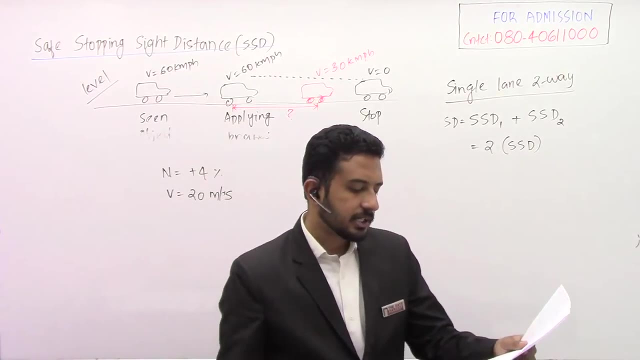 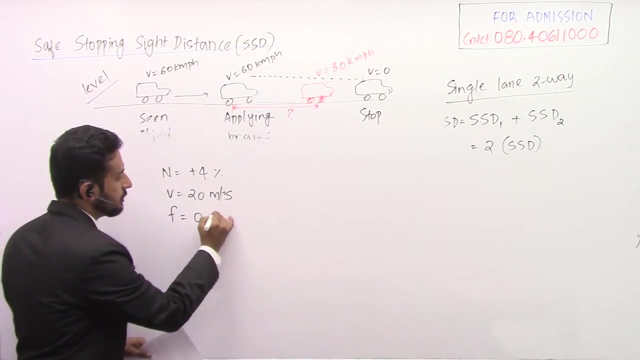 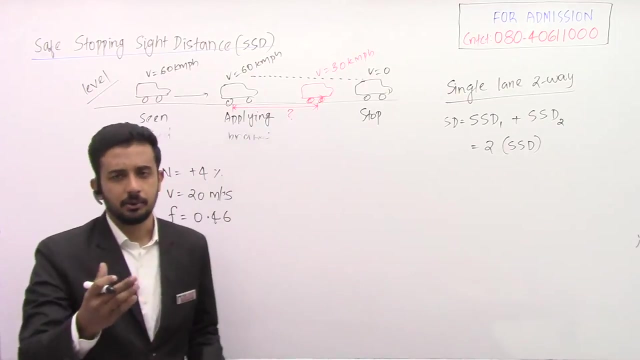 so speed is given as 20 meter per second. so no need to convert now. they have already given meter per second, so 20 meter per second. consider the coefficient of friction as 0.46. coefficient of friction is how much? 0.46? see, i told you for design we are taking from 0.35 to 0.4. i told you. 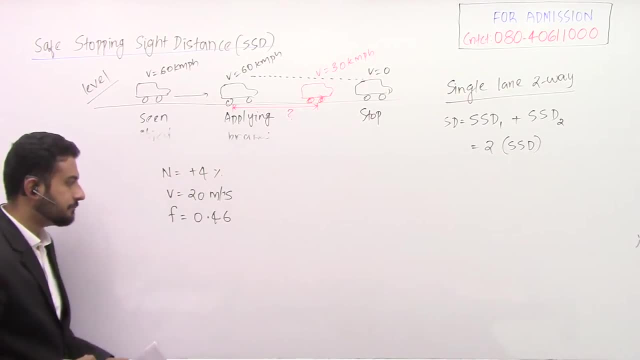 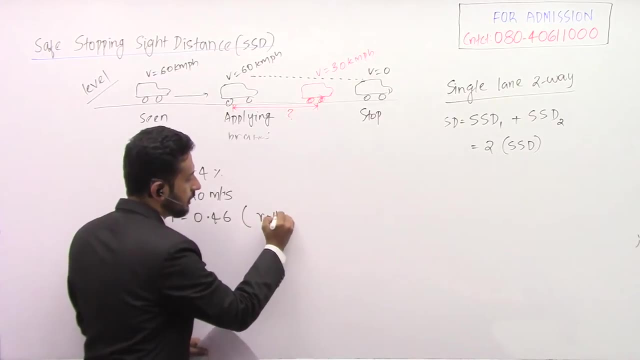 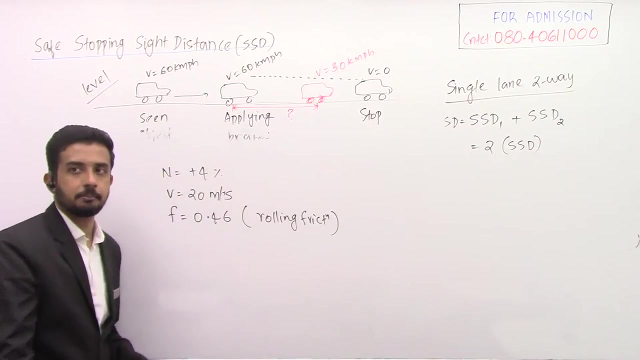 in case, if they are giving some other value, take as it is. okay, so 0.46. one more word is there for this longitudinal friction. it is also called as rolling friction, coefficient of longitudinal friction or coefficient of rolling friction. both are same. okay, so 0.46. and 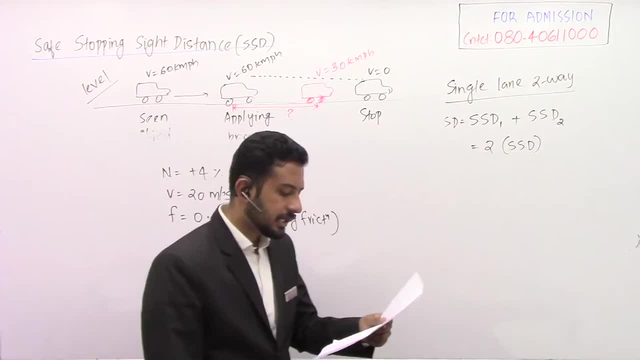 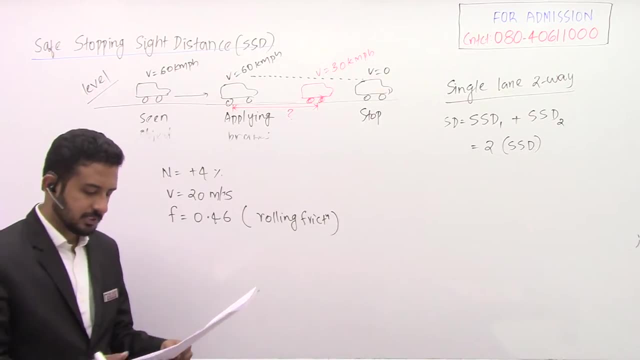 next sentence: what will be the braking distance of the car? what will be? sorry, sorry, sorry. one second. uh, some mistake, so 0.46. and acceleration due to gravity. acceleration due to gravity is 10 meter per second square after f value, take g is equal to 10 meter per second. 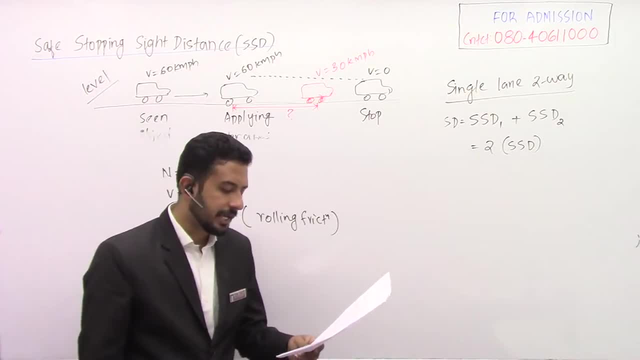 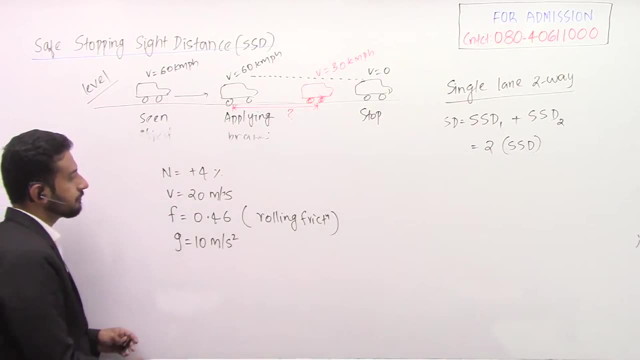 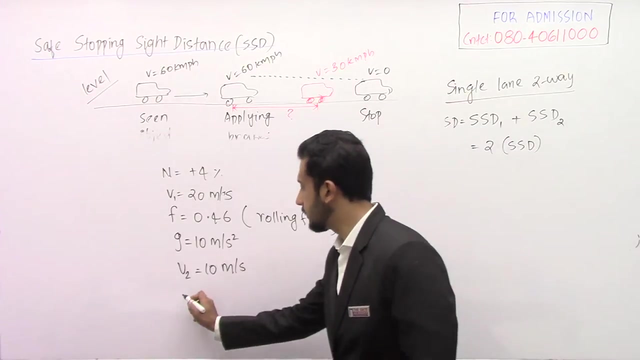 square. next sentence on applying the brakes. on applying the brakes to reach at a speed of 10 meter per second. applying the brakes to reach a speed of 10 meter per second, the required braking distance in meter. the required braking distance in meter will be dash. what will be that distance? required braking distance? 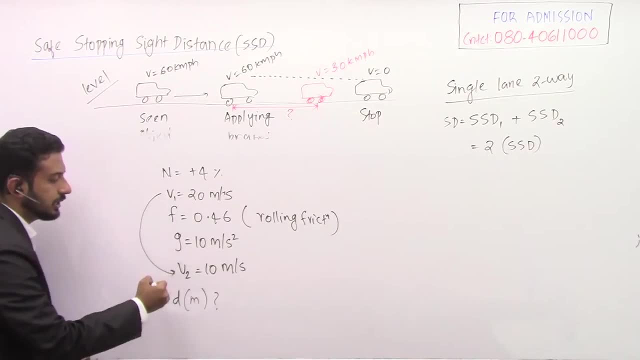 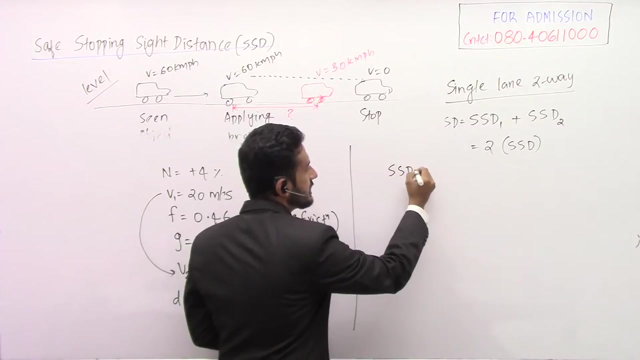 required braking distance to reach from this 20 to 10 meter, meter per second. you have to calculate in meters. yeah, do it. so what equation you have to use? we have already studied, see. stopping side distance is vt plus p, square by 2, g, f plus n, percentage by 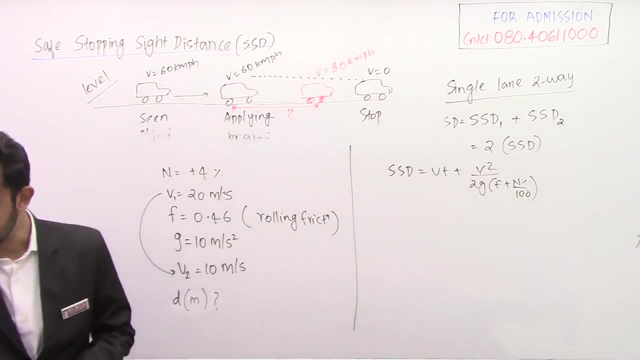 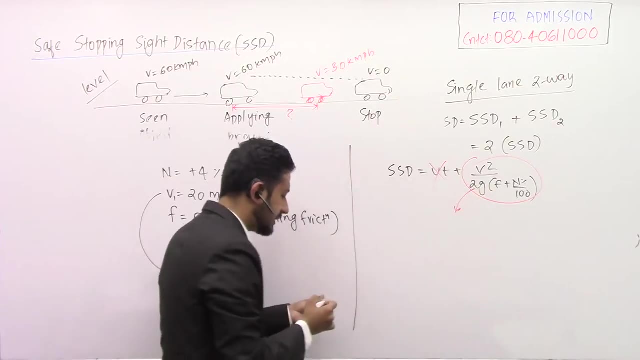 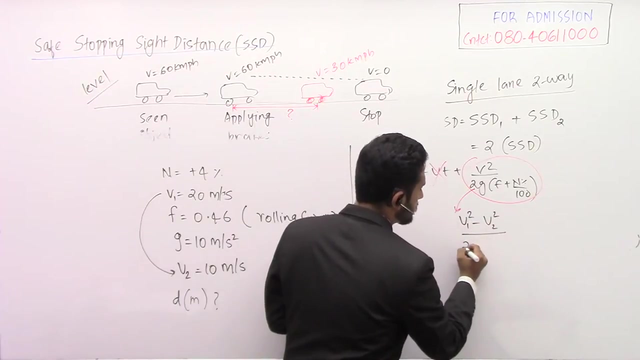 100. but see, we are not asking the stopping side distance. they are simply asking what is this portion right? we don't require this. so how to calculate this? i told you very good abhishek. if they are giving two values, what you have to do? v1 square minus v2 square. no need to remember the 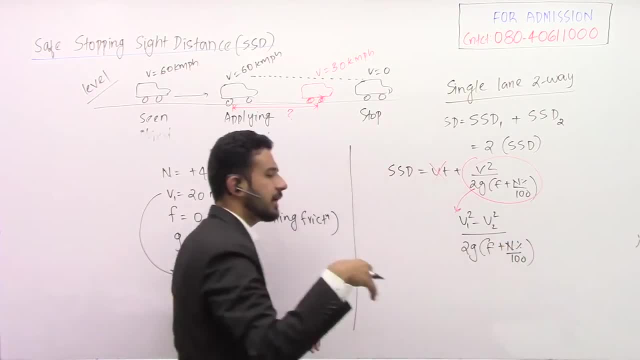 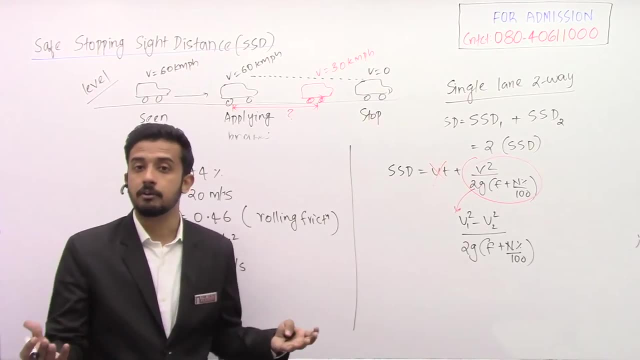 derivation and all the derivation i have given. see, maybe after a few days or few months, if you are taking the formula and checking v1 minus v2, square and all, what is this? don't feel confused. that's why i have given the derivation. okay, directly, you can use this equation now. so in 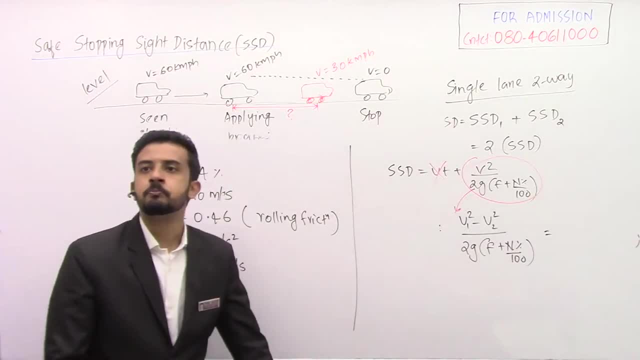 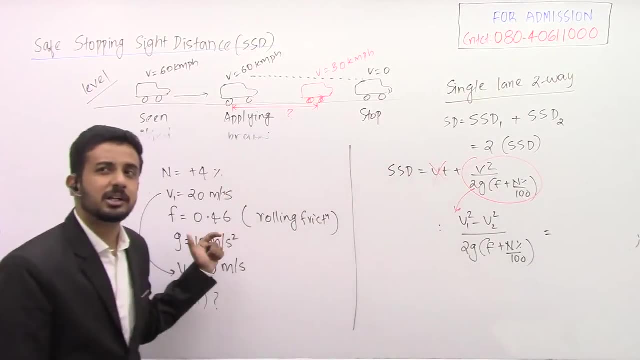 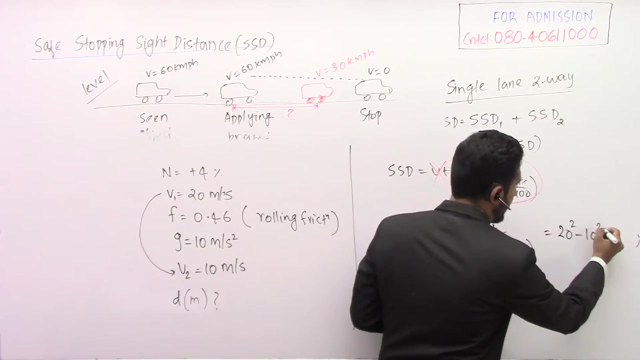 this case, no need to convert because it is already given into. very good, why don't you check the calculation once again? some minor mistakes may be there. i think you have again converted into meter per second and all okay. so it's already in meter per second. so 20 square minus 10 square, divided by 2 into: 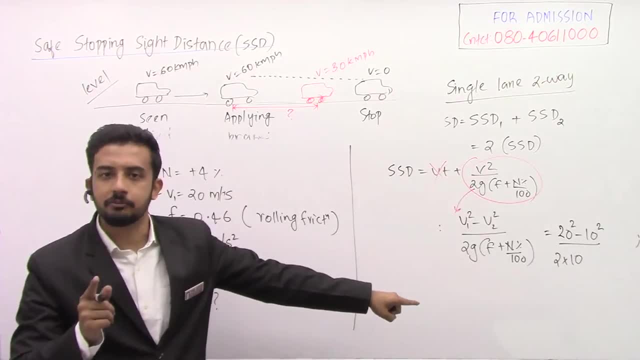 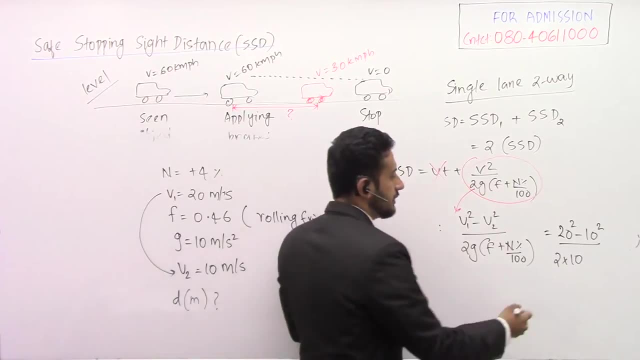 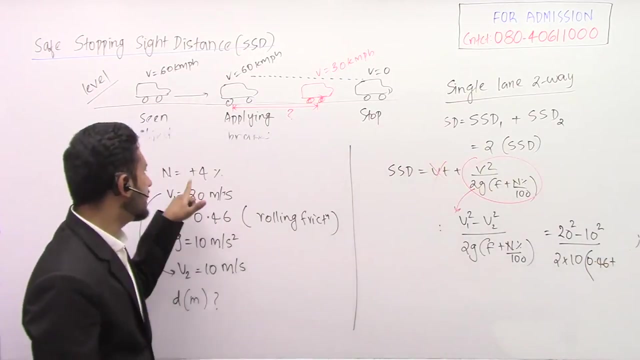 this thing g in which value you have to take. if they are giving 10, take 10. if you are taking 9.81, you are going to get something more value. okay, so into what is the f value? they have given 0.46, so it is a plus. right, already given it is plus or it is an. 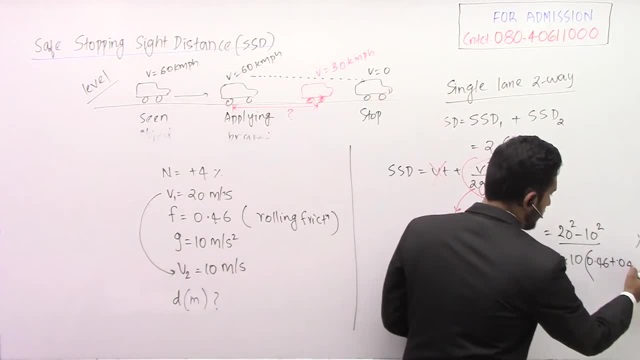 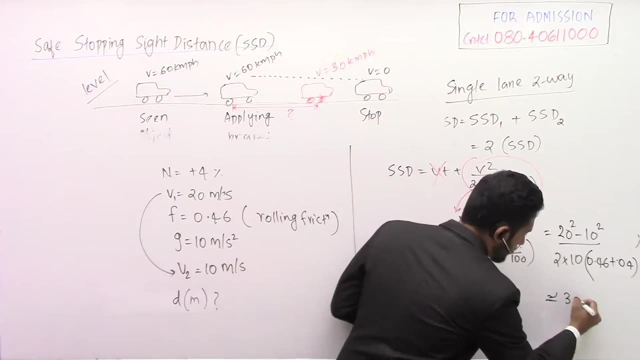 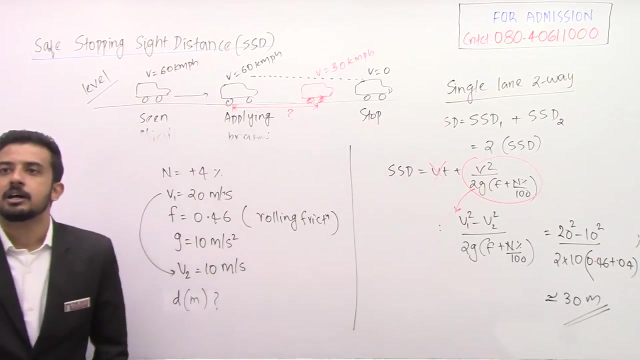 upward gradient of 4, percentage means 0.04. how much you are going to get? very good, everyone is getting approximately 30 meters. approximately 30 meters. are you getting? yeah, very good, john, very good, vishnu is getting good. uh, why don't check the solution? maybe somewhere you made a calculation. 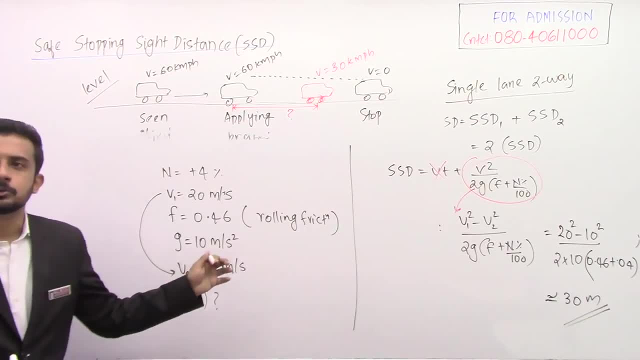 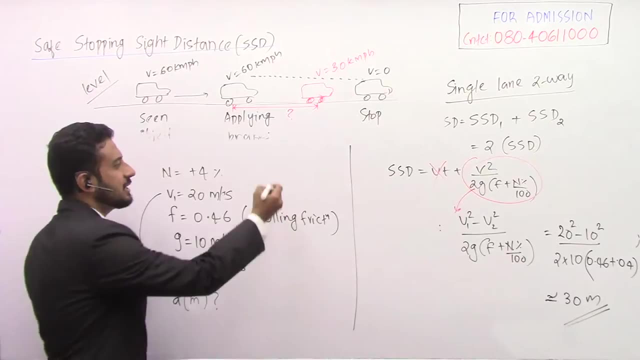 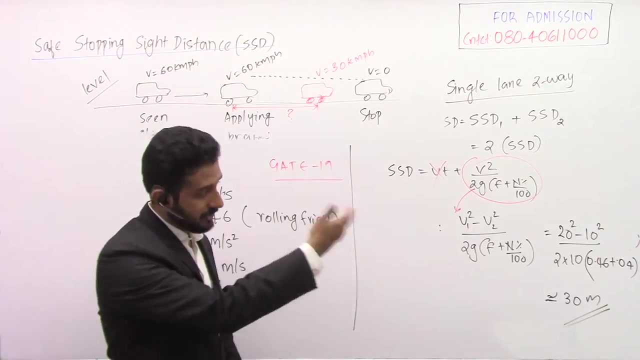 mistake. okay, i hope now you are getting. so what about this question? is an easy question or tough question? i will tell you: this is the toughest question asked from this concept for gate exam. this is a gate 19 question. recently, very recently, they asked the question. the previous questions which 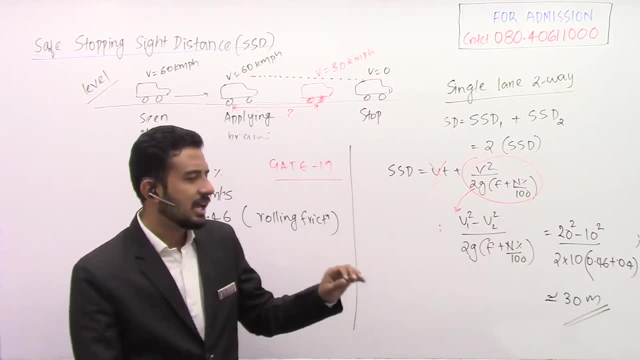 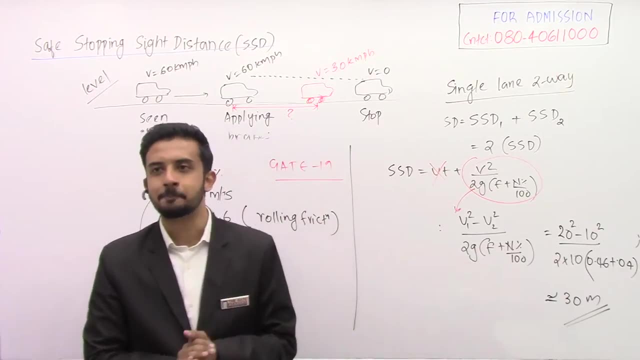 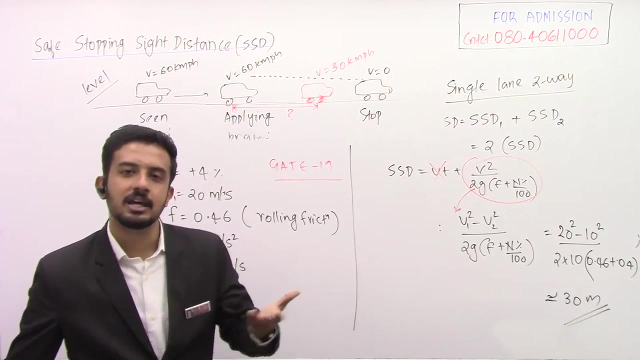 we have solved same type of gate questions asked. i have simply changed the value. say we have used some 60, 60 kmph instead of 60. they have asked some 70. that's it. so purposefully i have not given the value of that value of gate question because gate question also you can practice and check whether. 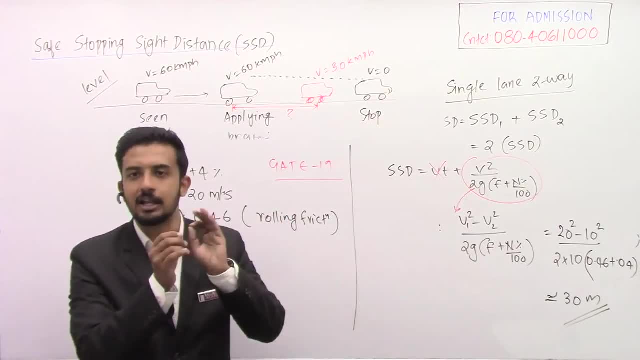 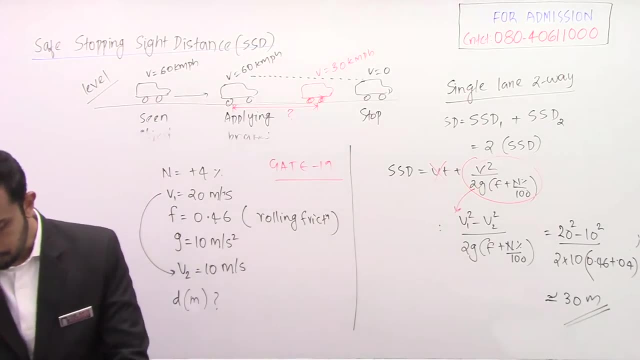 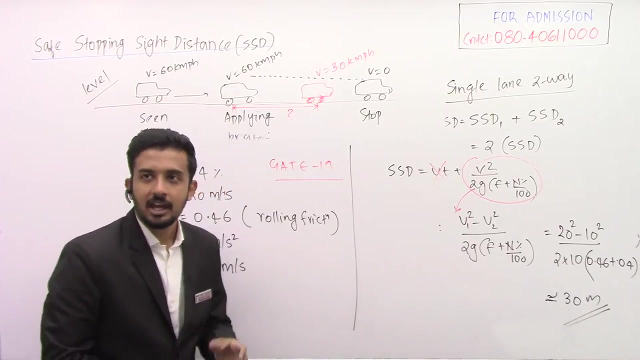 you are getting the same value or not. i've just changed the values. so many times they have asked the question whether you need one more question. we can. we can solve one more question right before winding up. okay, another, another, uh level of, or other way of asking question. okay, i'm just going. 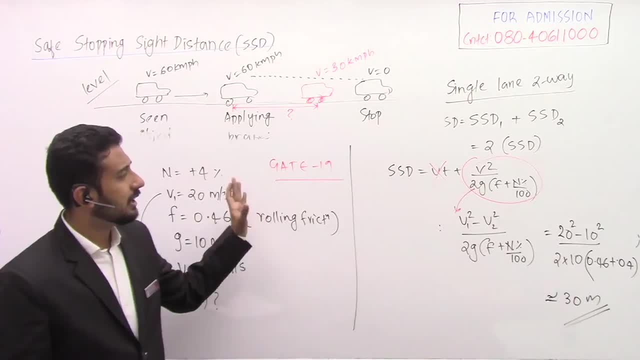 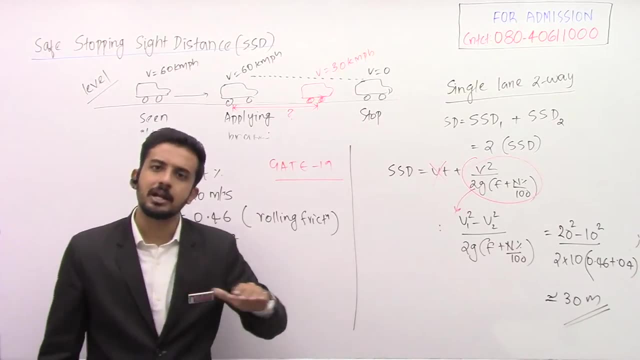 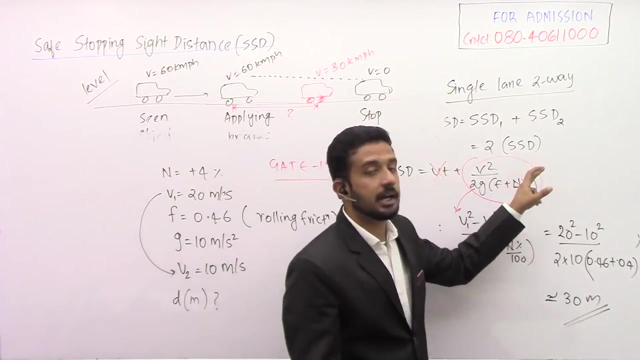 to give you one more question. so i told you: uh, either they can ask you in the same of a plain level road what it is if they are not giving you any gradient, which means by default it's a plain road, okay, vt plus v square by 2, gf okay. and if they are giving it's a two lane, oh sorry, a single. 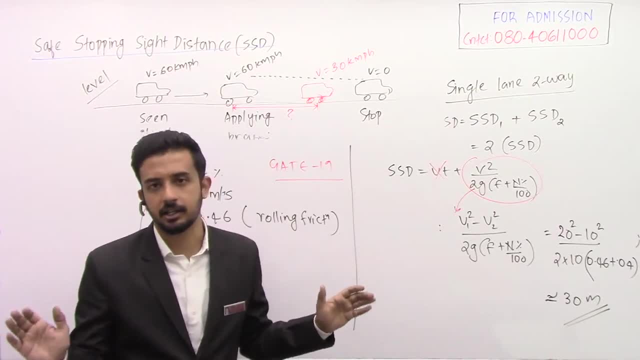 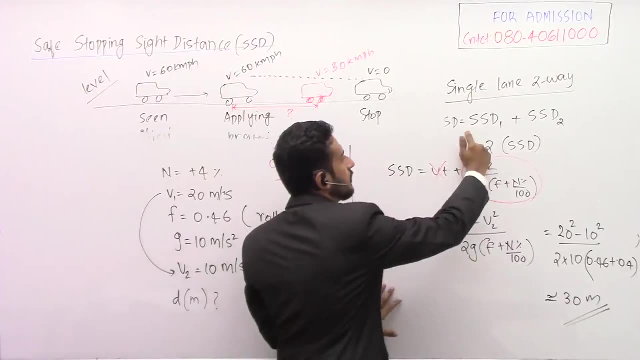 lane two-way road. in all other cases- general case- only if it is a single lane two-way, we have to multiply by two. if they are giving two values calculate separately and add it, most often they will not be giving like that. so two into ssd. and they will not be giving like that, so two into ssd. 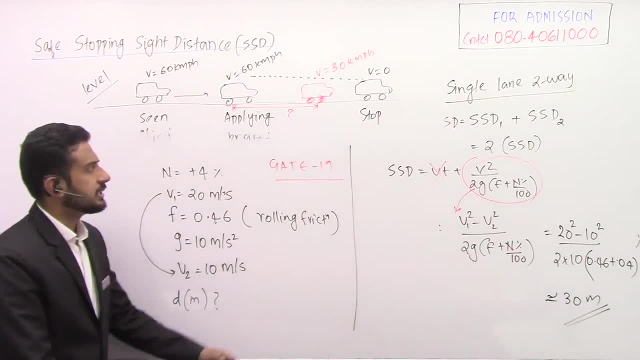 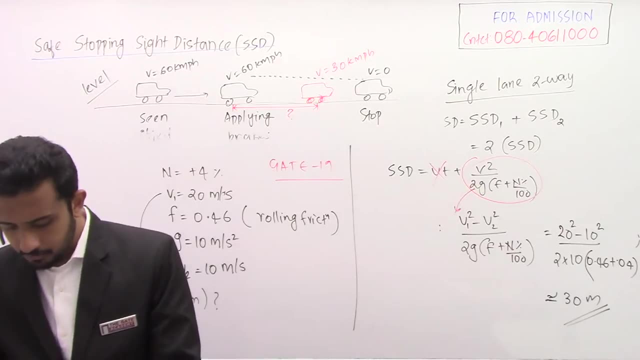 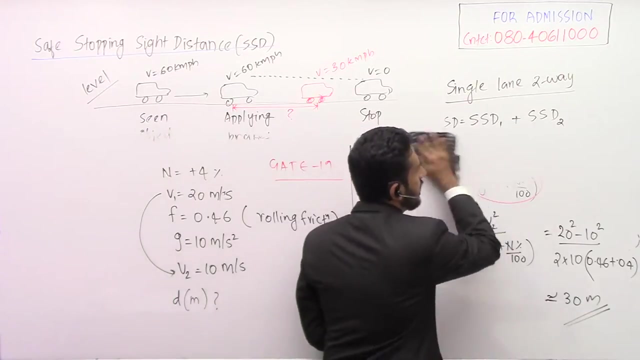 and uh, if they are giving gradient plus or minus, so that's it. if they are giving some twist like this, directly, you have to calculate like this: yeah, one more variety i'm going to give. so write the question: a vehicle is moving at a speed of. a vehicle is moving at a speed of 100 kilometer per 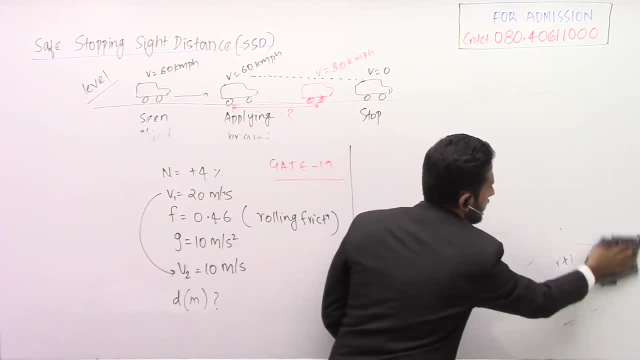 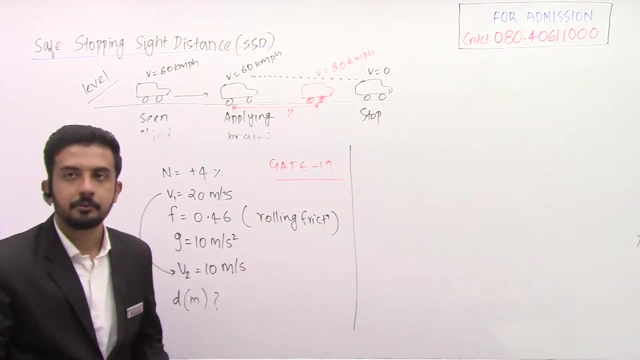 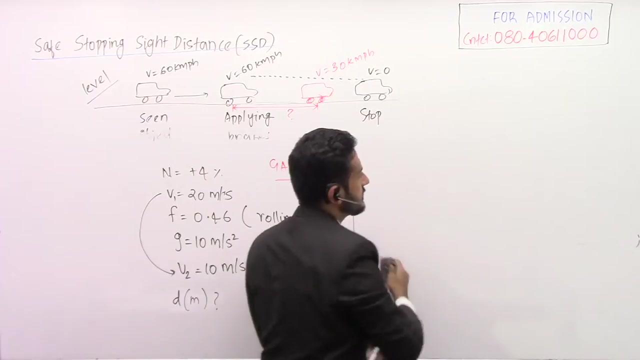 hour. a vehicle is moving at a speed of 100 kilometer per hour. if the reaction time of the. if the reaction time of the driver was found to be 2.45 seconds. if the reaction time of the driver was found to be 2.45 seconds. 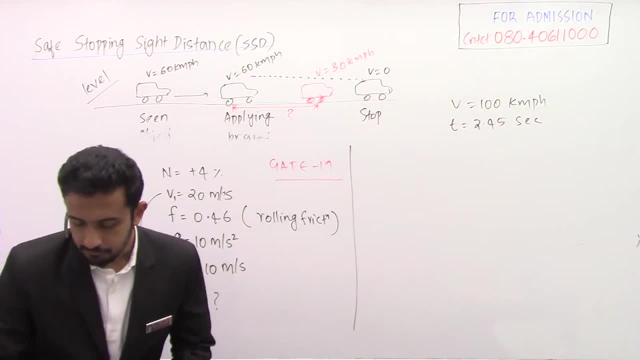 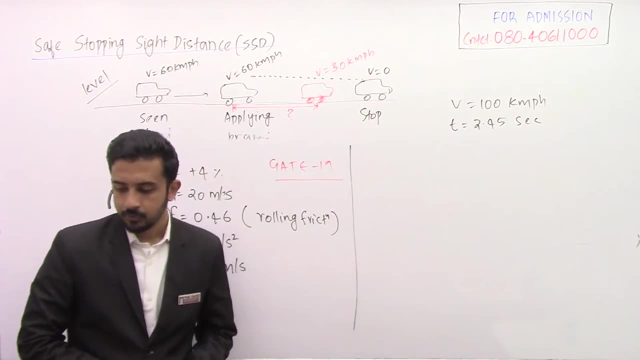 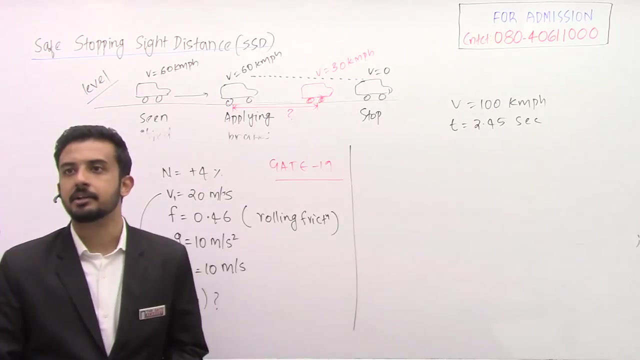 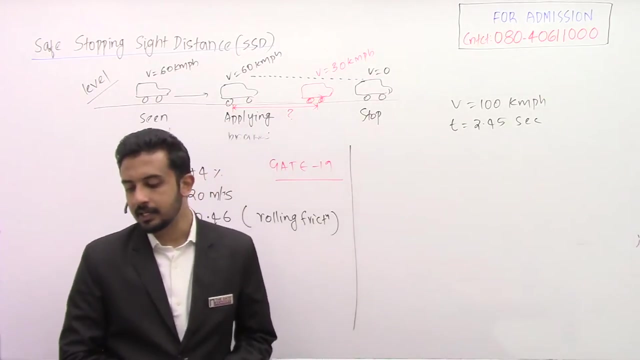 2.45 seconds. yeah, full stop. the reaction time of the driver was found to be 2.45 seconds. what will be the braking distance? what will be the braking distance if the lag distance and the braking distance are? what will be the braking distance if the lag distance and the braking distance are in the ratio? 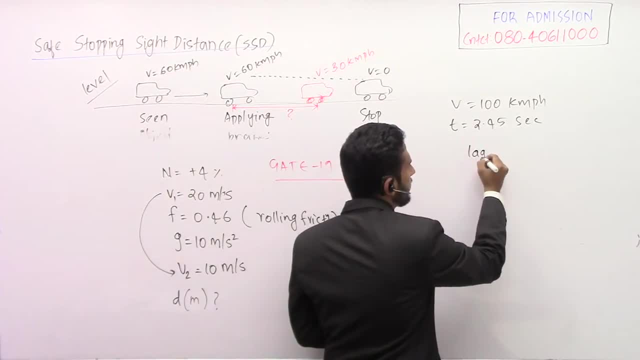 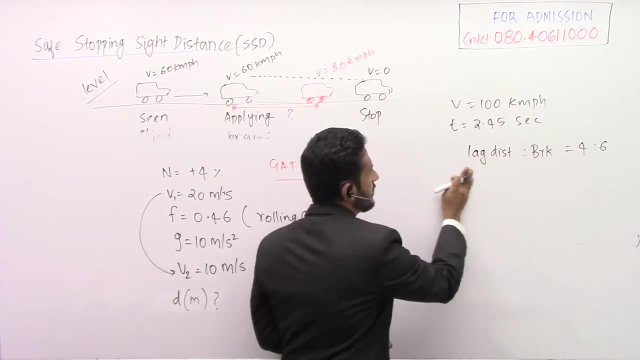 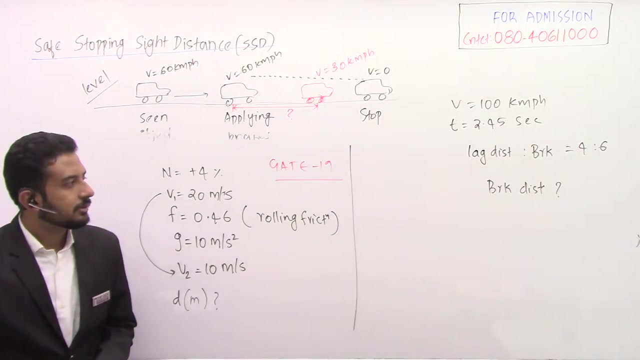 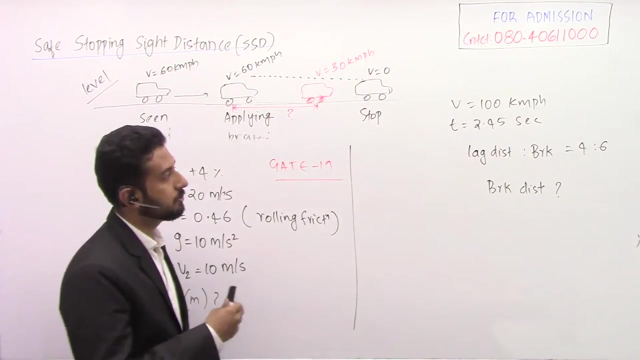 four is to six. if the lag distance and the braking distance are in the ratio four is to six. so this is given. and finally, what they are asking, what will be the braking distance? four is to six, so what will be the breaking distance? okay, so just see how to calculate that reaction time is given: four point two, point four, five. 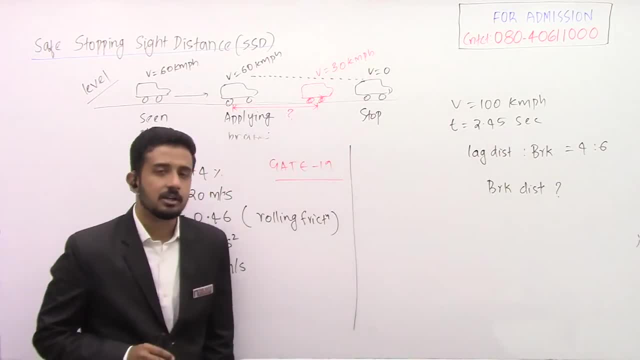 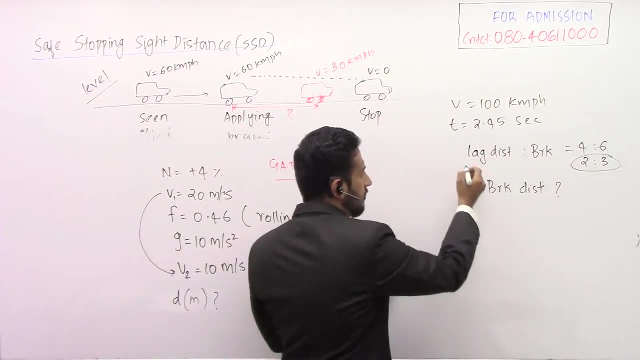 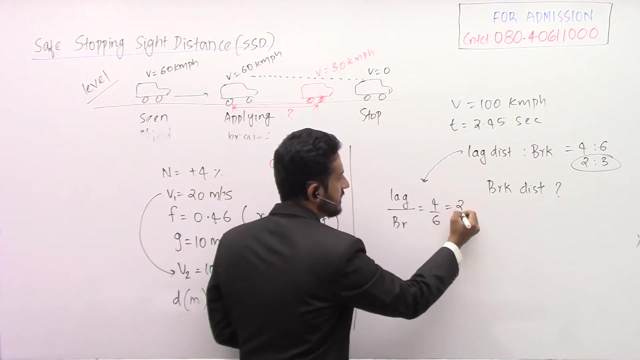 seconds and the lag to break distance is given as: four is to three, nothing but two is to sorry. four is to six, nothing but two is to three. whatever what it indicates, lag distance by break distance equal to four by six, or i can write it as two by three. both are same. 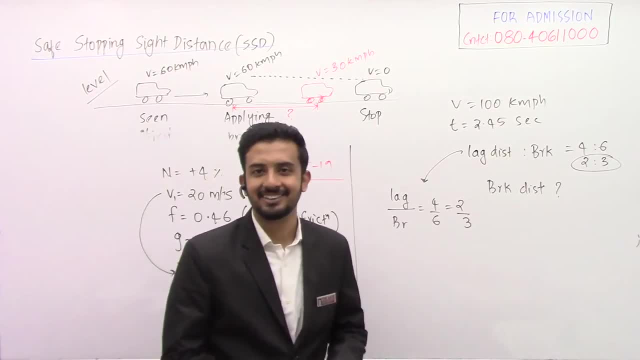 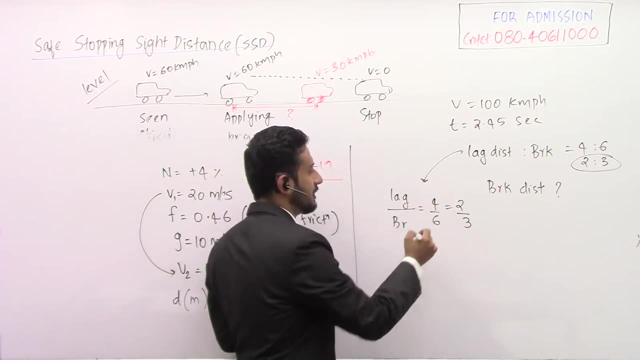 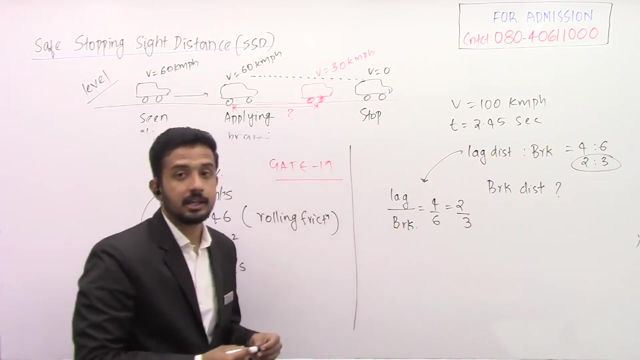 hope you take transportation for new batch in bangalore. yeah, hopefully we'll see lot of. we're having a lot of good faculties. in fact, whoever is free will come to you for taking class, or for those who are not able to to take the physical classes can take the offline class also. that is one of the important good thing. 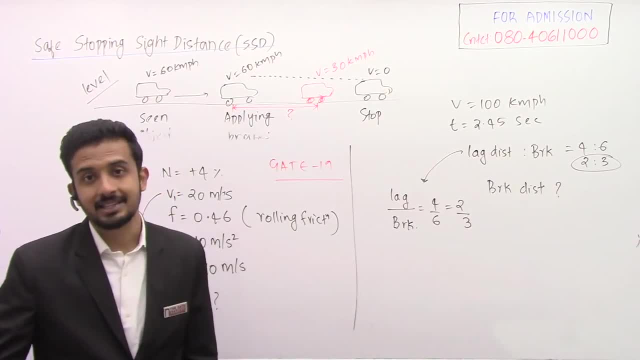 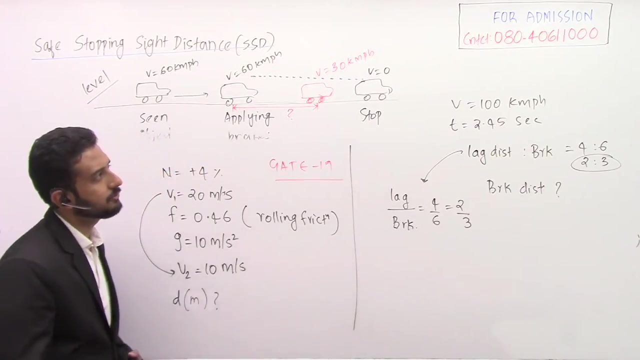 which is going on in the gate academy. if you are working somewhere or if you are studying, you are not getting time to go for the physical classes. then you can go for the online class also. online course is available, so you can call to that number, 08040611000, for more. 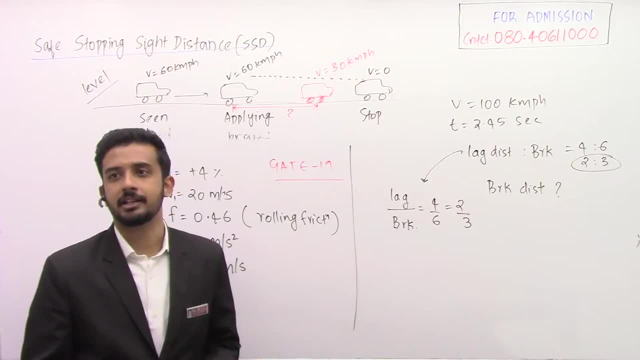 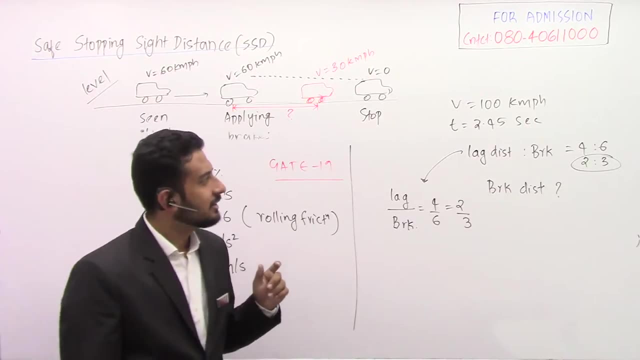 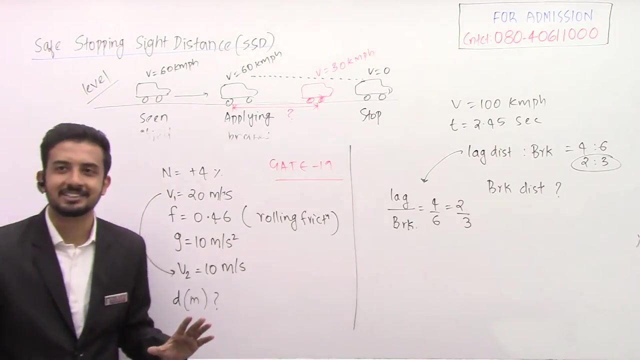 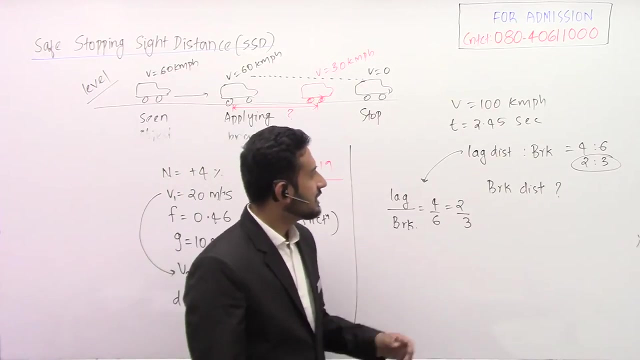 information regarding the courses. getting the answer for this question. are you getting confused? it's a tricky question. what is the answer for this? it's actually a simple question. you need only some 10 seconds to solve this. 102 very good, vishnu. see that speed and all we don't. yeah, yeah, very good, one or two. 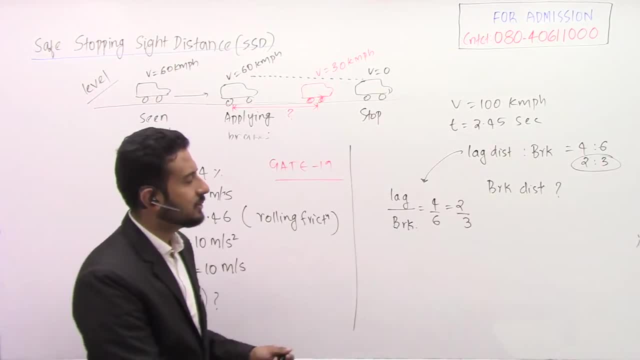 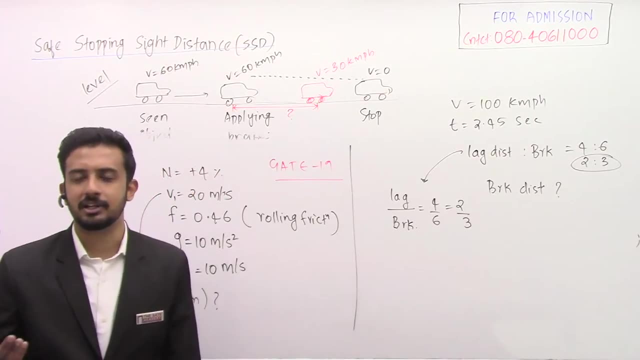 no need to get confused. and all from the given values, what they have given. speed is given, reaction time is given. see, suppose you might have to be thinking that what is the coefficient of friction? and all now? see, suppose the coefficient of friction is also given. let it be something. 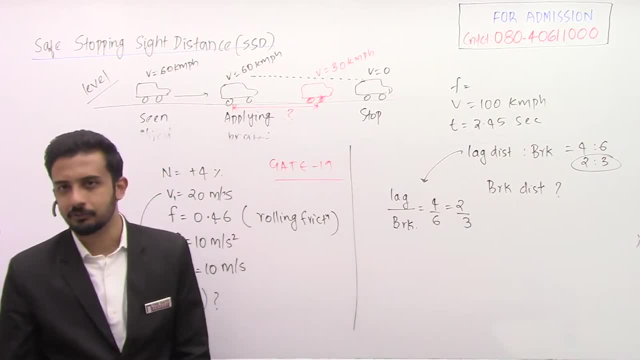 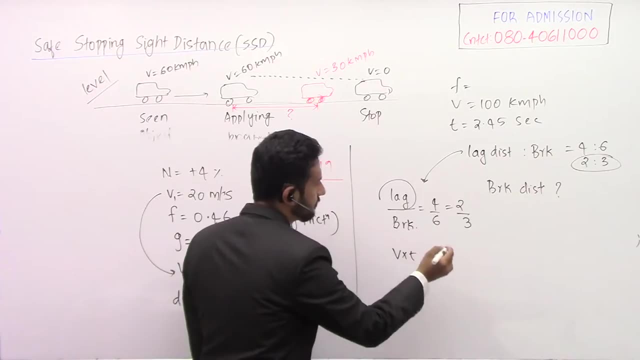 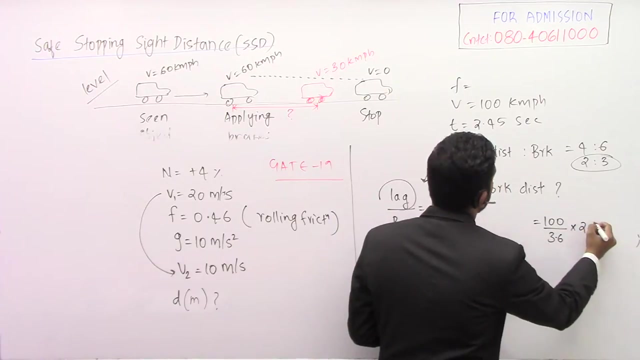 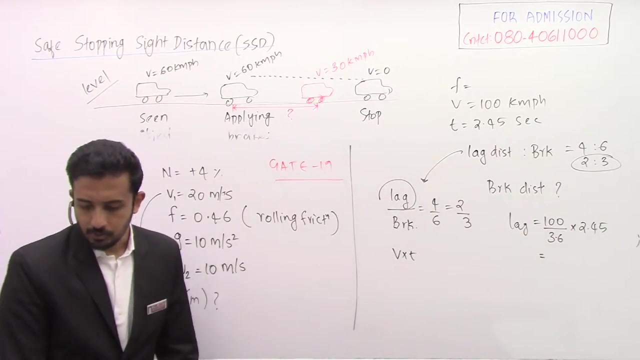 don't get confused because of that. we don't require the coefficient of friction here. right, yeah, very good, why don't? very good? what is the lag distance v into t? what is lag distance? so 100 divided by 3.6 into 2.45, how much is this lag distance, 100 by 3.6? so you will be getting some 68.05. this is i guess. 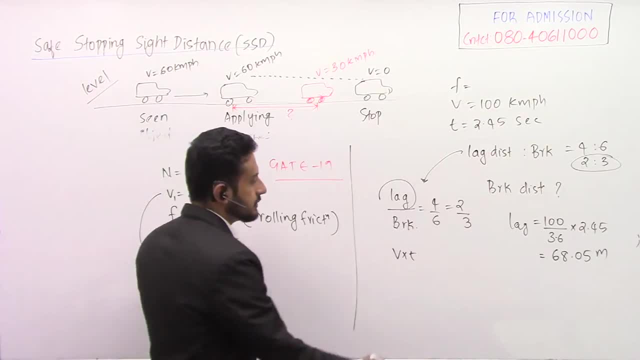 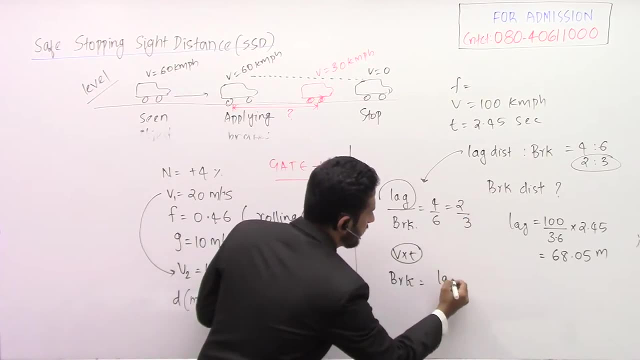 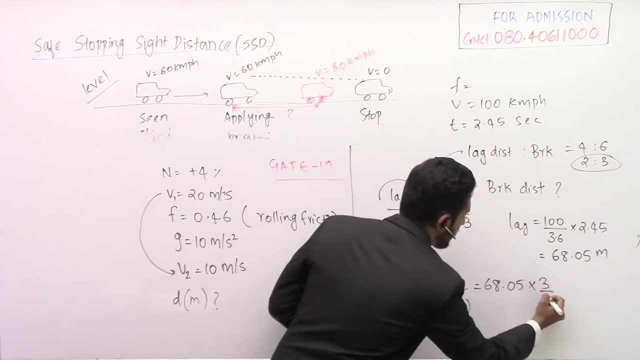 right now. yeah, good, good, abhishek, good, so this thing we have already got. then what will be the breaking distance? if you are taking breaking distance here, that will be lag distance by 2 by 3, or i can write it as 68.05 into 3 by 2. how much you are getting some approximately. 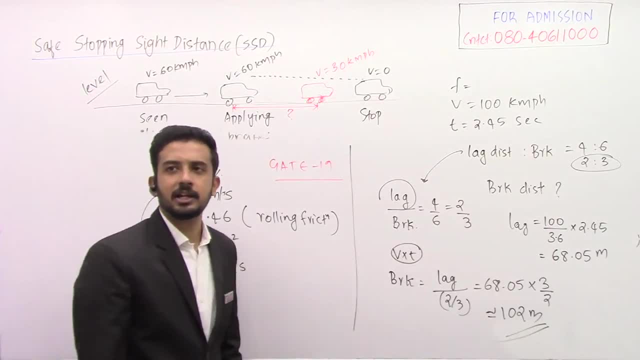 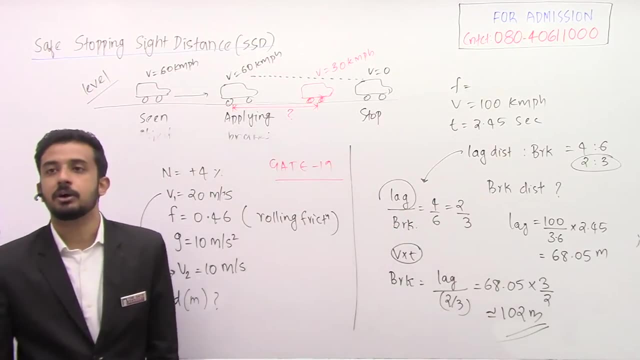 102 meter. very good, so i hope others are also getting the answer right. so in case, if they are giving some coefficient of friction value, don't get confused from the given values or don't think that array they have not given the friction value. how they, how we are going to calculate? okay, so these are the varieties of questions they might have asked. 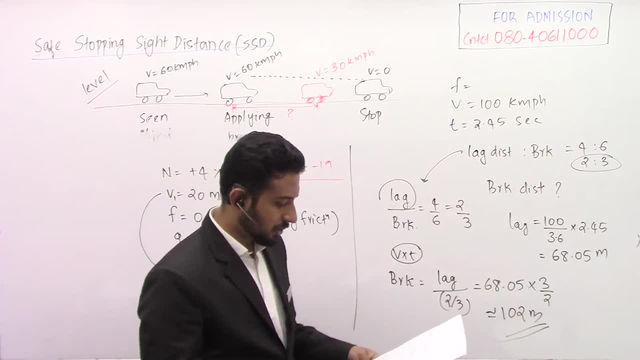 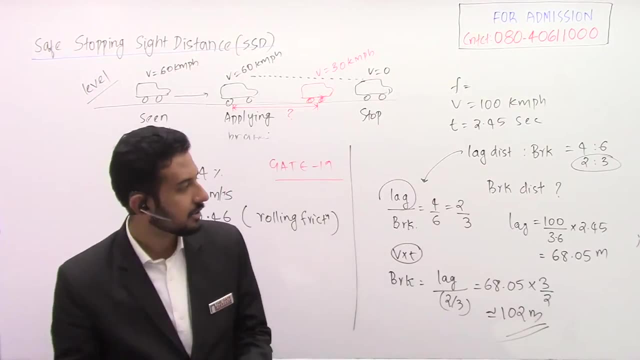 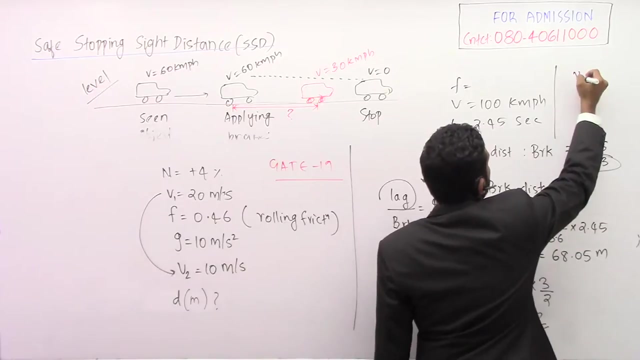 yeah, I told you. 2001 gate question was: what is the equation for breaking distance for an upward gradient of G? if the upward gradient is G, what is the breaking distance? options were: V square by 2 G F plus G. V square by 2 G F minus. 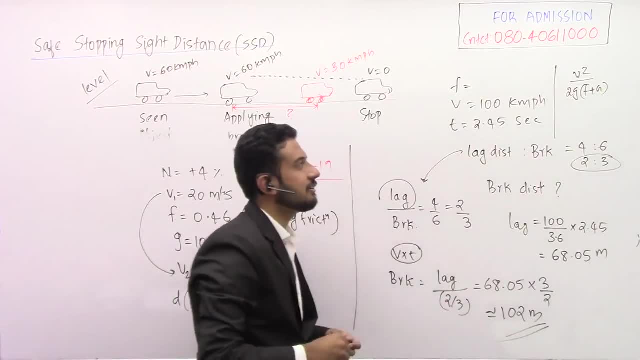 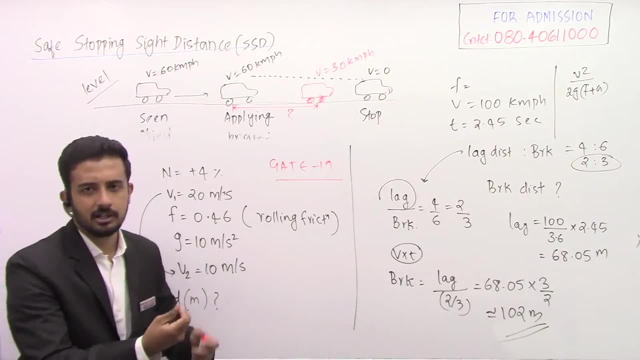 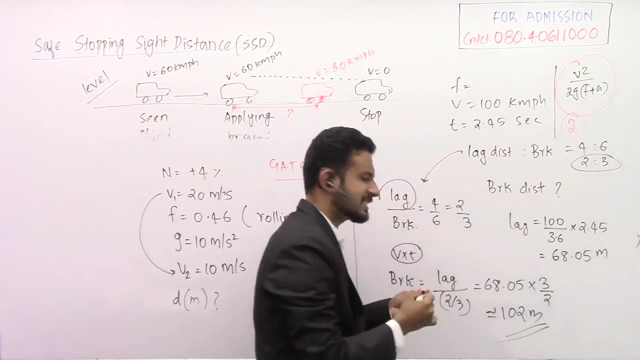 G V by 2 G F plus G, V by 2 G F minus G. what is that V square by 2 G F plus G? this is nothing but our decimal value. I have already told you for how much marks they ask this. for two marks, simply the equation, not even the calculation. so 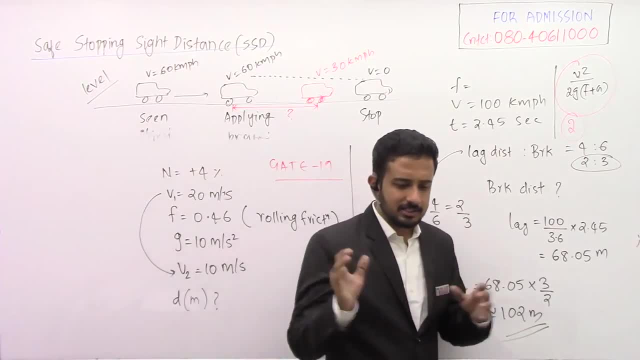 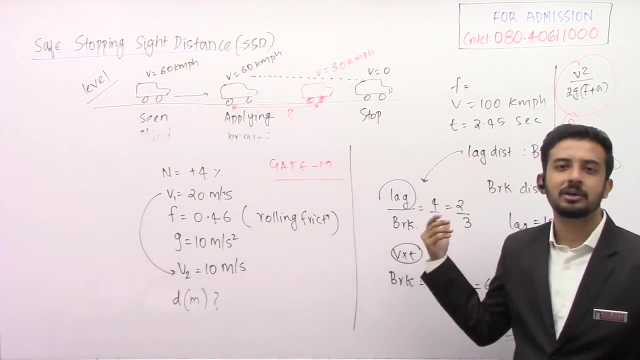 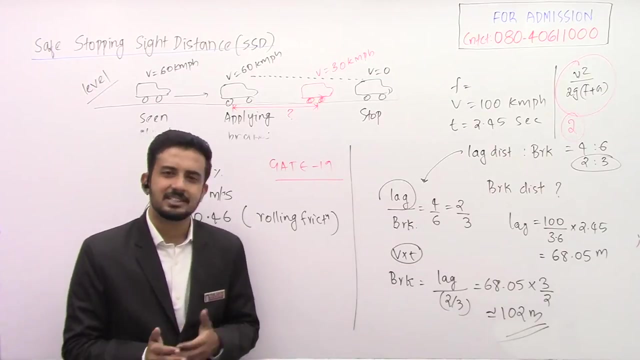 that's why I am telling the concept or the subjects. transportation, engineering is simple and more or less it's a beautiful subject. you easily, you are going to get the score. just imagine if you want to get a two marks from some other subjects. just imagine how much effort you are putting. 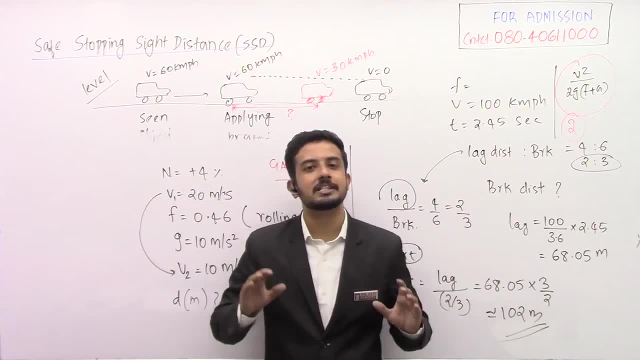 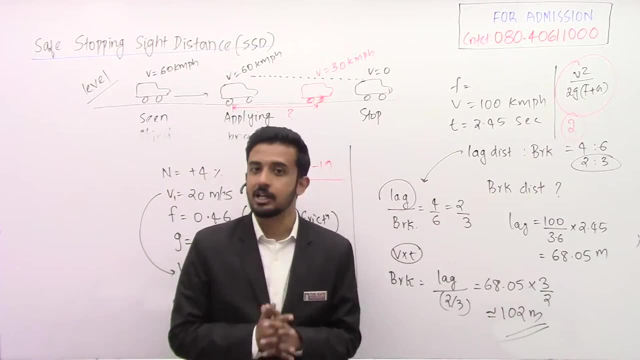 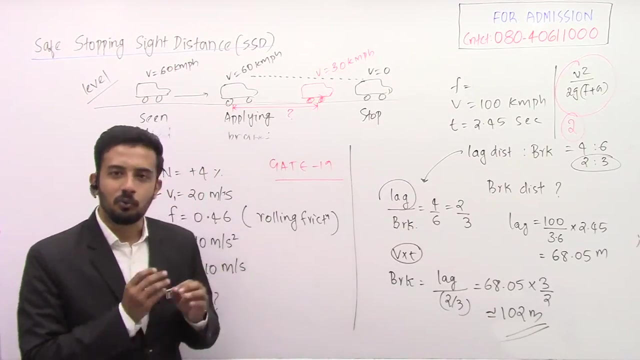 compare. yes, definitely you have to put some efforts for all the subjects to get a good score and to get into IITs or ISE or get into PS use. definitely you have to struggle a lot now. you have to struggle something. later. you will be getting the fruitful result right while struggling. you just have to struggle. 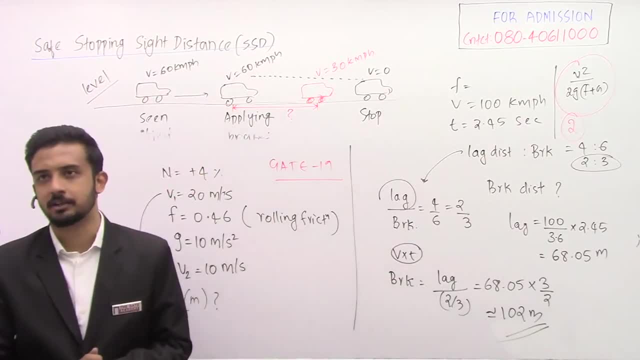 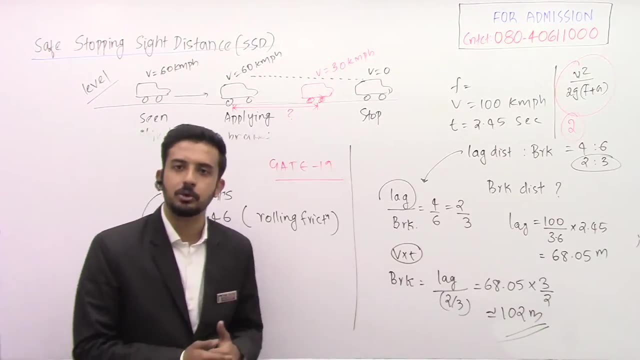 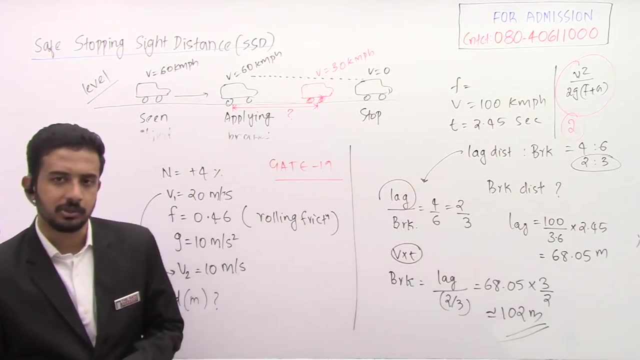 a little bit compared to other subjects for this particular subject. okay, so today we are winding up this session. so from the next session onwards, tomorrow, the same timing you will be getting from 11 to 1 pm. you will be getting the same same timing. you will be getting the remaining portions of geometry design. so 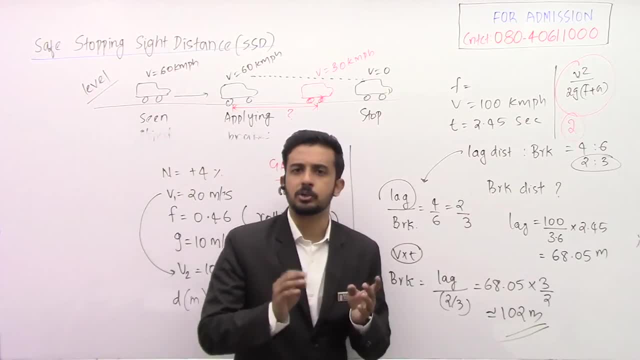 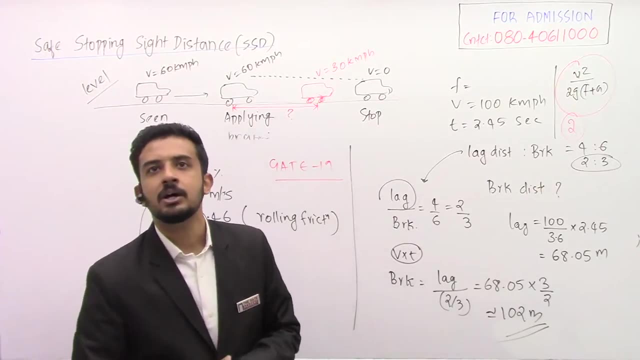 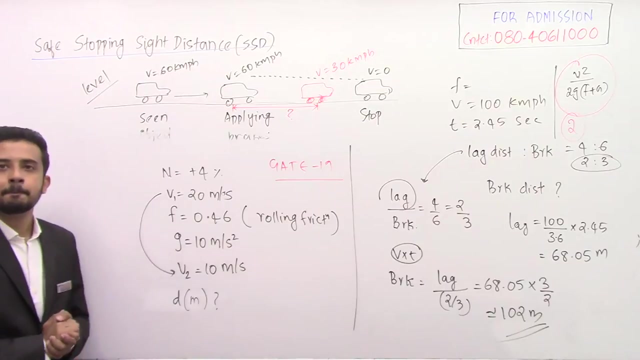 we'll be discussing the overtaking sighted distance in which all portions they can make some twist and they'll. we'll be seeing some other concepts like horizontal curve and all okay. so we are winding up today's session. if you are having any doubt for today's session, you can ask me. we'll be discussing now in it. 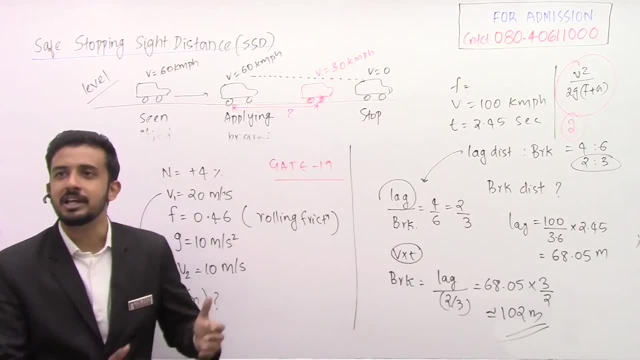 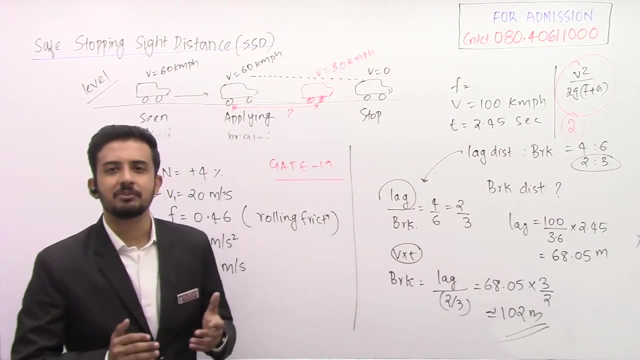 out? or again, how was the class? or should we do anything more or less? yeah, that's one more. one of the important thing: just share the link with your friends also. and if you are sharing with your friends, don't forget to subscribe to my channel. don't think that array, he will also listen. hey, you will also get the marks. 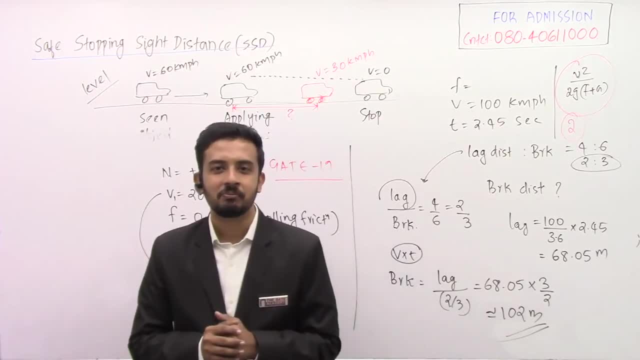 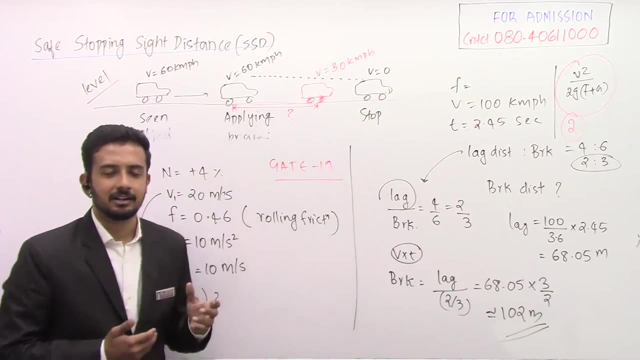 don't think that if you're sharing, you're doing some good thing. finally, the God will give you the result. okay, you will be getting some good marks if you are helping others also. okay, so share the link with your friends and the timetable of the remaining sessions- everything you will be getting. so 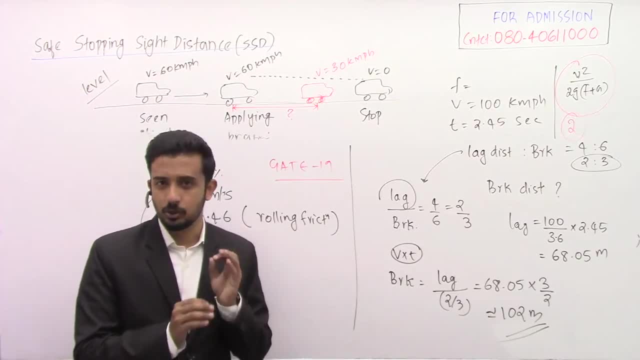 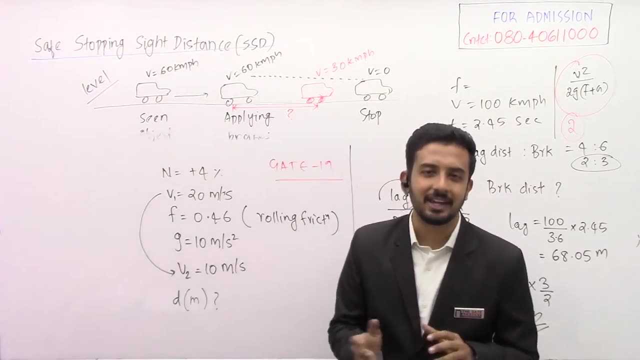 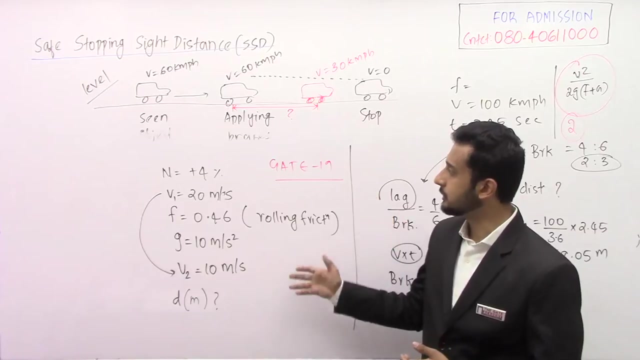 subscribe the channel and click on the bell icon so that you will be getting the instant notifications. okay, you will not be missing. sharing is caring. absolutely well, that's it. if you are carrying others, definitely the almighty will care about you also. okay, so share with your friends and, uh, go through the things. 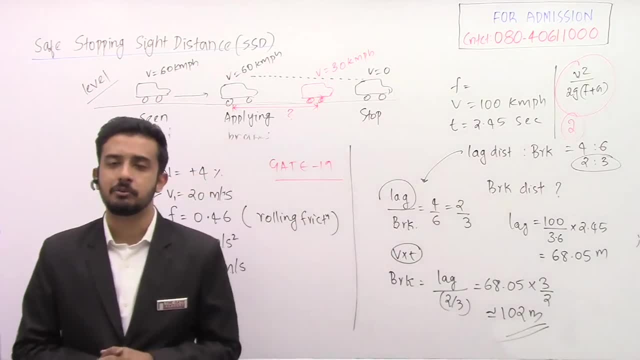 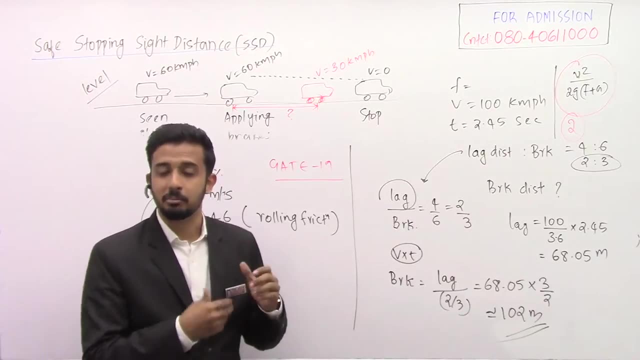 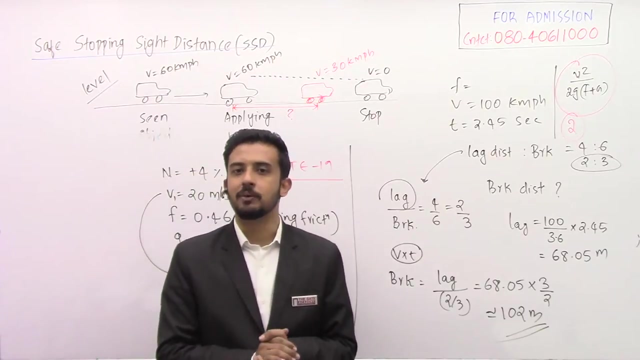 and yes, regarding overtaking sight distance, I have already done a video. it is available in our channel- regarding the minimum overtaking sight distance. you can go through that for better clarity so that in the next session tomorrow you'll be easily able to solve the questions. okay, so there is already a video available on minimum overtaking sight distance. 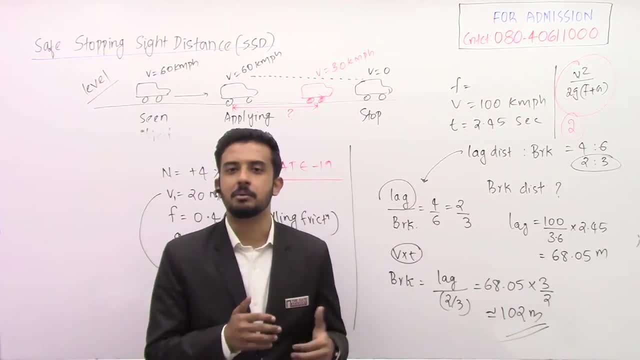 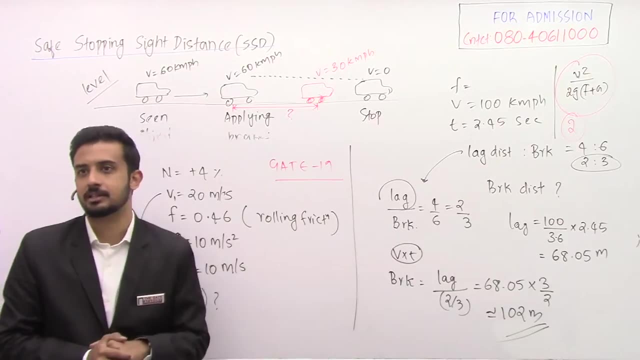 the gate academy channel. go through that. the it has taken by me only so you can go through that. it may be a one hour session. go through that. you will be easily getting whatever things we are going to discuss in the next class, okay. so thank you, john, for your comment. so we are winding up.